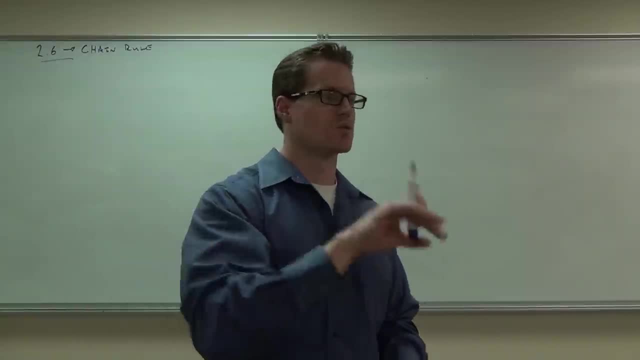 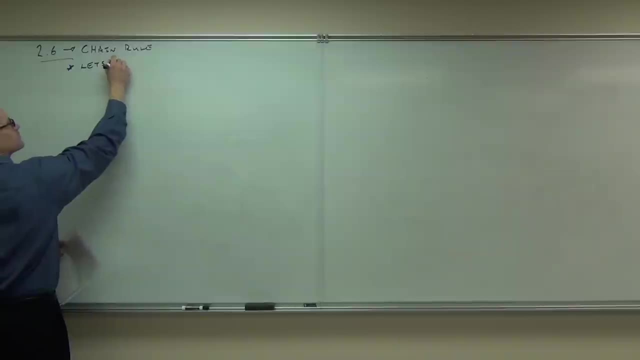 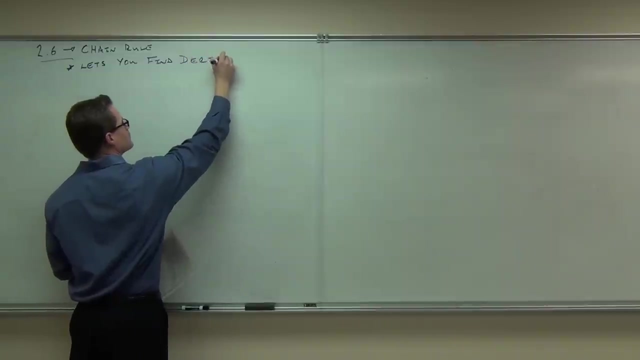 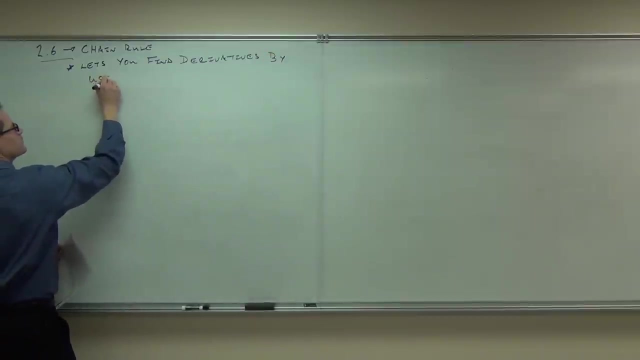 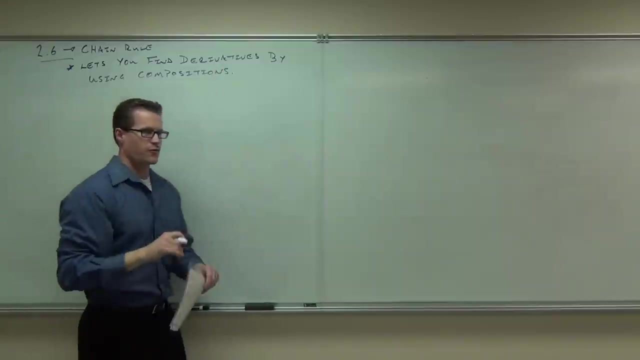 So what? this is what the chain rule does. it gives you a way to do derivatives with compositions. So it lets you take derivatives by using compositions And just to refresh your memory on why we might do this, I'll give you that example again. 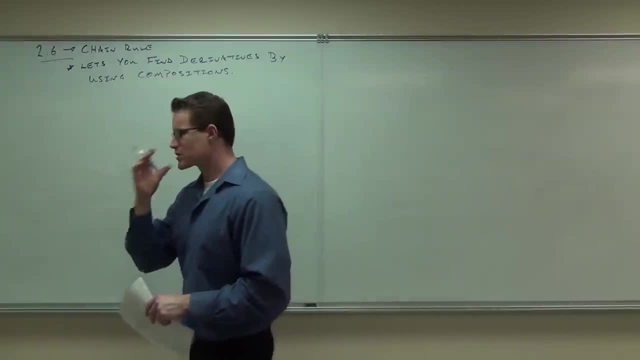 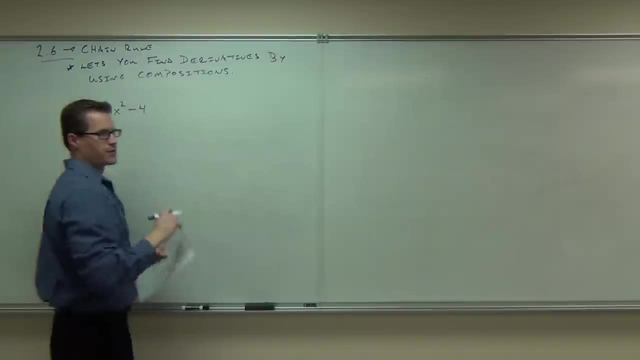 It's on the last video, so I want to make sure it's on this one as well. This is the reason why we want to learn the chain rule. I gave this to you earlier. I said: can you take the derivative of that thing? 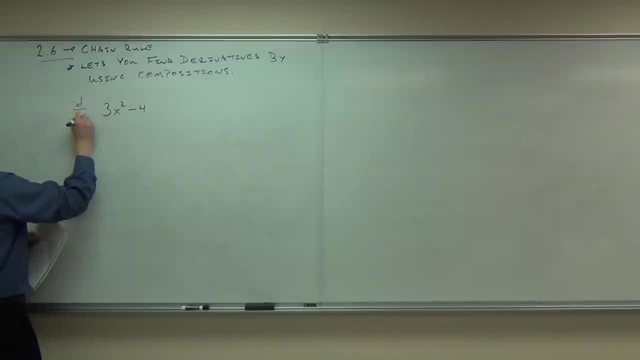 Easily. In fact, if I did this, derivative would be 6x, and then you're done, right. And I built on it a little bit. I said, okay, well, what if it's not that? What if it is squared? 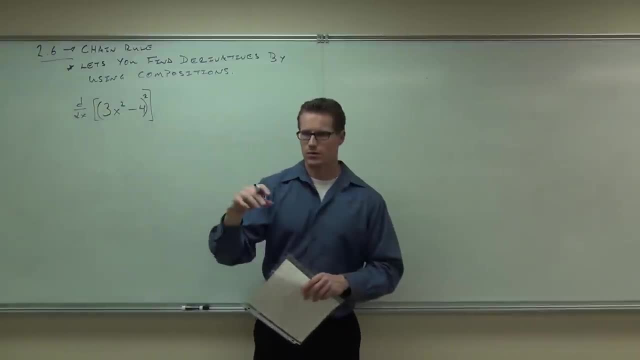 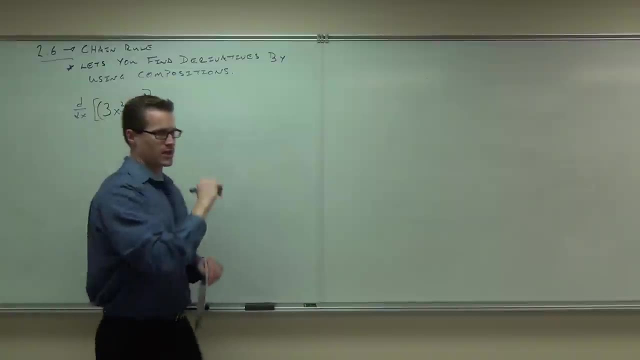 Could you still take the derivative? And it says, yeah, you probably foiled it out, So I distribute it and then take it term by term. I said, okay, well, what happens if it's cubed? And you go, I could still do the same thing. 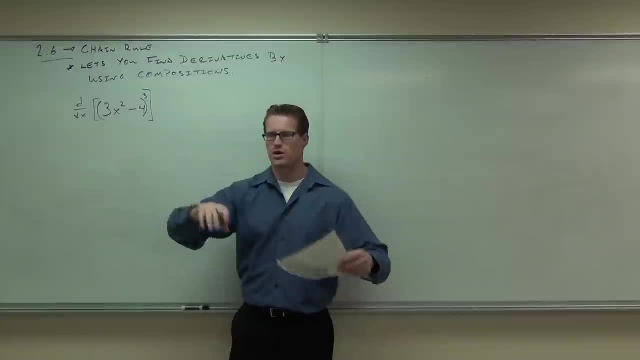 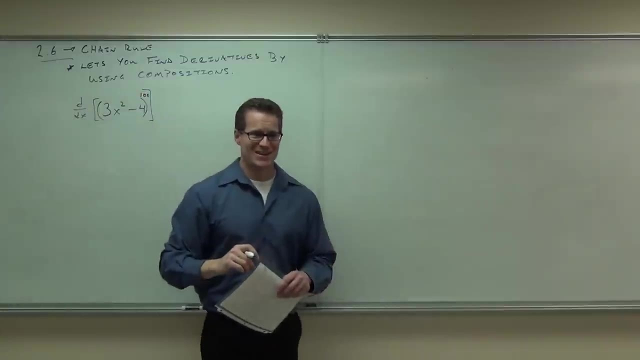 Or I could use the product rule. I could still do that- Distribute one of them, use product rule. But as soon as we get to things like this- and I think this is where I went- the oh crap, right You go. come on, man, are you serious? 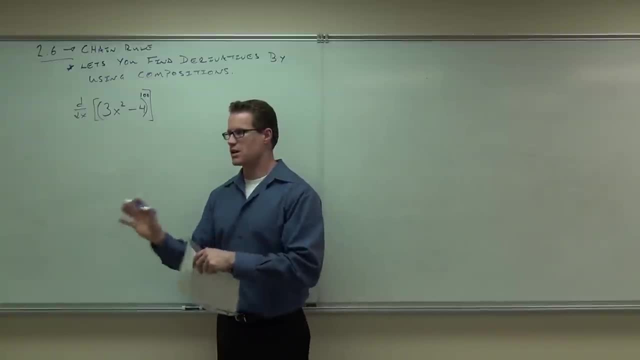 Do we really have to do that? Yeah, But if you think you're going to distribute this 100 times, that's just a waste of time. So there's got to be a better way to do derivatives of this, And, as a matter of fact, there is. 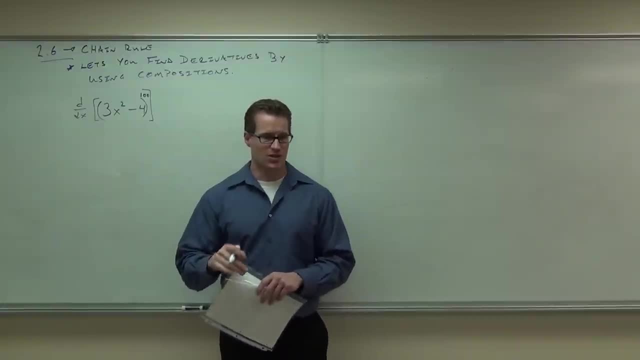 And it's actually not hard. It's kind of an easy way to do it And you're going to like this. So all the times where you had to distribute, remember like when you had this squared, you had to distribute that right. 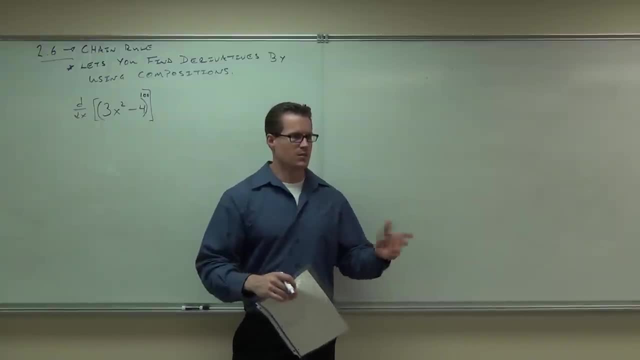 Like in the first set of homework, you're like: oh man, this is tedious. Well, end the tedium. Now this takes care of that. So any time you can see a composition, I'm going to show you the composition here in a second. 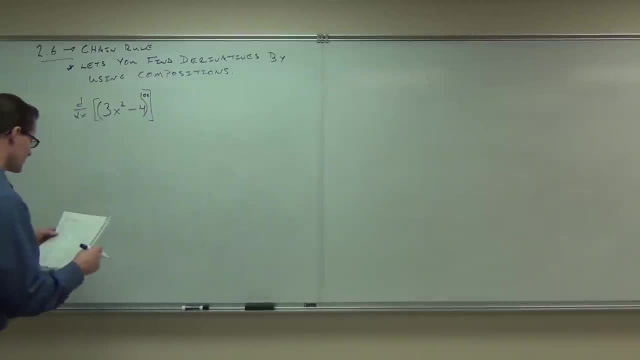 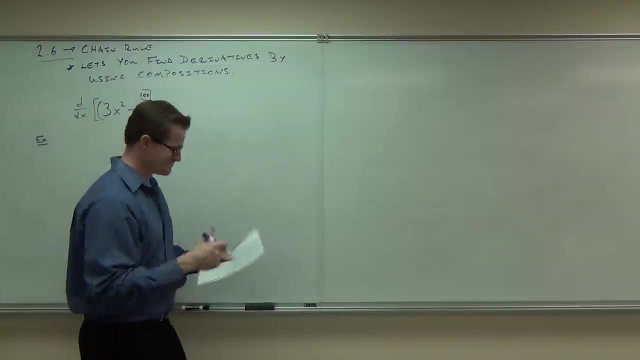 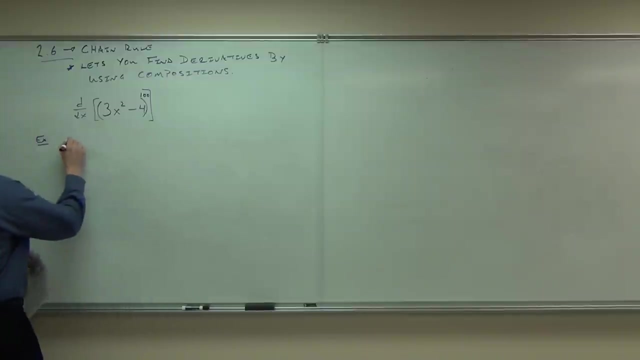 you can use the chain rule. So I come with theme music now. All right, The question is: can I express this thing as a composition? Which is why I had you cover compositions and had you go with the reverse of compositions: looking for a function within a function. 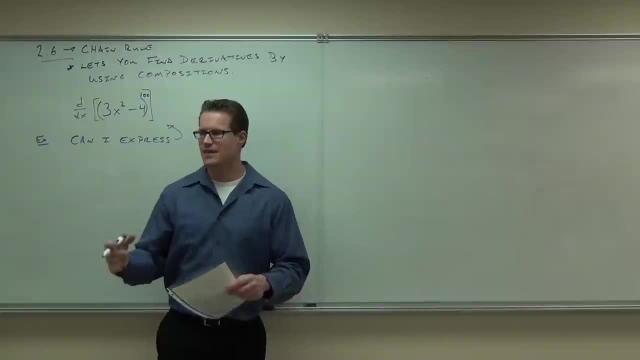 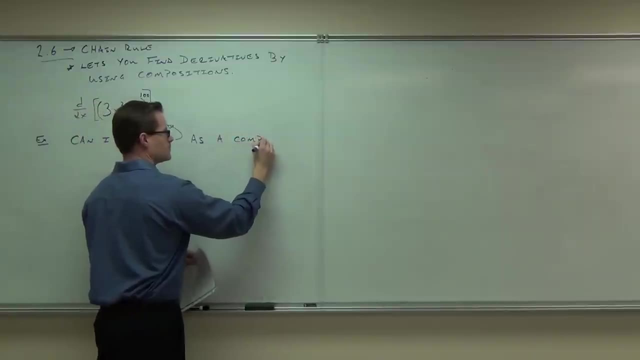 That's why we did that. So when we get to this point, like, oh yeah, I kind of understand that idea now, So Can I express this as a composition? And the answer is yeah, I can, And here's how you do it. 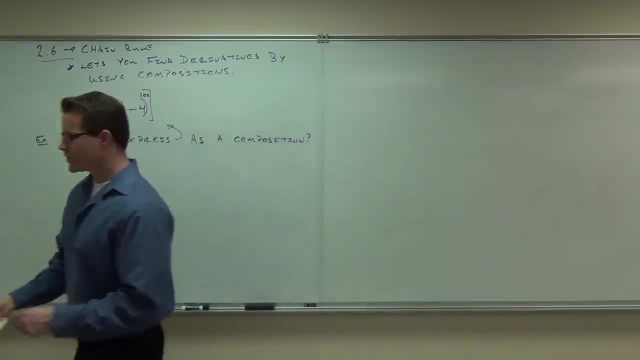 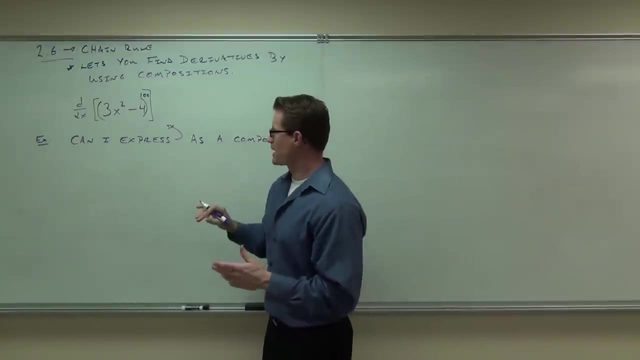 Here's a pretty basic way to do these things. What you're going to do, you're going to cover up the inside of your function. So what I mean by the inside here is the 3x squared minus 4.. You with me on that. 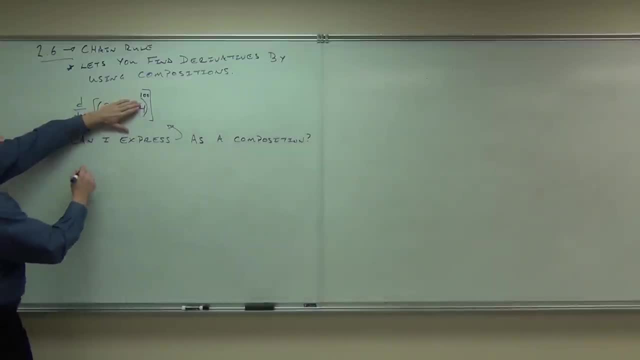 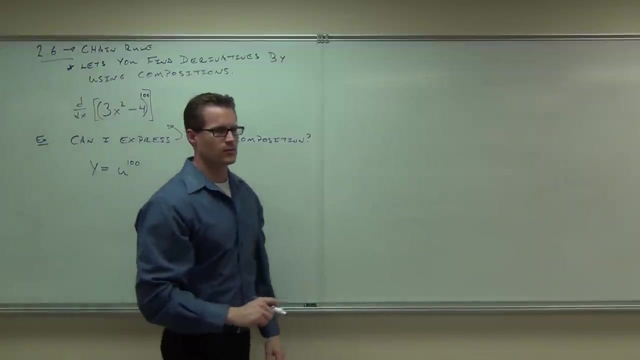 You're going to cover that up And you're going to go: okay, I'm going to make a function. y, equal to whatever you covered up, becomes an x. Like you know what. let's make it a, u, A, u to the 100th. 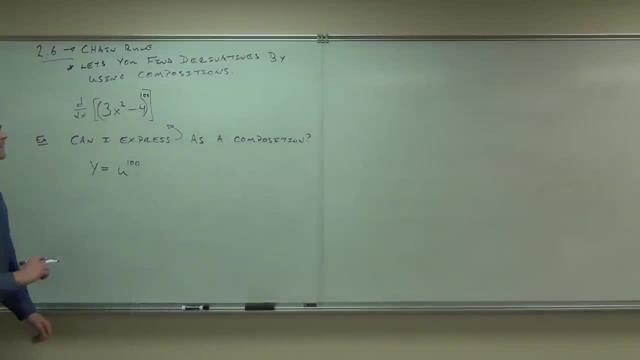 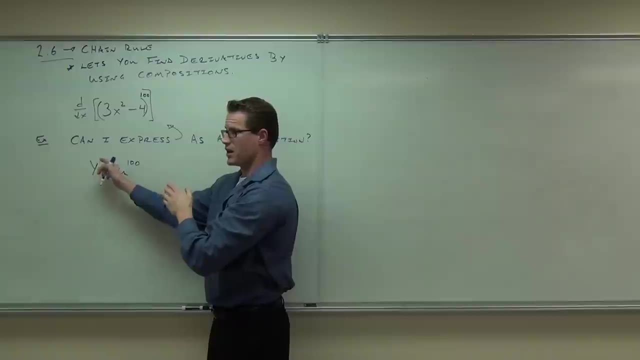 Make it a? u to the 100th. Do you see how I got that? Do you see that by holding this part out I get a function that's very basic. y equals u to the 100th. Do you see where the? u to the 100th is coming from? 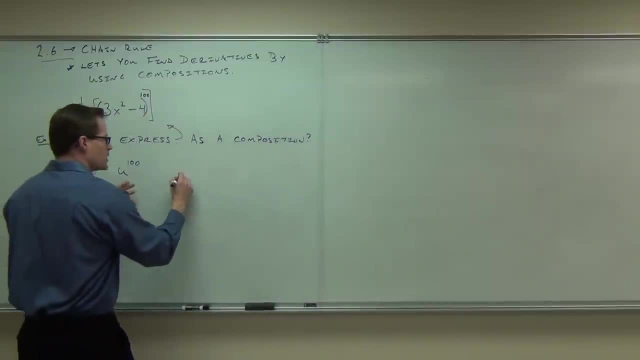 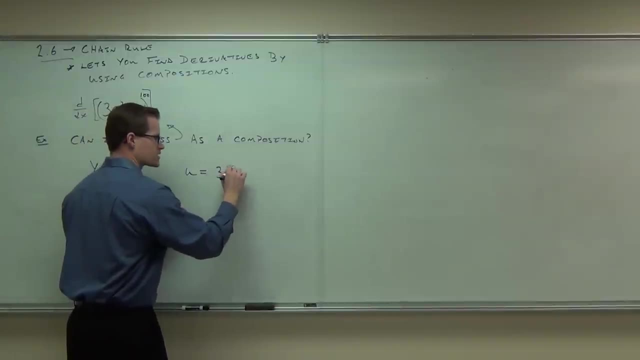 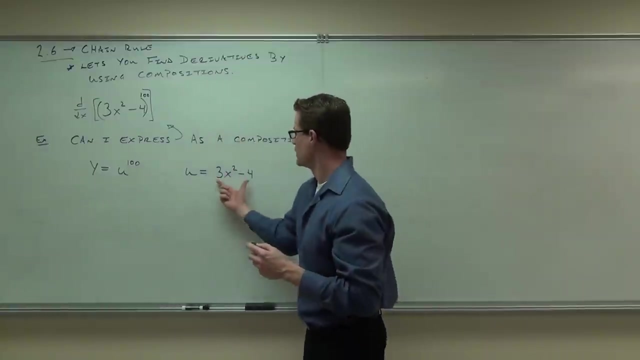 But then you have another function to express. You now need to say, okay, well, u is going to be what did you cover up? And that has to be your u And that would be a very basic composition. Do you see if I put the u in for this u? 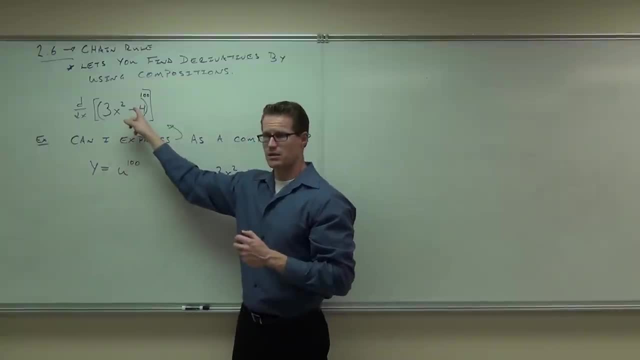 this expression for this u. I'm going to get that back again. Can you see the composition here? If you cover it up, you go- okay, that's u to the 100th and u is what's under my hand. 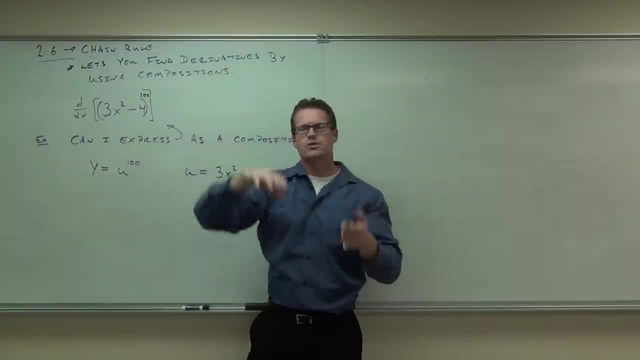 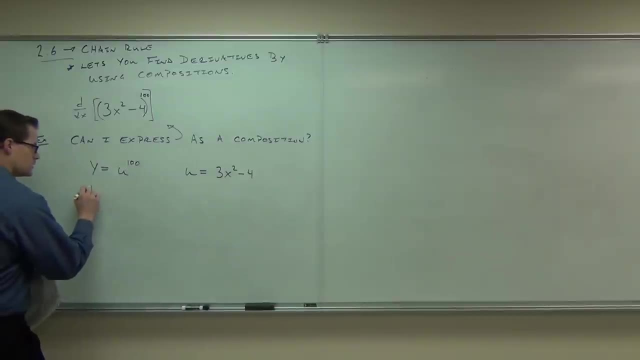 And that's how we get those two things. Rich, are you going to be okay with that? so far, So sure. this is a composition That's not bad at all. Well, could you find dy du? Could you find that? 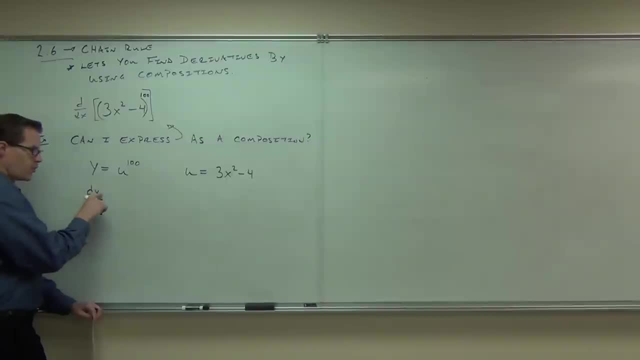 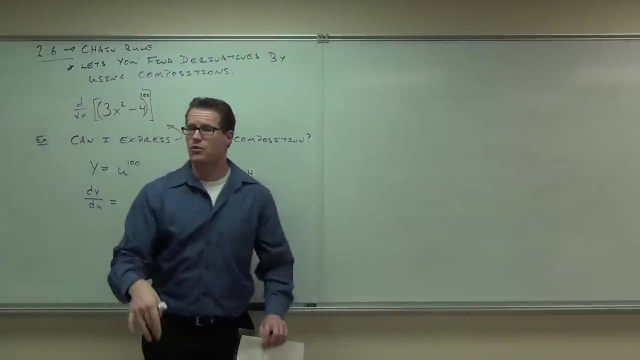 What's this mean to do? Derivative of y with respect to what? Oh with u. Okay, so do it. What's the derivative with respect to u? That should be a very easy one for us. 100 u to the 99th. 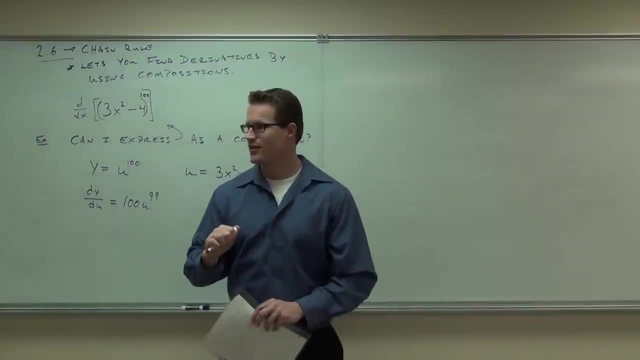 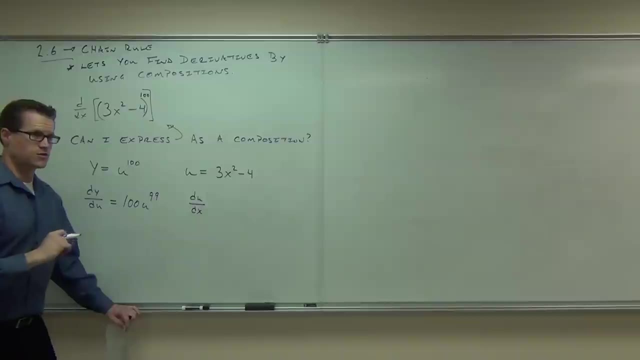 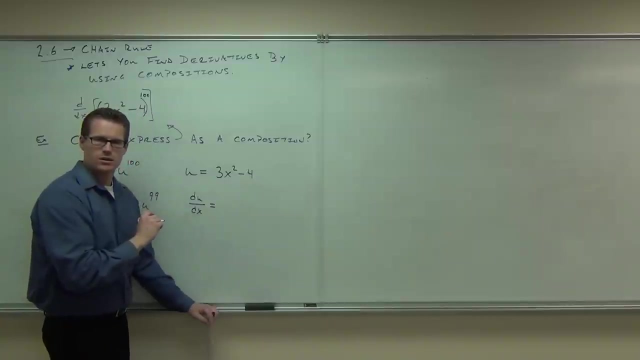 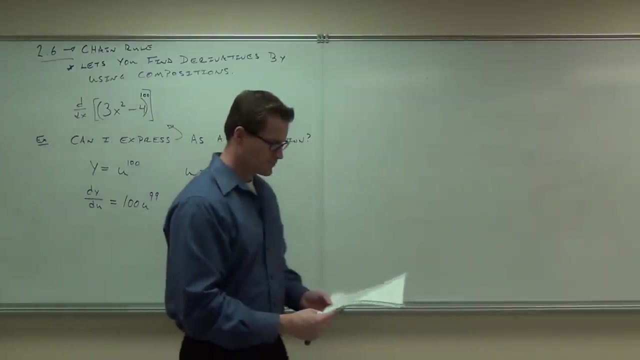 You okay with that so far? You sure Okay. Could you find du dx? Could you find du dx? That's the derivative of u with respect to x. How much is that going to be? That's the 6x. Are you okay with these two things so far? 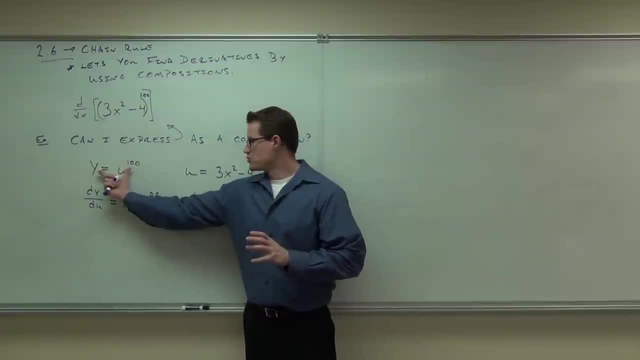 So we write this as a composition. We take the derivative of the first expression, That's the overlying function. We take the derivative of the inside expression. That's what we chose as our composition to compose into that. But the problem is this: 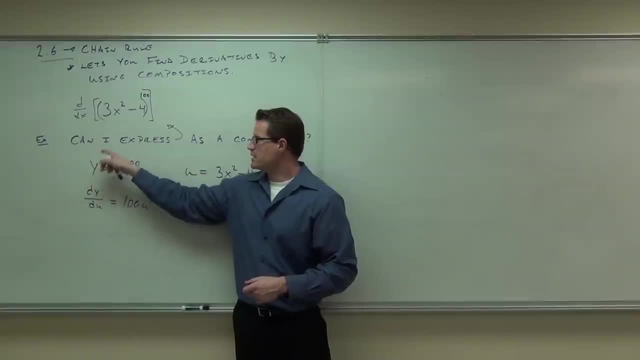 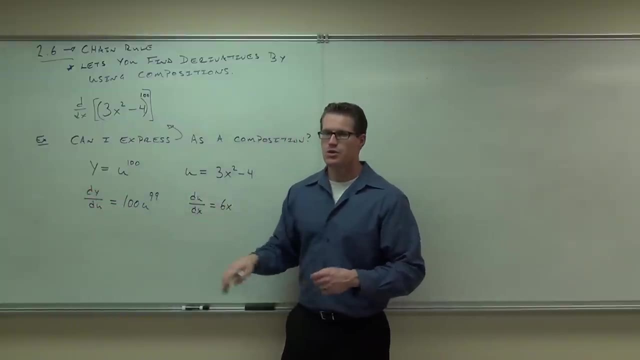 What we ultimately want to find is dy dx. right, We don't have that yet. We have dy du, We have du dx. But you're going to find out right now why we stick with this notation, because this is kind of cool. 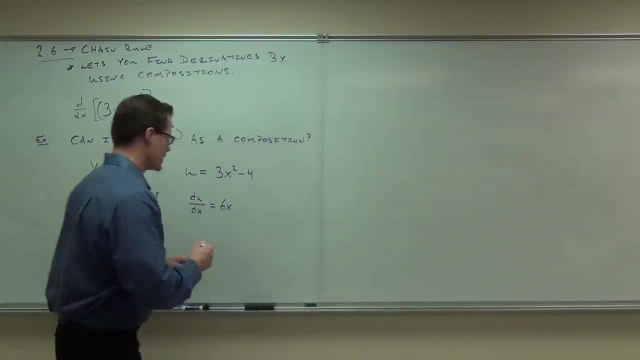 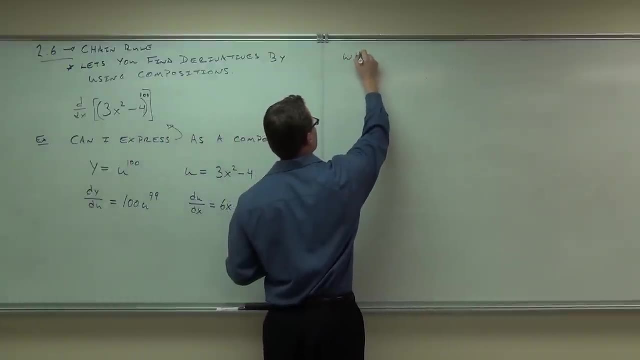 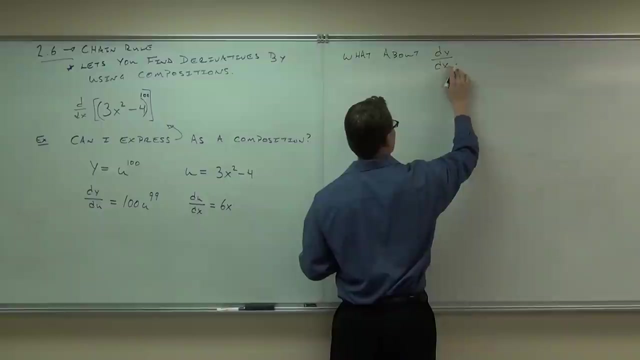 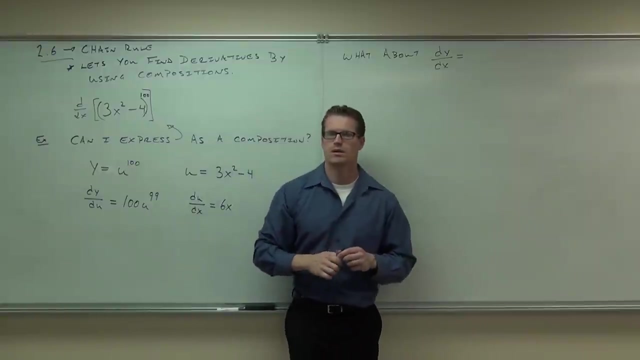 Are you ready for it? If we want to get dy dx, so what about dy dx? The question is, can we put these two things together in such a way that it will equal dy dx? For instance, I'm looking at a dy du and I'm looking at a du dx. 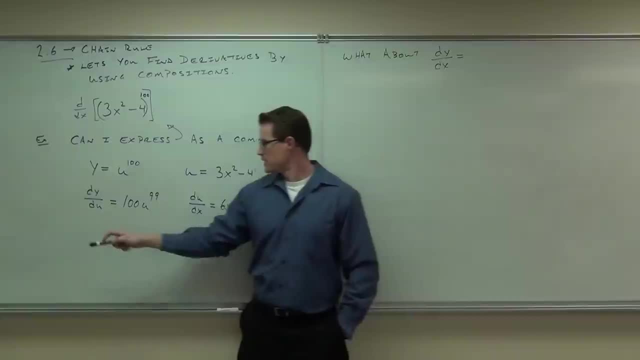 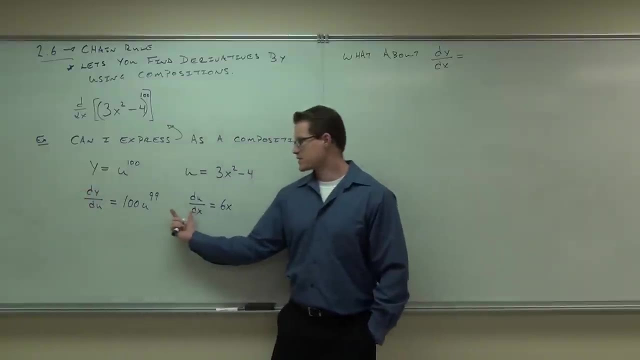 Do you notice how the du here is on the denominator and the du here is on the numerator And we have a dy on the numerator which we want and a dx on the denominator which we want? What operation can I put between this one and this one? 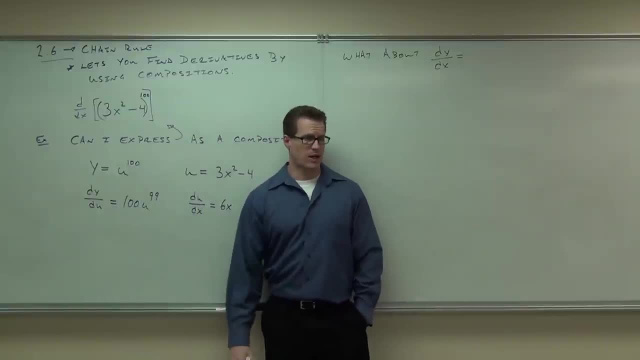 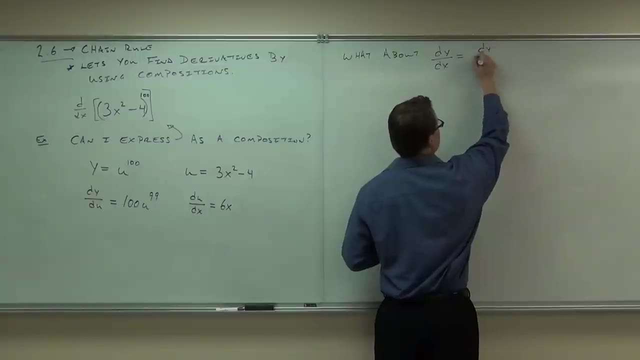 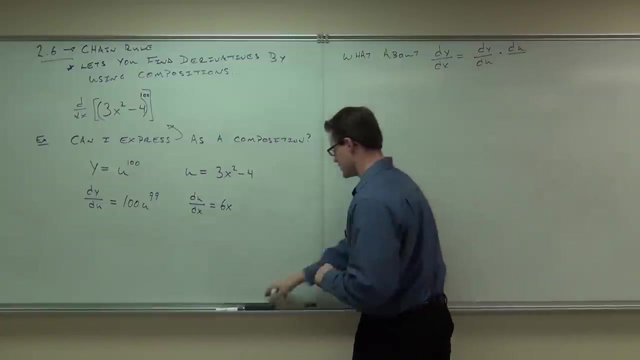 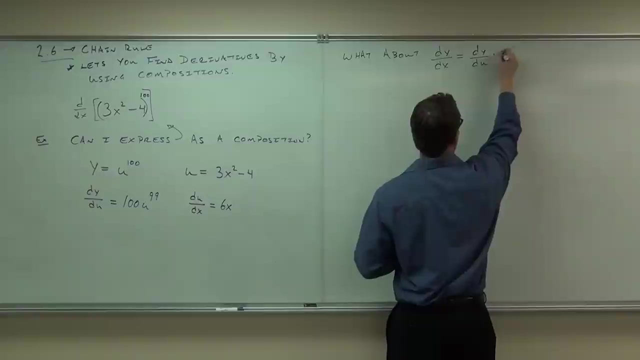 Okay, I'm going to put this one, so the du's will be gone and I get dy dx. You know what? Look at this. If I say, well, let's just take dy du, Let's multiply it, That was like an a, didn't it? 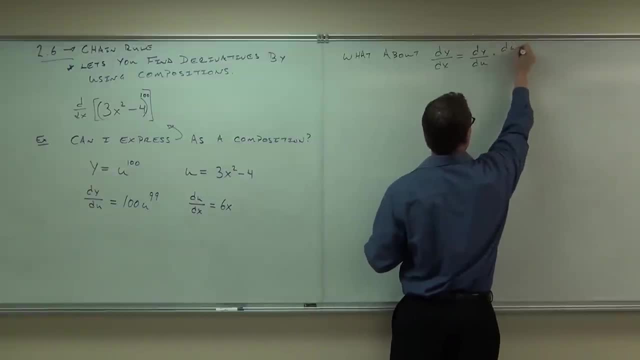 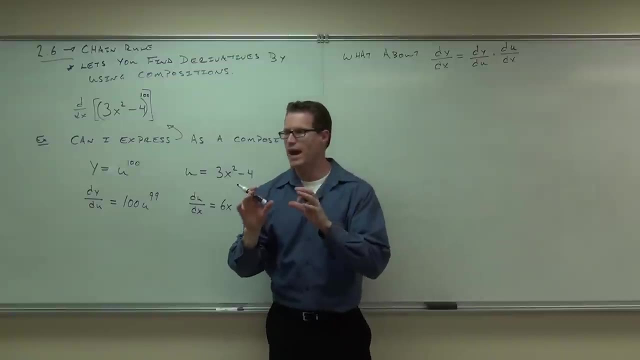 Let's multiply it by du dx. The beauty of this notation is that those little pieces do act like something you can cross out, something you can simplify. So what happens to the du's? in this case, They're gone. This right here is the chain rule. 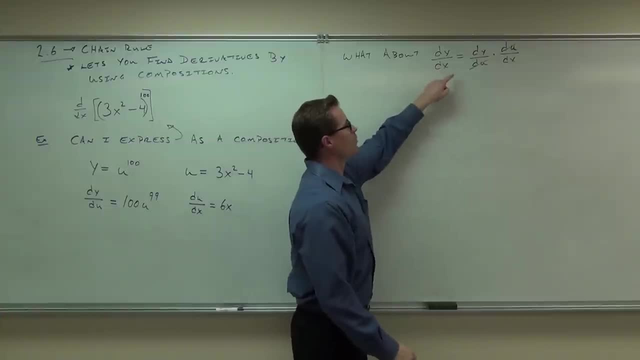 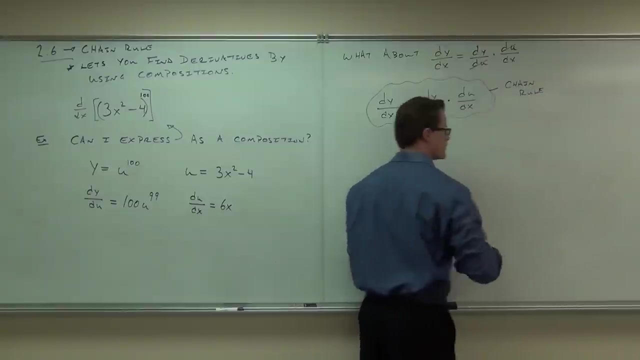 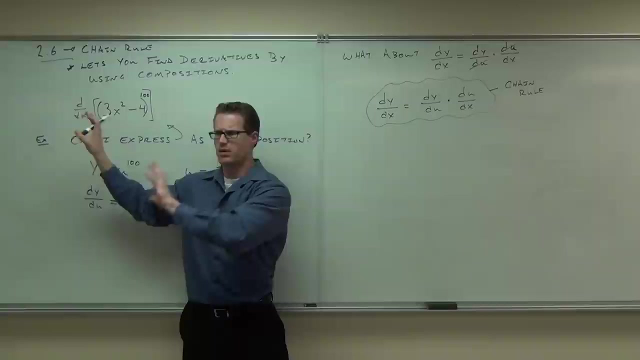 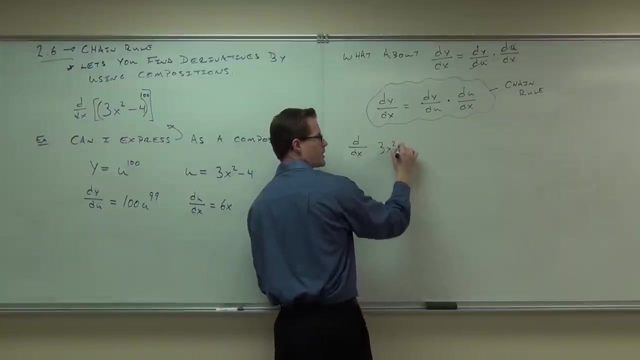 What it says is that dy dx will be equal to dy du times du dx. This is chain rule. That's the chain rule, Okay? So how do we use it in practice? Let's apply it to this scenario. okay, Let's ask you for d dx of 3x squared minus 4 to the 100th power. 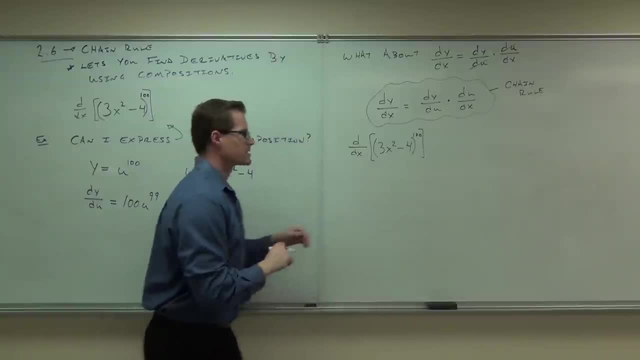 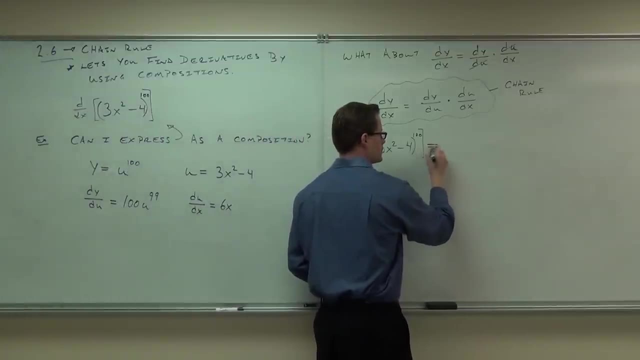 Who cares where you got that from. Can you do the derivative? Here's what it says. It says: take your dy du. Take your dy du. That's this Okay. I'll substitute that way: Take your dy du times your du dx. 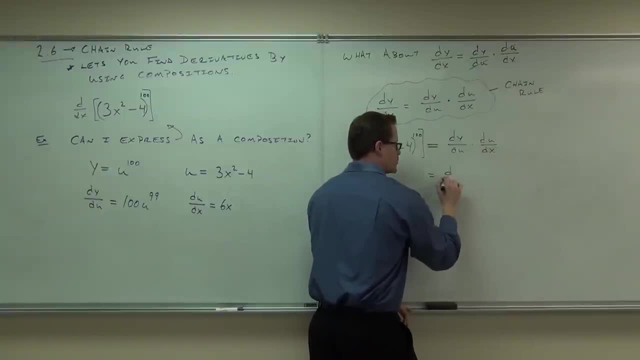 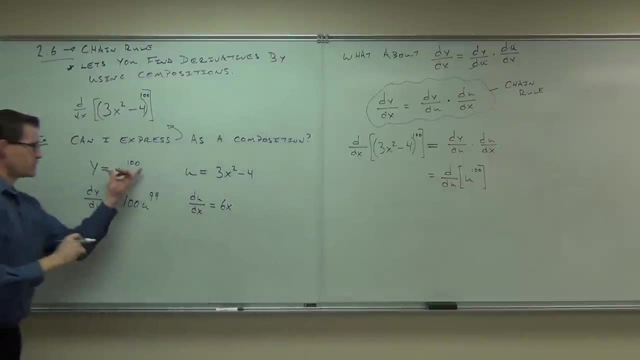 In our case, that's the derivative with respect to u of u to the 100th. That's where we got this right: Derivative with respect to u of u to the 100th. Are you seeing where that's coming from? 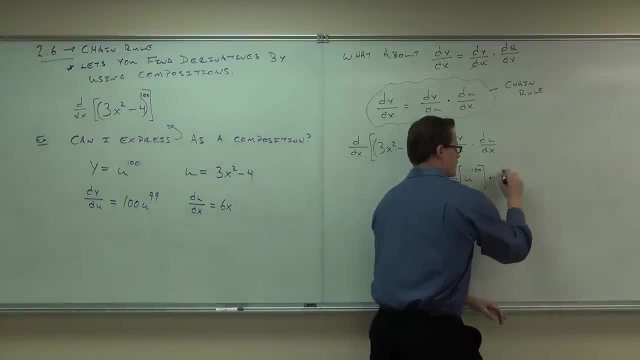 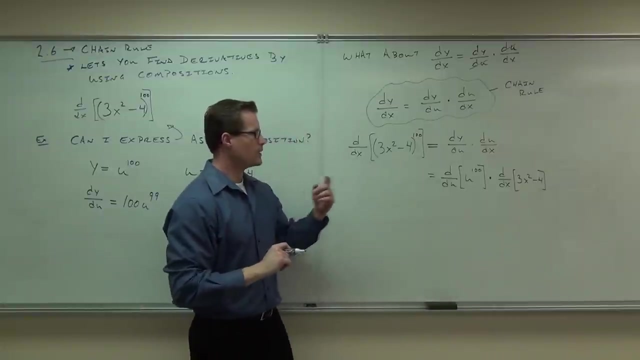 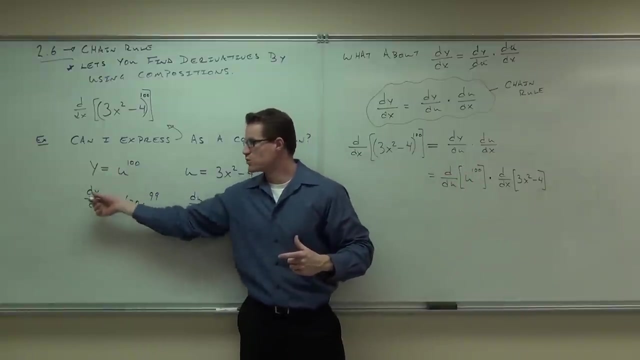 Then it says: times the derivative of the inside, the 3x squared minus 4.. That's the du dx. Do you see that dy du is this thing. It's the derivative of your function with respect to u. That's what this part is. 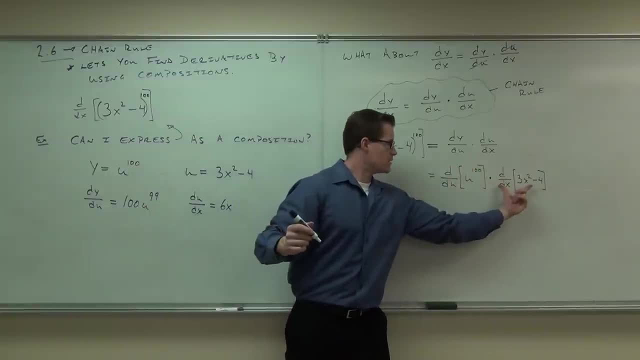 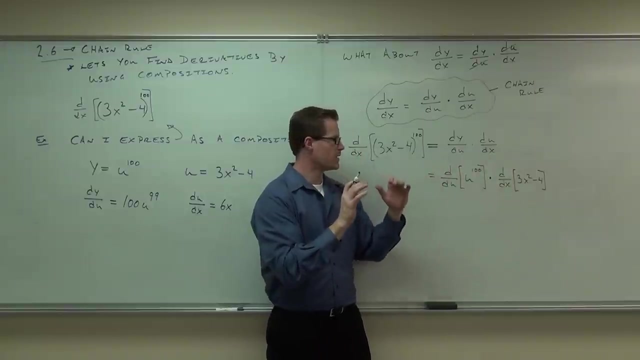 Are you okay with that? The du dx, that's the derivative of what you call u. The derivative of what you call u is the inside part. If we take that derivative, it says: multiply dy du times du dx. So take the derivative of the overlying function, multiply it by the derivative of the inside function. 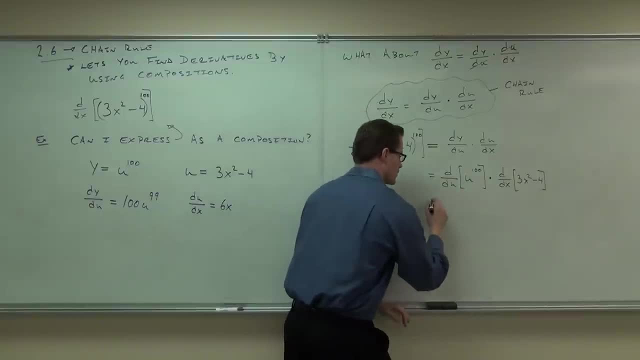 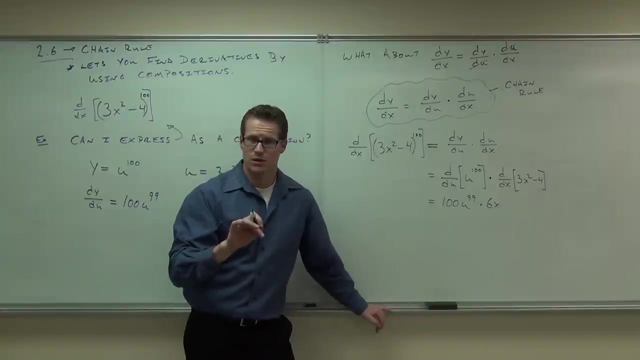 That's what this says to do. What was this again? Times? what was that again? Do you see a problem with this? Yeah, we have x's and we have u's. We want which one? We want x's. Do you know how much u is equal to? 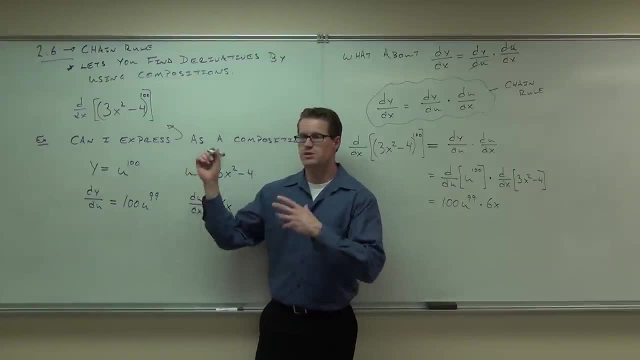 Sure, that's why you had this over here. So if we can do that substitution, we go. okay, the x looks great to me, but the u doesn't look so great. I want to make that u back into what u equals. 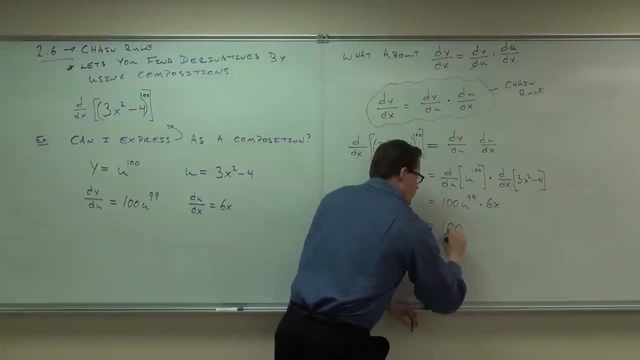 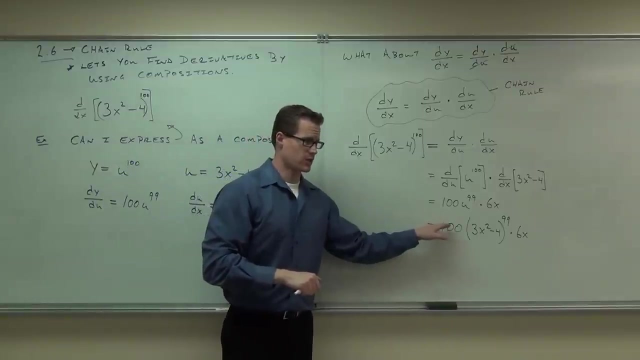 So let's do that. We'll get 100, 3x squared minus 4, because that's our u to what power? Don't forget about the 99th power. What's the exponent Times 6x? Now you could make it a little bit prettier, but I want to come back to this and talk about this for a second. okay. 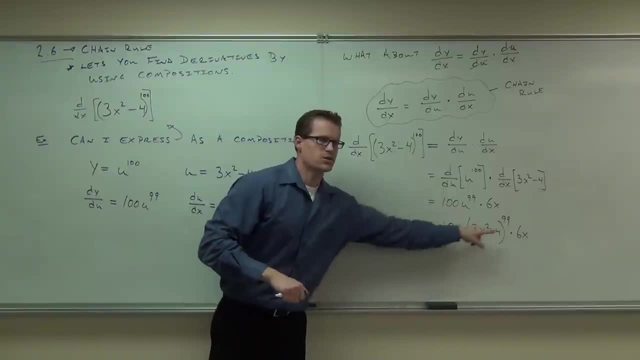 because I want you to see the practicality of the chain rule. Firstly, what are you going to do with this? You're going to do something with this. What are you going to do with the 6x? Multiply by what number? 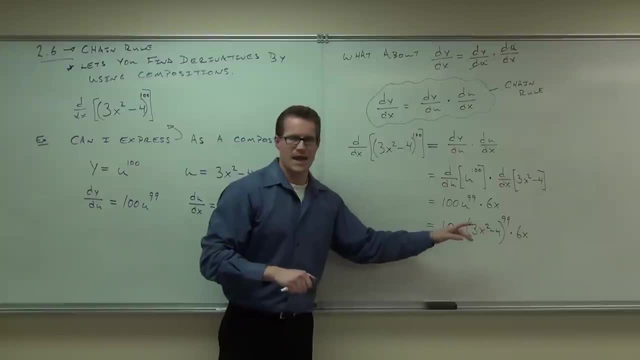 100.. Yeah, do that. Okay, don't leave it hanging out there as a times 6x at the end. Please, please, don't do this. Don't distribute the 100.. Okay, you can't do that because that's the exponent. 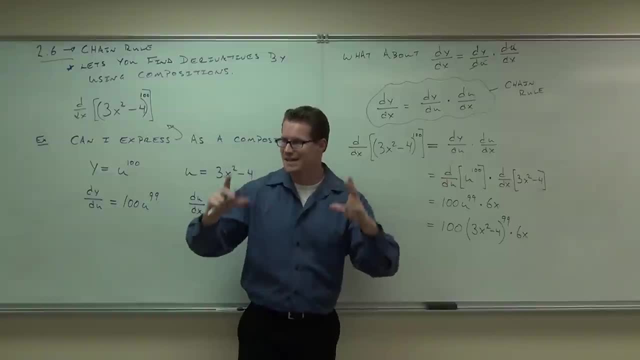 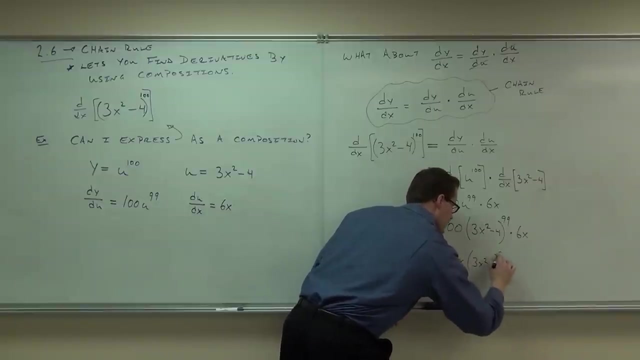 That says, in order to distribute the 100, you'd have to FOIL that out 99 times. Did you get it? Please, for heaven's sakes, don't do that. All right, don't do that. Just multiply this number, times this number, and we get 600x. 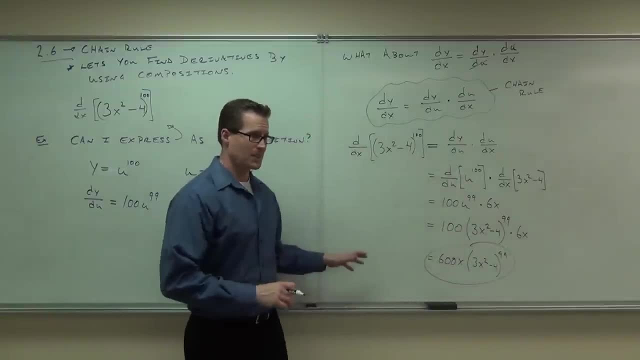 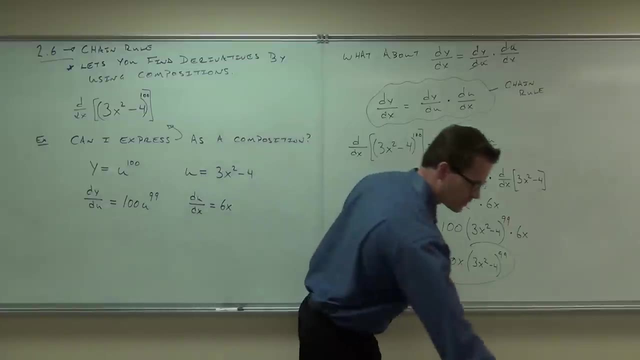 3x squared minus 4, all to the 99th power. That's it. That's a pretty easy way to do a derivative, isn't it Not too bad? Now let's look at what actually happens here, because I want you to see this. 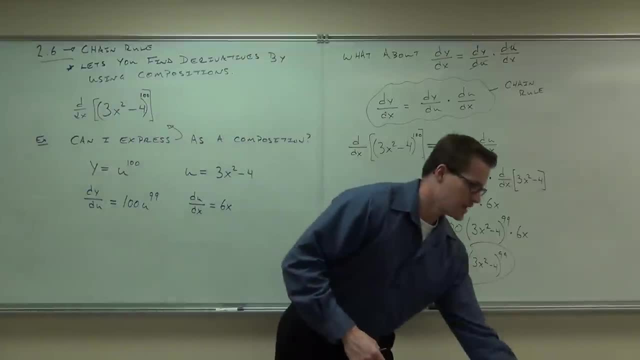 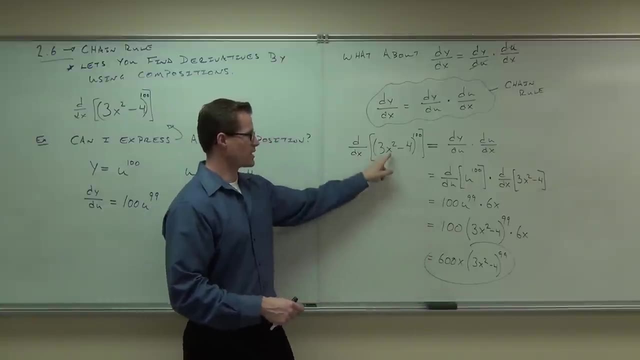 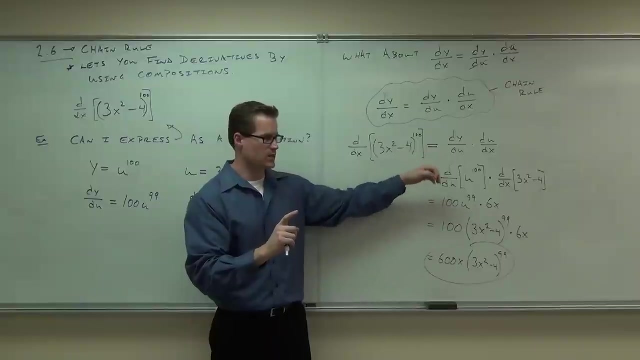 This is going to be, in general, what we did. Is there a way that you can get from here to at least- well, actually probably this step? We can get almost from here to here in one step, without showing a u, without showing a du dx and a dy du. 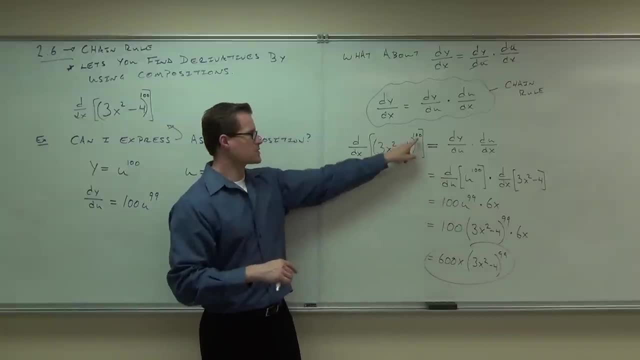 Without showing that stuff. I want you to think about what we're doing. Do you see what happens to the 100?? What happens to the 100?? Power rule. Yeah, that's basically just your power rule, Do you see it? 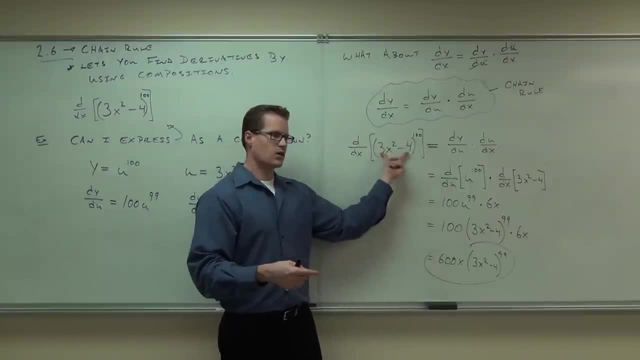 The 100 comes down to the front. You leave this thing alone. right, That's in the parentheses. It says you leave it alone. Why do you leave it alone? Because you end up substituting back in the u. That's why. 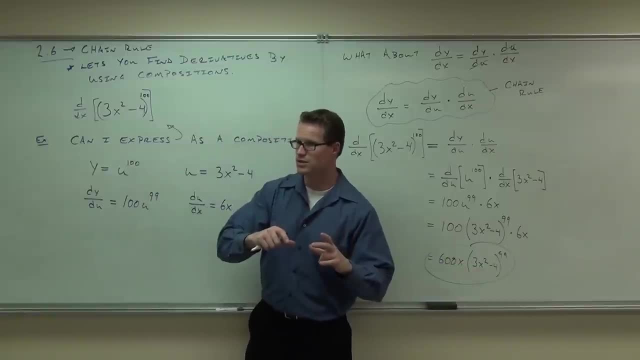 Because of the composition. you're going to get that u back again. Do you see that? You're going to have some u here? You're going to get that. So we have a u back again. That means you don't change the inside. 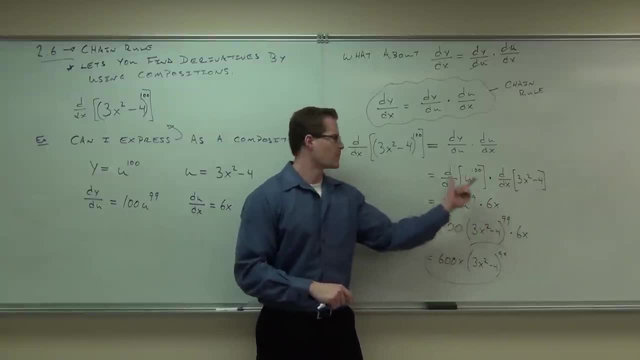 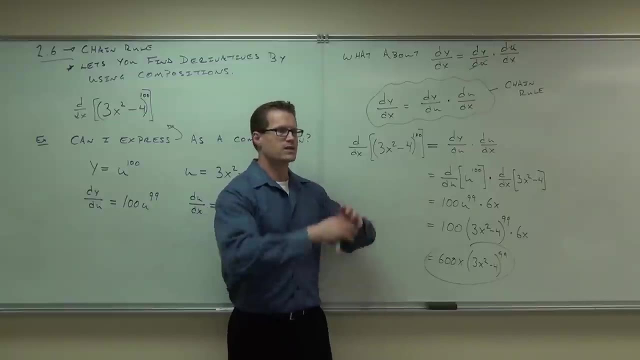 Where does this piece come from? Where does the 6x come from? Yeah, And this is called the general power rule. It's a corollary of the chain rule. The chain rule is the overall arching idea, But what we can do oftentimes with this is something called the general power rule. 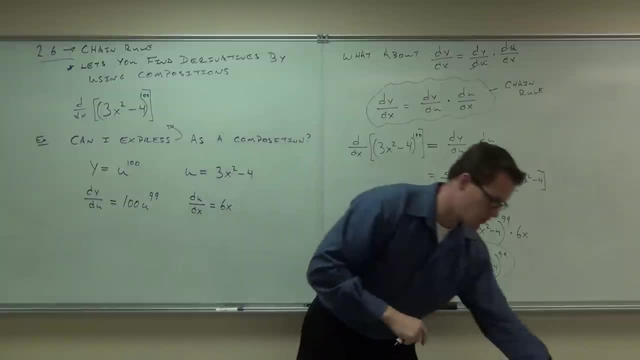 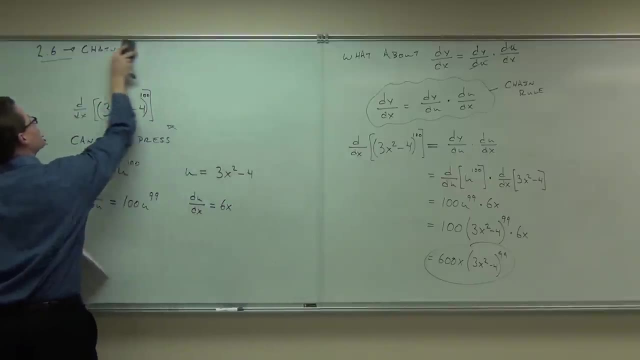 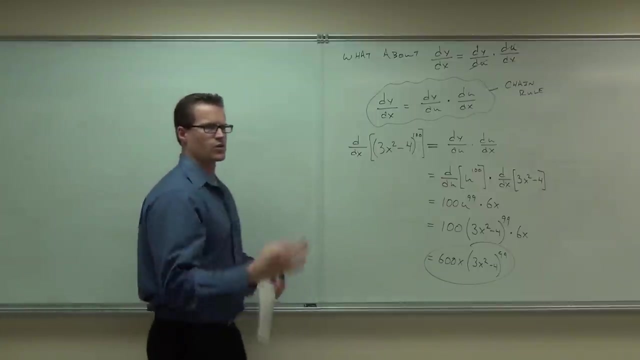 And it says: the power rule works in general. if you do this, And I'm going to show it to you right now: So, general power rule. So when you ask me, I thought you said there's only three rules. There really are. 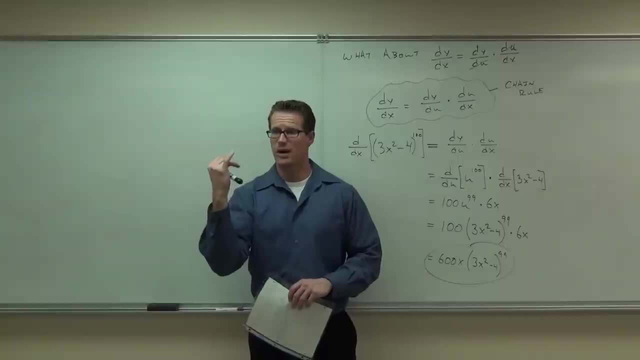 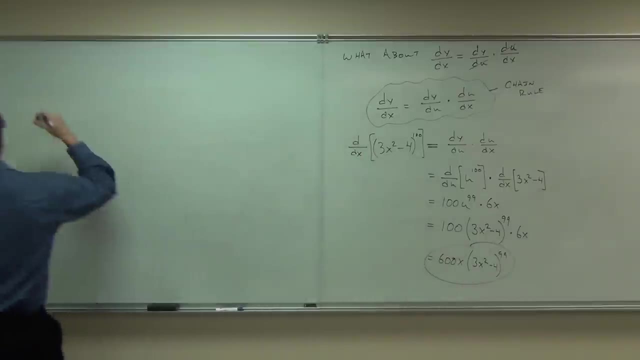 There's only the product rule, the quotient rule and the chain rule. However, the general power rule is like a little piece of the chain rule. You get the general power rule from the chain rule. Do you understand? So the general power rule says: 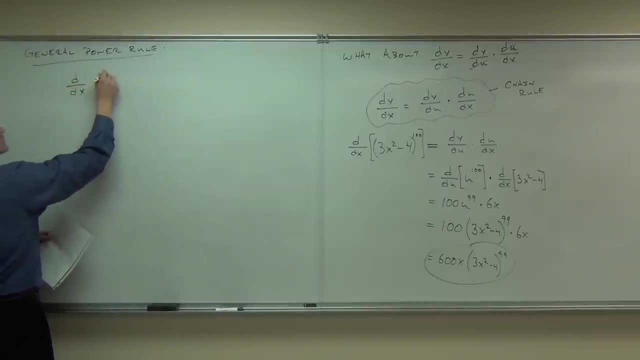 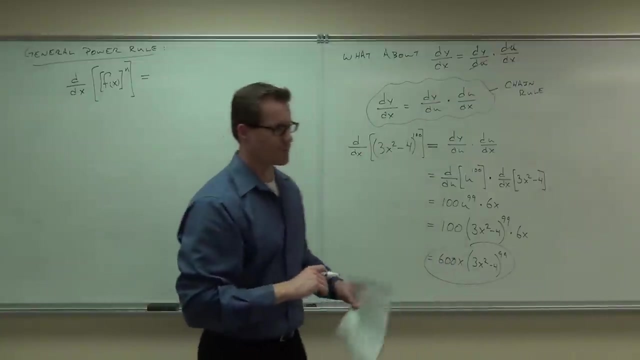 what if you need to take a derivative Of some function to some power? What if you need to take the derivative of some function to some power? Here's how you do it. This is called the chain rule, And here's how you do the chain rule. 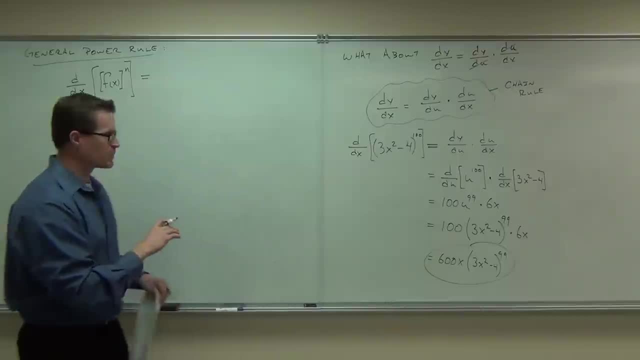 I can show it to you if you really want me to. This is what would happen. You'd say: okay, what's my function? You'd say: y equals u to the n. True, Where u would equal f of x. 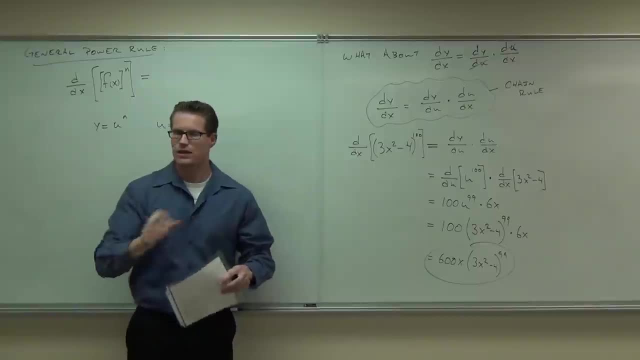 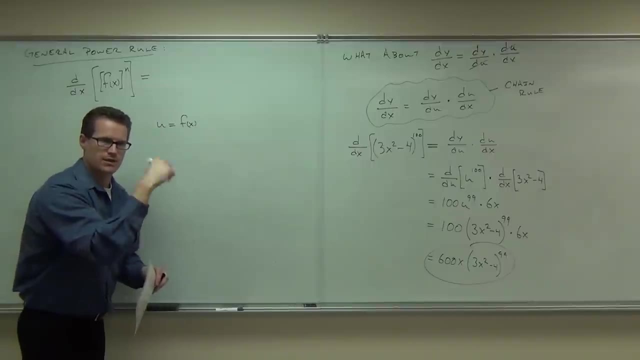 Do you believe me? You follow still. That's what the chain rule would say. Well, this says okay. if I took the derivative of u to the n, Remember your power rule. Power rule says: you bring down the exponent, You subtract one from it. 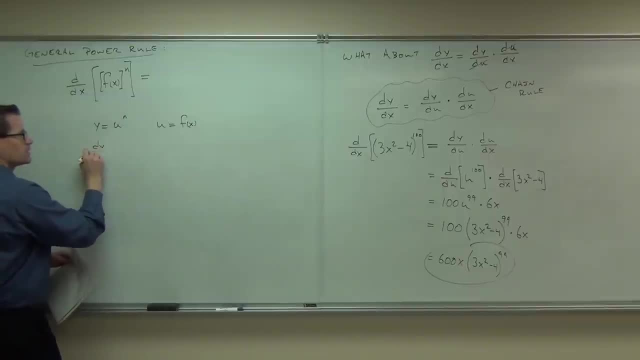 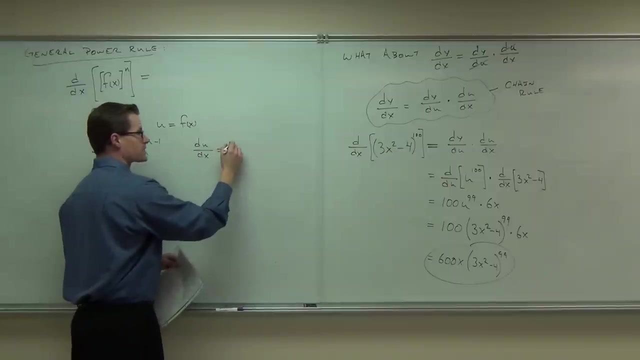 True, This would say: okay, dy. du would equal n? u to the n minus x, True u to the n minus 1.. Follow me so far. du dx would be the derivative of f of x. How do I want to write it? 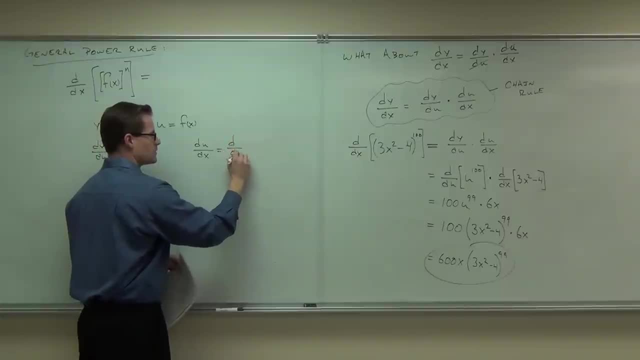 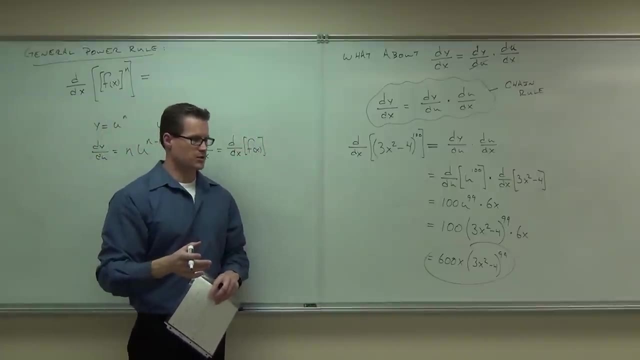 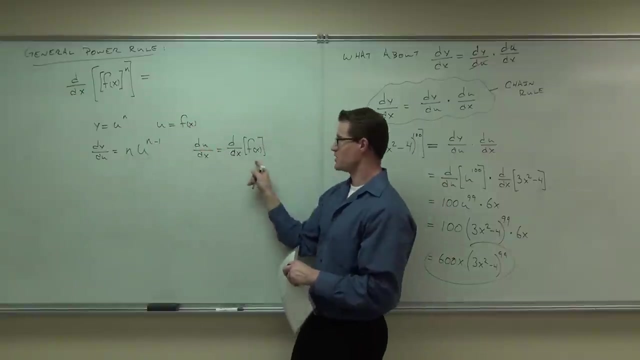 I'll just say this: The derivative of f of x, You could write f. prime of x. You could write that as well. Are you guys okay that the derivative of u to the n is n, u to the n minus 1.. And the derivative of f of x is the derivative of f of x. 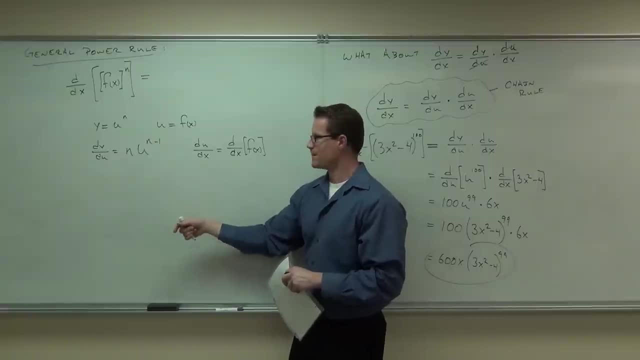 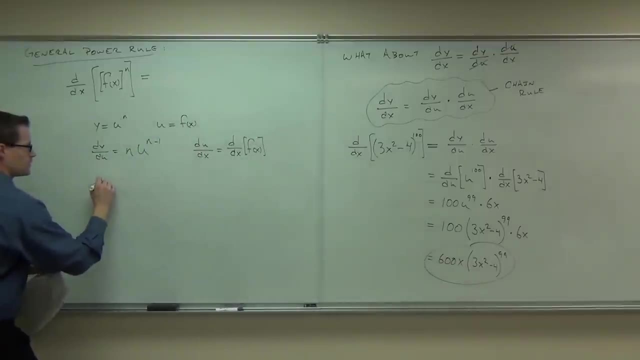 Does that make sense to you? I'll write it this way. so we have a formula in just a second. Do you see the chain rule at work? We have dy du, We have du dx. So in order to find dy dx, we'll have dy du times du dx. 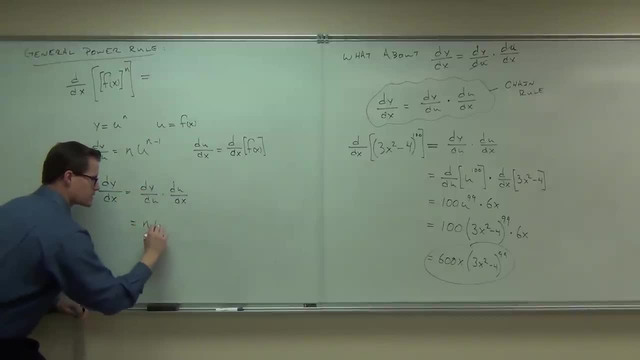 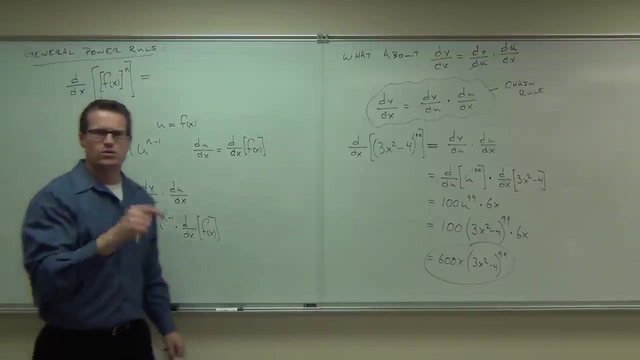 Well, what that says is: do a substitution, That's n? u to the n minus 1.. times the derivative of your function from the inside. How much is u? What's u equal to? Because we did that composition, What was u in our case? 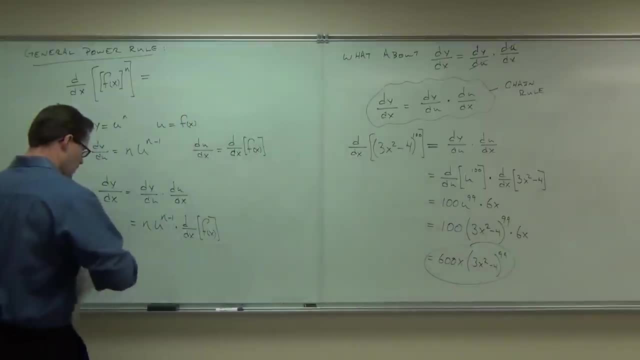 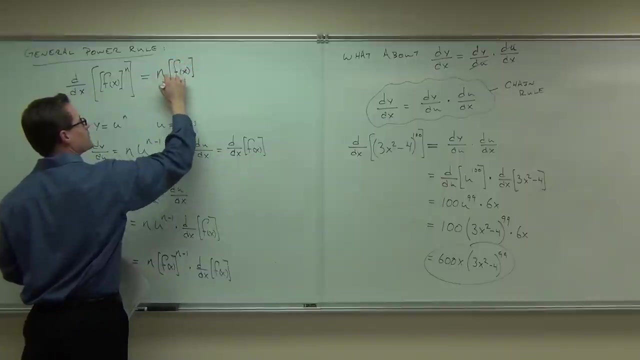 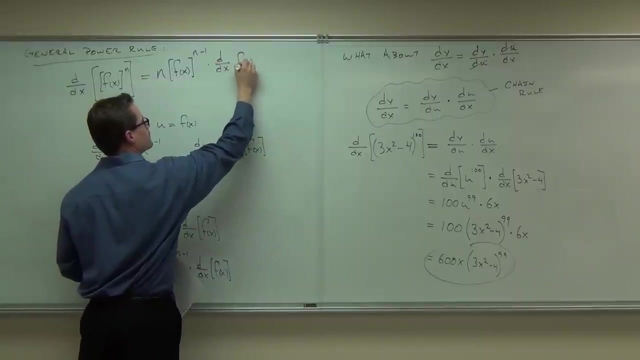 So do that substitution back into there, And what you end up getting is n f of x to the n minus x To the n minus 1.. d dx of f of x. Now, did we say anything about f of x at all? 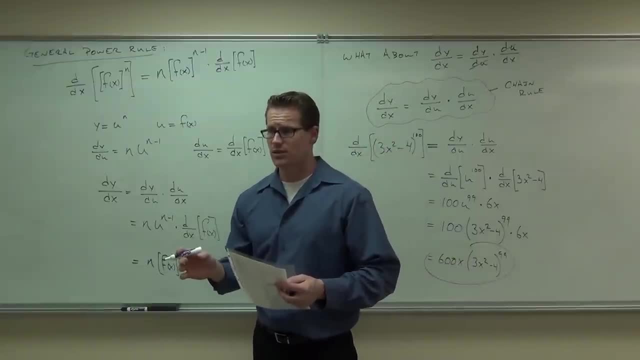 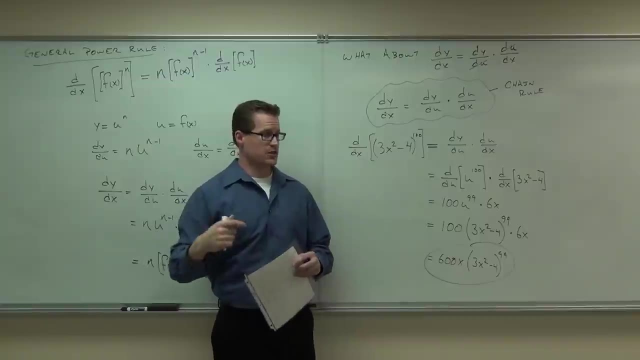 Do we make any qualifications about f of x? So then this should work in general, right? Any time we have a function raised to some power, we could use the chain rule on it. every single time. We led to a formula. I just invented this formula for you. 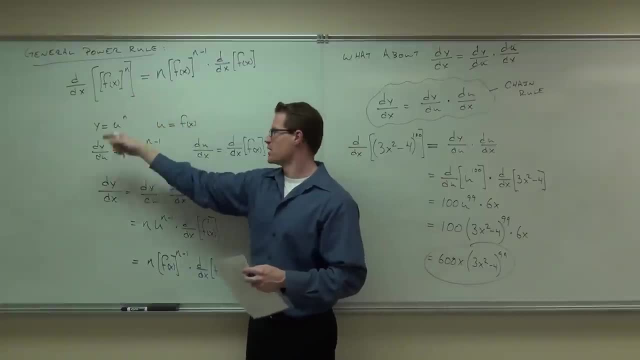 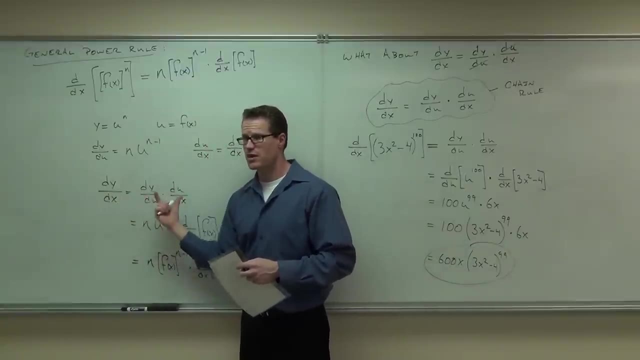 Did you guys see it? It's kind of cool, right? I invented the formula for you. We did a composition. We can do that. We took the derivative here. We took the derivative here. We know that to get dy dx we multiply those two things. 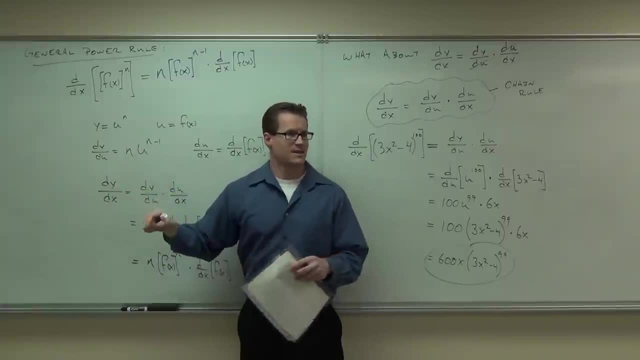 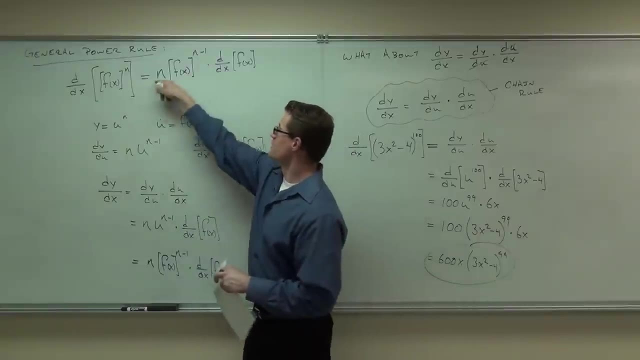 Then we just do our substitution back in for u. What that says is: if you want to take the derivative of some expression raised to some power, all you've got to do is take the derivative of the expression times the derivative of the inside. That's what you're doing. 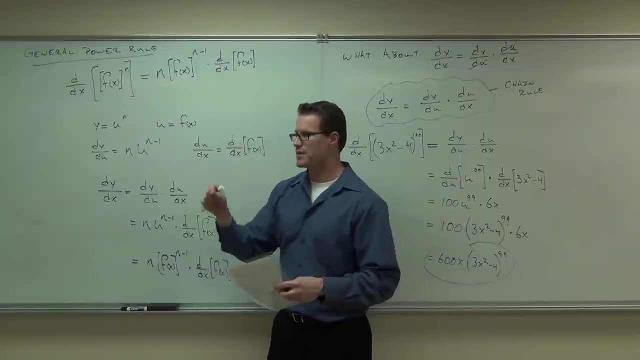 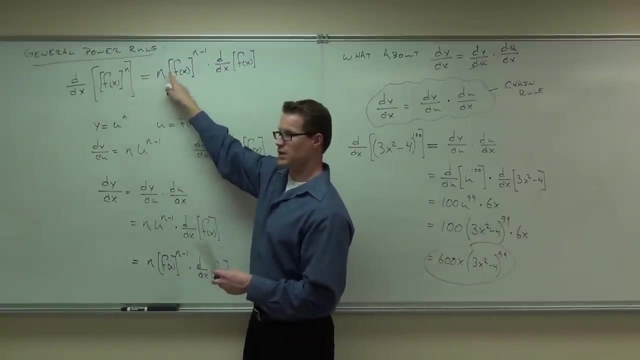 Bring down the exponent as usual, then multiply it by the derivative of the inside. That's what this says in English. Look at what it says. Bring down the exponent as usual, then multiply it by the derivative of the inside. That's what that says to do. 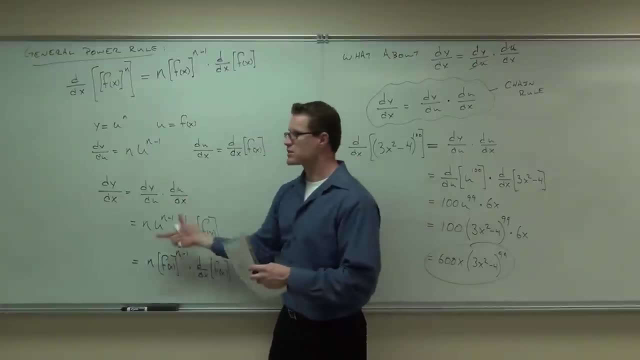 Raise your hand if you can. I feel okay with that. Do you have to show me all this to do it? No, I just proved it for you. This is kind of a proof for you to be able to do that You get it. 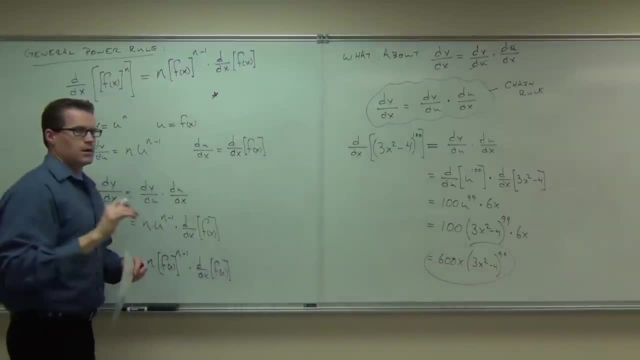 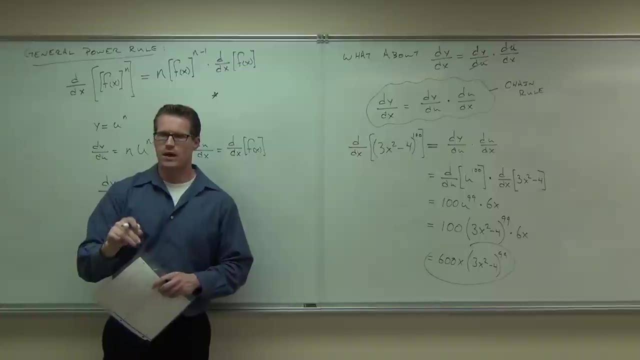 In English. if you want to do this in English, bring down the exponent as usual, as you normally do for the power rule. That's why it's called the general power rule. Bring down the exponent like it's a power rule, Just multiply it by the derivative of the inside. 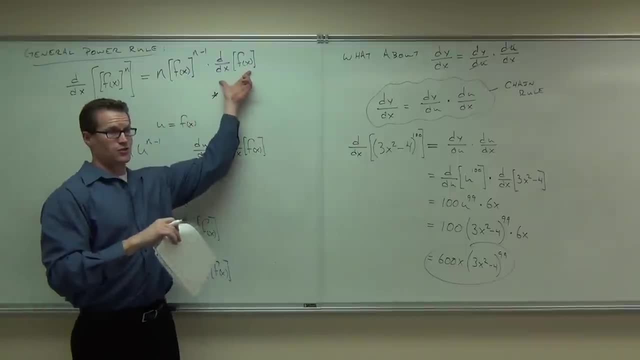 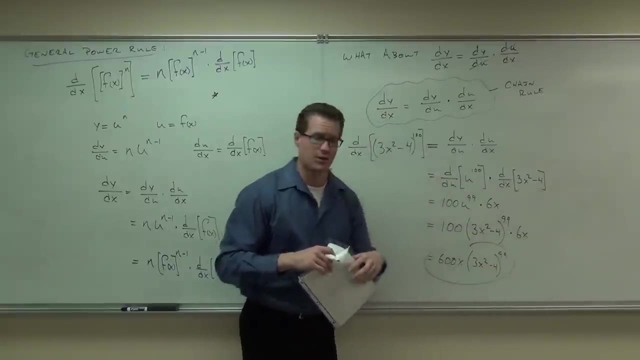 You just can't forget about the derivative of the inside, because this thing matters for sure. If you don't have the 6x here, does it affect your problem? No, Oh heck. yeah, by a long shot. So that does matter. 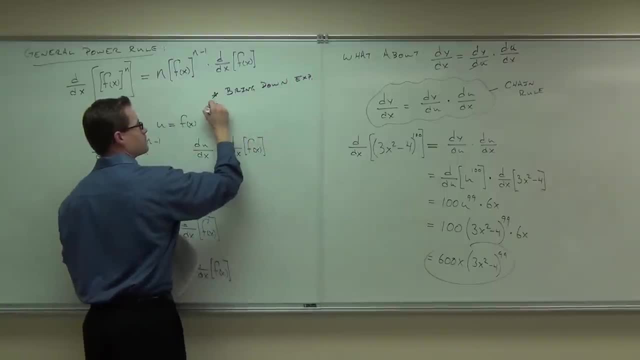 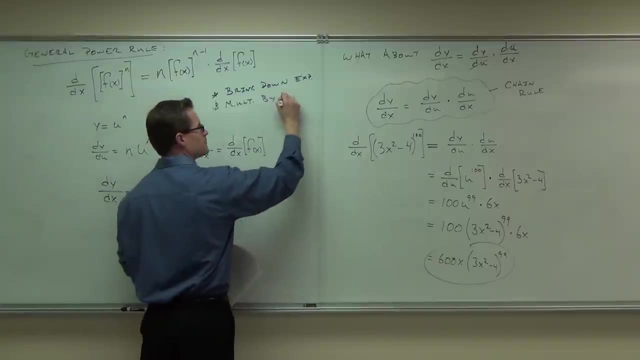 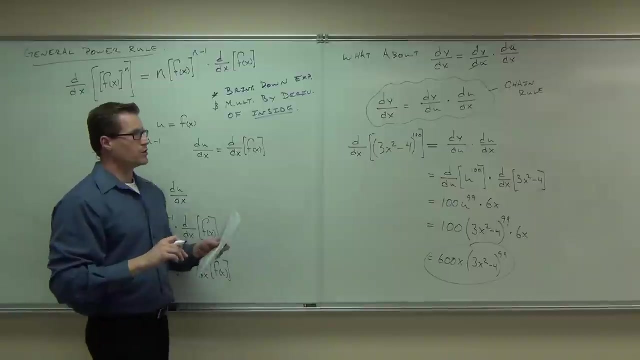 Bring down exponent and multiply by derivative of the inside. You get it. It does matter. You get it. Yeah, Would you like a couple of examples to kind of work through this? Oh, I don't need it. I don't know what you're talking about. And then after that I'll show you some more applications of the chain rule: Stuff that we can do with some trigonometry, which I know you're going to love, right? Stuff you can do with that that you can't forget, that you need to do with that. 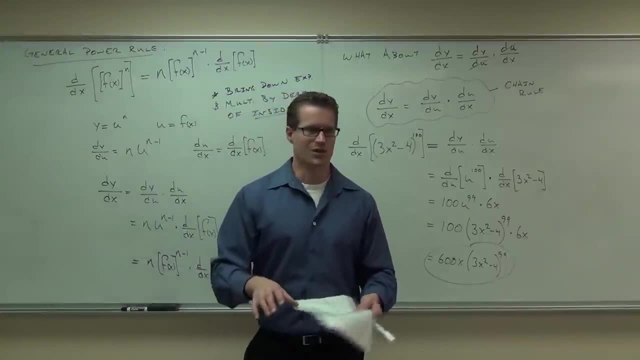 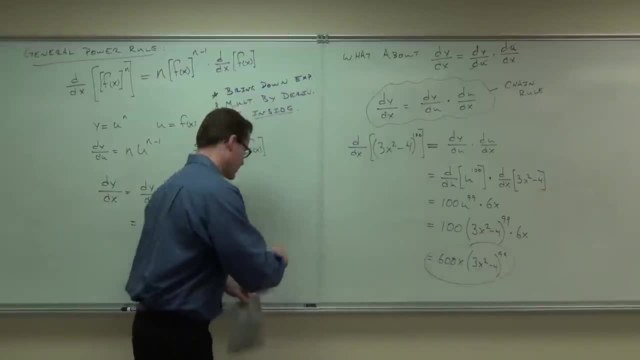 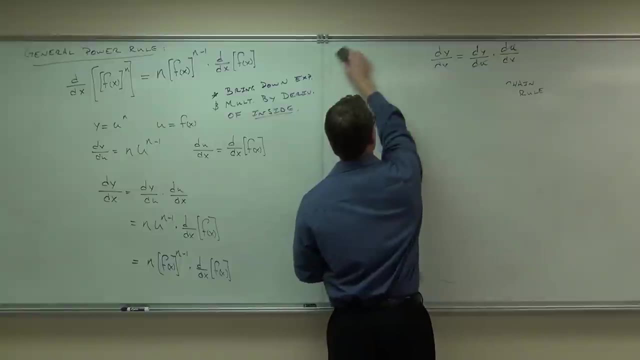 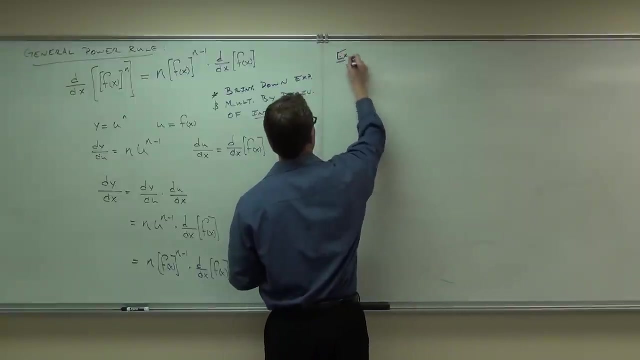 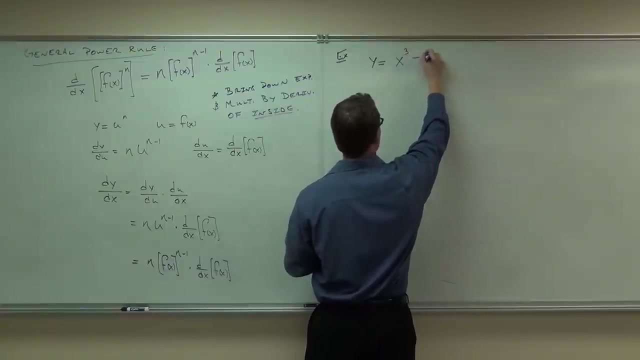 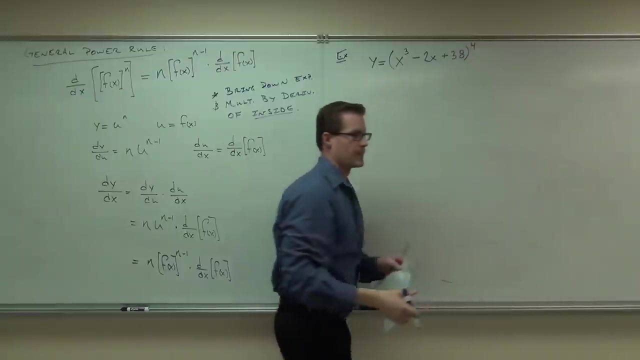 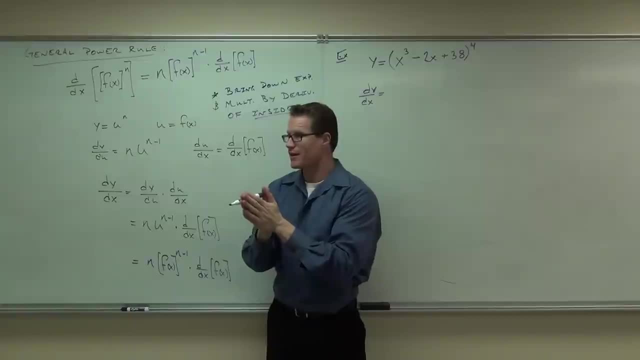 The answer is no. no, because this is a composition. Do you guys see the composition This? you could cover the whole thing up and call it u, or sorry, call it yeah. call it u to the fourth. y would equal u to the fourth and u would equal this stuff. 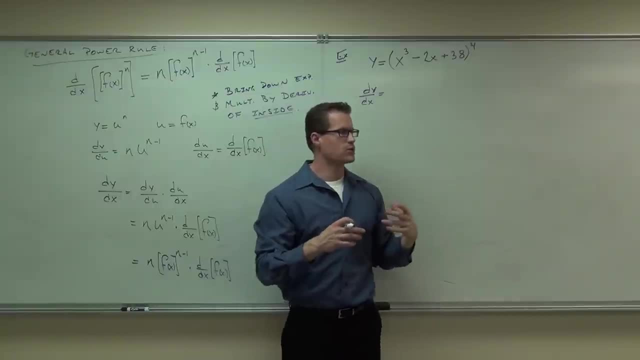 Does that make sense to you? We could do the chain rule here. Does this fall into the category of general power rule? Is it some function raised to an exponent? That's what we're looking for. Do you guys see the power rule in it? 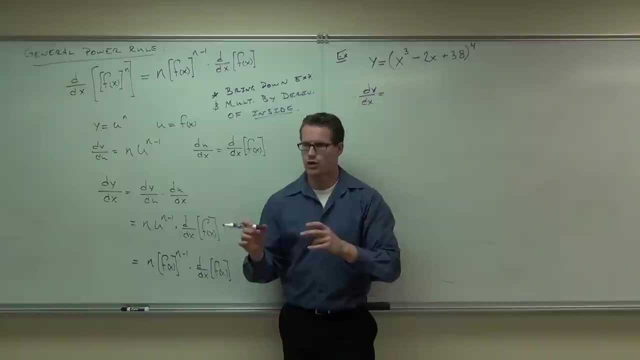 Have we got the power rule That says: here's what we're going to do? We're going to do the power rule just like we normally would. We'll bring down the exponent, we'll subtract one from it. Just don't forget to multiply by the derivative of the inside. 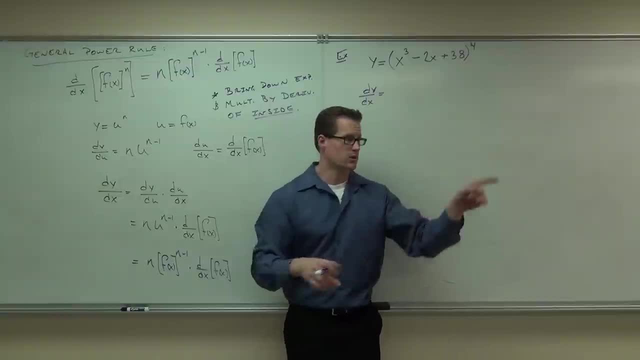 So you tell me what to do. now that we've talked about it, What do I do? Bring down the fourth? Good, four goes down. Do I still have an expression here? Yes, What's going to be on the inside of my expression? 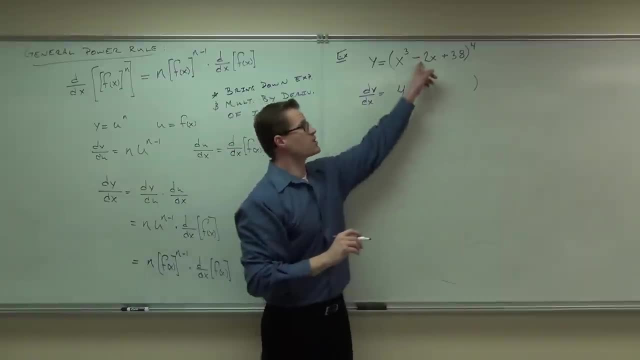 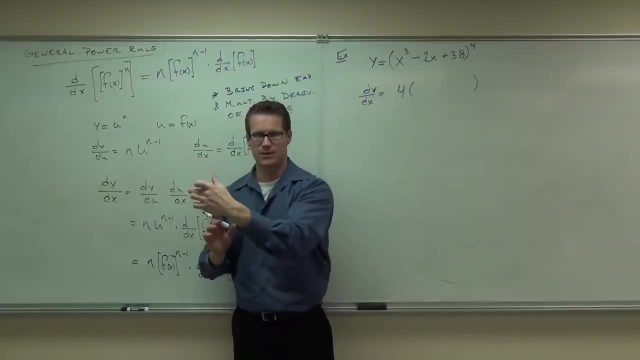 u. Do I change this at all from here to here? No, that's because that's the? u right, And you're going to be substituting back in for the? u ultimately at the very end of any problem, So that inside, that's not going to change. 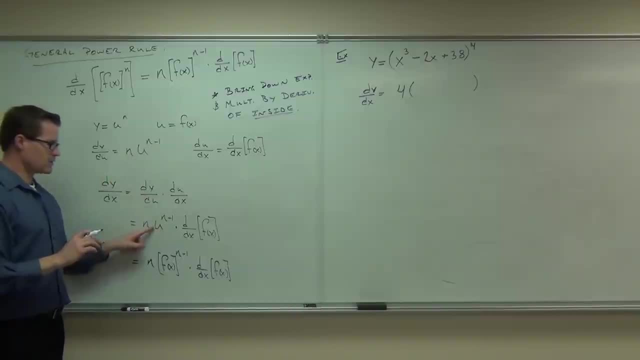 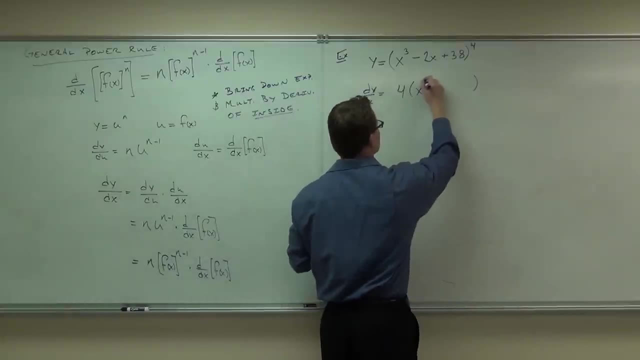 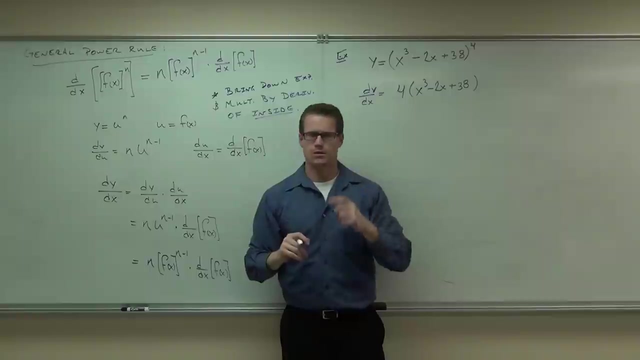 That's this. Look it See how we still have a u and we substitute back in the original function to that. That's the original function here. You're still going to have that. So far, so good. Yes, Wait a minute. 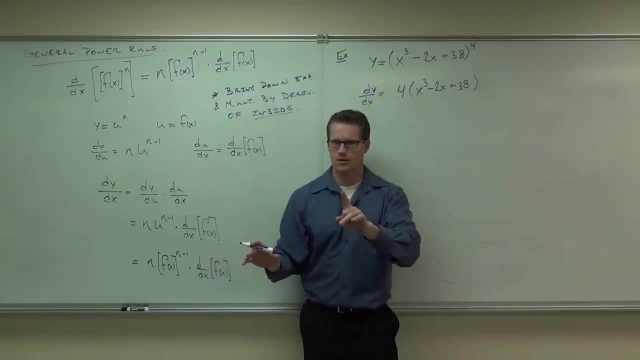 Right now. is this so far, so good? No, What's wrong? There's a derivative power. Don't really? you know what the biggest mistake people have? People do this: they bring that exponent and they forget to subtract from it. 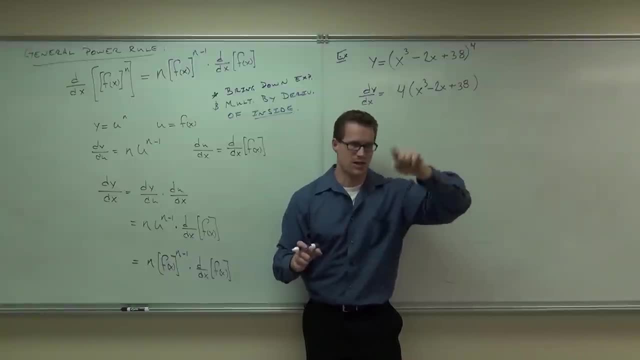 It's derivatives are not that hard right. in doing the general power rule, You know you're supposed to bring it down and subtract, People always forget the exponent. Don't forget the exponent. So we do bring it down, sure, but that four, that was an exponent of four. 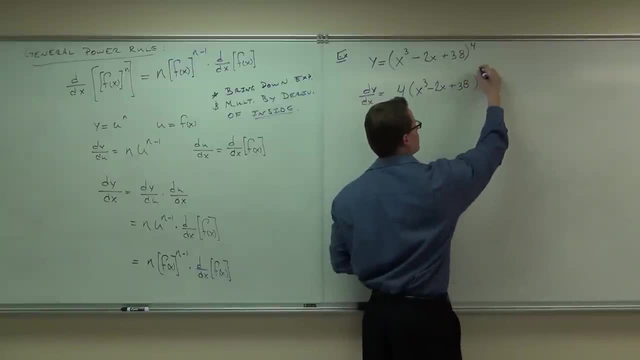 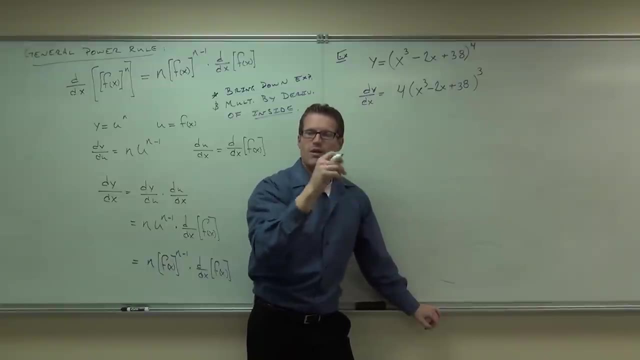 We subtract one from it, we're going to get Three. Is that okay? Is are we done now? No, We're good, though We bring down the exponent. we subtract one from it and now you get to do this part. 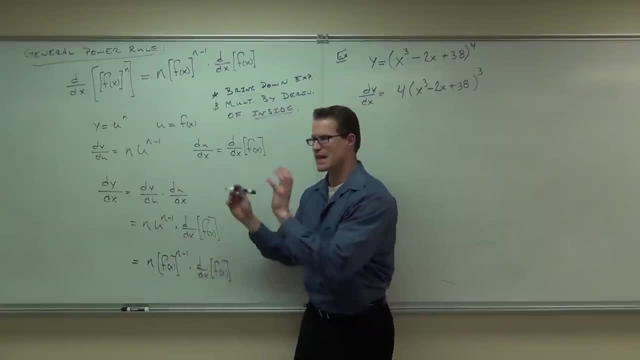 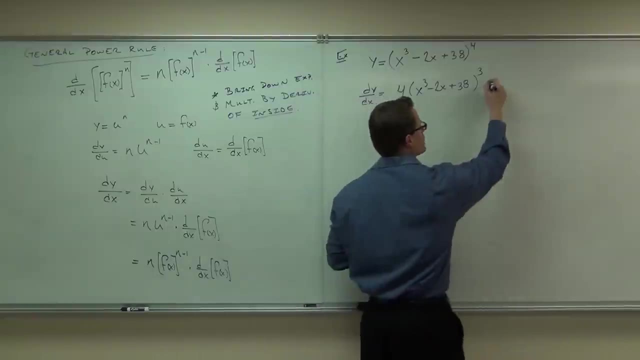 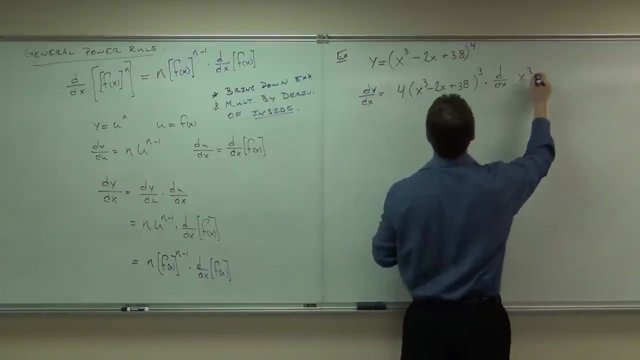 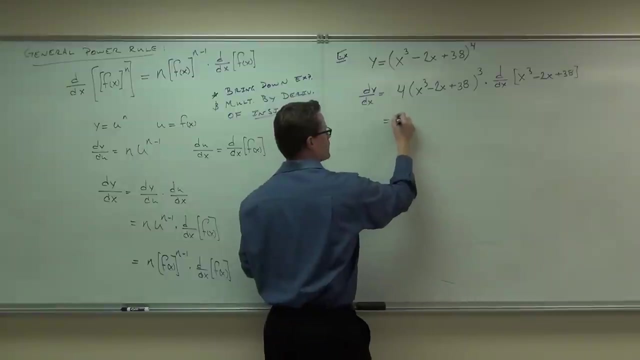 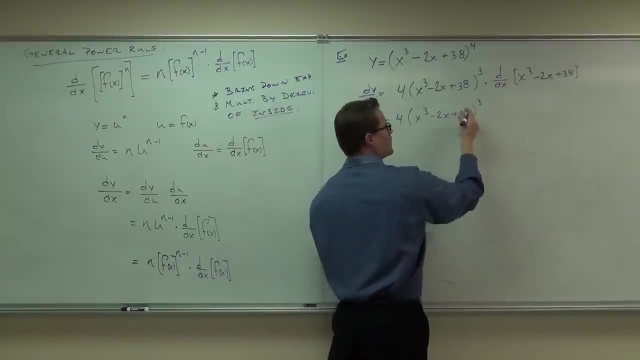 The derivative of whatever the inside is. The f of x is the inside of your general power rule. It says: do this, do the power rule, no problem, leave that alone and then multiply by the derivative of whatever was inside. Let's see we got four. got the same thing. notice how the calculus is done. 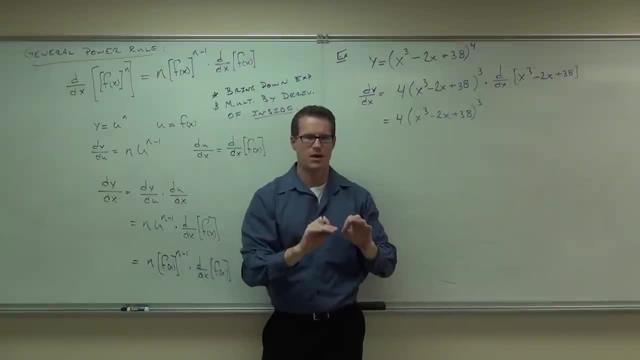 Do you see what I mean by follow the ddx? Do you see what I mean by that? It's all about where the ddx is. that's what your calculus is. So here this is staying the same. the only thing we got to worry about is that, over there, 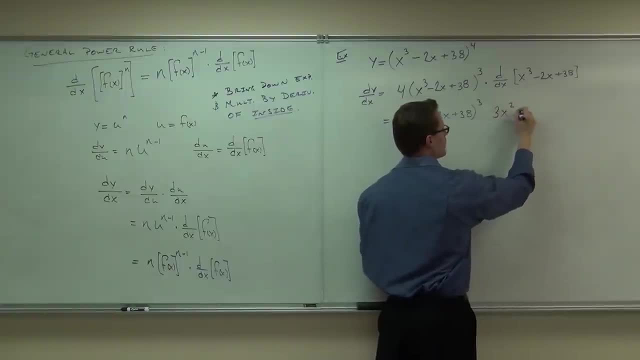 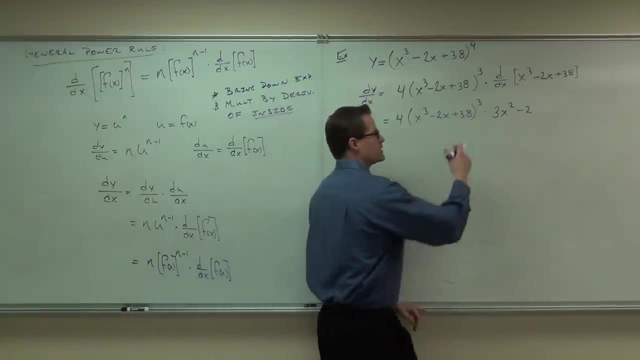 What is it? Three, Three times two? If I leave it just like this, am I going to mark points off from you? Yes, Absolutely. why Press the hand key? Press the hand key. Mm-hmm, I need to have. 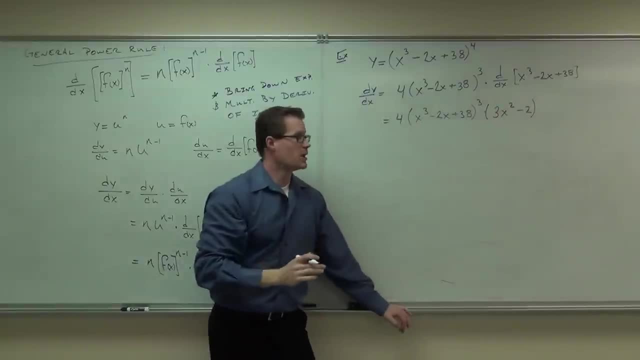 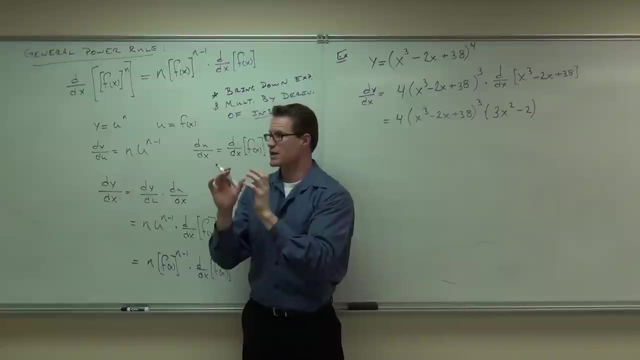 I need to have the parentheses. firstly, That says I'm multiplying the whole entire expression. Now you got a couple choices. You can move this thing out front and you can distribute that four into there if you'd like. Just make sure you have parentheses around it if you do it. 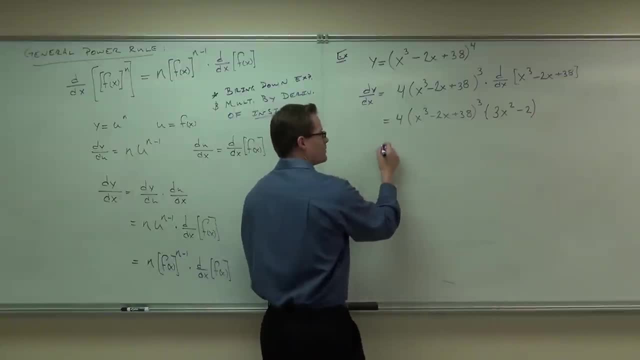 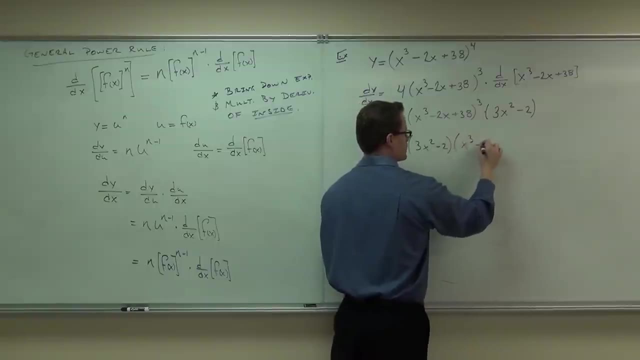 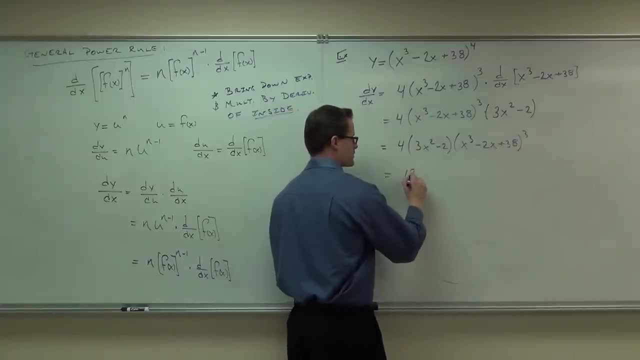 Does that make sense? So you might see a problem end like this, You might see a problem end like this, Or you might see the problem end like this: Just make sure you have parentheses there, or otherwise. yeah, I'm going to mark you off. 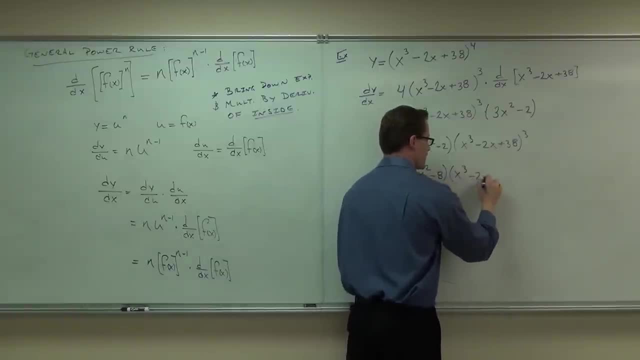 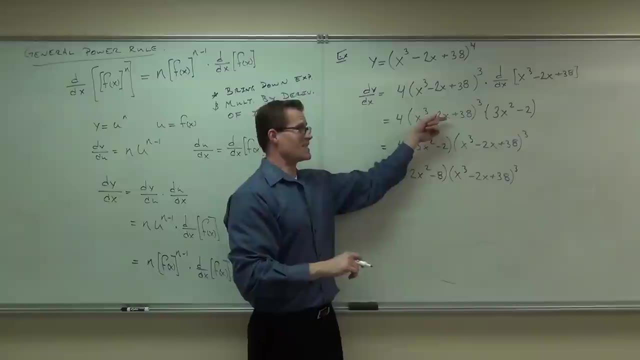 because that's a different statement. Now your question is: which one do you want, Mr Leonard, And I go as long as you need to hear: I'm happy with your calculus. Now I want one of these two. 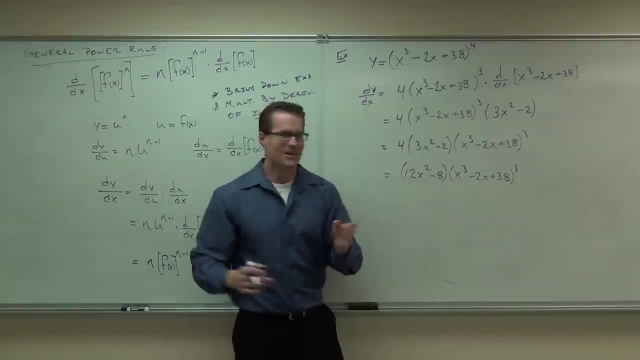 I want one of those two out of you. What I can't have you do, don't keep going. okay, There's no way you should ever foil this into the. actually, it would be foil right Outside, inside, whatever. 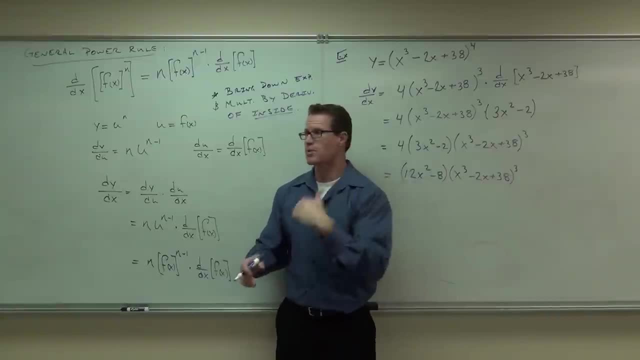 But you shouldn't ever do that because that's to the third power. You can't break the word. operations X ones come before distribution or multiplication does okay. So you can't break this rule. But this is: this would be perfectly appropriate. 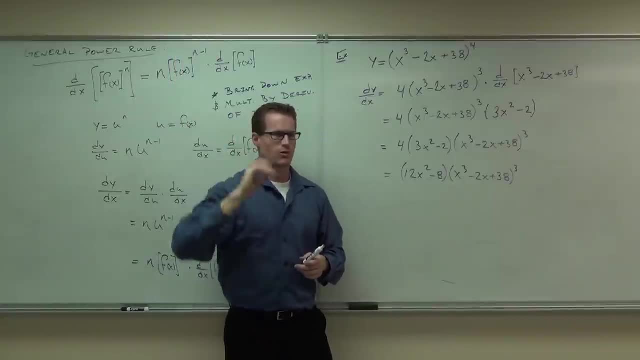 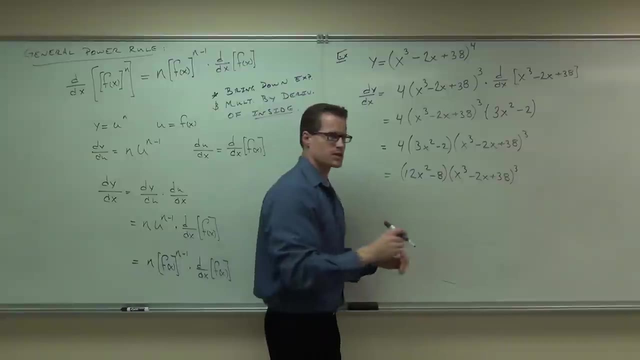 How many people feel okay with this so far? Are you ready to see that we've been doing this literally the entire time with our power rule? See the general means encompasses all right, So check this out. If I give you X to the sixth, just a simple example and I say: 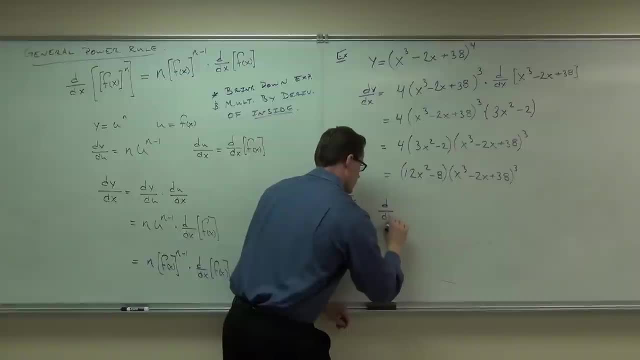 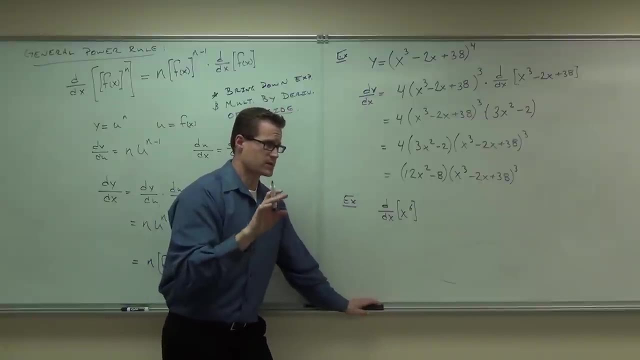 why don't you take The derivative of X to the sixth? You know inherently that that is 6X to the fifth, right. Okay, Inherently, X wasn't inherent, I guess because I taught it to you, But you know it nonetheless. 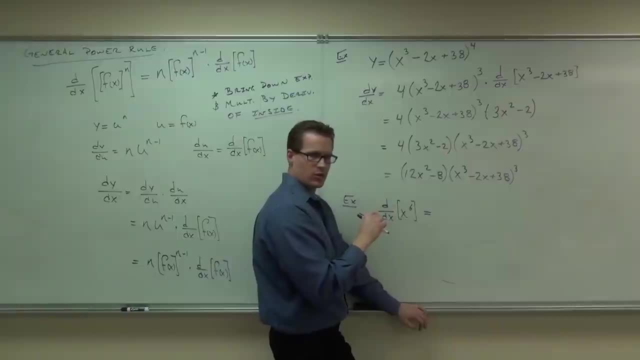 But if you apply, if you apply the general power rule to this, check it out. If you said, oh well, that's a function in terms of X, I'll write that a little better so you can really see it. I said that's a function in terms of X. 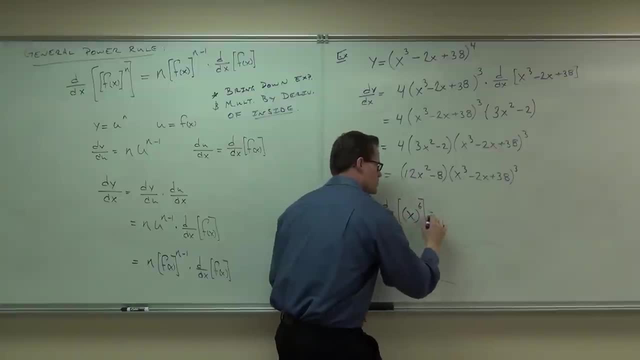 So you can really see it. If you said: oh well, that's a function in terms of X, could you do the general power rule to it? And the answer is yeah, you could Check it out. You would do the sixth, X to the fifth. 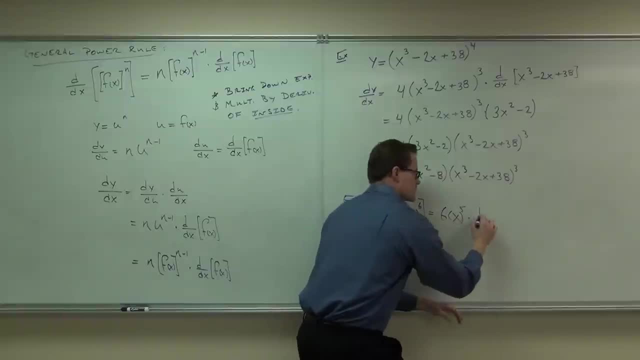 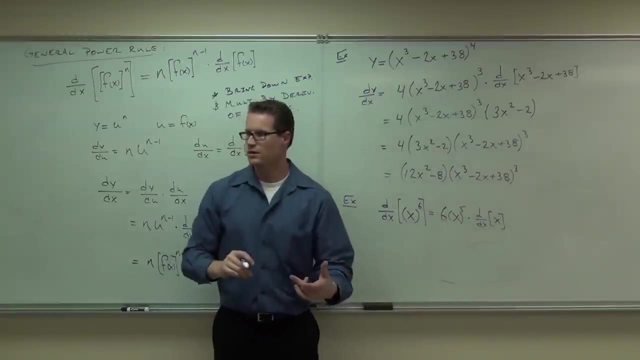 Remember- that would be in parentheses, right, Because that's your function Times- the derivative of whatever's inside. Only this time the inside is X. What's the derivative of X? That's why we didn't have to show that, because the derivative 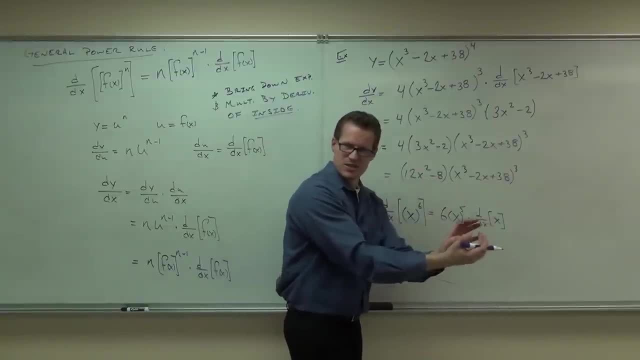 of the inside is always the same thing. It's always just X. Do you get it? We've been doing the general power rule. We've been doing the chain rule the whole time. It's just, it was simple. It was simpler because we didn't have that inside. 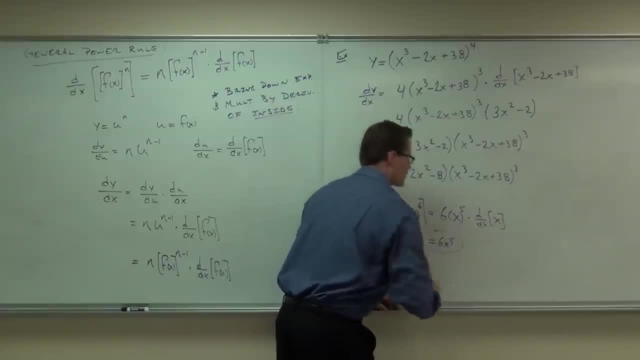 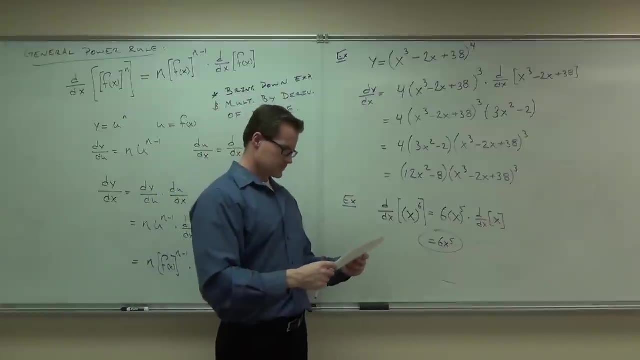 So that would become 1, and you get 6X to the fifth Interesting. We've been doing it. That's why it's called the general power rule, and we had the power rule before You. ready to keep going? Yes, 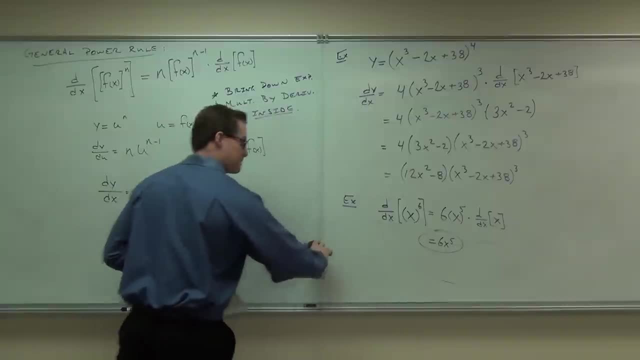 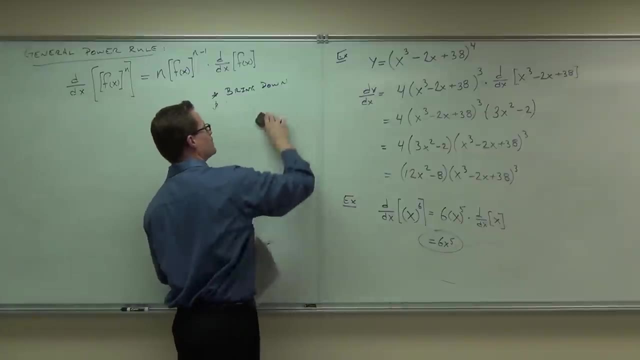 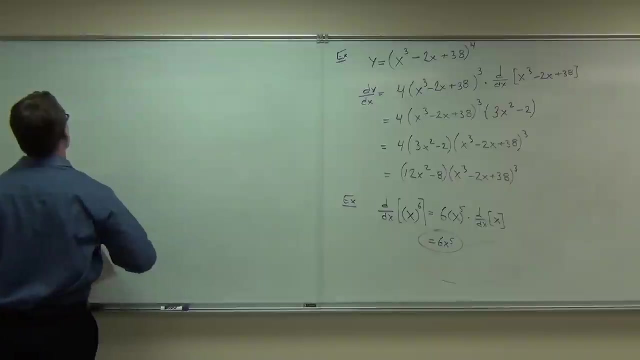 Okay, Let's try a few more. We're going to start building on this idea, though A small power sheet, because this is too late. Okay, Excuse me, Can you hear me? I'm gonna guess it's not working. 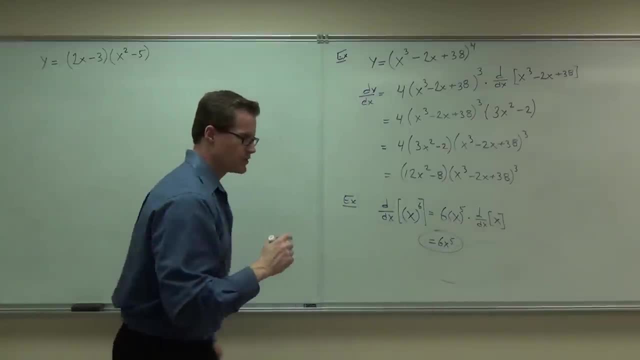 Oh, The computer needs to be still Okay. Yeah, So Three시다 and one第二, One, two, three, four. Okay, All right, All right, We're all good guys, All right, Good. 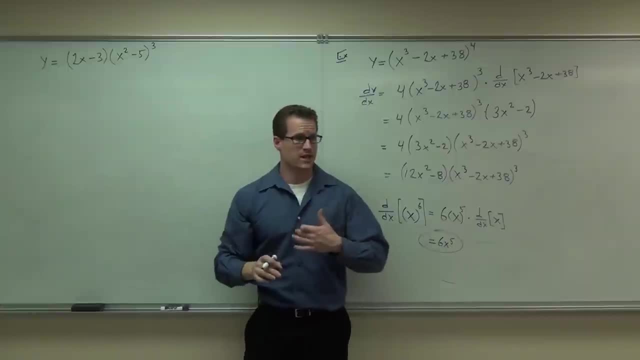 Give me two ways to do that problem. One: Who do you mean? there's a stems? Do you still want to distribute? No, in fact, if they gave that to you before, that would be how you had to do that, right. 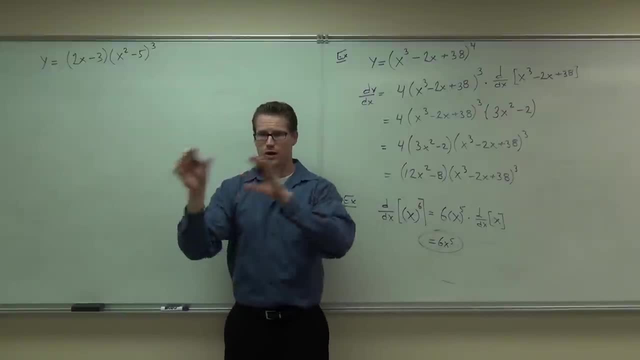 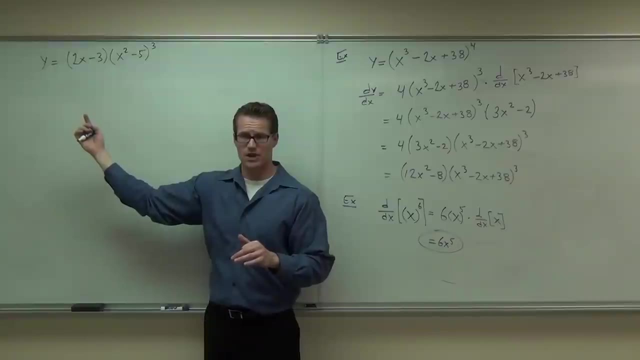 Because there was no way to get rid of that three for you without FOILing that all out and then distributing, Or FOILing at least this out, and then using product rule. In fact, maybe you had to do that on a couple of your examples and it's like: 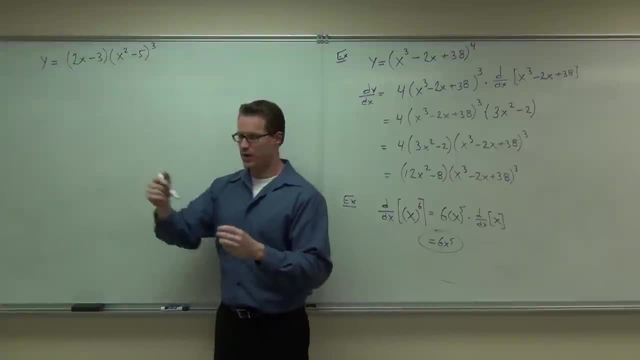 Darn exponents. But now let's look at this for what it is. This is a derivative. Can you see a product rule in it? still, Yeah, Can you see a general power rule in it? right now, Yes, Question is, which one comes first? 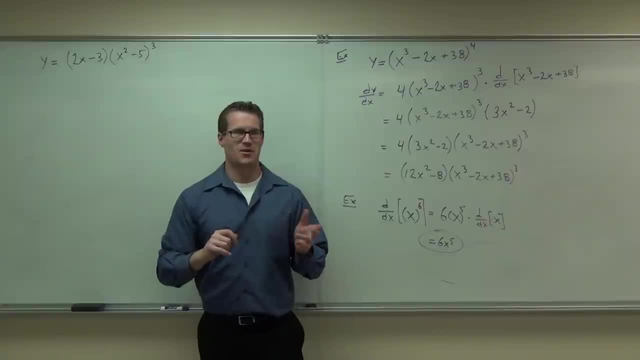 General power rule on product. Well, half of you are right. Which half is the question? Which one working from the outside, in which one encompasses more of the problem? You should be able to say this. You should be able to say: this whole thing has to do with. 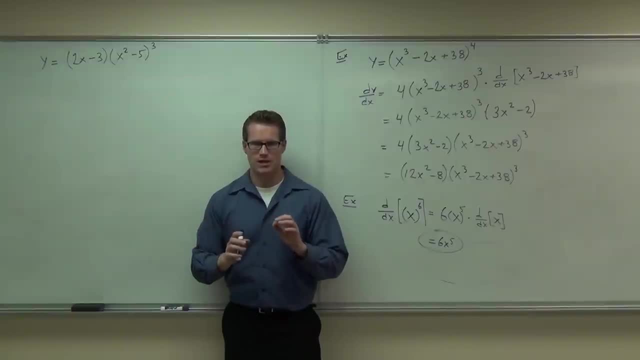 does the whole thing have to do with the general power rule, Which means: is that exponent of 3 applied to the whole thing right now, Then that does not come first. Is the product rule applied to the whole thing right now, Then that comes first. 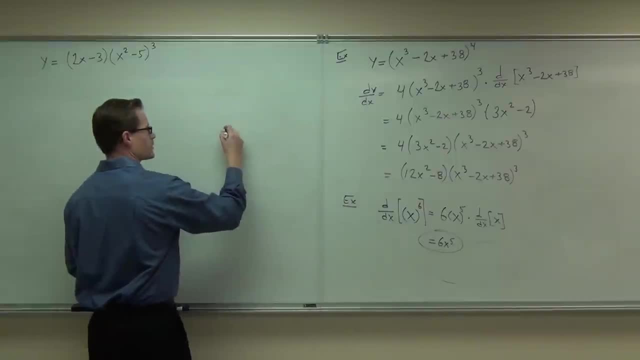 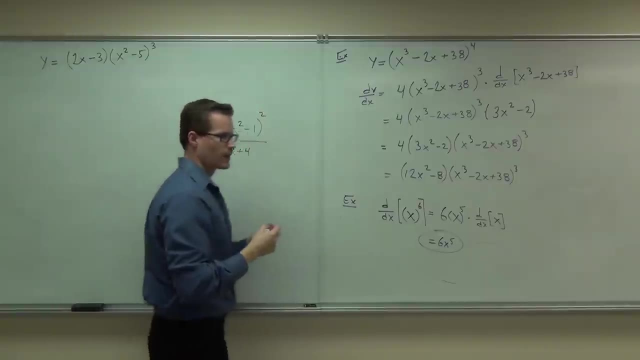 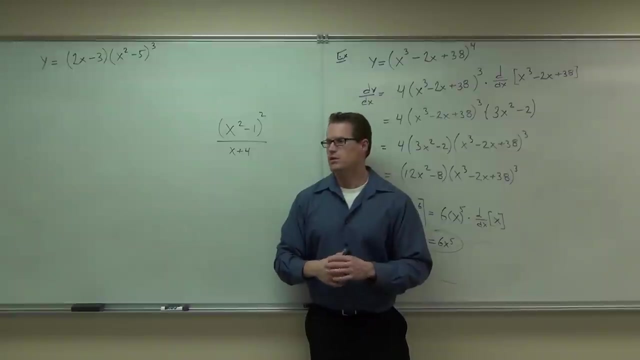 Does that make sense to you? It'd be the same as this question: Which one would come first, a general power rule or a quotient rule? What do you think? Definitely a yeah, The general power rule is only applied to this little top part, right? 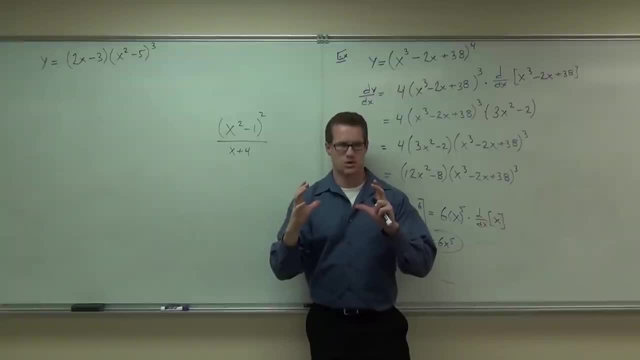 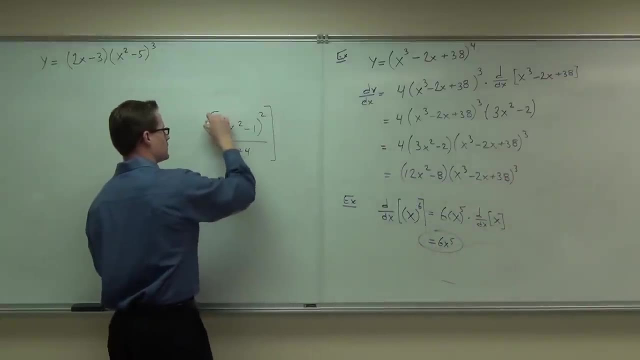 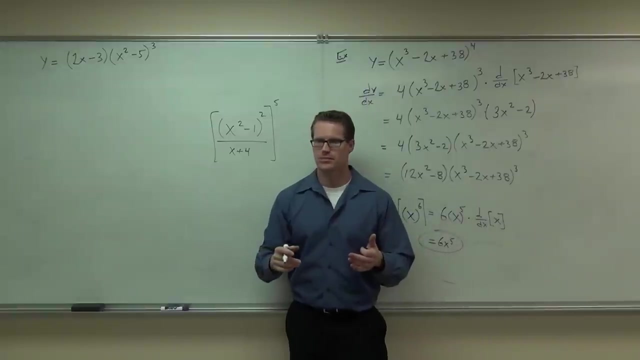 It doesn't encompass the whole problem. The quotient rule encompasses the whole problem. That would come first, working from the outside inside. Now, if I did this, you'd hate me first off. Which would come first in this case? Chain rule. 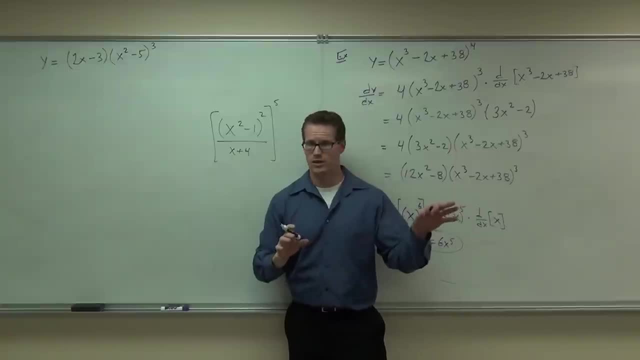 Chain rule. In our specific case this would be: you can say chain rule, that's fine. This would also be called the general power rule. Do you see it, General power rule? and then you would do the quotient rule, Then general power rule. 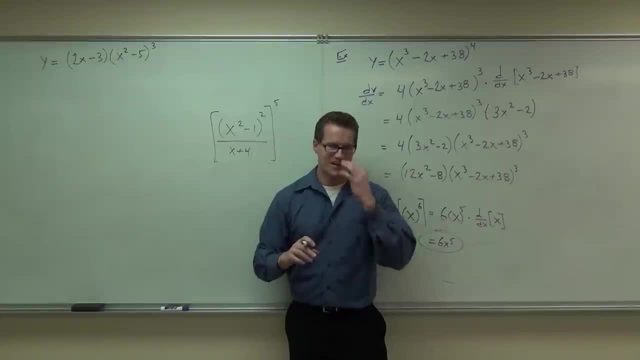 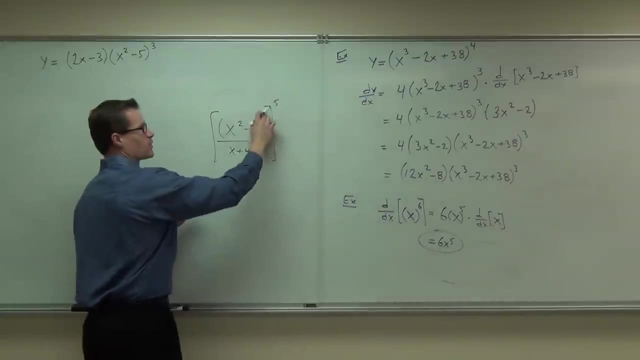 And then general power rule inside of that. yeah, OK, that would be nasty. One way that you could make this easier, if you're looking at it, you could take both this exponent and say: OK, this is now to the tenth and that's to the fifth. 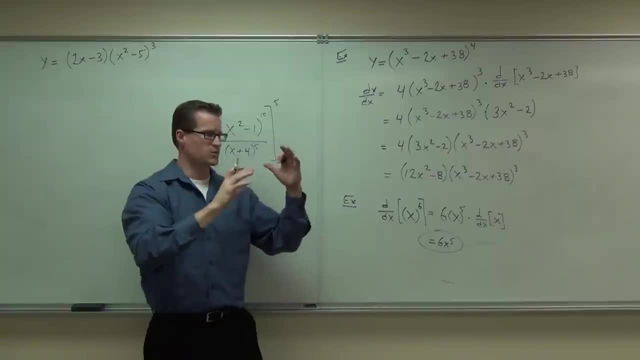 That might make it actually a little bit easier. But starting out you would see the general- I'm just making a point here- You'd see the general power rule first. Do you see what I'm talking about? You see the product rule first here. 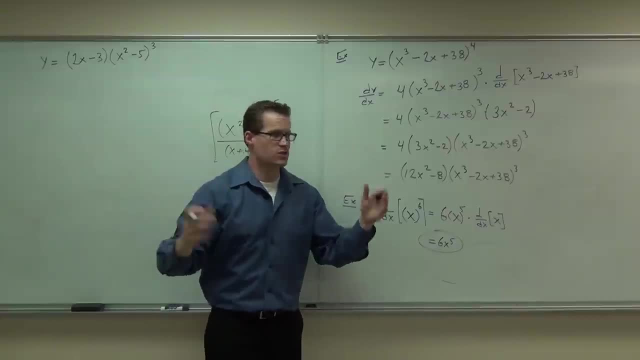 It encompasses the whole problem, And that's how you diagnose these things. What do you do? first, Whatever's encompassing the whole problem, And then you work your way into it, You work your way inside and you follow the DDX. 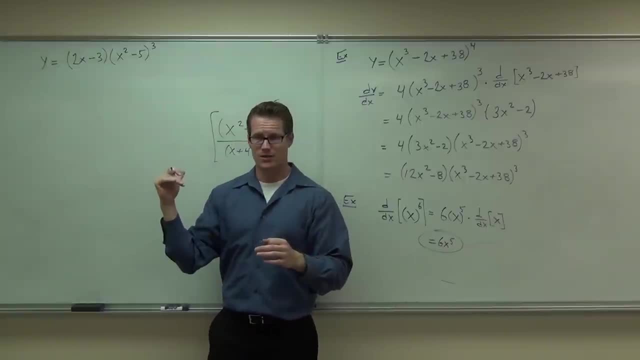 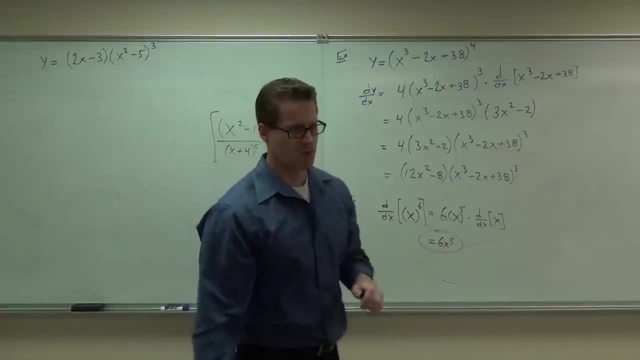 And the DDX will tell you what to do. Are you ready to do this problem? Let's do it. So, first thing we see: OK, connecting this thing is a multiplication. That means a product rule. Set up the product rule. 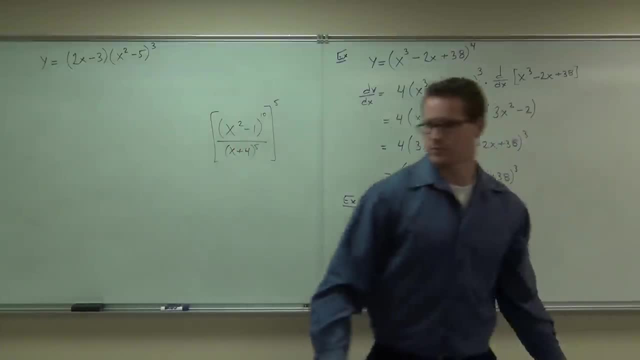 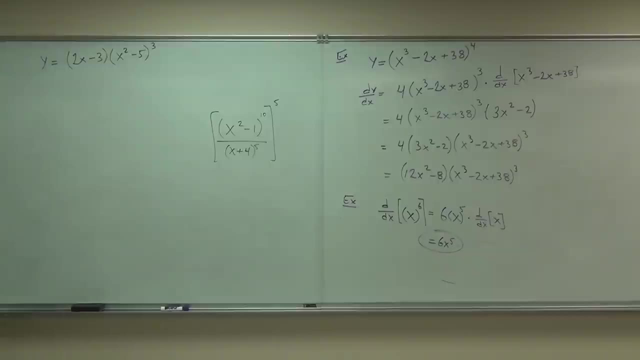 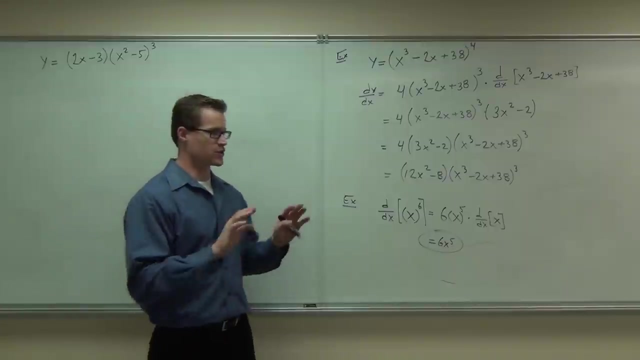 Go for it. This one, The cubed root of that- is going to stay in with that function. Just do the product rule right now, And we'll talk about the next part later. Just do the product rule and set it up. Don't take the derivatives yet. 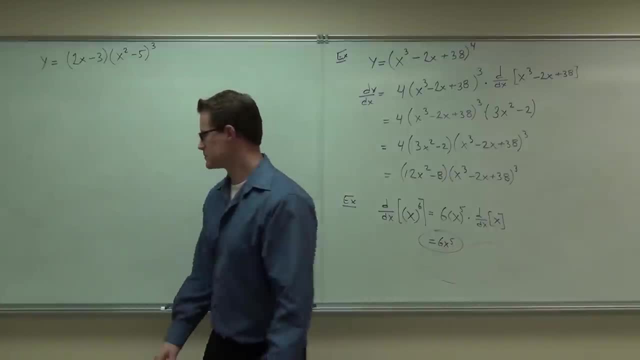 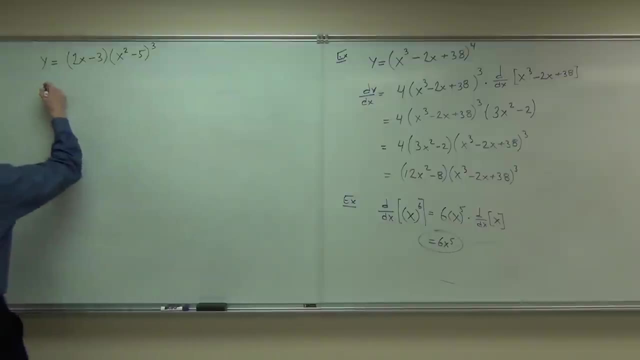 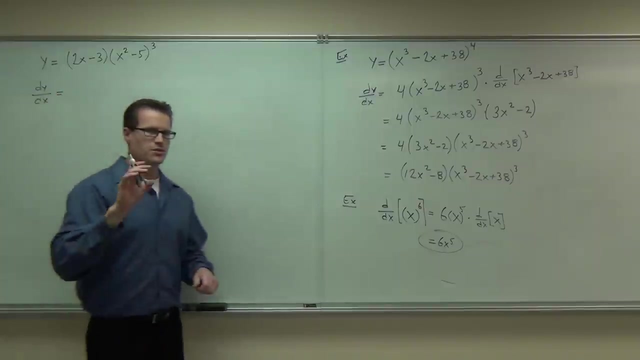 Just set up the product rule. Set up the product rule. Why don't you take, no, don't do the derivative, Just set up the product rule. The product rule should say the derivative of the first times, the second plus the first times the derivative of the second. 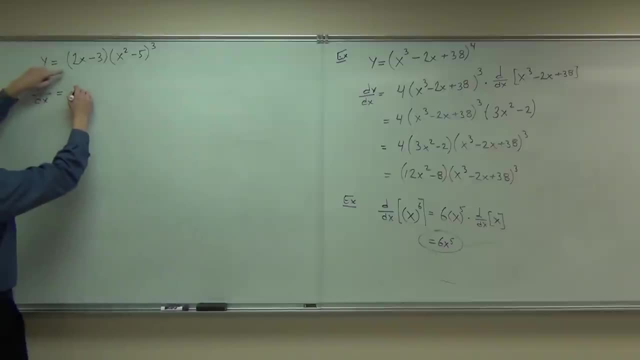 Were you all able to do that? Yes, So this is what I mean by that: The derivative of the first times the second. Is that the second? No, That's the second. Yes, That 3 has to tag along with that piece. 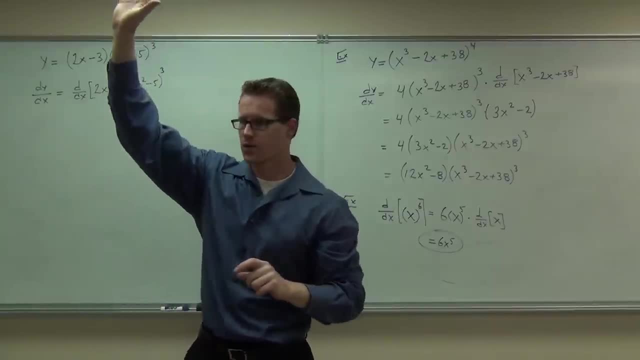 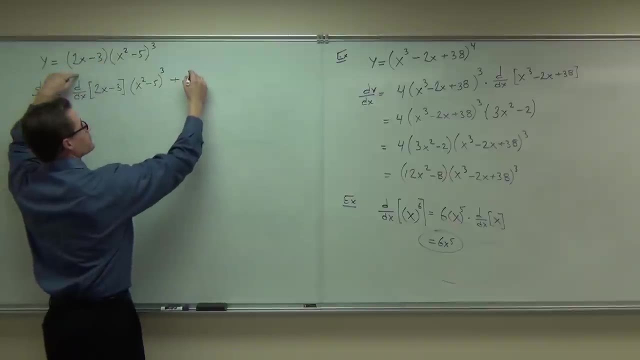 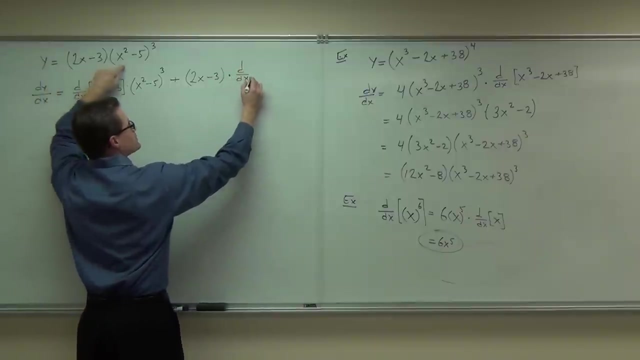 if you're going to do the product rule, Rich, have you got that so far? OK, good deal, You have the exponent right. Then you do a plus, And you do So derivative of the first times. the second plus the first times, the derivative of the second. 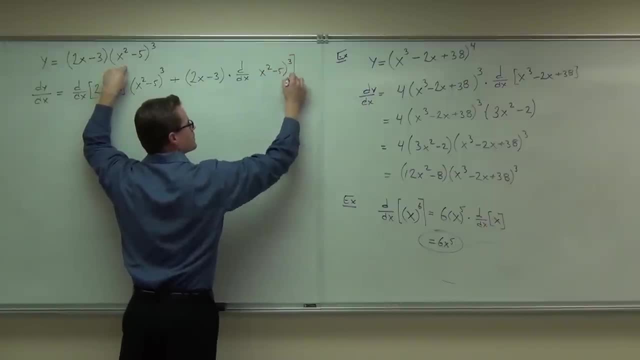 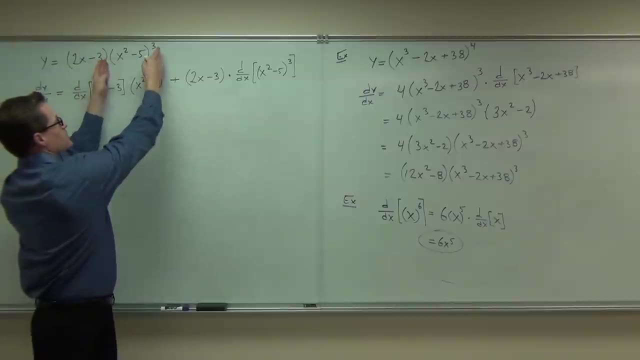 Do you? Yes For us. here's what it said. This was the first function of x And this was the second function of x. It was being multiplied right, So you have to take just those two pieces. That's what you were doing here. 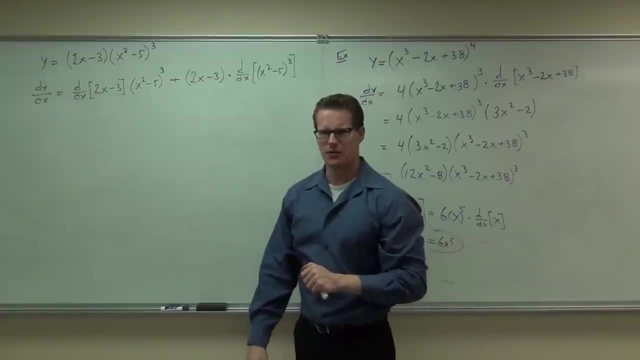 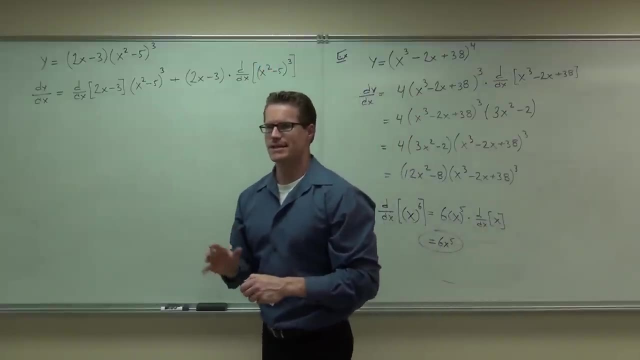 OK, I'm crooked, aren't I? I'm always like that. I think. How many of you feel all right with this so far? Try to be more straight on the next one. Now you follow the ddx and you just 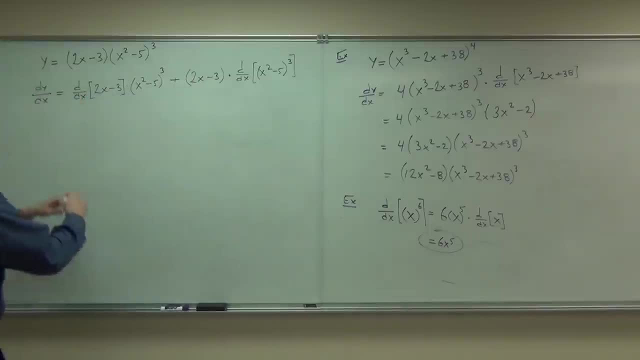 do what it tells you to do, because that's your calculus. So we just take derivatives piece by piece as they appear. So, piece by piece as they appear says: can you take the derivative of this thing right there? That's actually quite an easy one. 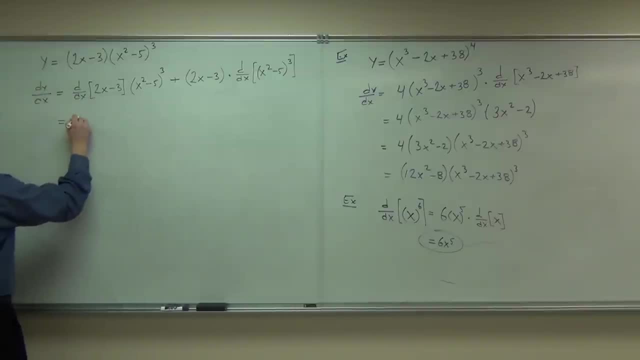 What's the derivative of that? So this says: all right, 2.. Do I take the derivative of that? No. No, it has no ddx, It's just a derivative. Do I take the derivative of this: No. 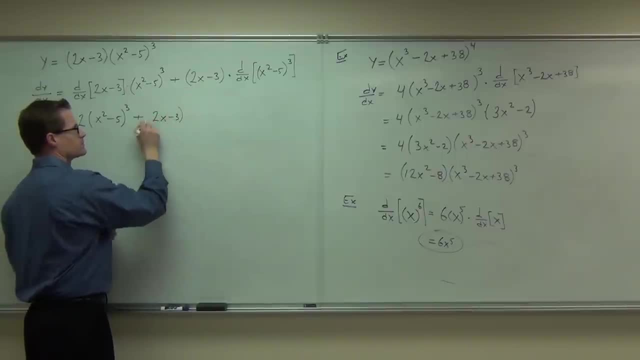 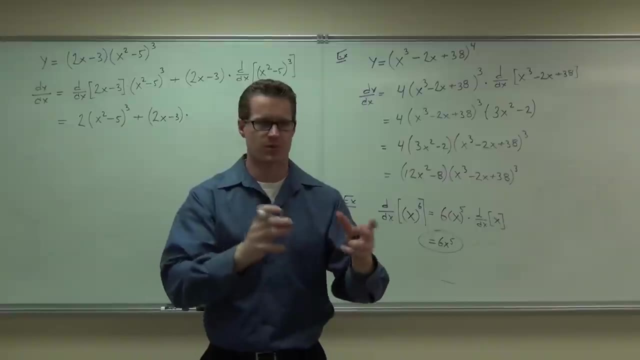 So I just write it. And now we get down to this piece And notice how it's basically. the product rule lets you break it up as problems within problems within problems. None of it's going to get any harder than this, It's just you might have more rules encompassing it. 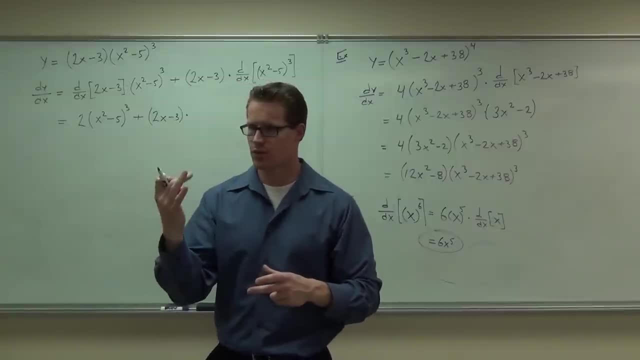 So if you can follow the rules down- you know the three rules: the chain rule, quotient rule, product rule. You know how to go from the outside inside. Just follow your ddx, You'll be OK. Now, that's easier said than done, all right. 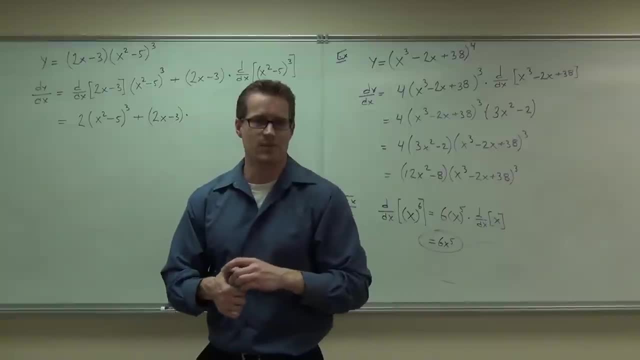 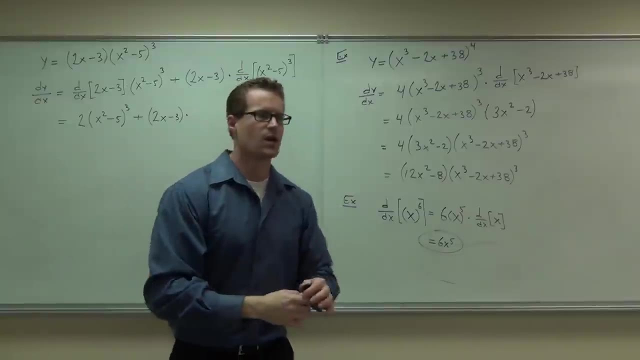 I know some of these problems are very tasking, But if you can do that, that's the fundamentals here. You look from the outside, inside, start with the big rules and follow the ddx And then use rules within rules, within rules. 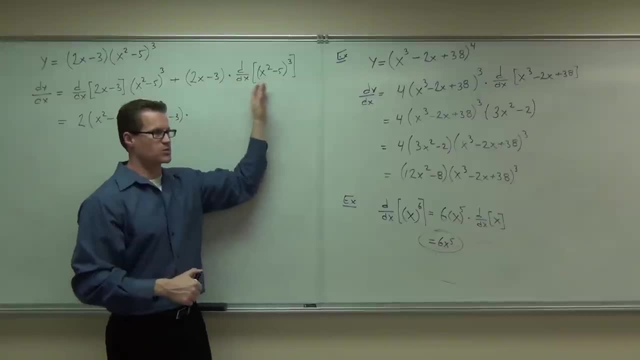 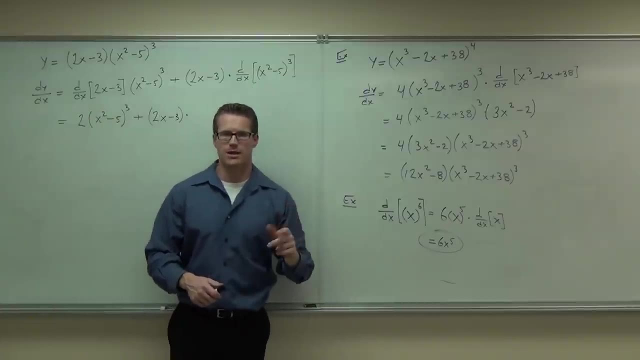 So on this one we look at this and you say: can I do that piece, that derivative? It's basically a problem within a problem. What's the derivative of x squared minus 5 to the third? What rule do you need for that? 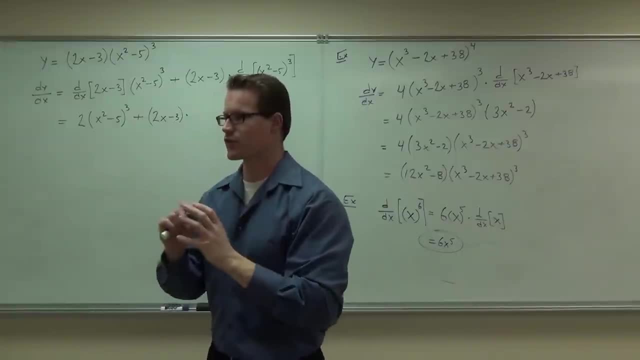 Chain rule or the corollary to that, because this is a specific version and this version of the chain rule is called the what? General power rule. So this was a product rule And inside of that I had a general power rule. 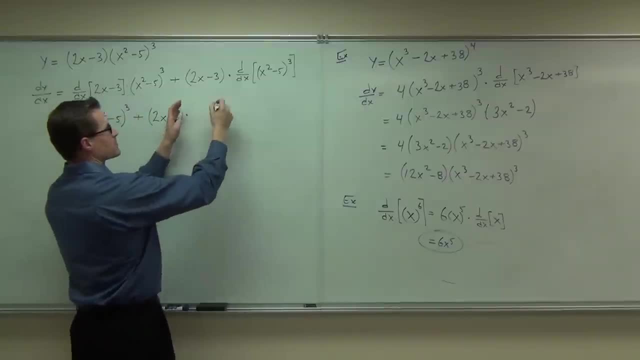 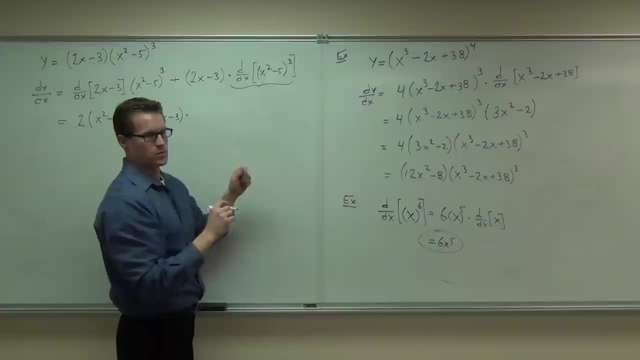 General power rule says: well, what I'm going to do is so for this piece. what do I do? So notice I'm here right now. I bring down the 3.. Very good, What do I have next, please? 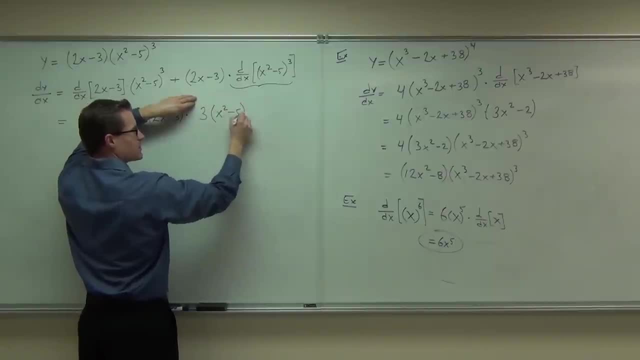 x squared minus 5.. Good, I don't change that inside. I don't change that to the what exponent Square. Oh, don't forget that. And then I'm done. That's right Times. the derivative of the inside. 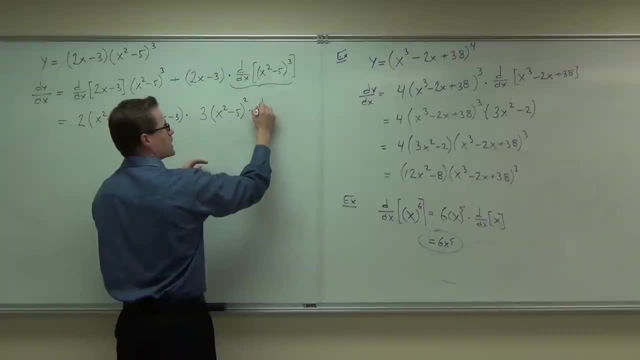 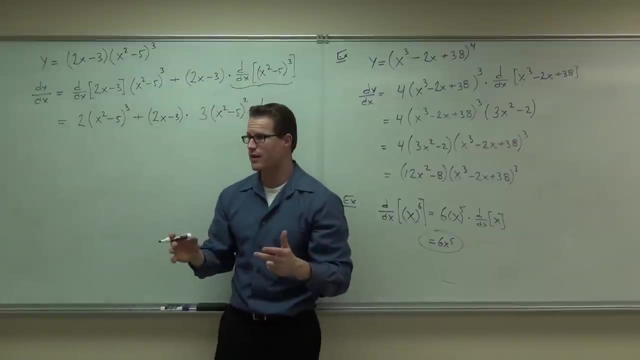 That's the chain rule, That is the general power rule Times the derivative, And I want you to write it out. I want to see this. I don't want you doing the math in your head right now. We're just barely learning it. 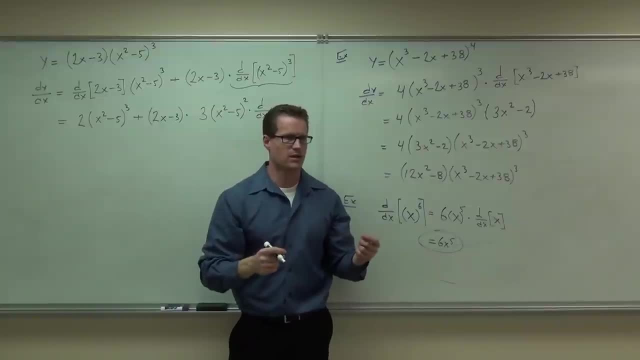 I know that eventually some of you are going to be able to just do these in your head In this class. for right now, wait until you get to 4b to do that. For right now, I want to see your work that way. 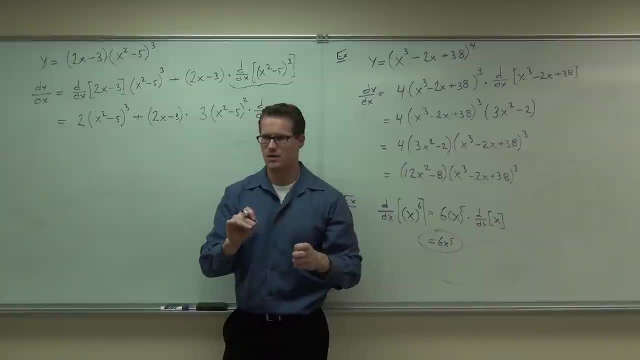 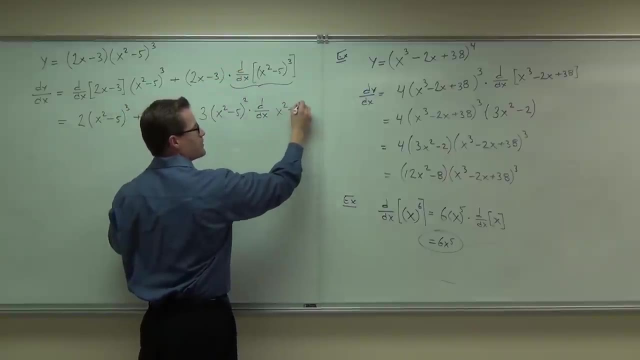 If you make a mistake. I'm not saying you will, But if you do, I want to see where that's happening. Do you get me? Do you get me? Show me those steps? OK Times. the derivative of x squared minus 5.. 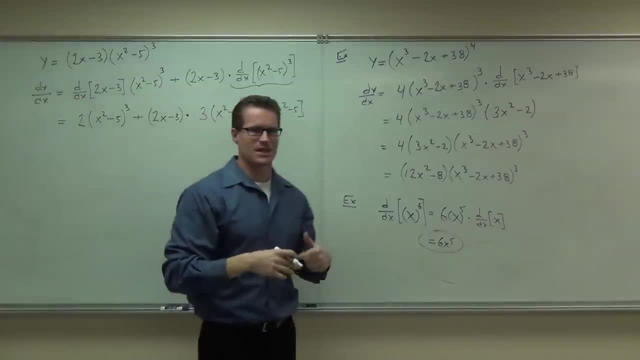 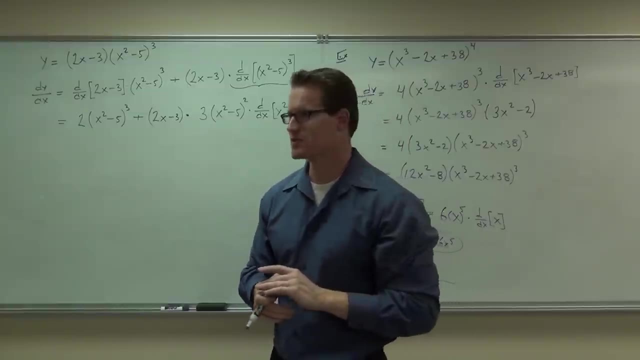 Remember that we're multiplying here. Are there any other ddx's to take care of? Yeah, OK, I hope so. Yes, we do, We have a ddx. What's the derivative of this little piece? So if you follow that ddx down, that, 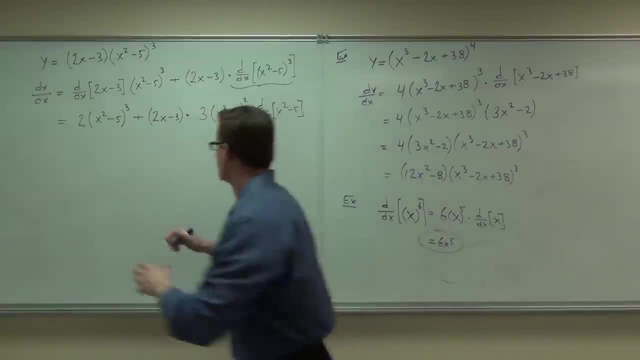 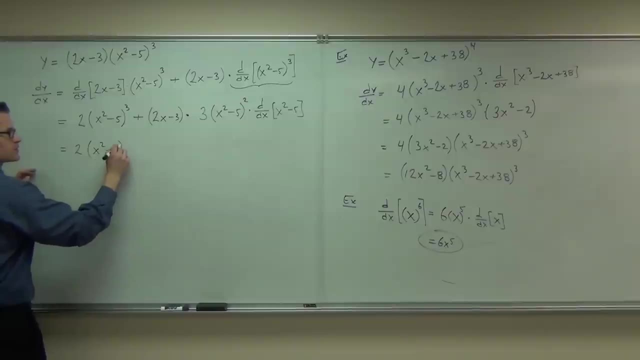 tells you where to take the derivative of or what to take the derivative of. So we're basically all done up until that point. We have 2x squared minus 5 to the third. Let's not mess up any exponents: 2x minus 3 times 3x squared minus 5 to the second times. 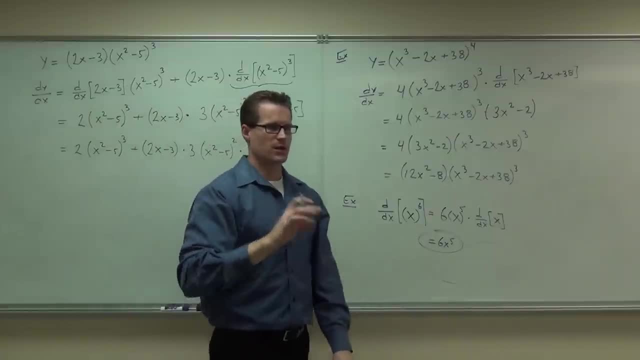 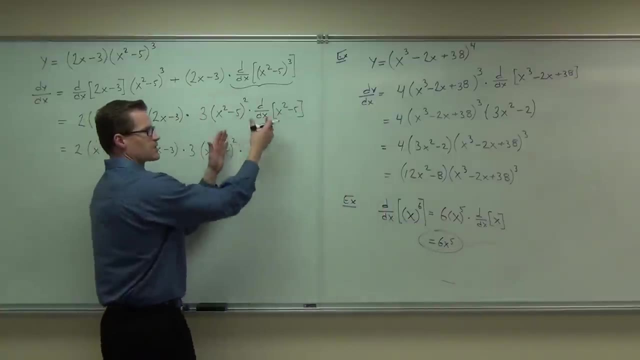 what is the derivative of that little piece? Notice how we kind of eliminated some of the bigger rules right. In fact we used product rule That helped us down to just have one more rule left. We had a general power rule. Now we have just a very simple power rule. 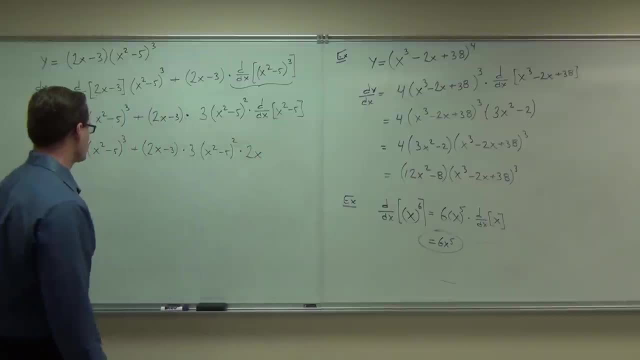 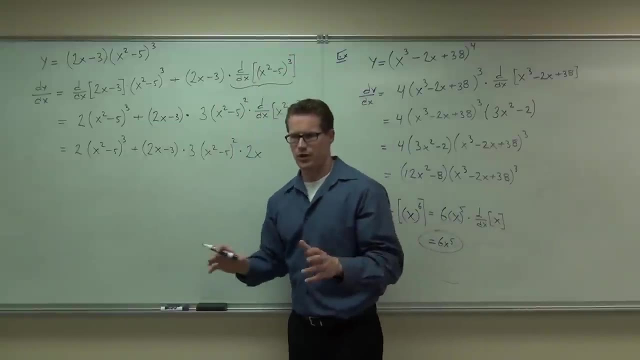 OK, And we're good to go. Richie, I feel OK with this. so far, You can't get this over with. Now we're going to make it prettier by using a little bit of algebra And you're going to see something. 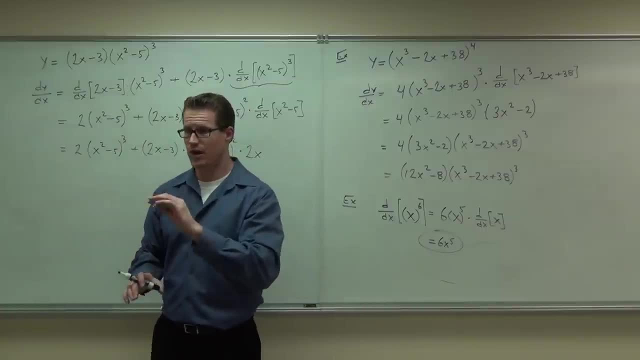 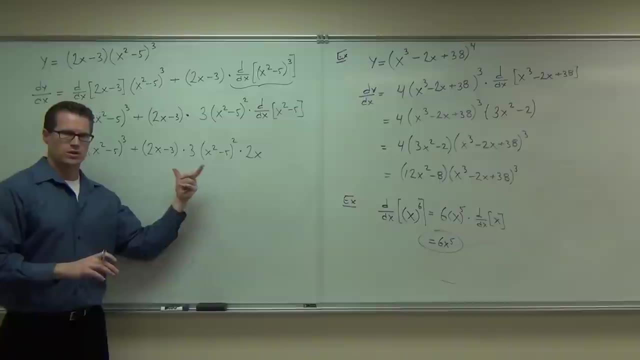 that happens often when you have a product rule that involves a general power rule, You're going to see some pieces that keep reappearing. See how that thing appeared again with our product rule Because you had the original and then you took a general power rule, where that piece shows up again. 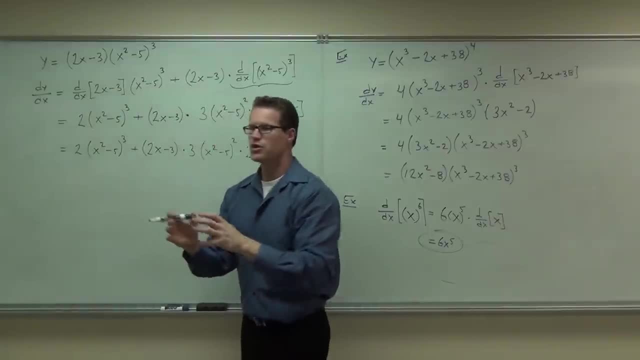 A lot of times that happens. What happens when you do the product rule and you have a general power rule? You're going to want to factor that at the end. It makes things a lot nicer. So I'll show you what I'm talking about. 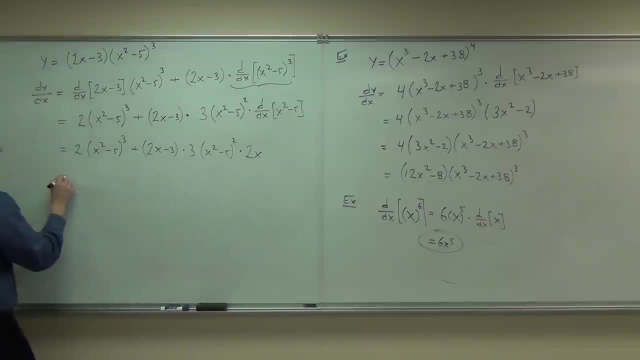 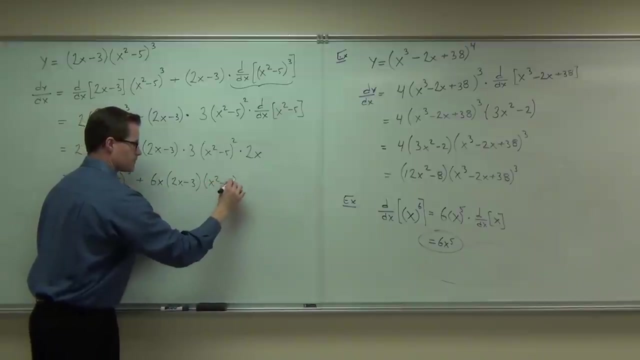 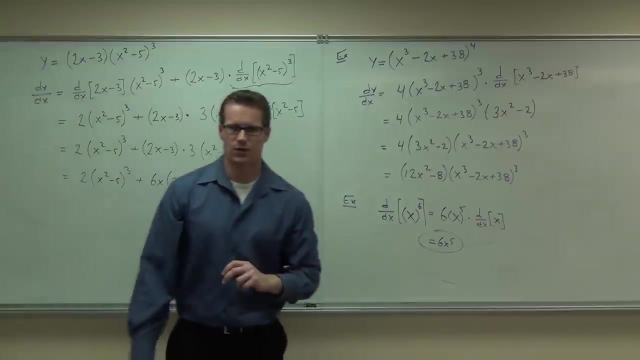 If we go ahead and maybe make this just a little bit prettier, we have this. This becomes 6x, like that. Are you OK with that so far? Yes, no. Do you see the factorization of what I'm talking about? 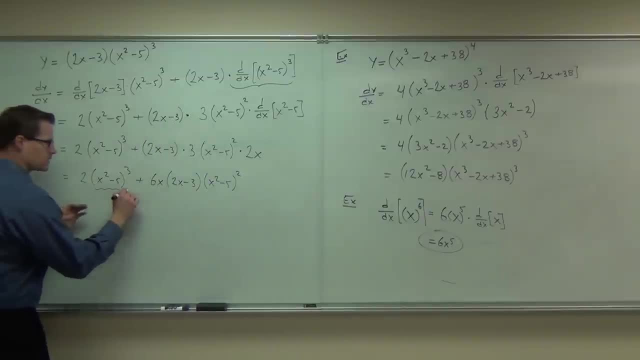 We have this big factor and this big factor right there We can pull out. What can we pull out of that? If I pull out the x squared minus 5 squared, what I end with is 2.. 2's still there. 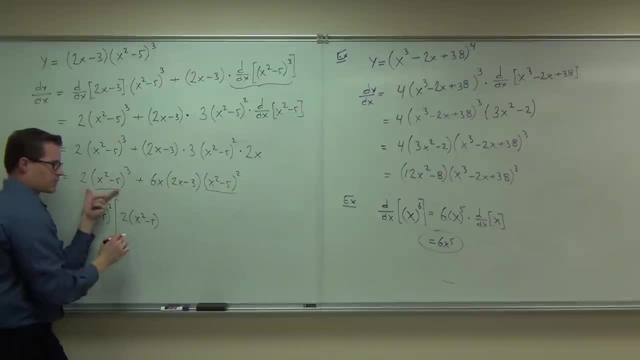 2's still there. x squared minus 5 to what power? 1. Good, because I pulled out two of those things. Does that make sense to you? Plus 6x, 2x minus 3.. Are there any of these left? 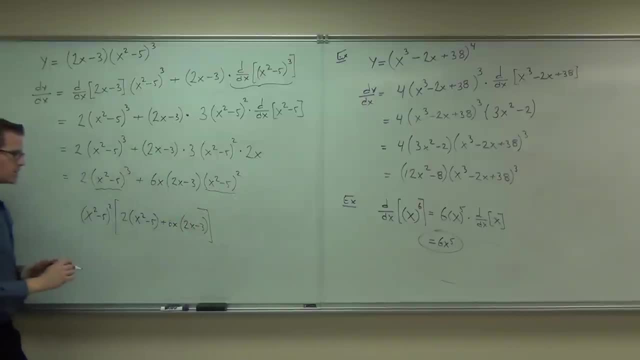 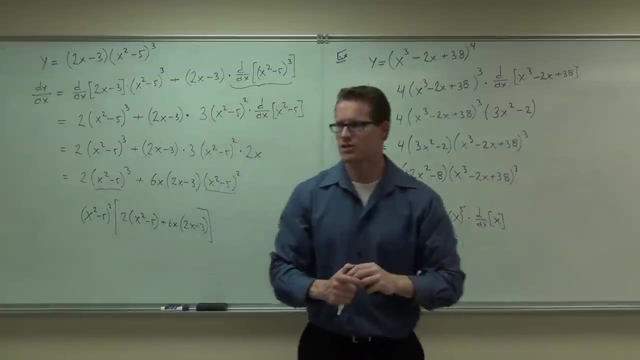 No, I factored that out. Notice, you can get the same thing if you distribute. This distributes and give you this, This distributes and give you that. So that's factorization right there. I'm pretty sure you feel all right with that so far. 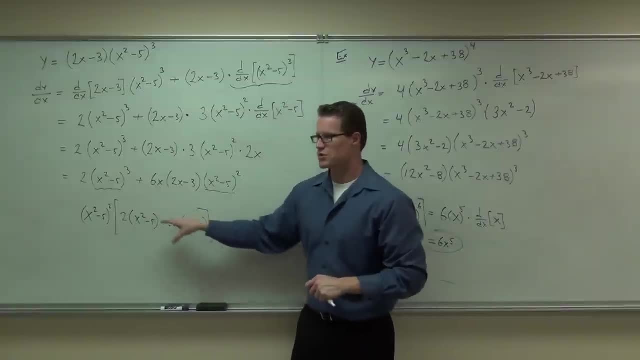 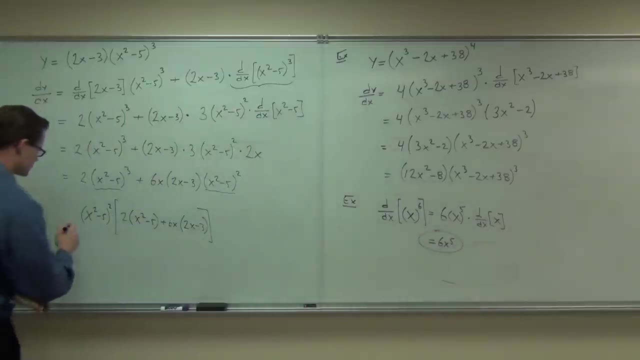 The next thing you do: distribute this and combine like terms. If you distribute this and combine like terms, you'll have a much simpler looking polynomial In here. we get our 2x squared minus 10.. We get our 12x squared minus 18x. 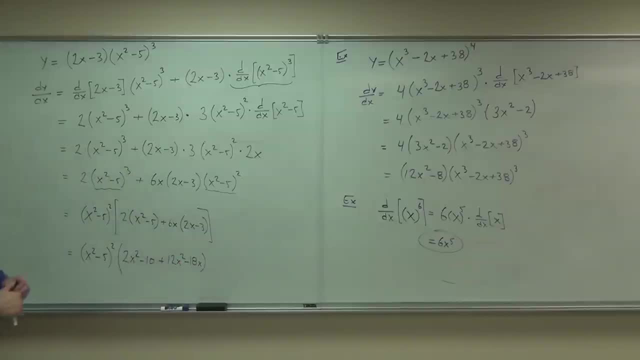 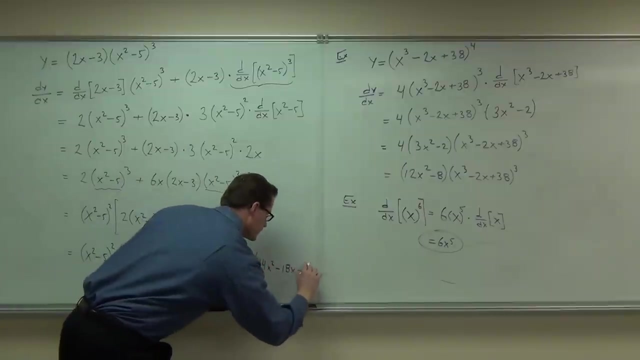 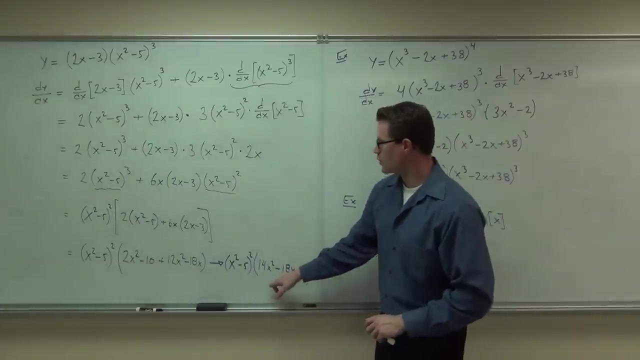 If I did it right. did I do it right? Yes, If we combine some of those like terms, I'm seeing 14x squared. I'm seeing minus 18x minus 10.. Now, hopefully it's not just me, but this thing looks a whole lot more concise than that thing. 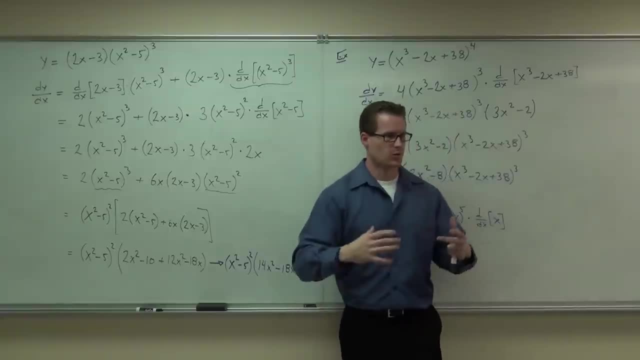 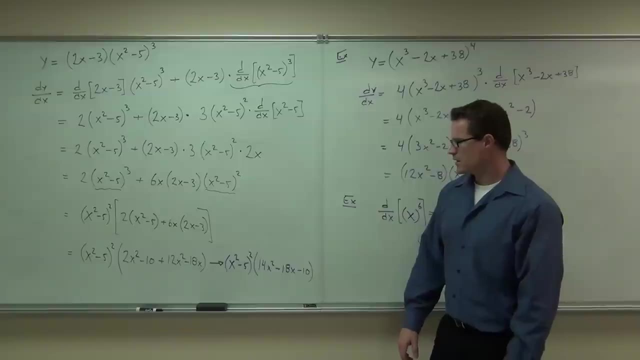 Does it not? It looks prettier, It looks better, It looks more concise, more wrapped up, And that's where we want to end our derivatives, if we can make it that far. Show of hands: how many people feel okay with what we've done so far? 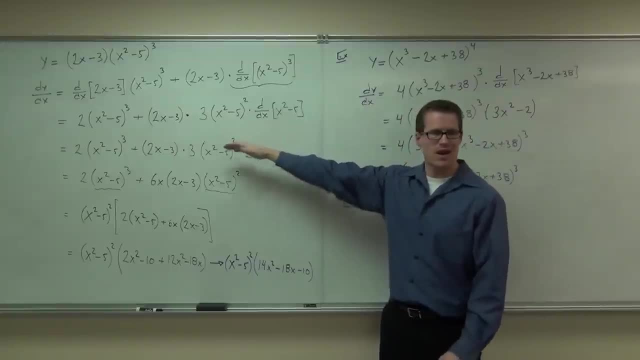 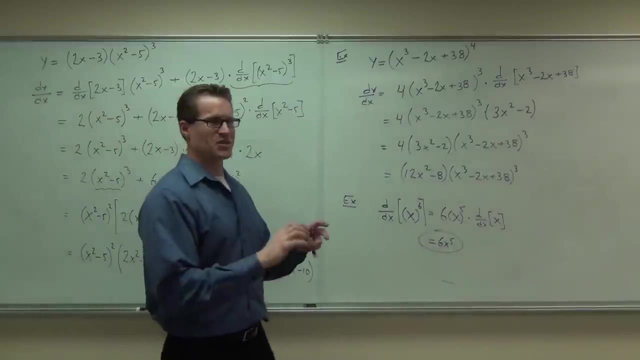 At least up to the calculus being done part. Are you okay with the calculus being done part? After that, it's just algebra, some manipulation. That's okay, We can do that. By the way, this is the part where people lose track in this class of what you're actually doing. 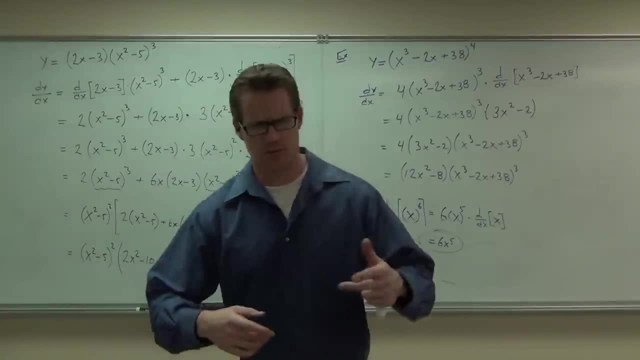 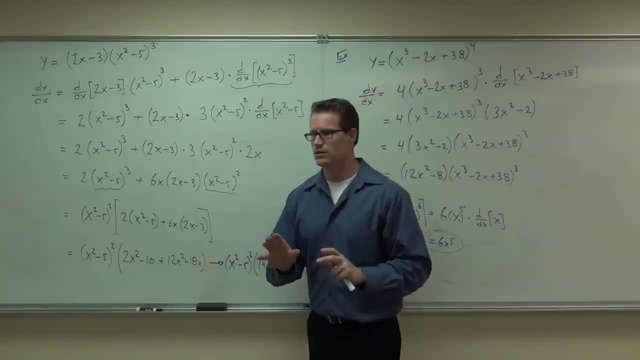 Okay, They just get to the, they go. oh yeah, general rule and part rule and partial rule and chain rule. They lose track of what you're doing. What did we just do? We found the what Slope? We found the slope. 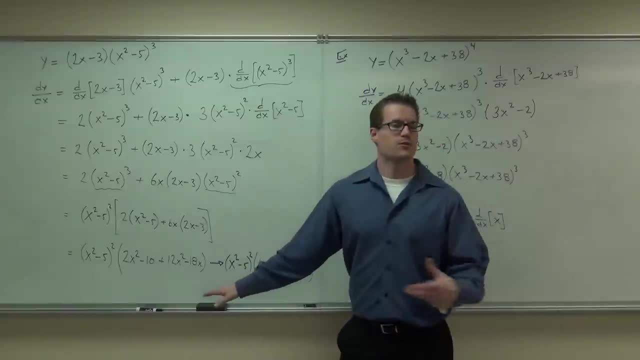 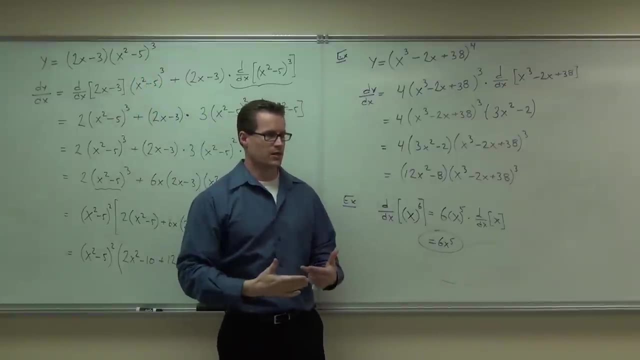 That's. all we're doing is find the slope. This is the slope, This is the formula for the slope of that curve at any point that I want. So could I still find that equation of a tangent line at a point? Sure, I plug in the x coordinate to here to find my slope. 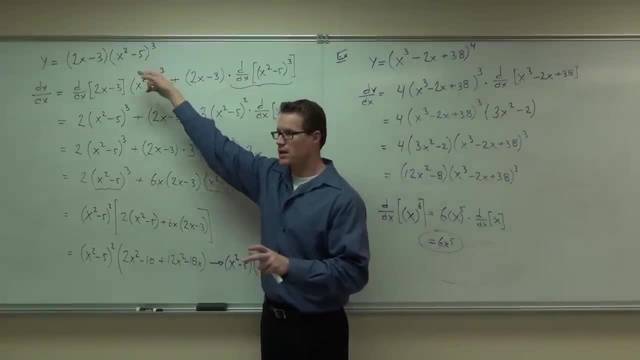 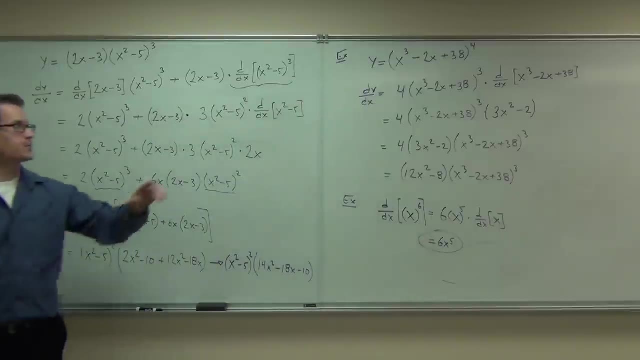 I plug my x coordinate into here. I plug my x coordinate into here to find my point. Then use y minus y1 equals mx minus x1.. That's all we're doing, Okay. We're finding slope. Or, if this is a position curve, we're finding velocity or rate of change. 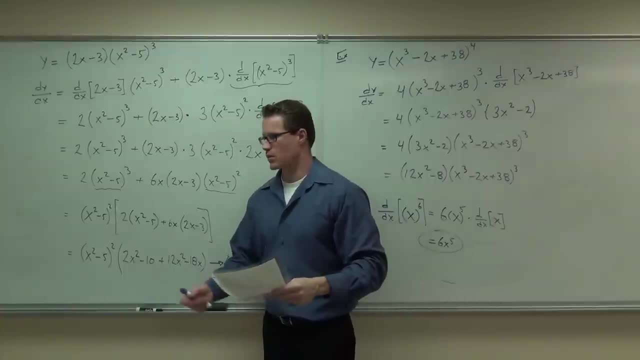 Or if it's a cost function, we're finding marginal cost, marginal profit, things like that. Very interesting stuff. Let's try a few more. I need to show you how the chain rule is going to affect something to do with like a trig function. 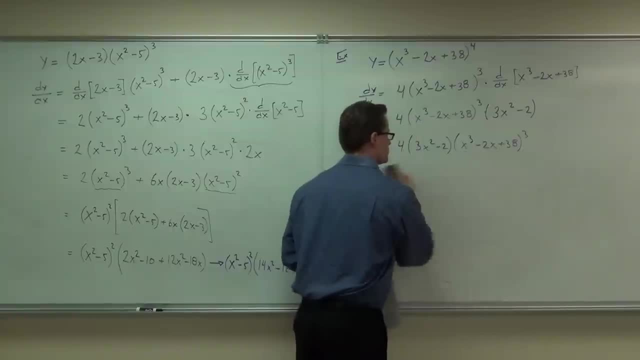 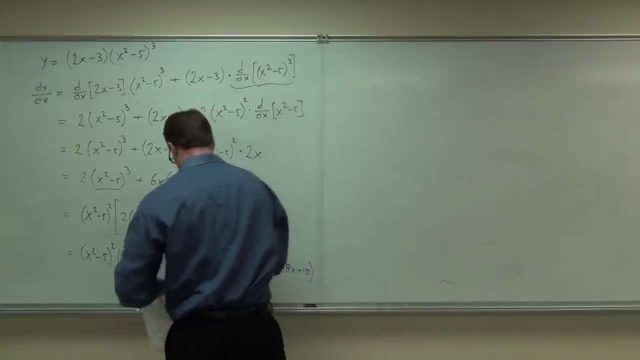 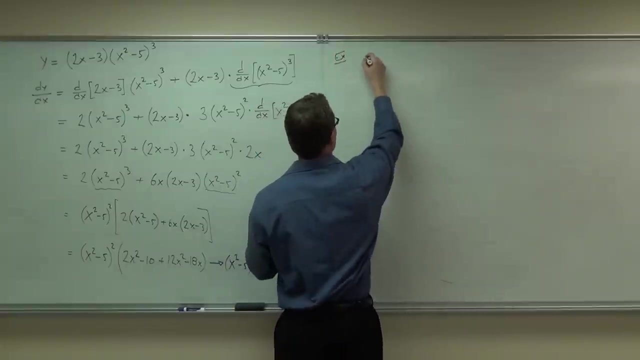 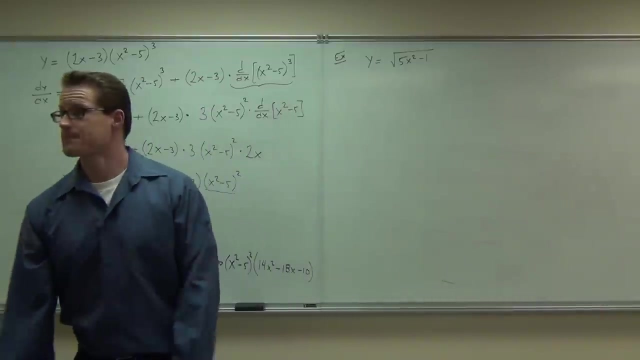 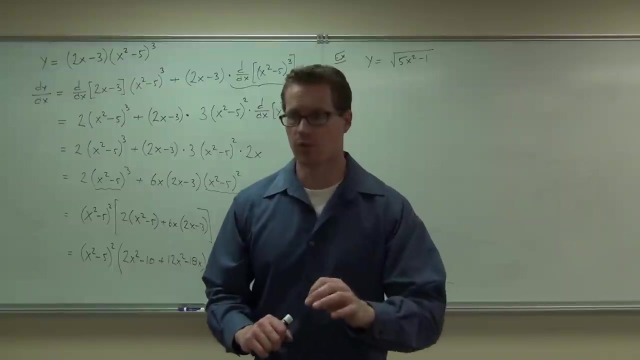 And that will probably be about our day. Does the chain rule still apply? Yeah, What do you think? Seven, Do I have a function within a function? basically, That's what you're asking, Because if you do, then you have a chain rule. 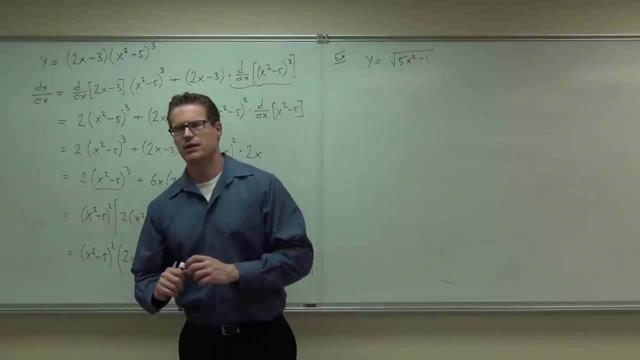 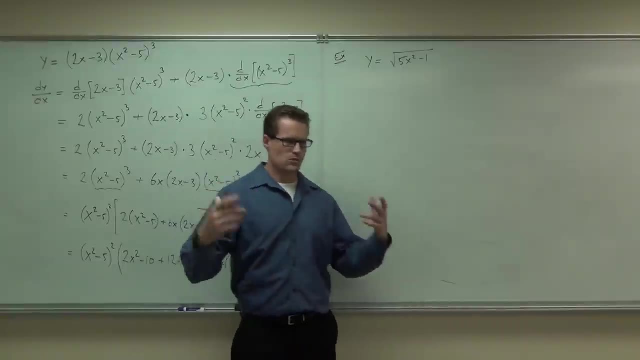 Do I have a general power rule here? Yes, Well, explain that, Explain how I have a general power rule, because I don't see an exponent right now. So, in order to do this, well, hopefully you remember this from the last couple sections. 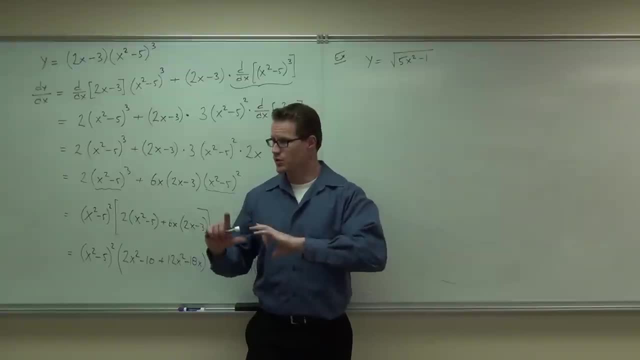 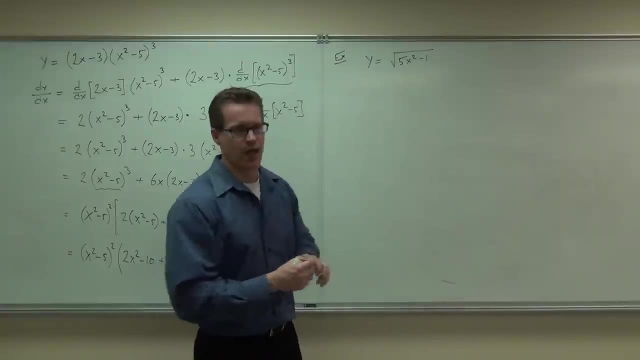 In order to do the derivative, you really need to represent roots as exponents, right? Because we know we deal with that. We subtract one from them. You can't subtract one from a square root unless you write it as a one-half. 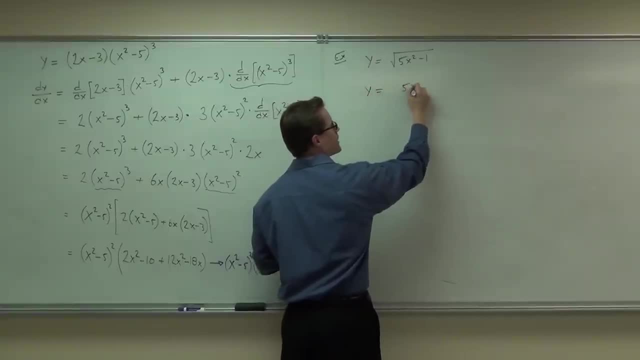 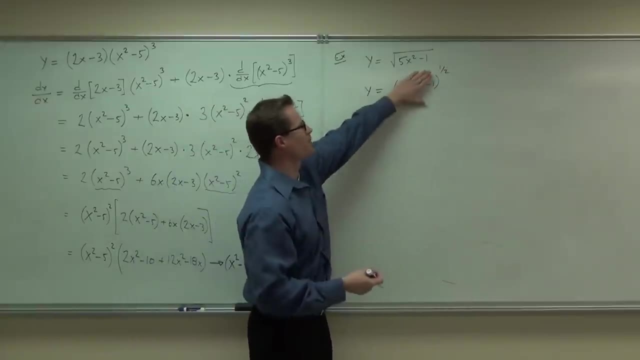 So first thing to do is go: yeah, all right, I know that this is 5x squared minus 1 in parentheses, to the one-half power, And that right there says aha, aha. Look if you can cover it up. you're talking about a composition within parentheses. 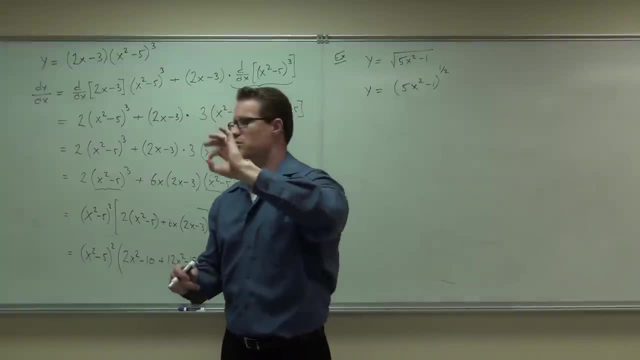 You're talking about a composition, That means chain rule applies In this case. it's an exponent, so the general power rule applies. Why don't you go ahead and try it? Go for it. You're at that point at this stage. 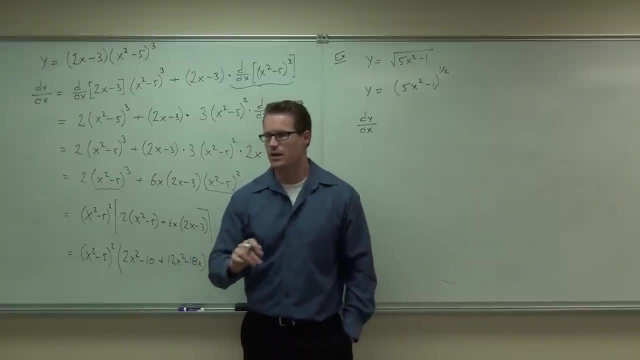 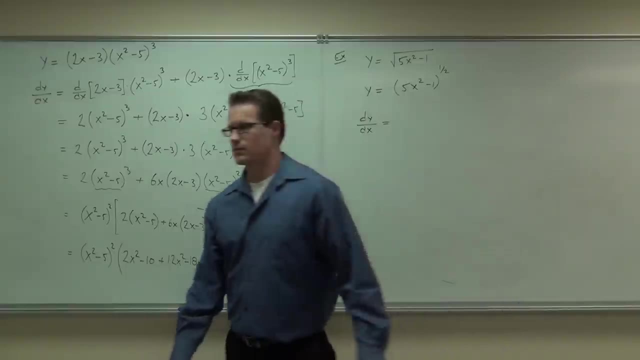 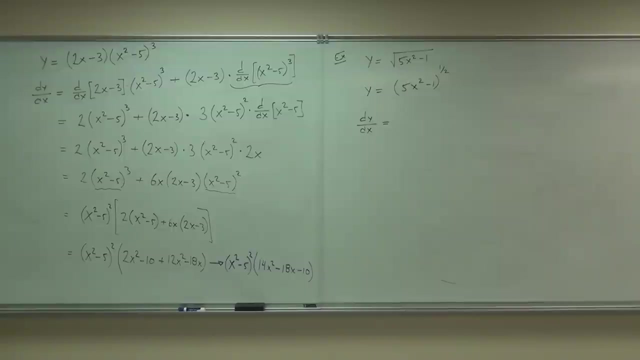 Remember, I really don't want you doing the work all in your head. I want to see the steps right now. I want to see the DDX written out. Did you make it that far? One-half, 5x squared minus 1 to the negative one-half. 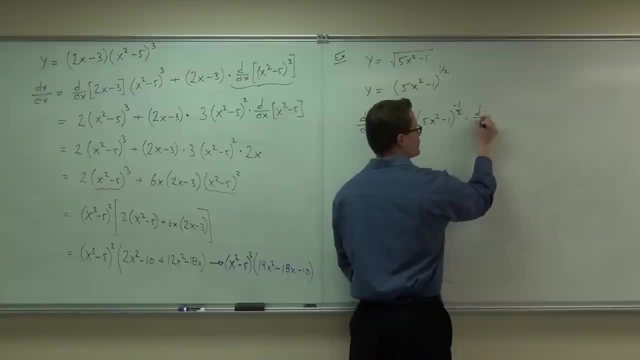 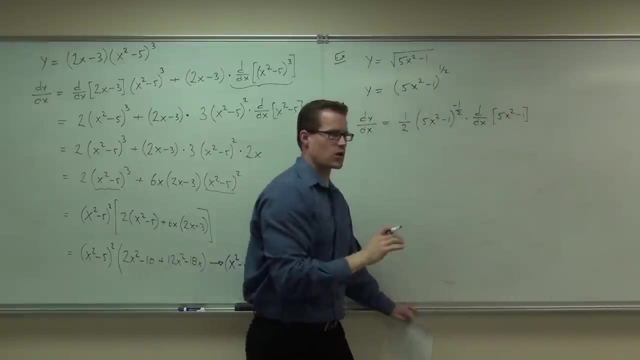 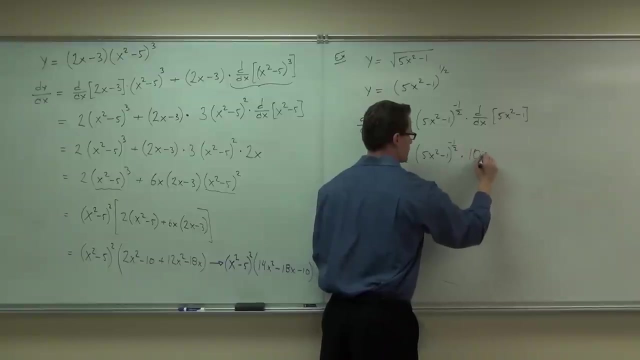 Cool. Inside doesn't change for now. And then we take the derivative of the function itself, the inside function of our composition or the piece of our composition. If we take that derivative, then we're just about done. Did you get the 10x too? 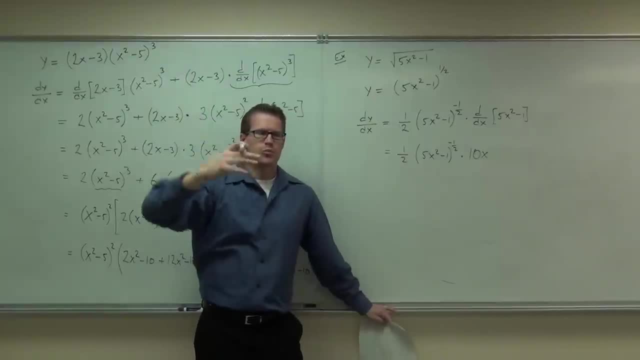 How many people got exactly that on their paper? Good for you. Now make it a little prettier. Here's how you can make it a little prettier: The one-half and the 10, that simplifies. That simplifies and gives you 5.. 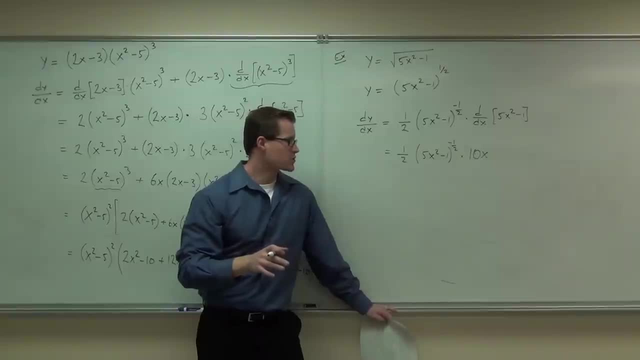 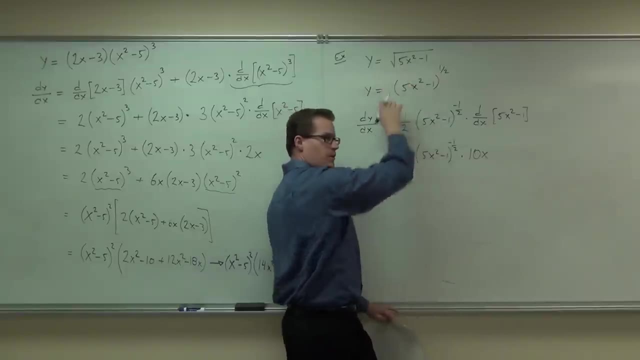 So we have 5x and then we have this 5x squared minus 1 to the negative one-half. How you can write that, How you can write that appropriately- would be: since you started as a square root, you probably want to end with some sort of root. 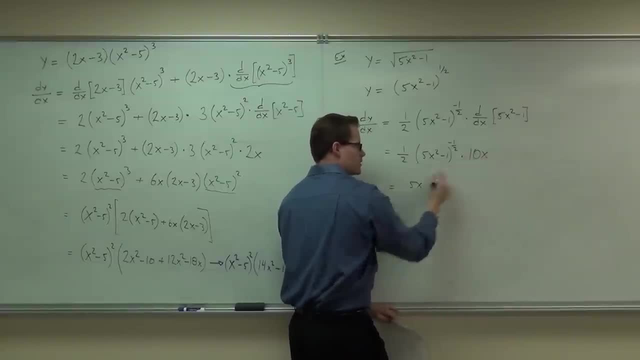 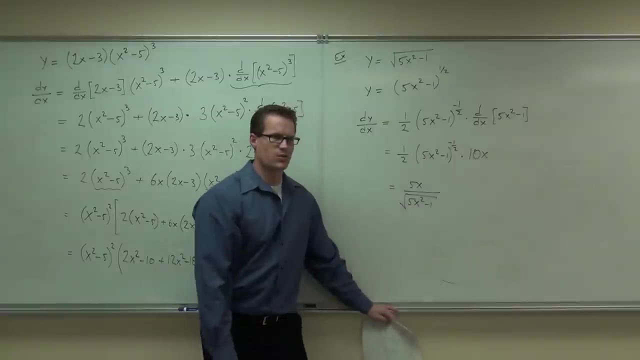 We want 5x on the numerator, 5x on the numerator, 5x squared minus 1, and a square root on the denominator. Do you see why it's on the denominator? firstly, It's that negative one-half that moves to the denominator. 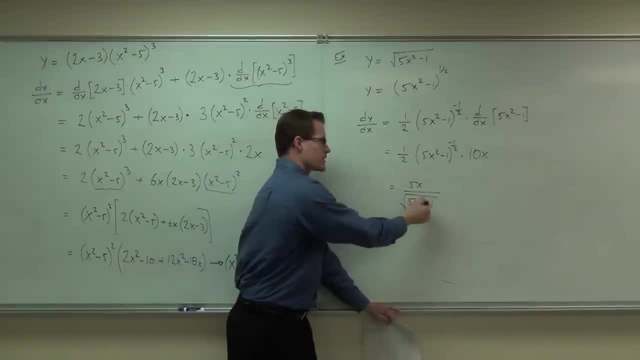 The one-half becomes positive. That's a square root. Can I cross out the 5x and the 5x squared? No, Oh heck. no, I see that. I see that all day long. All right, I agree. 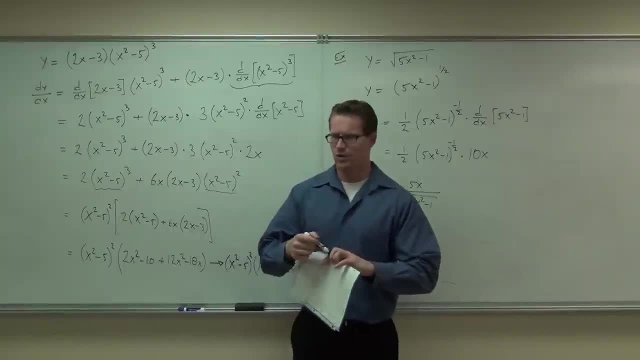 But no, we can't do that. Are you ready to move on from the general power rule? Because that's about all I can show you with that. I mean it doesn't change after this. If you can do these couple problems, you're okay so far. 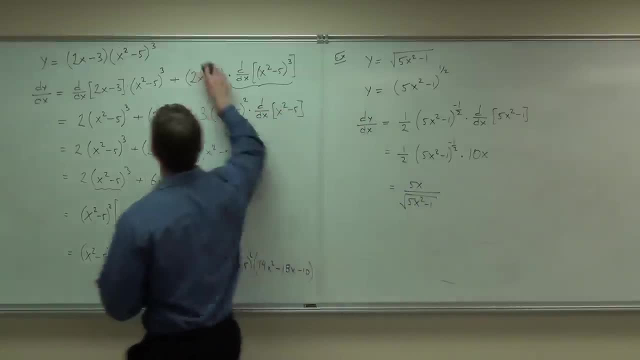 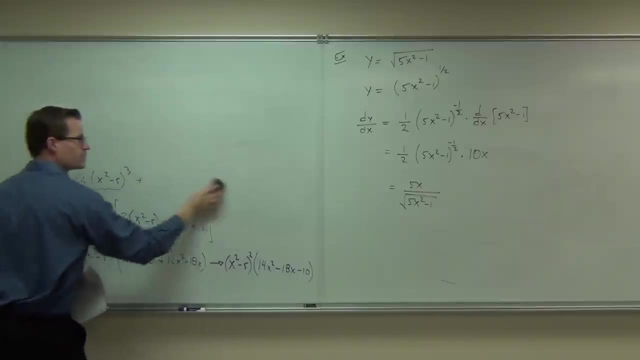 Are you okay so far? Wouldn't even an exponential form still be acceptable If it's given to you that way? What I'm expecting most of the time is it's actually not going to be that way Most of the time. if I give it to you as exponents, exponents are fine. 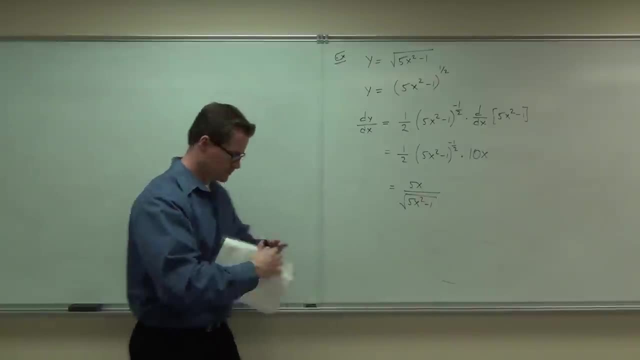 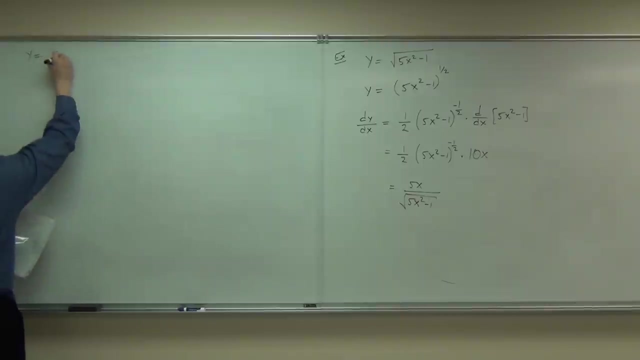 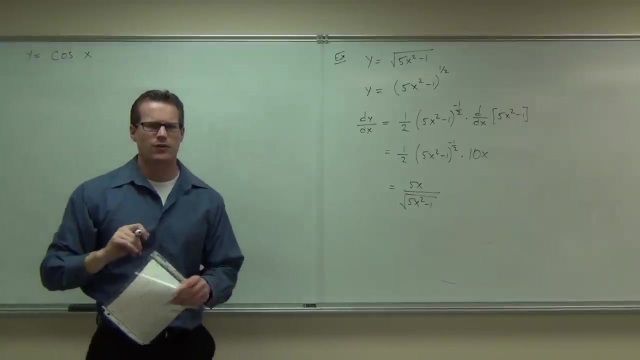 If I give it to you as roots, change it back to roots. Can you do that derivative? That would be what folks- Oh, very good, You're memorizing it. Fantastic. Can you do that derivative? Yes, Yes. 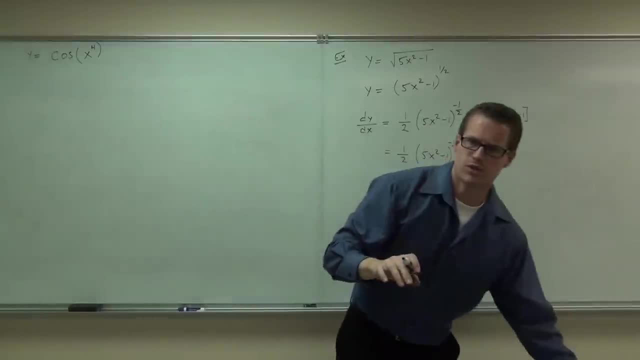 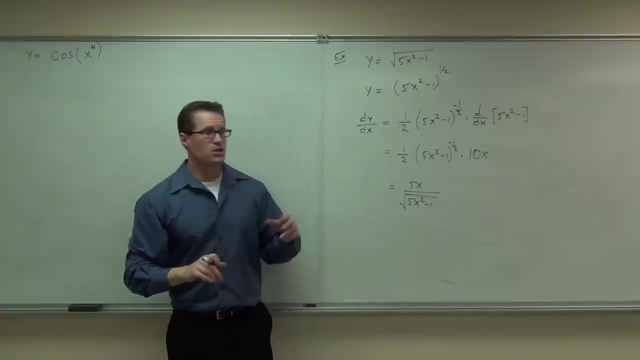 Yes. So the answer is no, not with what you know. Well, actually yes, because we just talked about, But not what you knew before today, The answer would be no. But let's look at it. Do you have a composition going on in this? 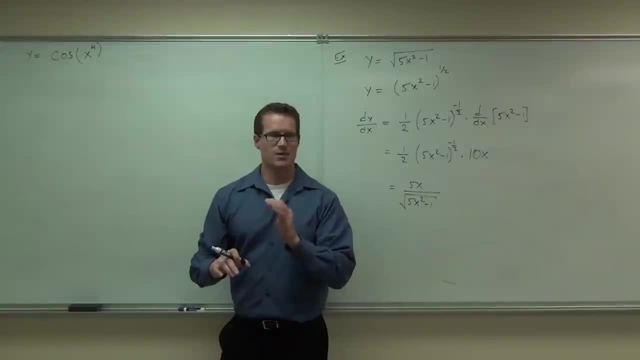 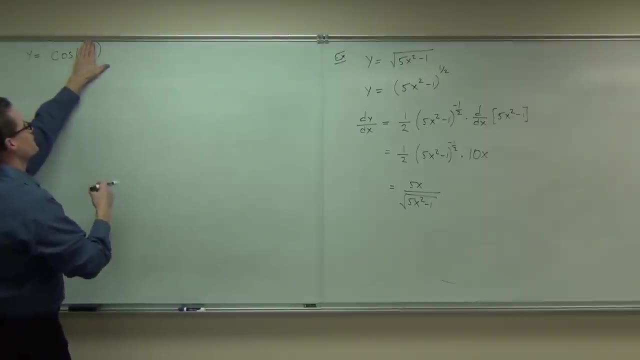 Which means can you cover up a piece of it and get some other function? basically, If I cover this part up, so I say: cover up the inside. We're always talking about covering up the inside, Cover the inside and say, well, let's let Y equals cosine of U. 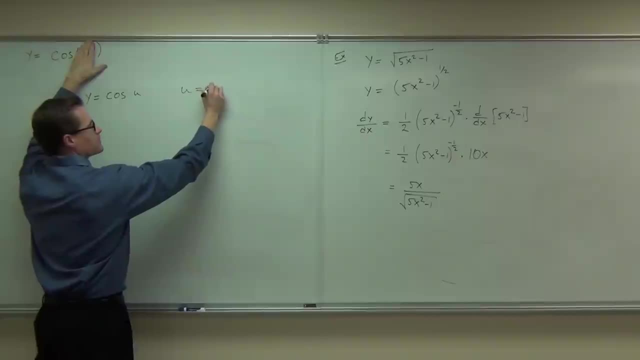 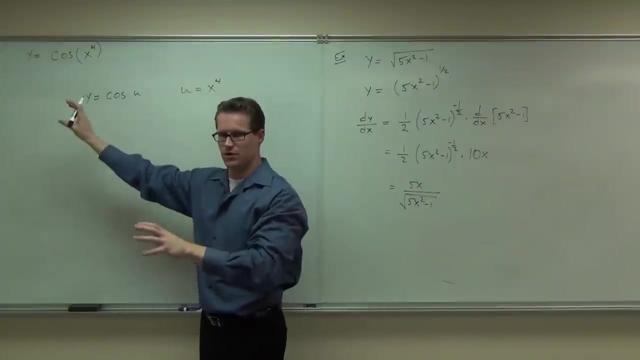 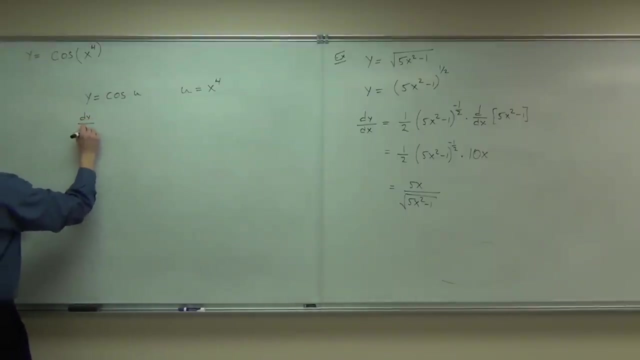 And U equals whatever's under my hand. Would that be an appropriate composition? Because if I let the U go in for U, in fact X to the fourth go in for U, then I get that back again, right? Well, if we find our DYDU, what's DYDU here, ladies? 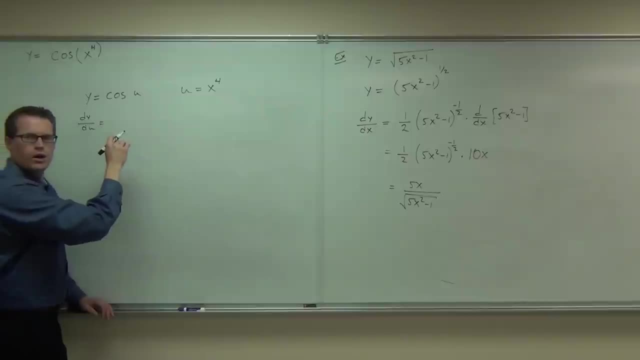 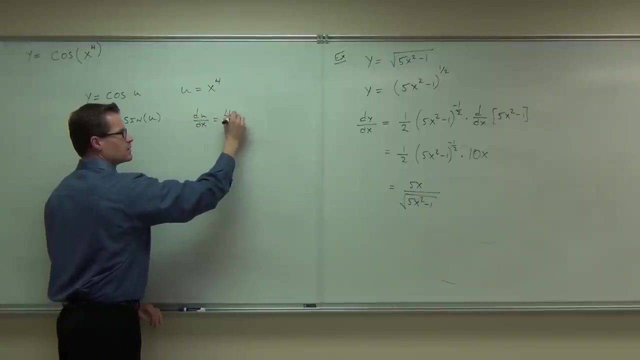 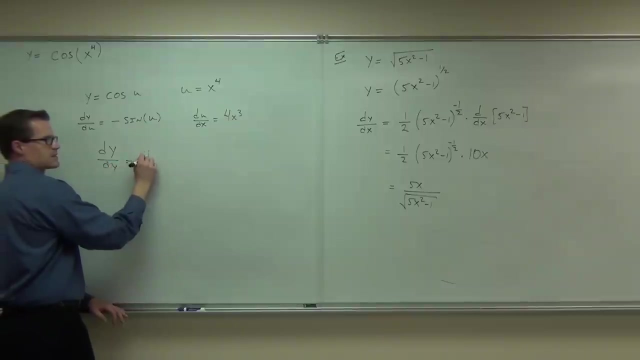 and gentlemen, We just talked about it: Negative sign, Negative sign, what U U? Negative sign U and DUDX, What's DUDX? And we knew that DYDX is DYDU times DUDX, True, True story. 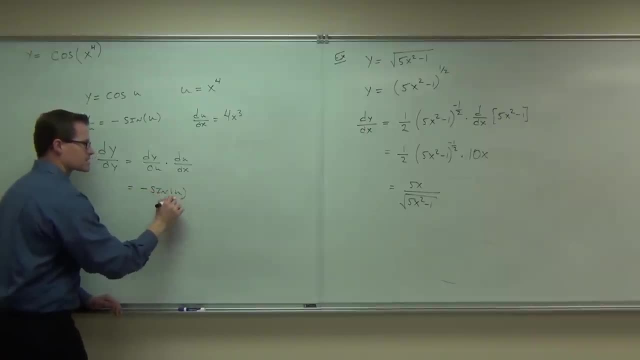 This is negative sign. This is negative sign U because that's DYDU, That's this Times DUDX, which is 4X cubed DYDU, DUDX, DYDU, times DUDX. That's chain rule. 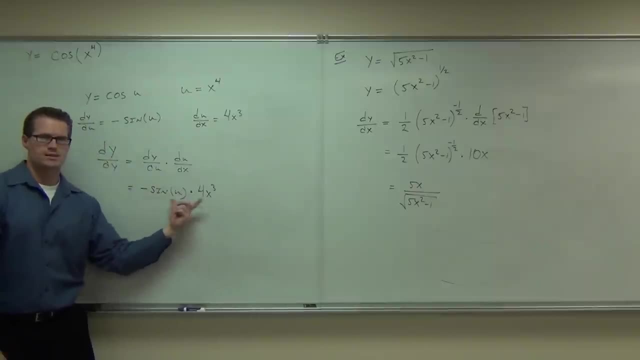 We just talked about that. That's this right here. What's the one last thing that I need to do? Substitute. Why do I need to substitute? Don't want to end with U's and X's. We'll make it prettier, but that's the one I want to talk about. 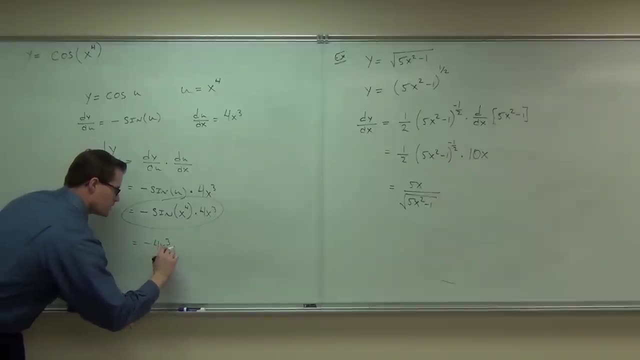 This will ultimately become negative. 4X cubed sine of X to the 4th. That would be the derivative of that curve. Are you okay with how to do that? We've got 4X cubed up front. Notice what you can't do. 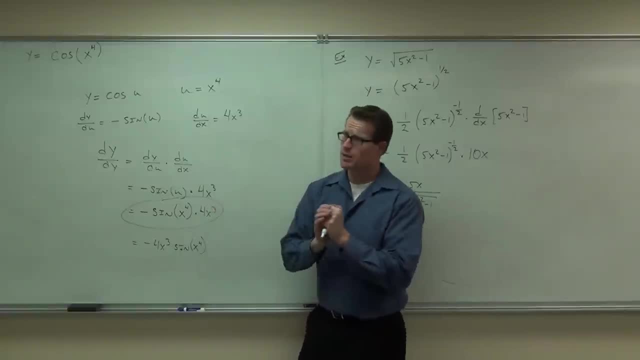 Oh, please, goodness, I'll do this. Please, don't, please, please, don't ever multiply those. That's an angle. This is not This. you cannot make 4X to the 7th. If you do that, I'm going to burn your paper. 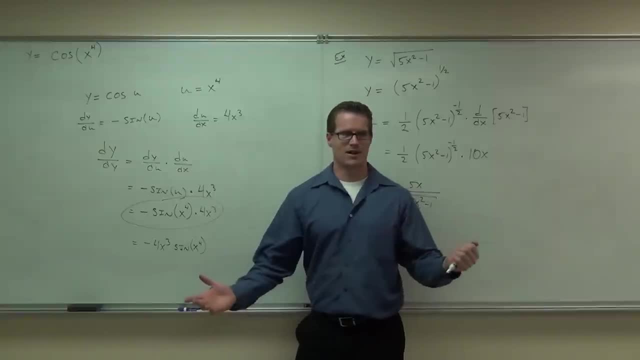 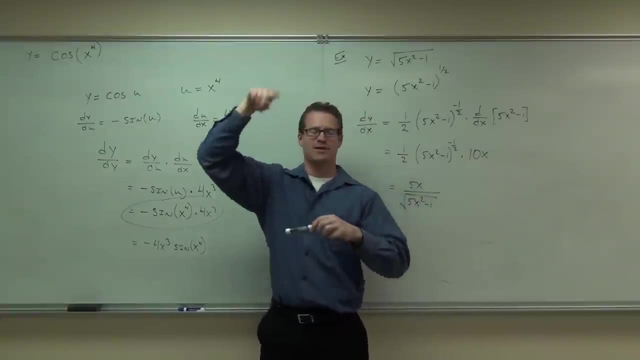 I'll burn it. Gone, What homework. I didn't see any homework from you. I'm just going to burn it. This is an embarrassment. I'm just going to do that, Just kidding. I wouldn't burn it, but I will go no, with like five exclamation points and underline it. 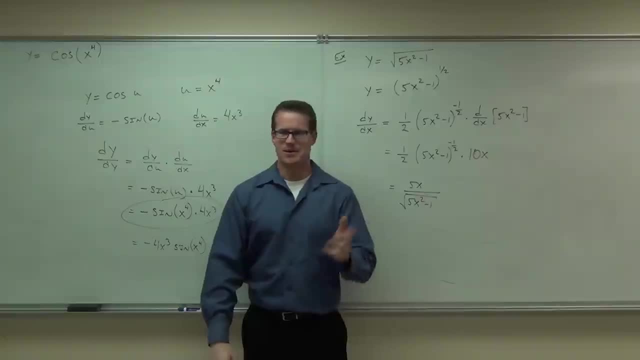 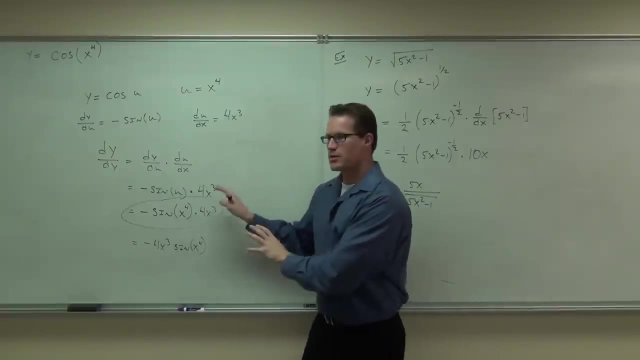 and scribble on it and stomp on it. That's about it. I'm not going to kick a puppy, Not that bad. but are you okay with this? Here's what this says in English. We'll stop here. This says: in order to do the chain rule with this type of thing. 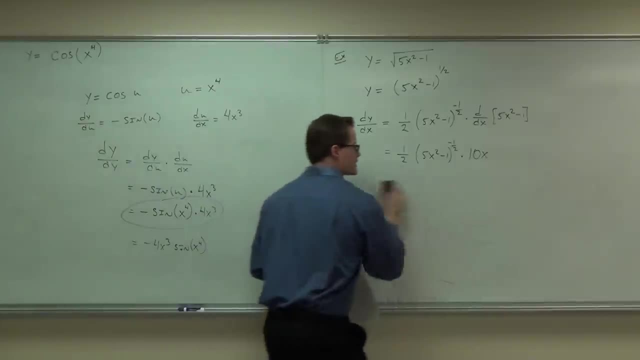 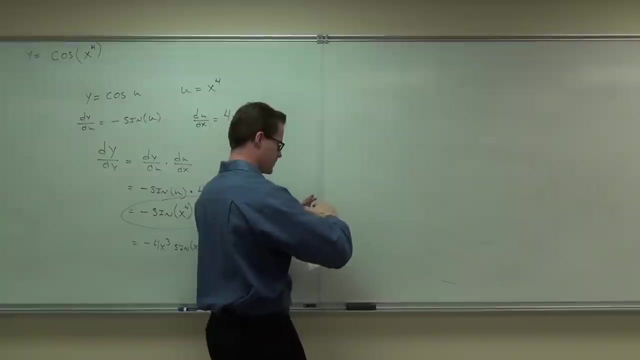 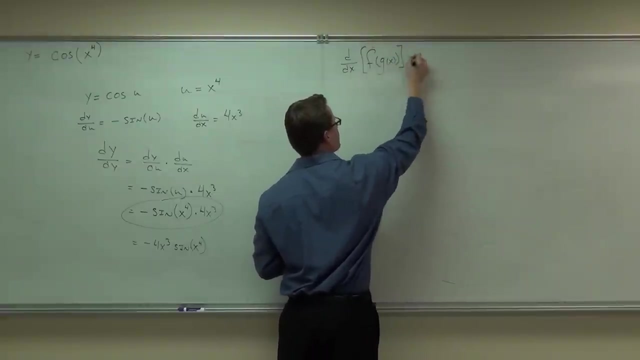 you really don't need to show me this. This is just the underlying work. Here's what it says in English. Well, I have a little bit of calculus. It says: if you want to take the derivative of composition, such as we just had right now, here's what this said to do. 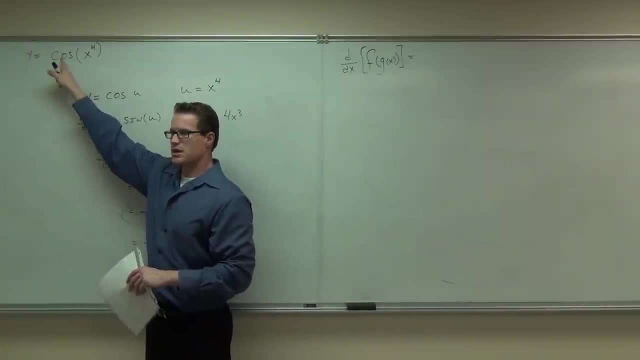 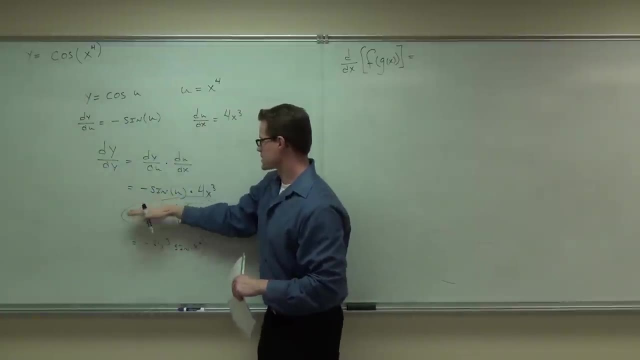 It says: I want you to take the derivative. Look what it does, please. It says: take the derivative of cosine, right? What's the derivative of cosine? Negative sine, Negative sine, and leave the inside alone. Does that look familiar? That's exactly what we do with general power rule, right there. 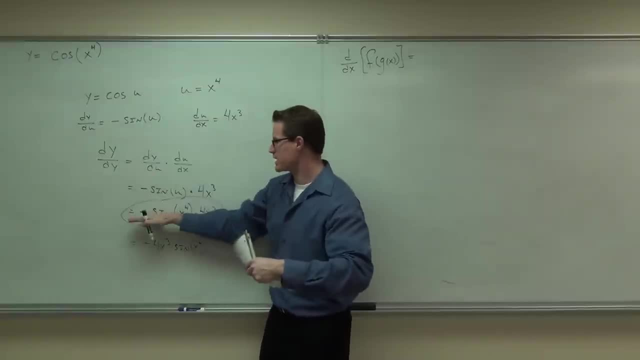 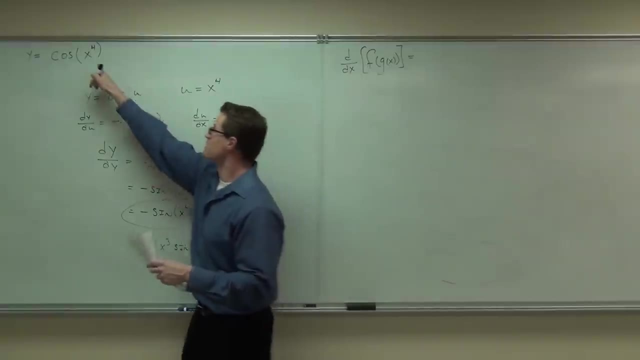 Take the derivative of the outside, The outside function, the cosine in this case, but then you just can't forget to multiply by the derivative of whatever the inside was. And that's what this says. Take the derivative of the inside and multiply it. 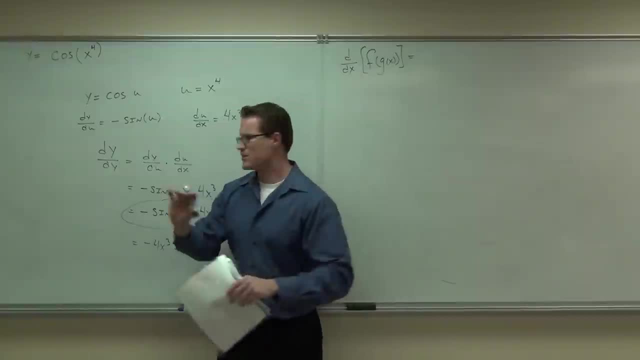 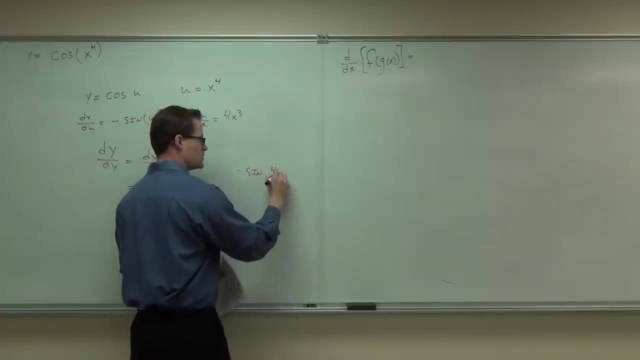 That's what we do with general power rule. A lot of people do this. They'll give me this all day long. Oh, it kills me, They say. oh yeah, the answer is negative. sine of 4x cubed. 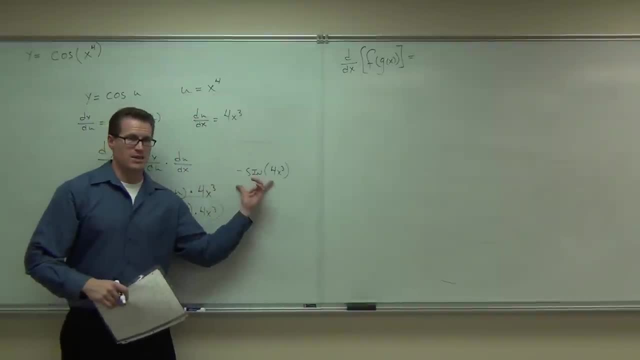 I get that all day long. See the common mistake that people would make to get that. They go: oh yeah. derivative of cosine, negative sine. Derivative of the inside 4x cubed. Is this right? No, because they have not applied the chain rule. 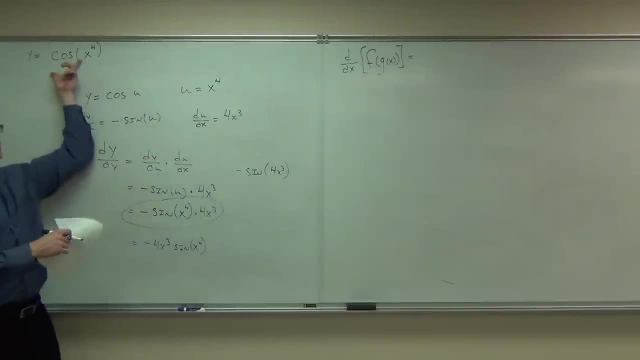 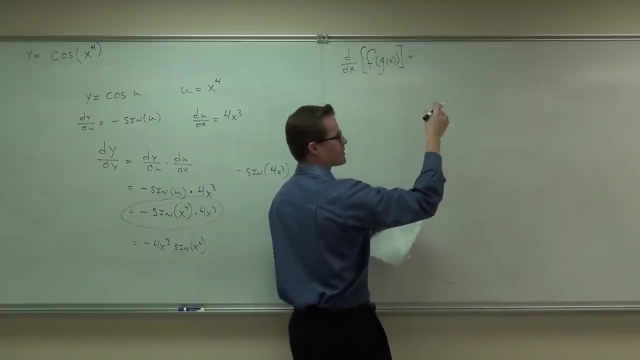 Chain rule says you have a composition. here You need to take the derivative of your function. sure, leave the inside alone, then multiply by the derivative of the inside. So this says you take- I'm going to use a kind of combination of rules here. 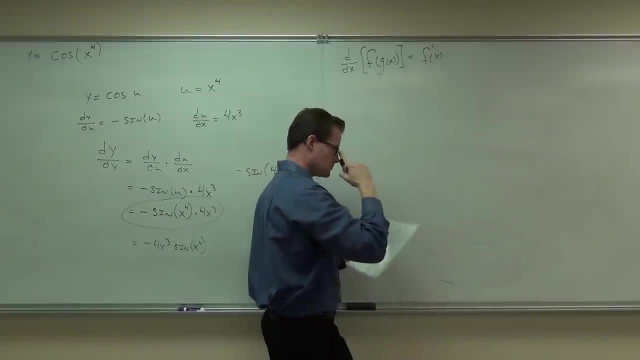 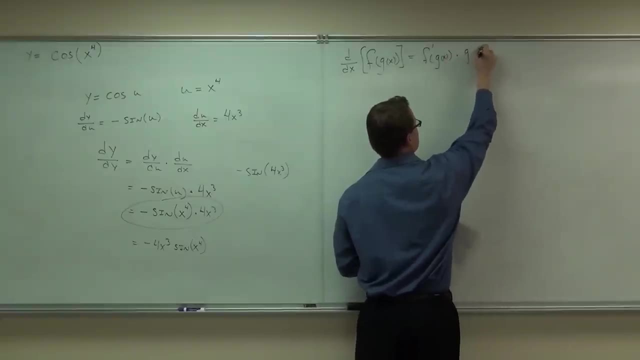 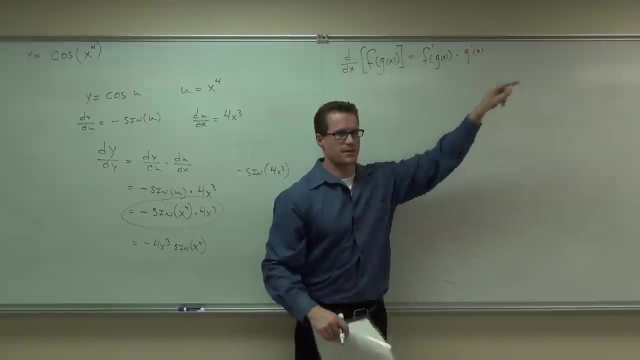 or sorry notation: you take f prime of x. I'm sorry. f prime of g of x times g prime of x. That's what you do. Derivative of the outside- leave the inside alone. times the derivative of the inside. 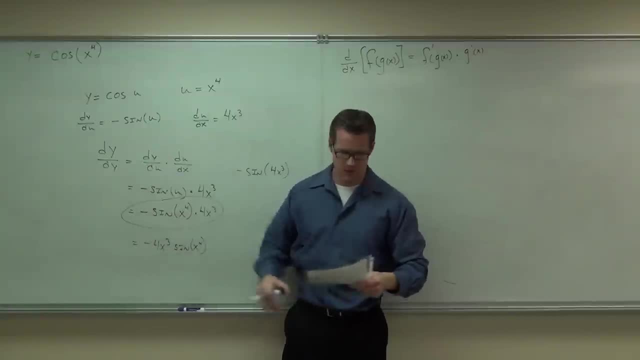 And that's exactly. do you see that over here? Do you see what that means for us here? Okay, good, Derivative of the function times, the derivative of the inside, and that's what we're doing. How many people feel okay with what we talked about so far? 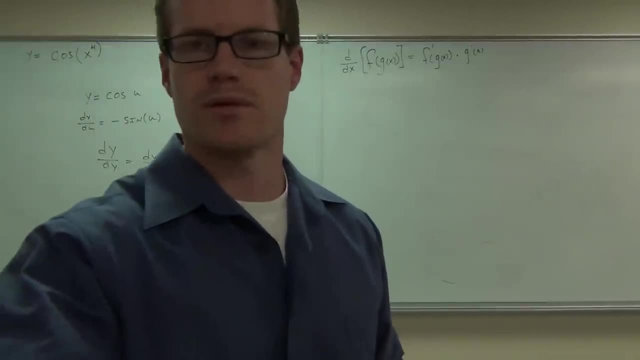 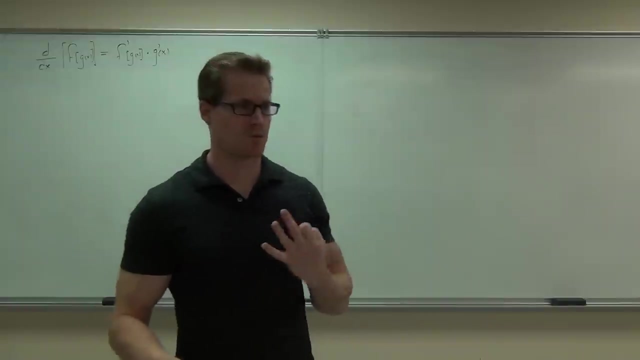 I will start here next time with a couple more chain rules and then we'll keep on moving. So today we are practicing. All we are practicing today is applications of the three rules that we talked about: Chain rule, which includes the general power rule. 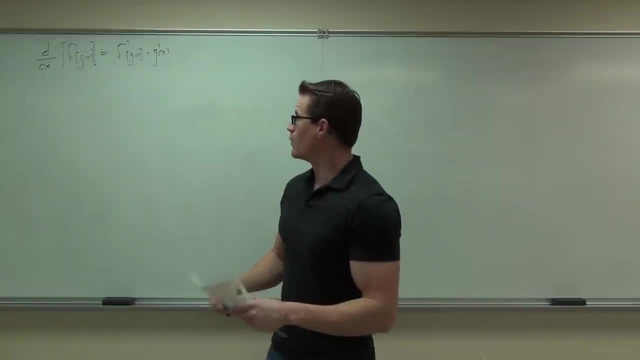 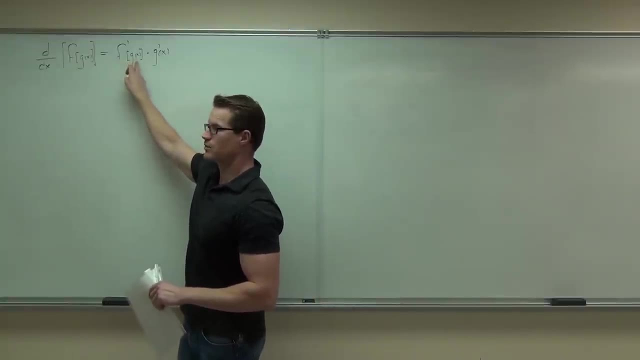 The product rule and the function rule. that's pretty much it. What you know from the chain rule is this. This says in English: you take the derivative of the function, leave the inside alone and you multiply it by the derivative of the inside. 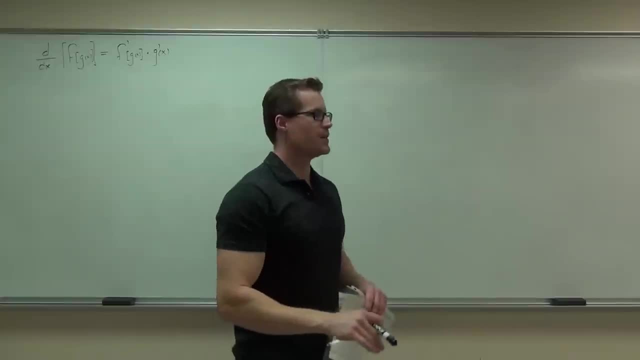 If you can remember that for the chain rule, you're good to go, We'll start simply. then I'm going to start building on some nasty looking problems, Oh my gosh. And it'll take us maybe the whole board to do. 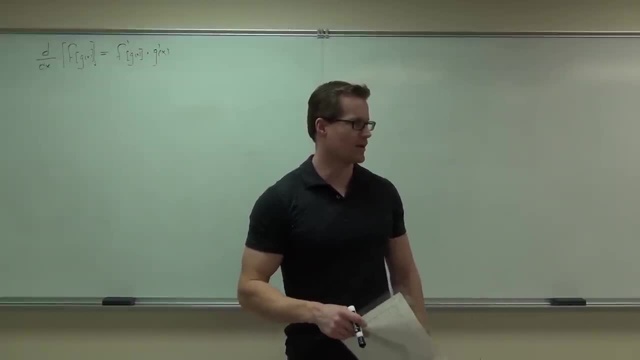 But you need to see them because your homework shouldn't be like that too. okay, I don't want to leave you hanging on this stuff. So we're going to do examples. We're going to do examples. We're going to do examples pretty much all day. 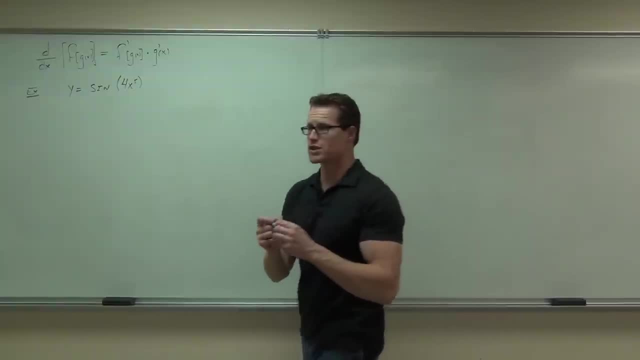 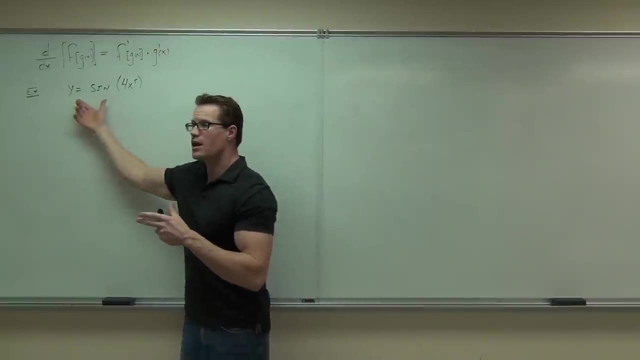 Okay, sine of 4x to the 5th, a couple questions for you. First thing: is this a product rule? Okay, so product rules apply, because this is actually a function. This is really a composition. You know a lot of people who really don't understand trigonometry. they go: oh yeah. 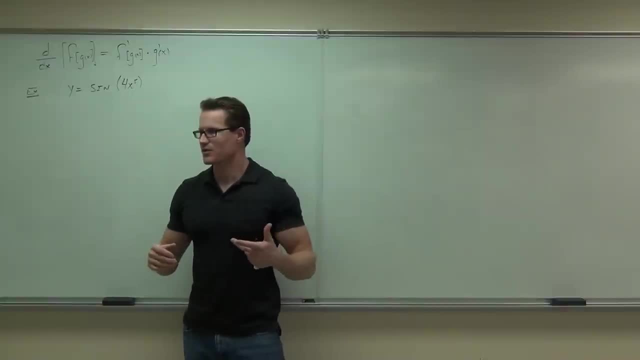 it's sine times 4x, 4x to the 5th, which is not really what we're doing, right, You can't take if I just give you sine, that's meaningless, That doesn't mean sine, that means a sin, right. 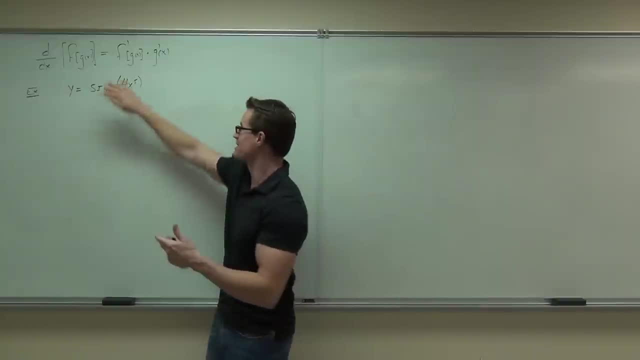 Now, if I give you sine with an angle, that means sine. okay, I'm not going to write sin on your paper. You're not going to write sin. If you write sin without this, you're sinning. You're sinning, right. 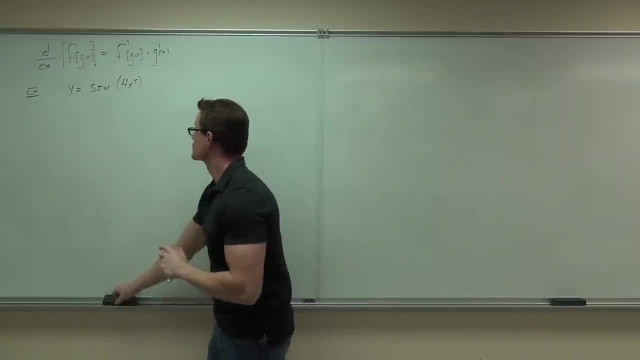 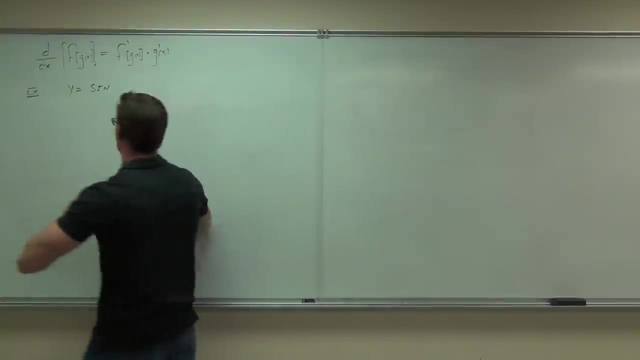 You have to have this part, You have to have something with it. If you just have this, that right. that's not sine by itself isn't meaningless. It must have something attached to it. So this is not a product rule. 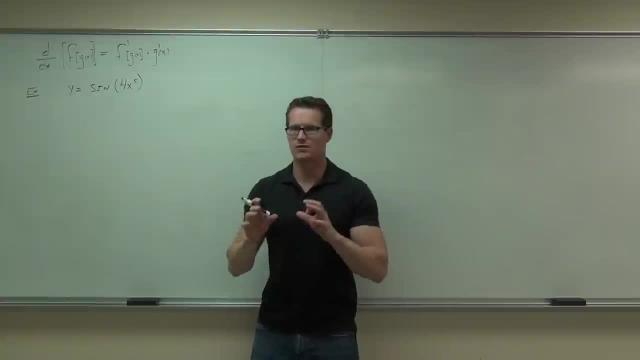 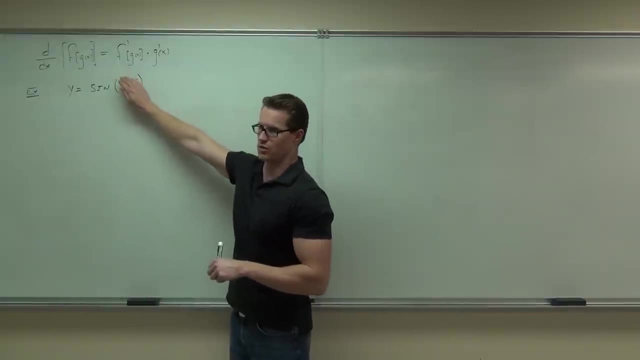 What this is is a composition of two functions, a composition of 4x to the 5th into sine. What that means whenever you see a composition is: a chain rule will work. If you can cover up a piece of it and you still have a function, that means it's a chain rule. 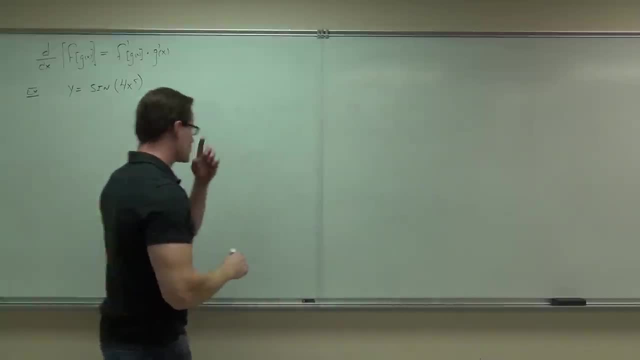 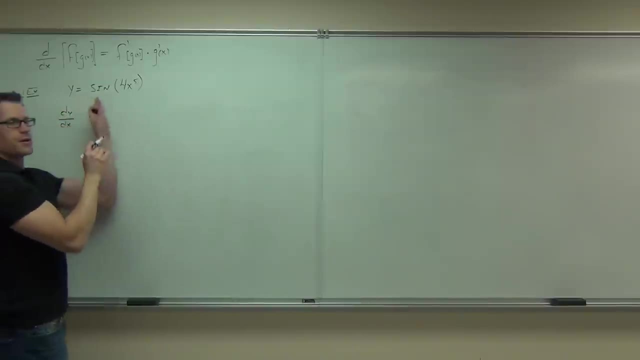 You okay with that. That's a chain rule right there. So if we use the chain rule, the chain rule says this. it says: in order to find dy dx, you're going to take the derivative of the function, yes, but you're going to at first leave the inside of it alone. 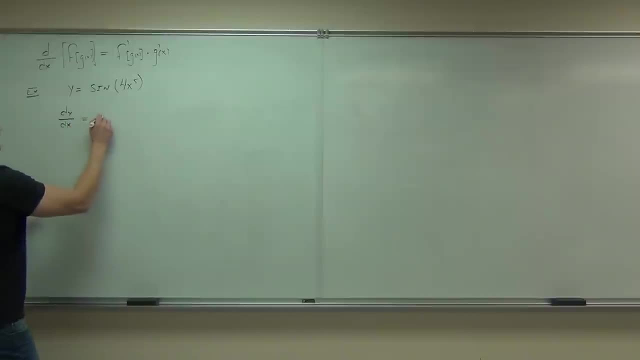 So what's the derivative? The derivative, everybody- of sine Cosine. So we do the cosine. yes. Do we take the derivative of 4x to the 5th right here? No, That's going to stay long. 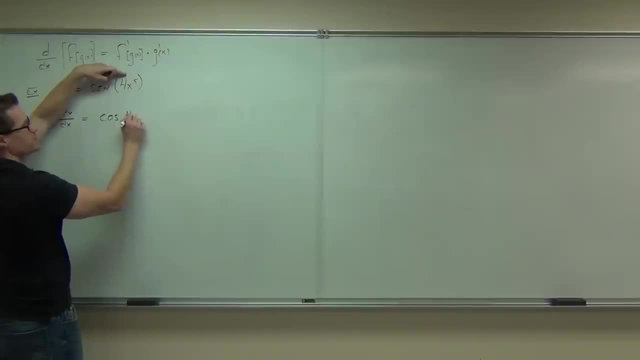 That's this part. Okay, that's the g of x. That says 4x to the 5th. This says you don't even change g of x and we didn't change g of x times. ah, the derivative of g of x. 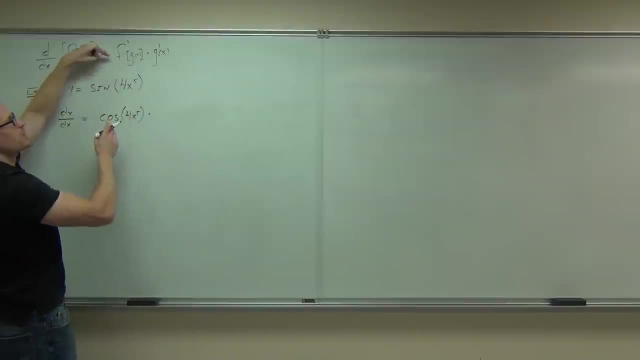 That's where you get the derivative of the inside. You don't match it all together. You don't take this derivative and the derivative and put it right here. That's not what you do. This should be: cosine of 20x to the 4th. 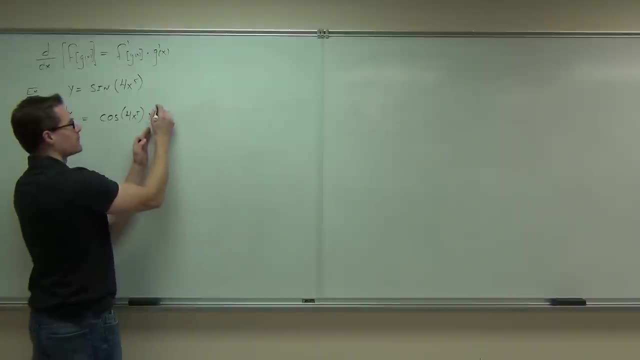 That's not it. You take this derivative later and you multiply it- and I want to see it written out 4x to the 5th, like that- And then you take the derivative. What's the derivative of 4x to the 5th? 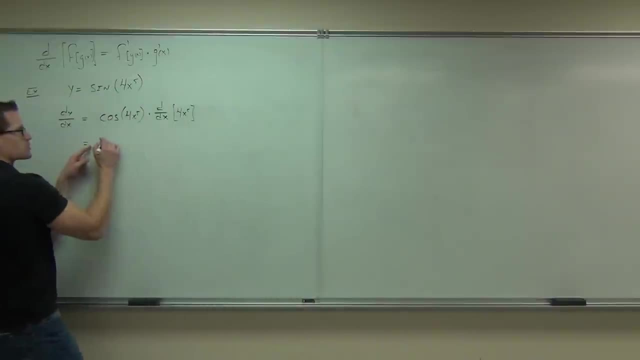 20x to the 4th. That's where we're getting that from. So we're going to have a 20x to the 4th times cosine. you don't even need that times of 4x to the 5th. 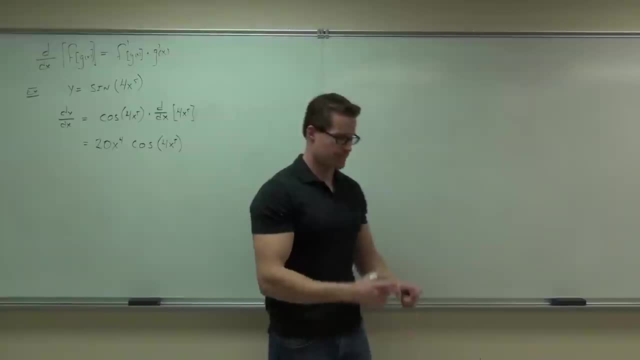 That right there. that's our derivative. That was a chain rule. So on the test, you want to see ddx? Yeah, I absolutely want to see that. Okay, The way I'm showing you things in class is the way I want to see them on your test. 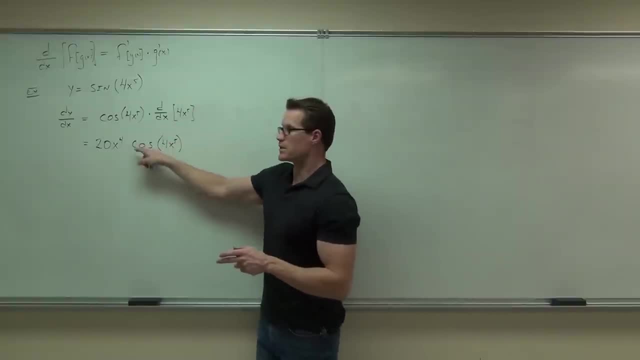 because I'm going to grade each little part. I'm going to look for this. I'm going to look for this. There's only two steps. Don't get lazy and not show me your steps. You okay with that one? Yeah, that's a pretty basic one. 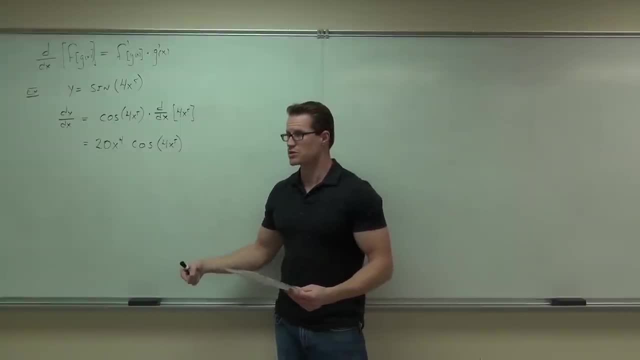 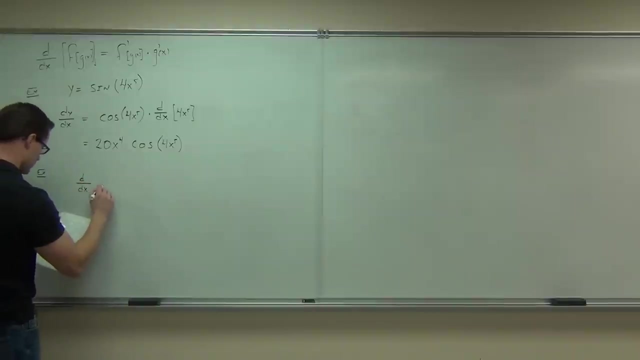 We're going to start building them up now. I'm going to start incorporating more and more rules so you can start seeing them. You ready for it? Yeah, Let's do this. You know a really good note to write down here, or at least think about. 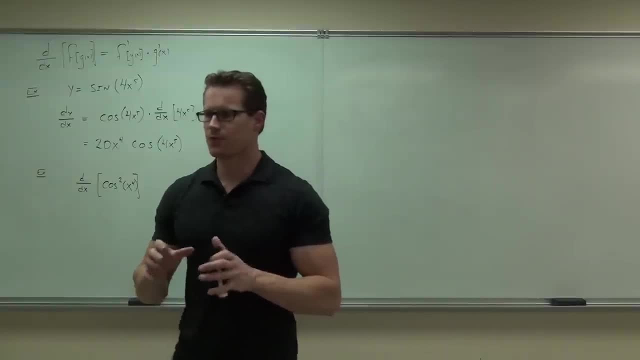 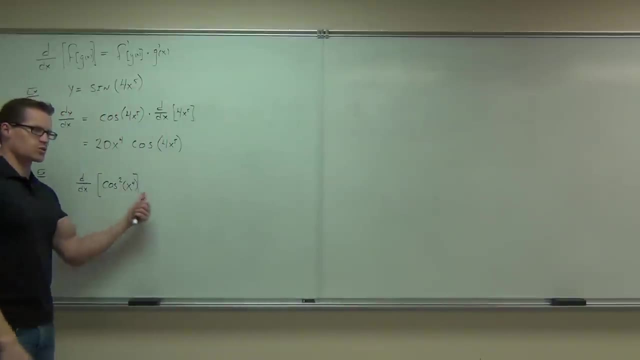 you want to think about the rules that you're going to have to do before you start your problem. Mostly, you think about the most encompassing rule here. So when you look at this problem, what does this actually mean? What does the cosine squared x to the fourth mean? 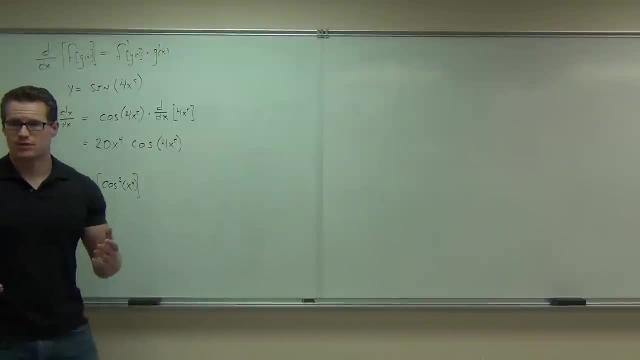 Cosine x to the fourth times. cosine x to the fourth. Write it like that. Give yourself a chance at this problem Instead of just leaving it like this. maybe you write it as cosine x to the fourth squared. Is that clear? Yeah? 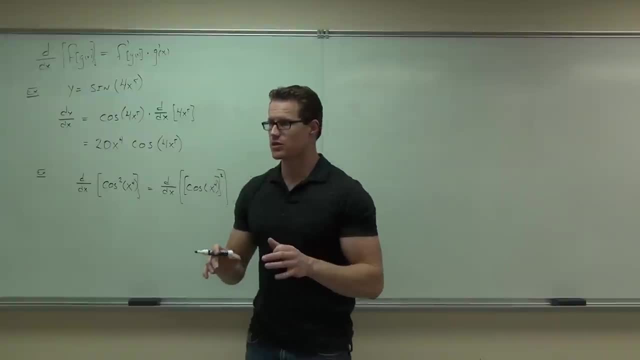 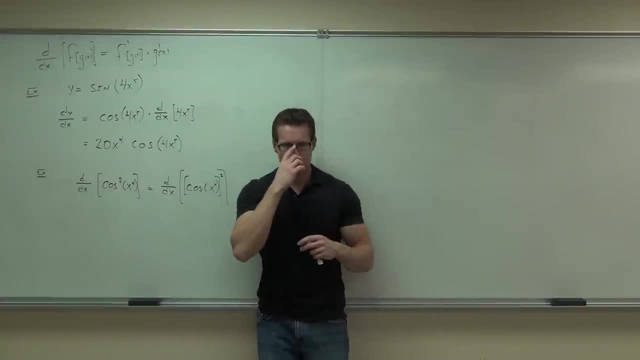 You okay with that so far? Yeah, Yeah, Let's think. Start with our rules. Which rule encompasses the whole problem? Is it a chain rule? Is it a general power rule? I see two of them. right now. What I'm going to use a specific. 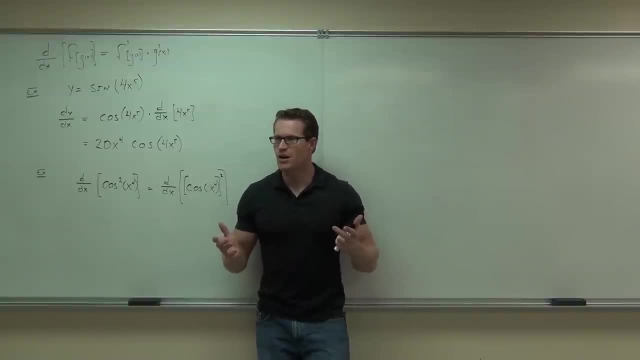 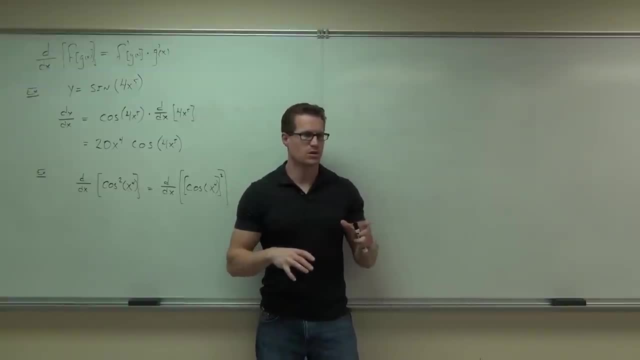 The two. And what does that two say to do? General power rule. That's the general power rule. Now, it is a chain rule, but it's a specific chain rule. It's like a correlated chain rule. It's called the general power rule. 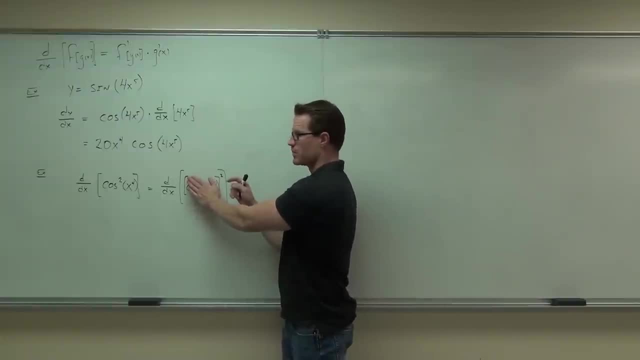 So what this says is: I have, if you can cover it up, remember that it's a chain rule. It's a specific chain rule because it has a power. It says: general power rule, General power rule, aye, aye. 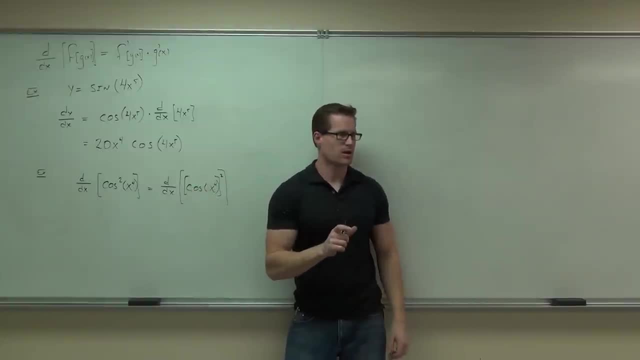 And then inside of that, you're probably gonna have a chain rule. Do you see the chain rule as well? If we start with the largest rule- I say largest because it's the one that comes with everything- You start with that, then you can follow your DDX. 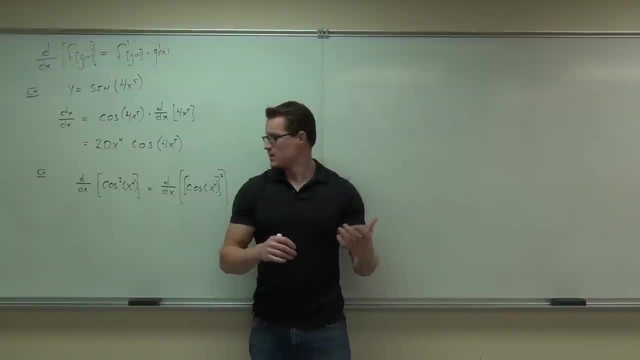 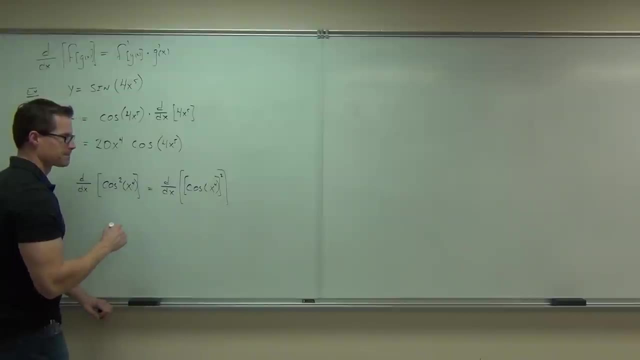 But it's all about how you start. You gotta think about that first, You with me. So let's go ahead and do our DDX. What happens to this thing? What are we gonna do? So this two goes out front, all right. 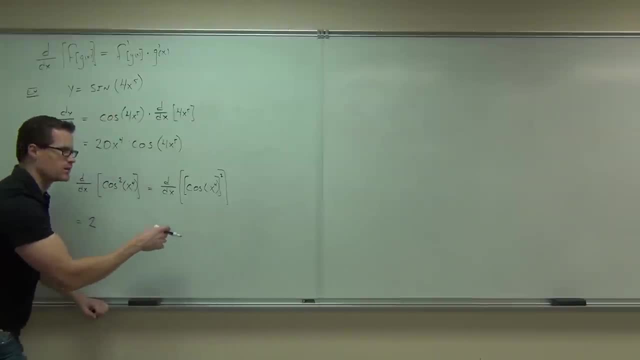 And I'm gonna have what's next. Come on tell me, Does this change for my general power rule? So I'm still gonna have a cosine X to the fourth. To what power One? So do I need a bracket with a little one? 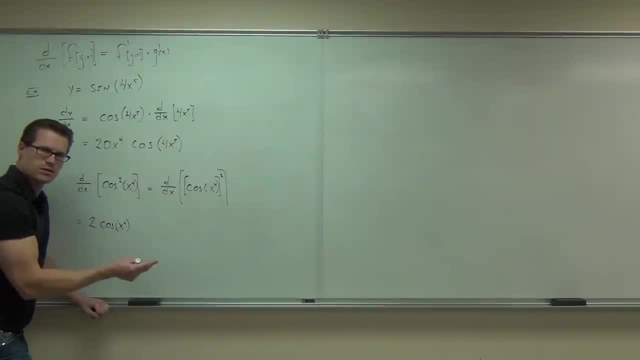 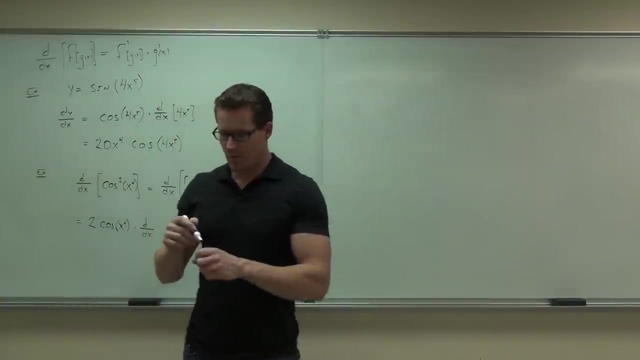 Is this okay on how to get there, And then I'm done. No, No, what The derivative of x to the fourth? Just x to the fourth? What's the derivative that should come next? Remember when you do a general power rule: 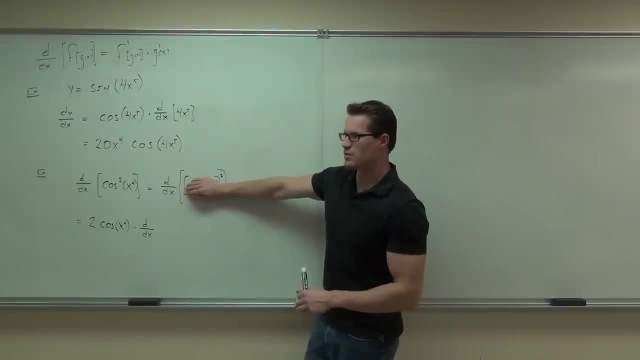 you cover that whole thing up, right You go. okay, take the derivative of what's under my hand. It says: you move the two down, you subtract one from it. That's great, and you don't change what's under my hand. 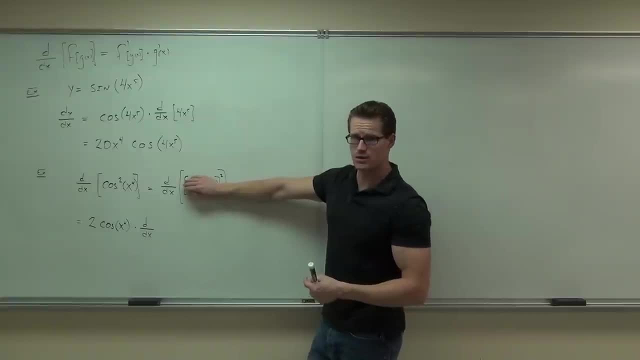 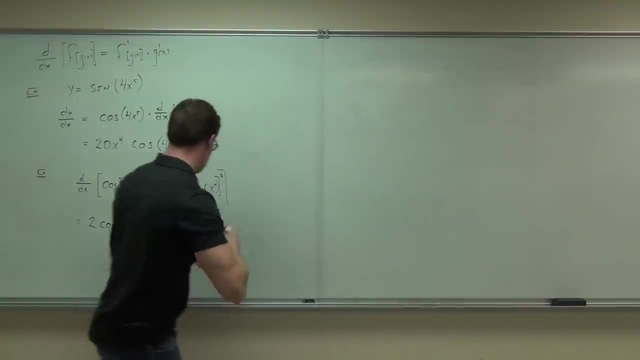 That's this part, But then you have to take the derivative of everything that's under my hand. Do you get me? So it's not just x to the fourth. it's what Cosine The whole thing. Oh, this is gonna be brutal. 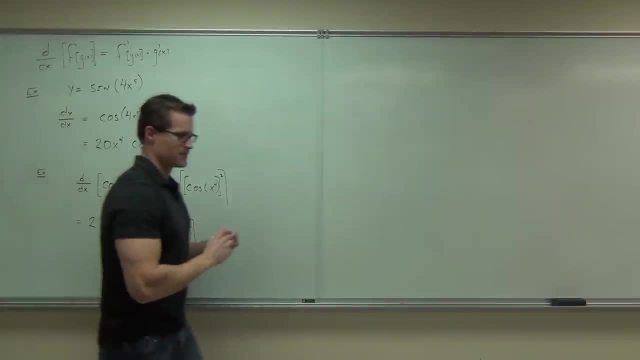 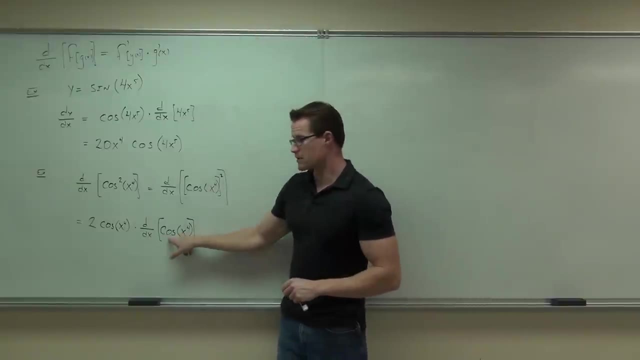 No, no, no, not brutal Fun Tonight, Yes, tonight, Richard, do you have to be okay with this? Richard, do you have to be okay with that? so far, You see where you see y you have a cosine there. 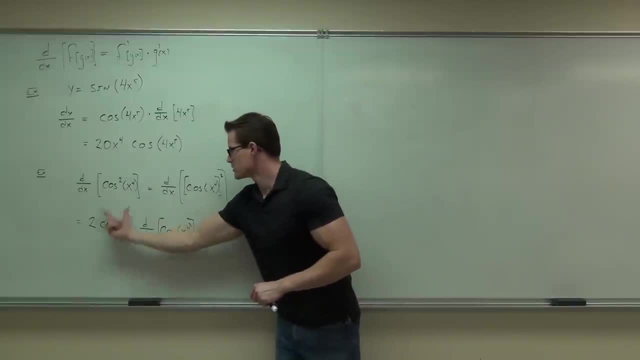 Do you see why you have a cosine there, This one. you do not change This one. you take the derivative of the entire inside function. That's how the general power rule, aka the chain rule, works. Derivative of the function times: the derivative. 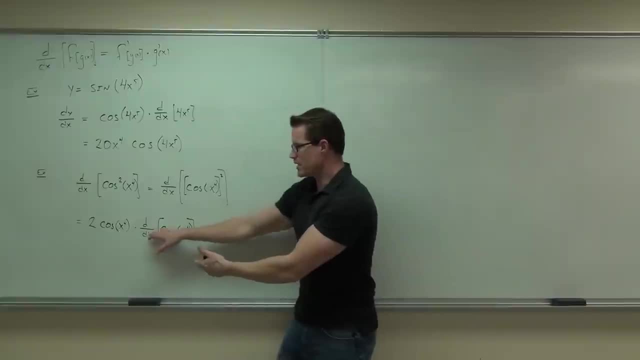 of the inside. But now you're done with the calculus up to this point. Now you follow your DDX and this has broken down your problem, made it a little bit easier. Can you take the derivative of cosine x to the fourth? 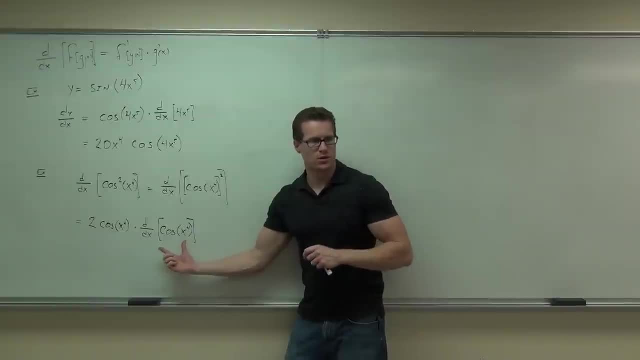 What rule is that Chain rule? That's the chain rule. The chain rule says: you take the derivative of your function times, the derivative of your inside- That's what it says- to do: The derivative of your function times, the derivative of your inside. 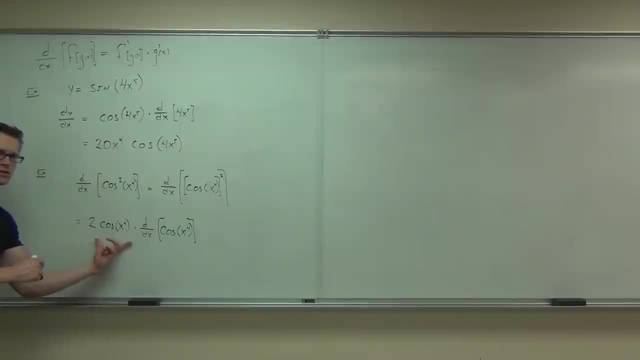 So you tell me, does any of this change Times? We'll take the derivative of cosine x to the fourth. What's the derivative of cosine x to the fourth? Let's think about that. It says you take the derivative of. it says derivative of your overlying function. 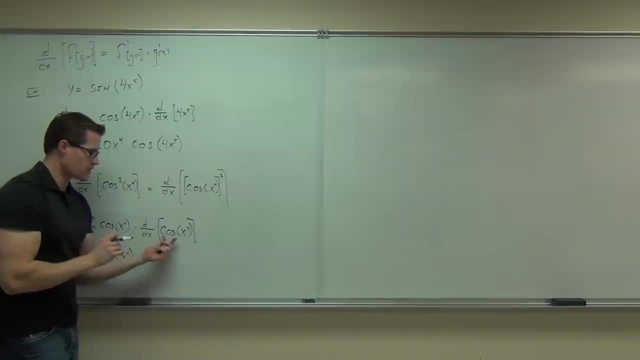 Okay, that's the thing that you're composing into. So, derivative of cosine. you need to take that first. What's the derivative of cosine? Negative sine, Negative sine. Okay, so I'm gonna put that in a bracket because it's negative. 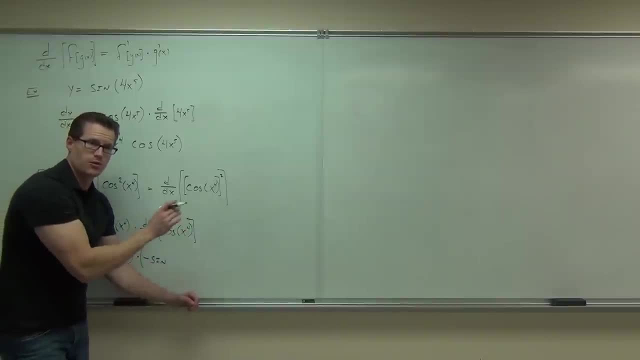 Negative sine. hey, negative sine of what Is it still? x to the fourth or four, x cubed. X to the fourth? Good, because chain rule says you do this, but you'll leave this piece alone for two. You leave that alone for just a second. 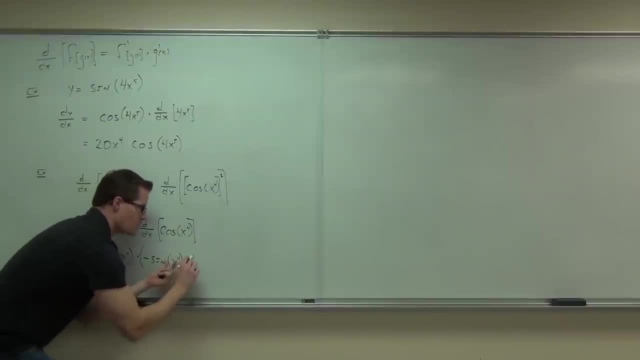 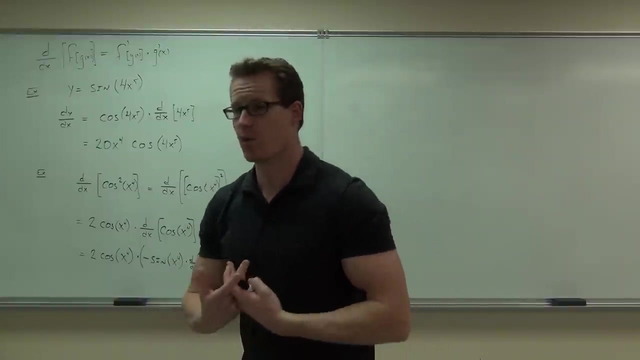 You leave that alone. In order to find the derivative of this, you multiply it by that. So we're starting to build these rules on top of each other, and you really gotta be good at what rule comes first. If you are, then you follow the DDX and it's just fine. 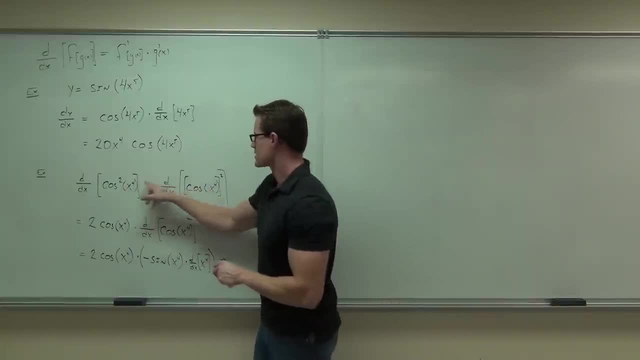 But you gotta find that first rule. Once you do that, we said, okay, this probably should be written like this: This is general power rule. You bring it down, you leave it alone, you multiply it by the derivative of the inside. 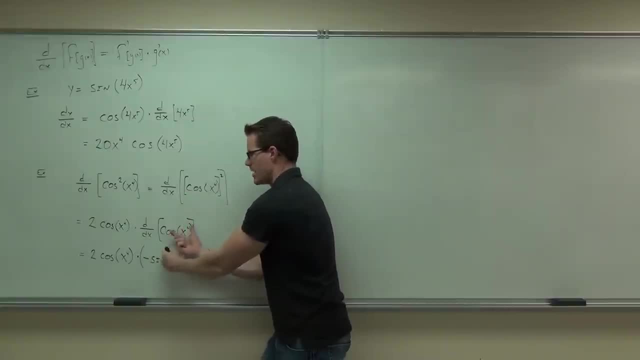 That's where we're getting that from You. okay with that. After that calculus is done, Just keep on writing. keep on writing. This. DDX says: take the derivative of this thing. Now, this is a chain rule. Chain rule says: I take the derivative of cosine, got it. 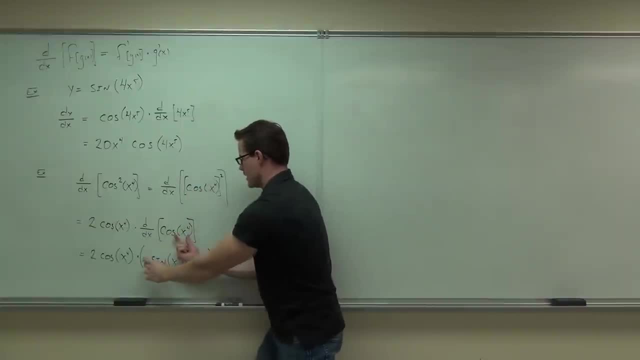 But I leave the inside alone, just like you left the inside alone here. I leave the inside alone And then I multiply by the derivative of the inside. That's where that's coming from, Rich. how do you feel about that so far? 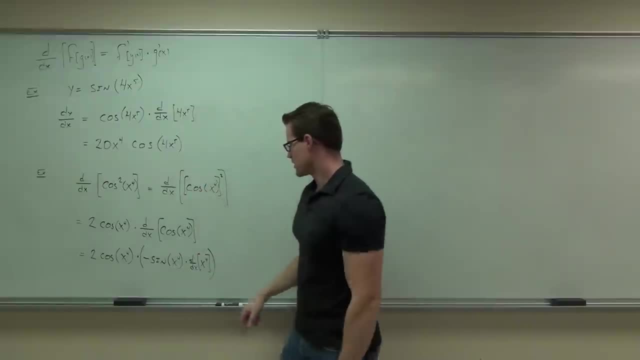 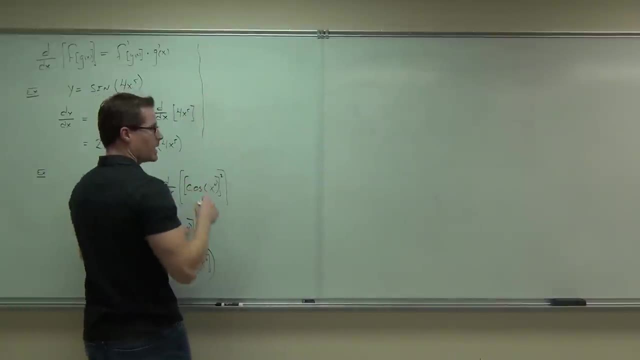 Good, all right, We're almost done. We only have one little teeny derivative to take. What is it? Yeah, you know what. Every time you do a set. it makes it easier Sometimes, But every time you use a rule. 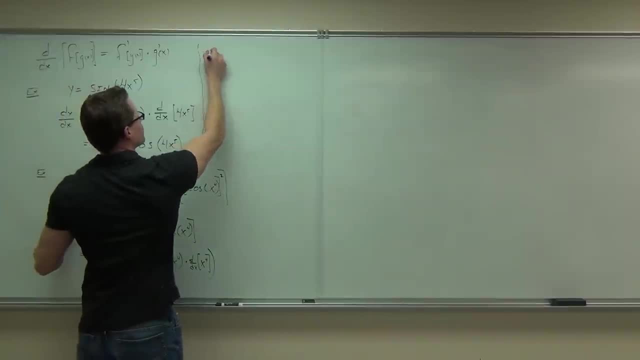 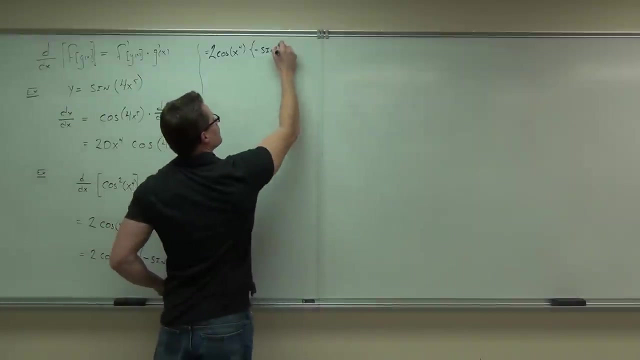 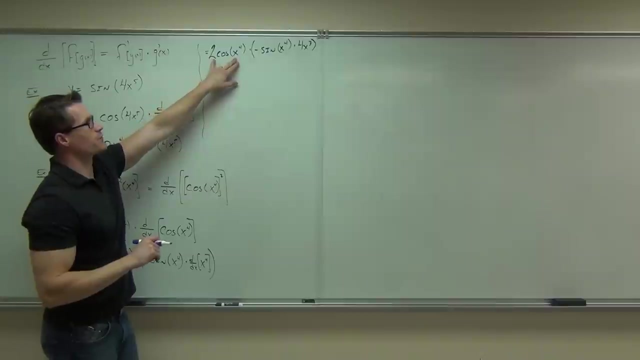 it breaks down into little pieces for you. There you go, Times. what is that? Four, I don't know Cool. Negative, oh I'm sorry. two. cosine X to the fourth times negative. sine X to the fourth times four. X cubed. 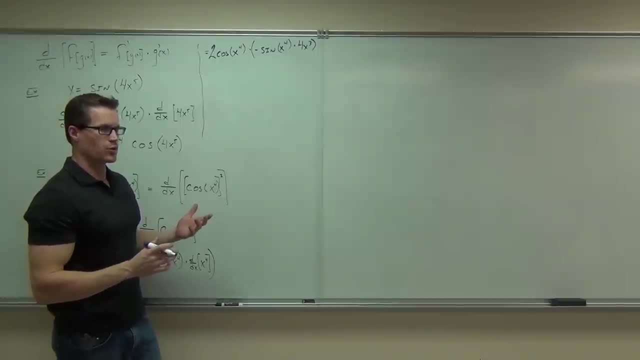 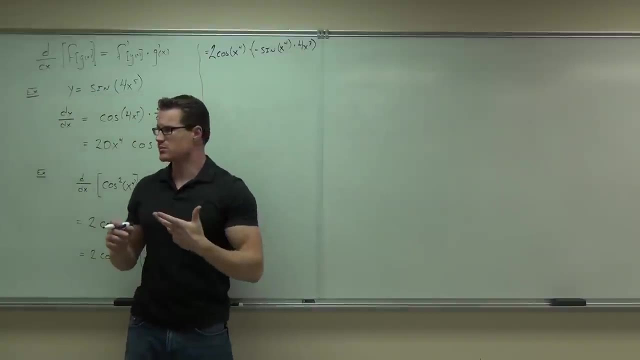 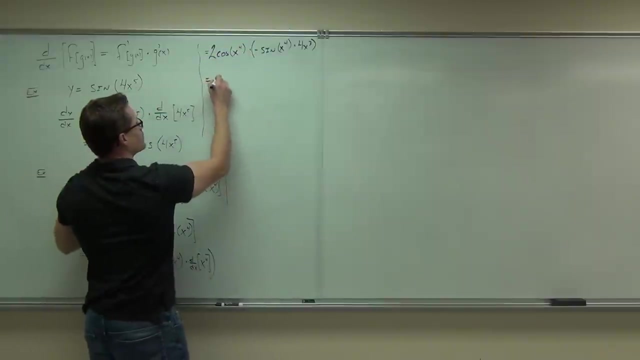 Just to make it maybe a little prettier up here. prettier would mean you have a negative, you've got a 4x cubed and you have a 2. they're all being multiplied together. you see the multiplication. take that stuff together, so this will be 8 negative negative, 8 X to the third. then 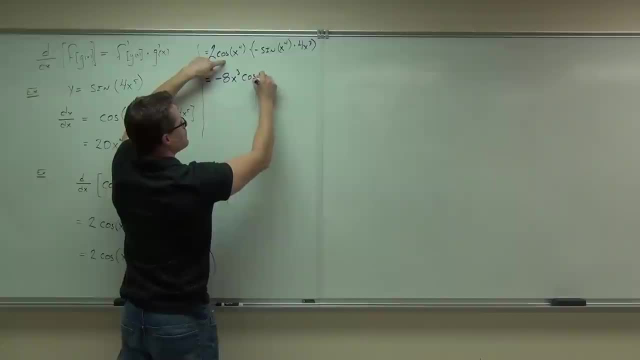 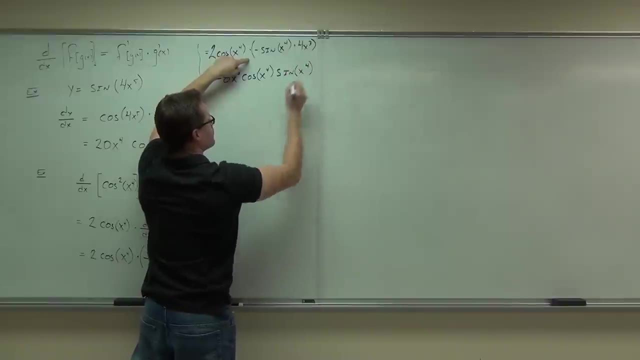 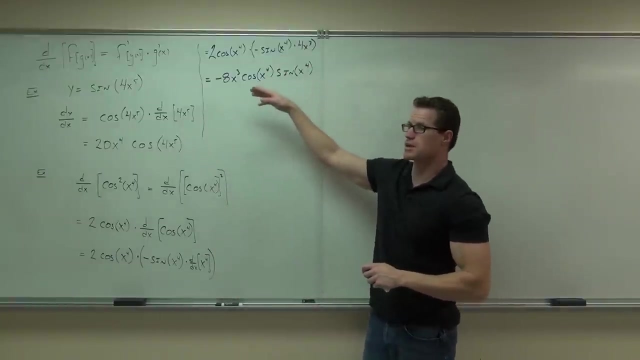 the cosine or the sine, and then the sine, and that's how I'd like to see your problem after this. it's just algebra, it's just putting a couple things together. you have 2 times negative, 1 times 4. that's your coefficient, that's negative 8, the X to the third, we 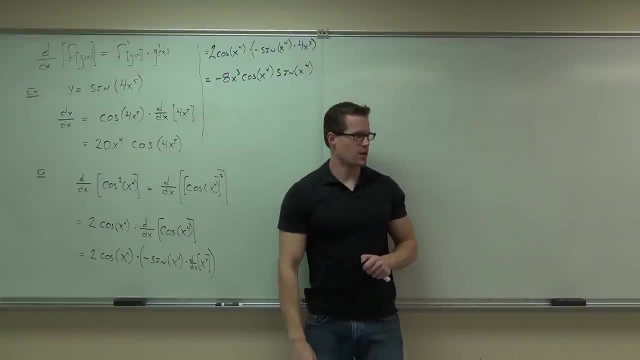 typically like to bring that up front. can you follow that? yes, no. if yes, great. if not, do you have a question about it? yes, we're here, are we good? my middle guys, people at home, just kidding, can't see you. you guys, on what? what? if I could see? 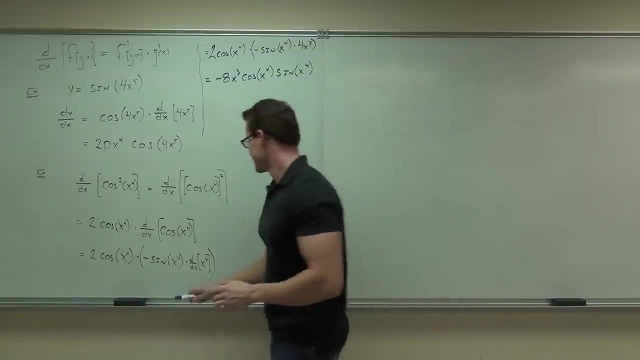 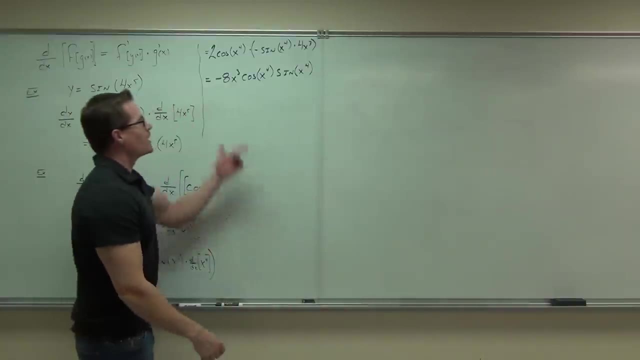 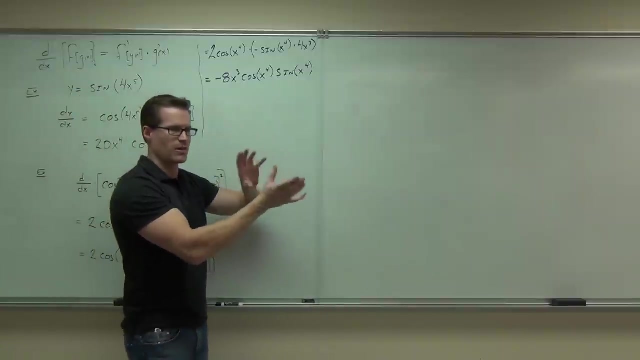 you. they figure out when it doesn't matter which order the sign, because I know that doesn't matter. this is technically right, right, this is it. so no matter of how you, because in multiplications, commutative, associative, doesn't matter how you group, of how you put in order, we typically just write. 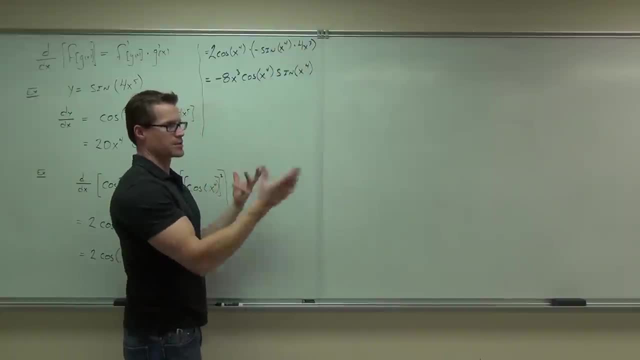 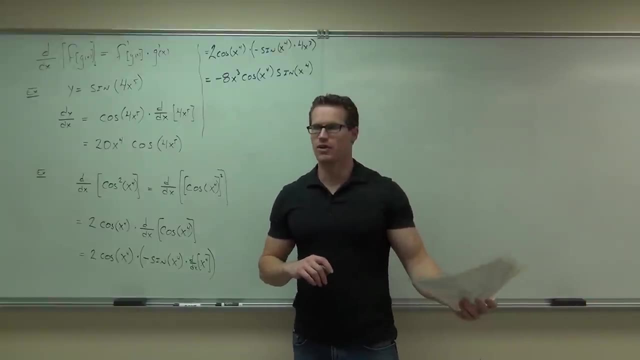 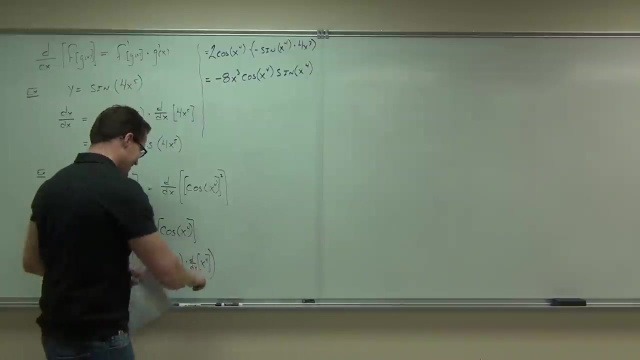 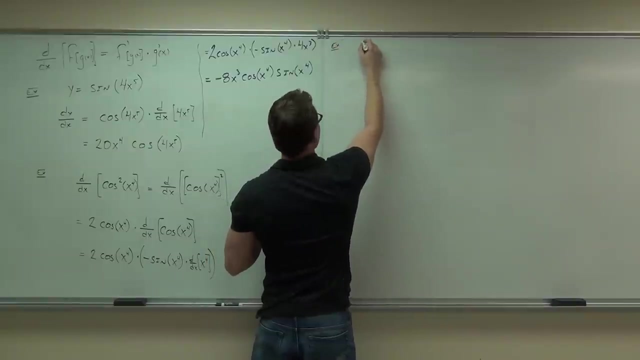 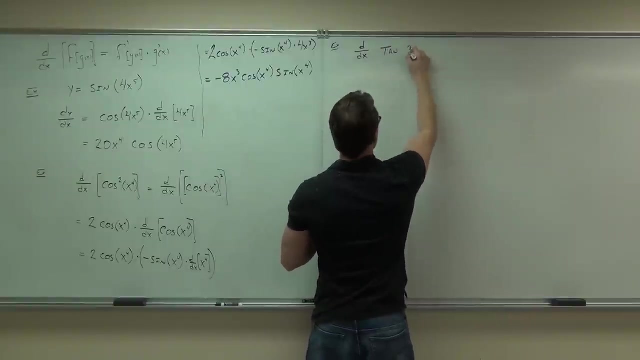 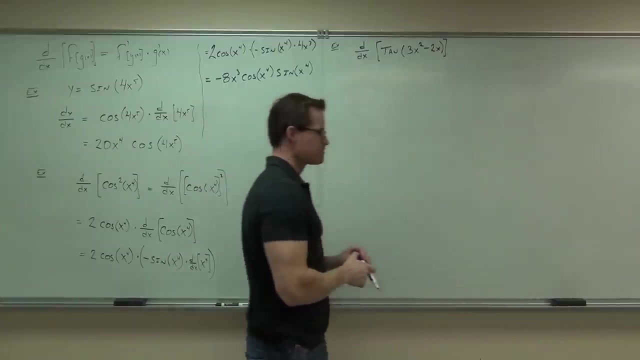 numbers and single variables first and then signs and cosines. that's just how we do it. can we move on? are you ready to move on to one similar? is there a choice? I guess you just leave, you're gonna stay. no, no choice, you guys, okay, okay. 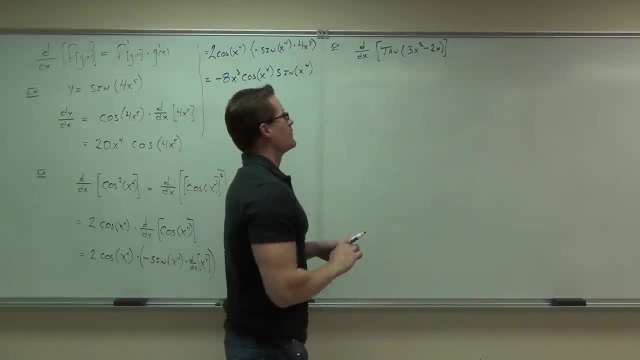 problem If I had done this. would it be a friendly problem? No, it would be your enemy. If I did that, what would you do? first, A chain rule- they're both chain rules, but a chain rule or a general power rule, General power rule- That would be just very similar. 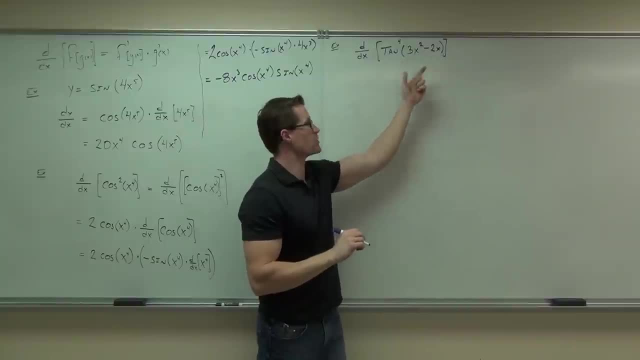 to that problem, You would have to bring down the four, all of this to the third power, derivative of the entire inside thing. Do you see it? Without the power? without the power, what are we talking about here? Chain rule, That's the chain rule, If you can cover something. 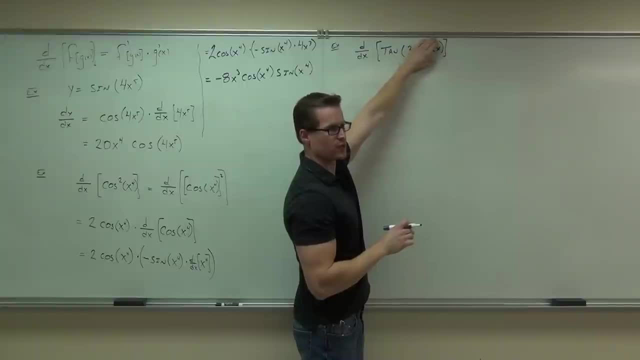 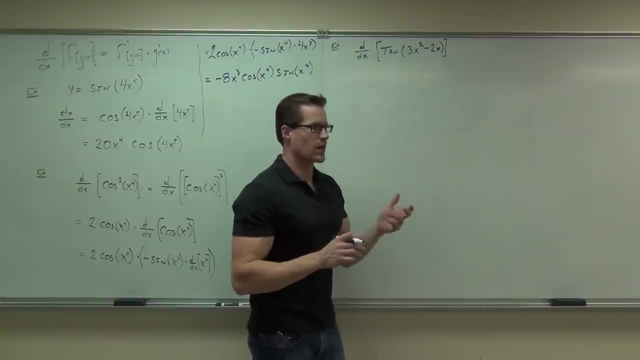 up and you still have a function that's typically a chain rule. so we still have a chain rule right here. It's not a product rule. that's not a product. it's tangent of something. that's a chain rule, it's a composition. Well, let's do that. How does a chain rule work? 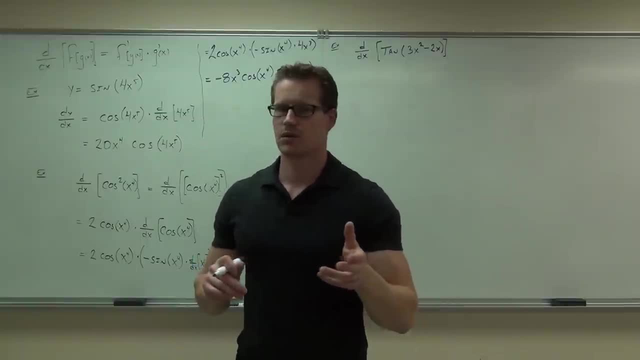 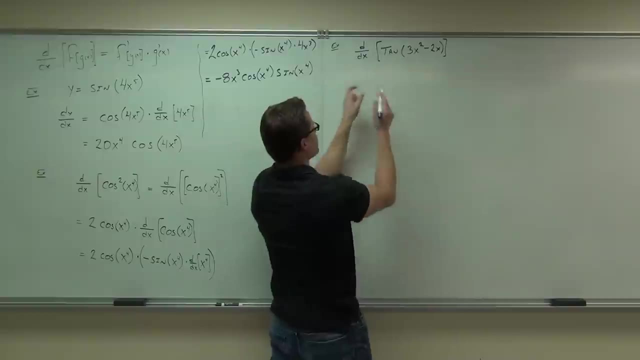 What should we do first? please Wait. do what now? Okay, cool, so leave this alone, take the derivative of that thing. So this says I'm going to have: oh, tangent of that thing is tan what's tan. Very good, Make some flashcards. know those derivatives Secant. 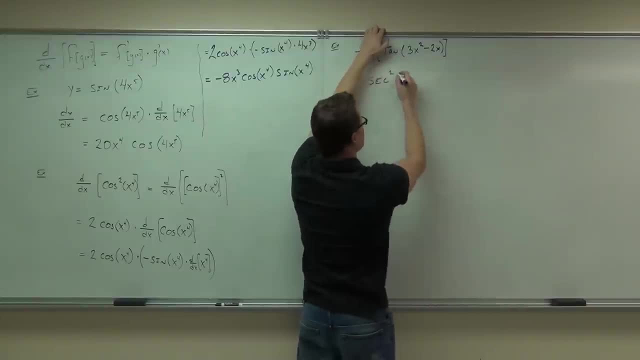 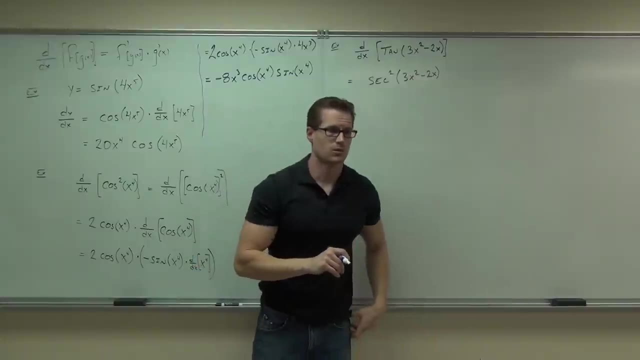 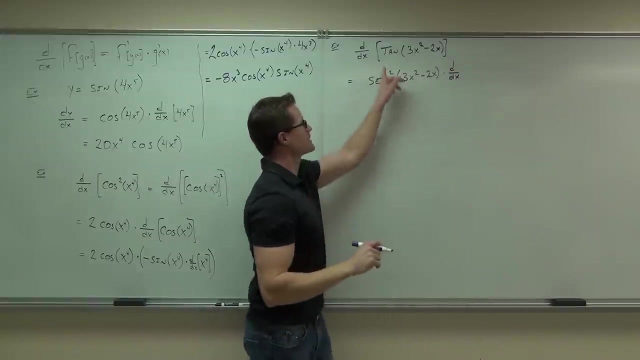 squared. does the inside change for us right now? Okay then No, no. Can you tell me what the inside is here? Is it tan of this or just this, Just that part? This is just a chain rule. It says: derivative of tan the secant squared, leave the inside. 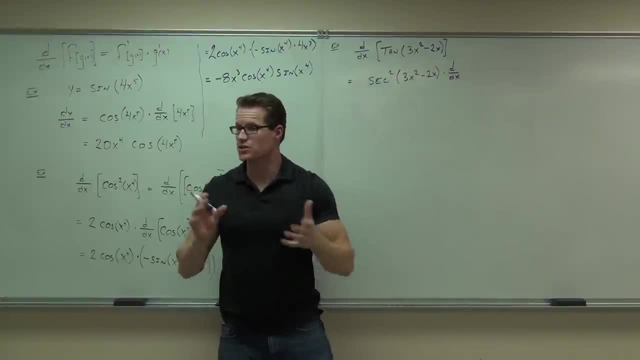 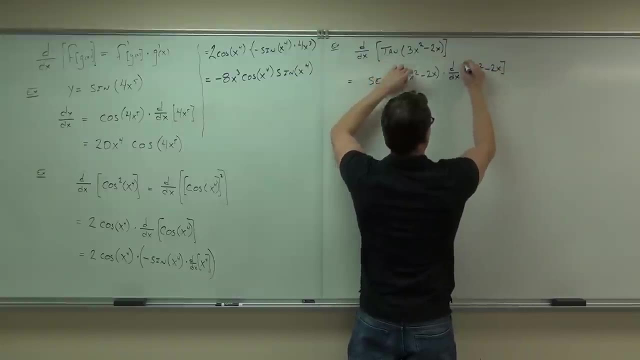 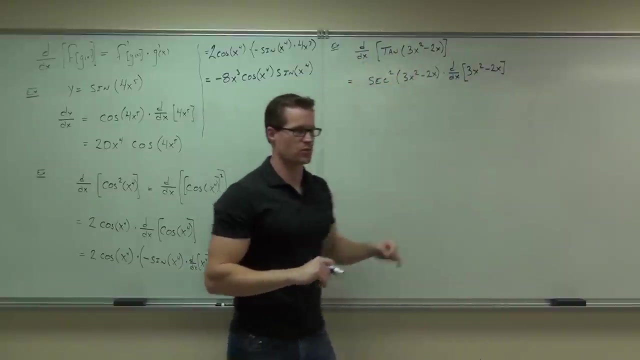 alone. then multiply by the derivative of the inside. That's what the chain rule says to do. in English: Got it Secant, squared, cool. Inside doesn't change derivative of the inside. That's the chain rule at work, Not too bad. what are we going to do? Just, 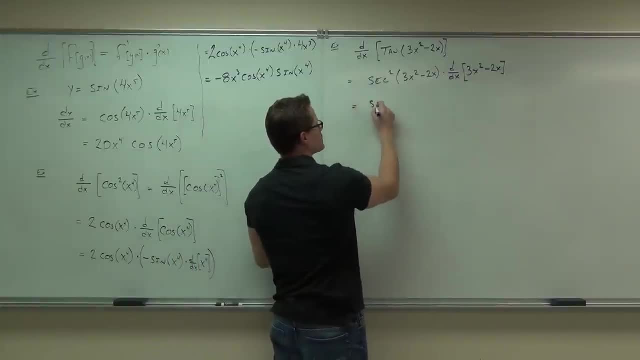 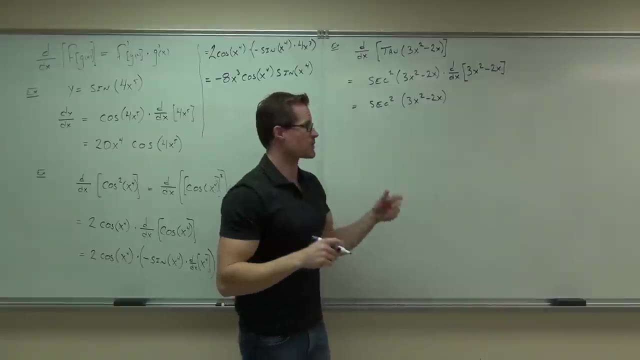 follow the DDX. This is basically done. You're going to get a secant squared, but what people often forget to do is this piece of it. They really often forget to do the chain rule. They'll do this for me, but they'll. 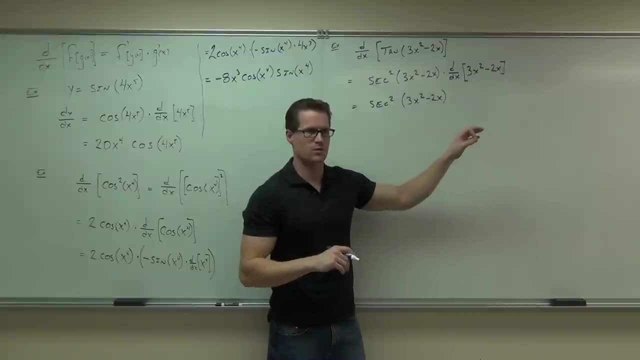 forget this part. I can't have you forget that part. That's a big part, That's a really big part. Or they will do secant squared and then they'll take the derivative and just mash it together. So if you're giving me this, well that's, that's the derivative of tan. 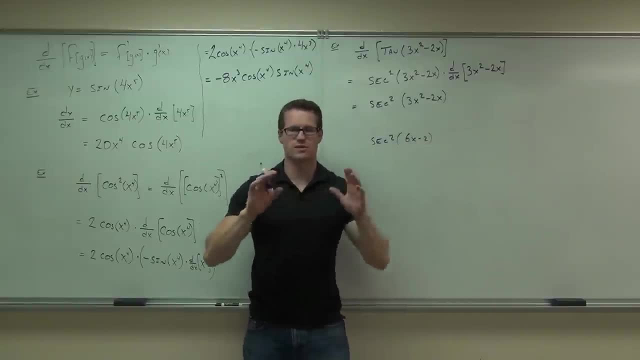 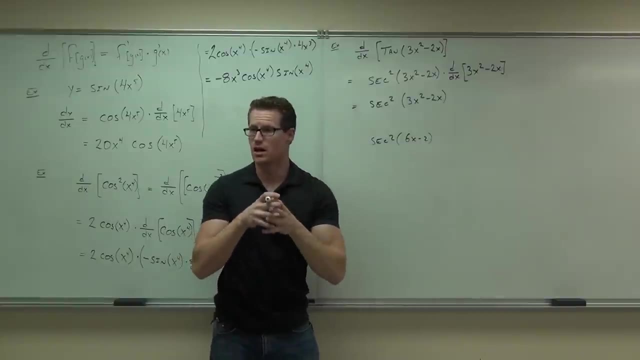 Well, that's. that's not even nearly right. You've changed the angle, you've messed that problem up right. That's not what we're talking about. You can't just take derivative of this and derivative of that. This is definitely a chain rule because it is a composition. 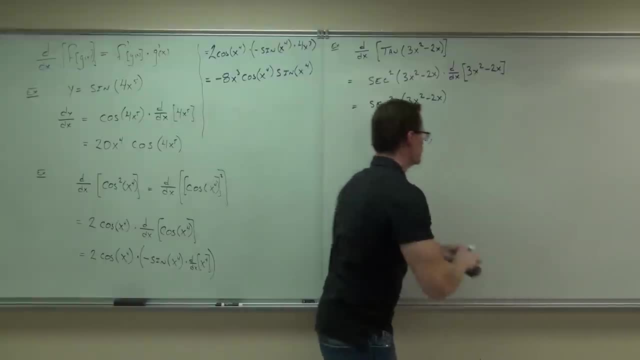 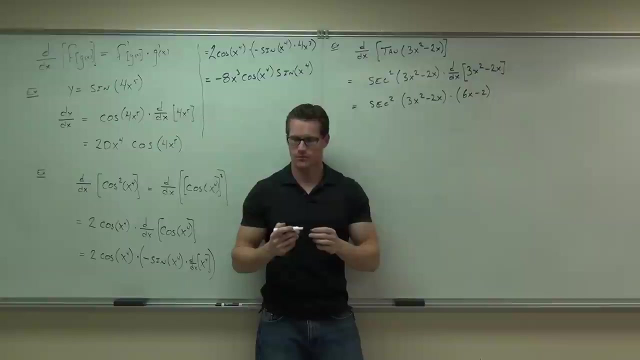 See the difference there. So for us, we've got a no, no, no, no, Not that. This is what is it. Oh yeah, I just wrote it. Another question: can I distribute that? Why can't you? Why can't you? What is that? That's an angle. It's actually an angle. that's. 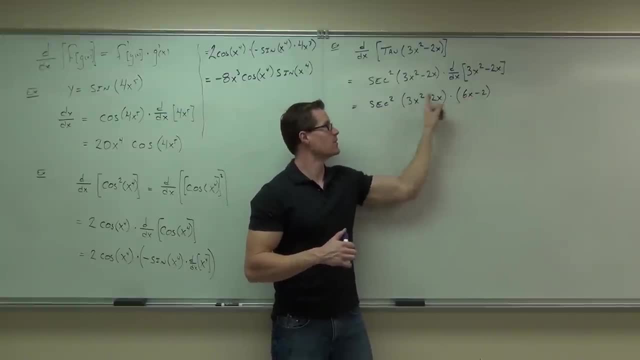 related to this. I mean this: No, these two. Can you distribute these two Negatory This? that's not an angle. This is attached to that secant squared. That's part of it. You can't change the angle. You can't change the angle. What we can do is move this to the front. so 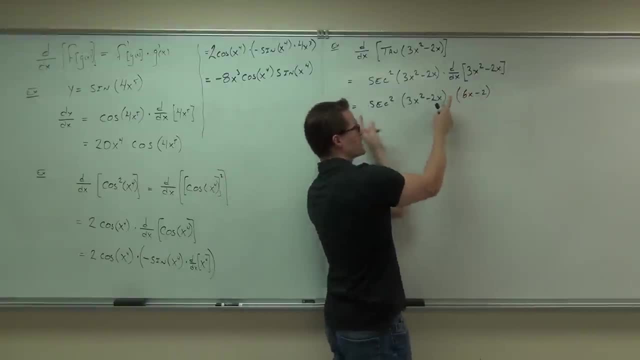 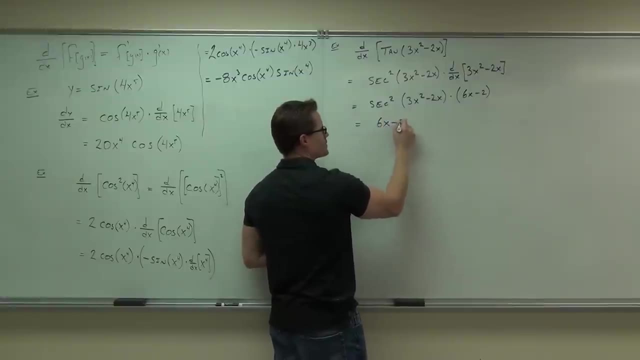 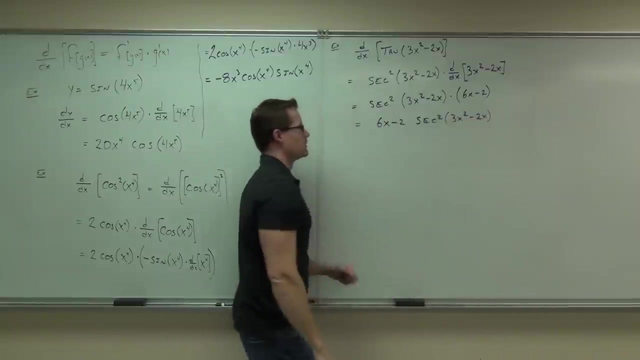 you can see it. You probably wouldn't want to take this thing in and take the whole thing. You wouldn't want to do that, It's already factored for you. nicely, Don't do that. Just leave it as 6x minus 2, secant squared. 3x squared minus 2x. Tell me one huge thing. I'm going. 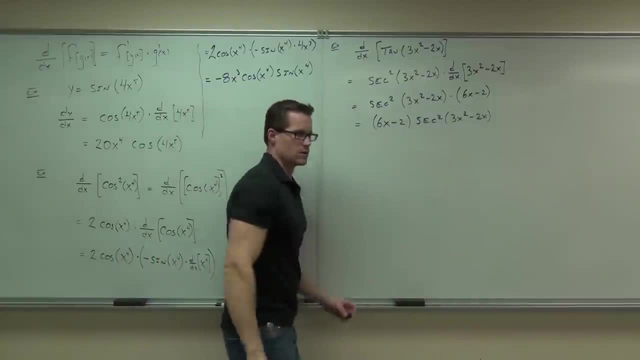 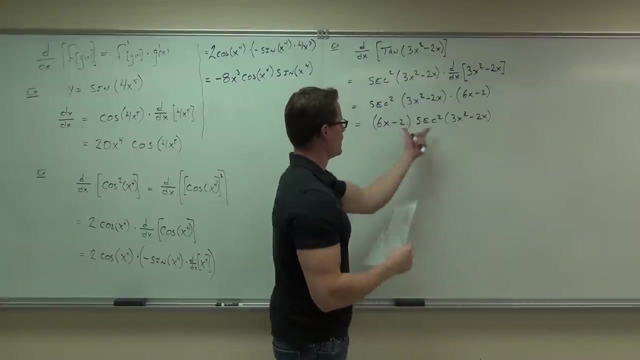 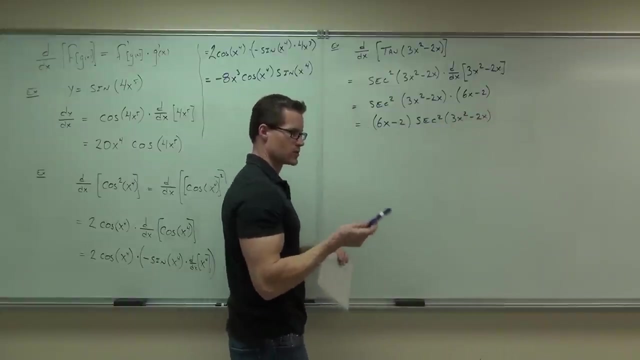 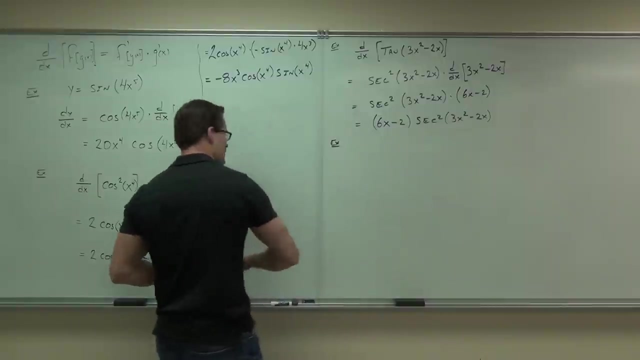 to mark you off on For sure. Yeah, for sure. Still okay, Yes, All right, Ready to keep going. Yeah, like that, Like that. Yeah, You could. It would be irrelevant, but you could. Okay, See, now we're having fun. 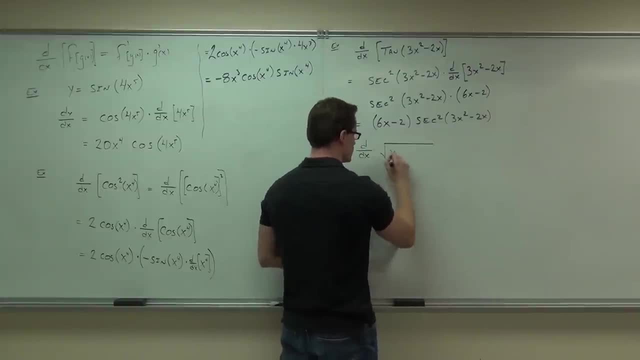 No, no, no, no. You know what I'll be. no, I'm not going to be nice There. Great way to say thank you. I was just going to give you an x, but I want you to see what happens. 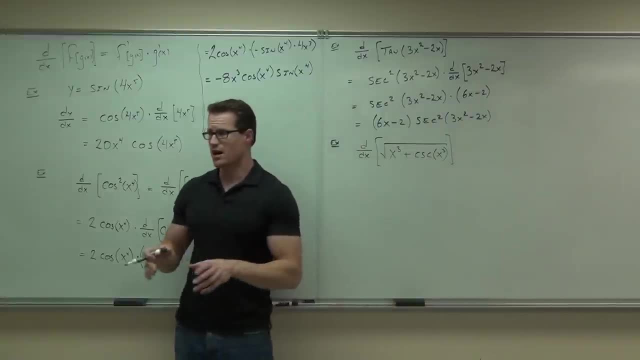 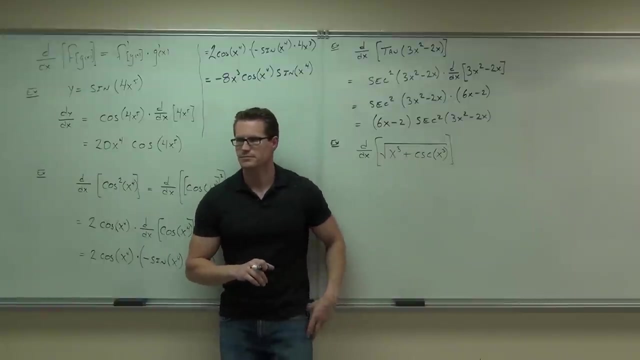 So this will be a little bit more difficult. Trust me, you want the more difficult ones now. That way, your homework seems easier. If I just give you all the easy ones now, your homework should seem much easier. Okay, I'm lost. What do I do? Why would you say a general power rule? Okay, So chain. 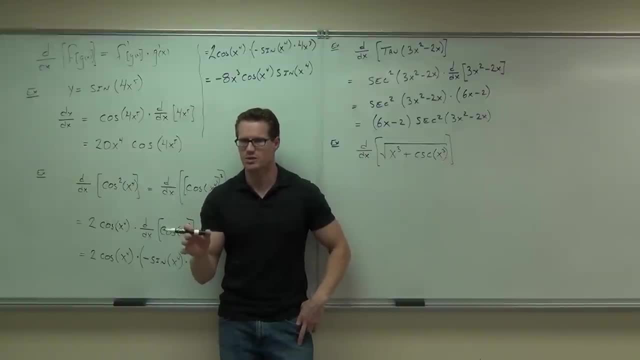 rule, general power rule- same thing, but we're going to say general power rule when we have the exponent, so we can classify this a little bit better in our heads. okay, So if I say chain rule right now, me, I'm looking here, I'm looking there, So this I'm going. 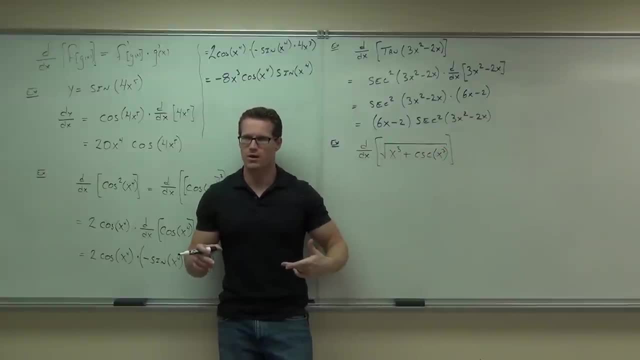 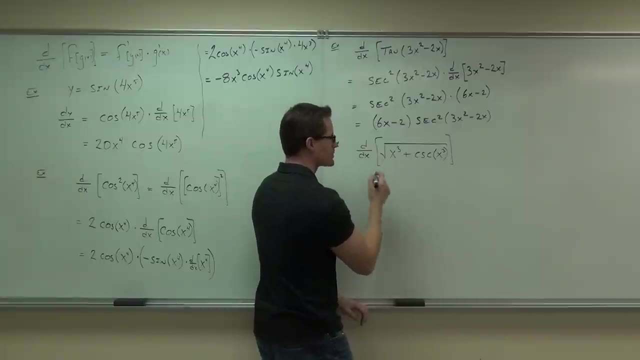 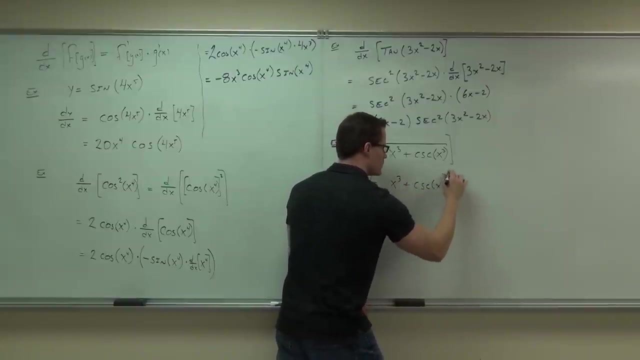 to call that a general power rule. I'm going to call that a general power rule for this class. Okay, okay. Do you see the general power rule at work? See how it covers the whole entire expression? So perhaps write it this way, because we know, in order to take these derivatives, we've got to have exponents. 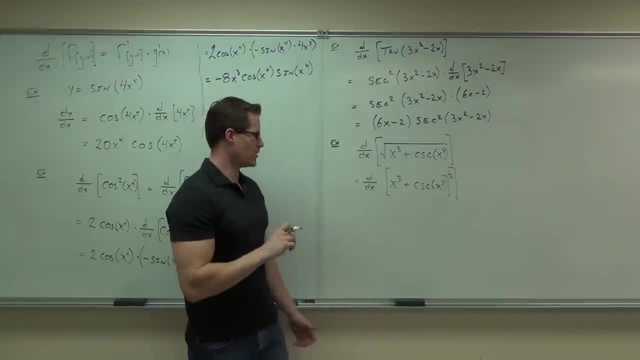 So far, so good. Am I? Oh, I am Shoot Better, Much more better. Okay, tell me what to do. Come on, you guys should be rolling with this stuff at this point. This should be like: okay, we're. 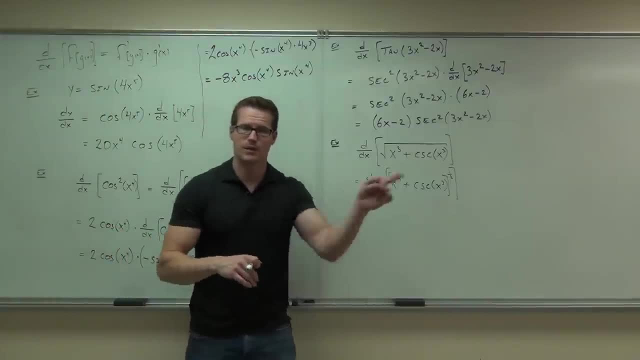 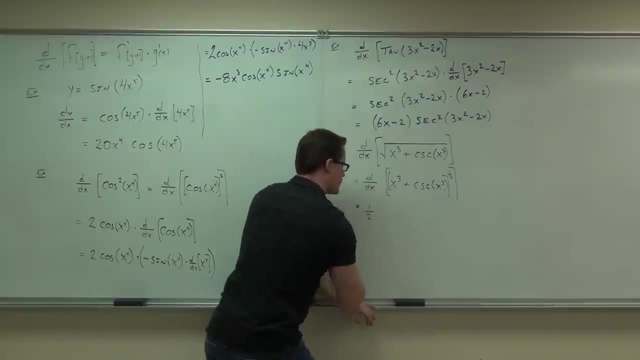 getting there. Not perfect, but we're getting there. What do we do? Move that one out in front. Good, Because this is general power rule, right? General power rule says: bring it down, write whatever's on the inside. Okay. 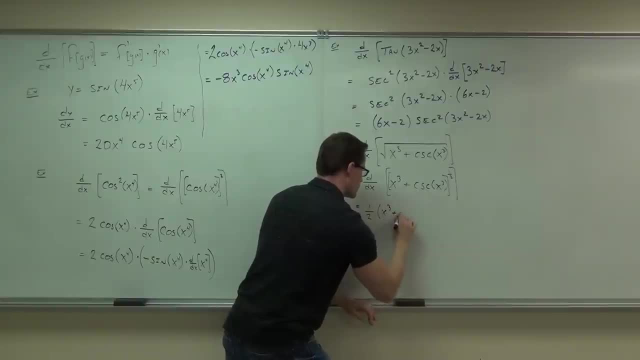 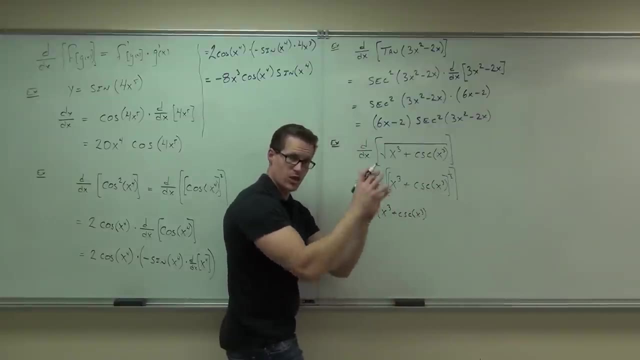 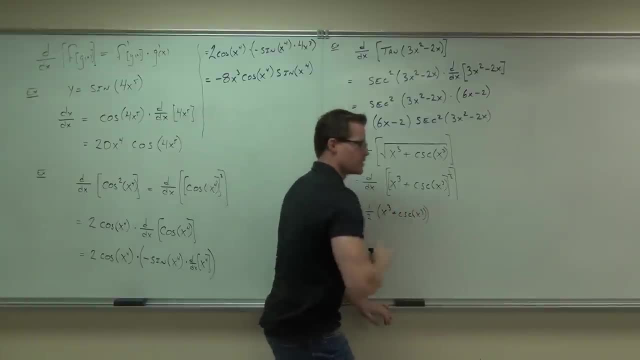 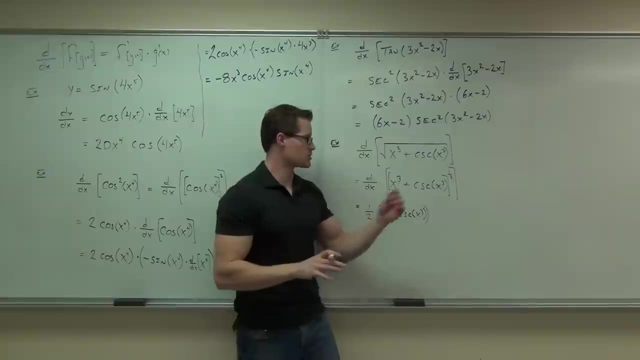 also includes a general power rule. Do I still have an exponent? Negative one half, Negative one half? Or do I just get rid of that exponent? Do I still have an exponent here? Yes, Yes, Don't forget about that exponent, man. Oh my gosh, if you just move down to one half. 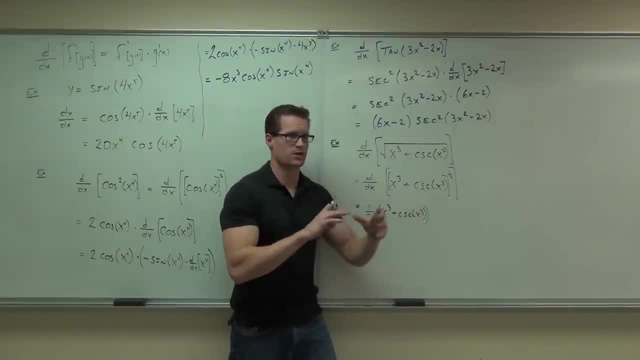 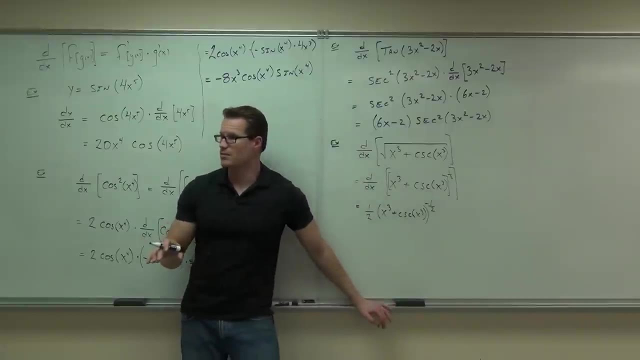 and forget that that's a big deal because you've eliminated a square root on the denominator there. So this really needs that negative one half. Do you see where the negative one, where one half, is coming from? Conduction of your duty. you feel okay with it. 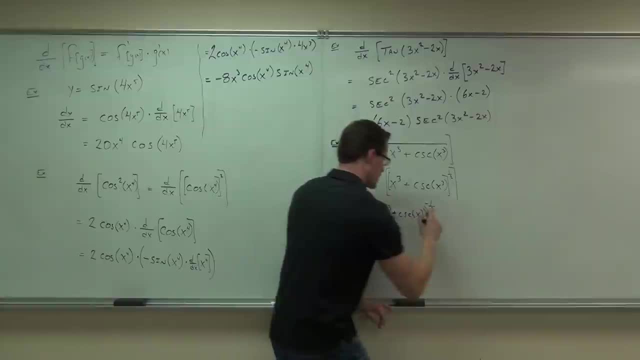 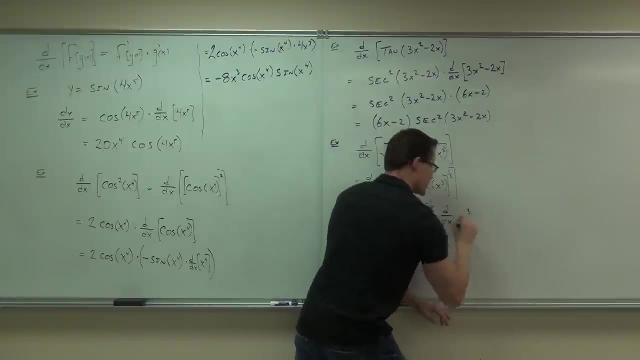 Now what do I do? Multiply by the derivative of the inside. Okay, times derivative, derivative, derivative. Take the derivative of the inside. Yeah, take the derivative of the inside, Take the derivative inside. So the general power rule says: bring it down. 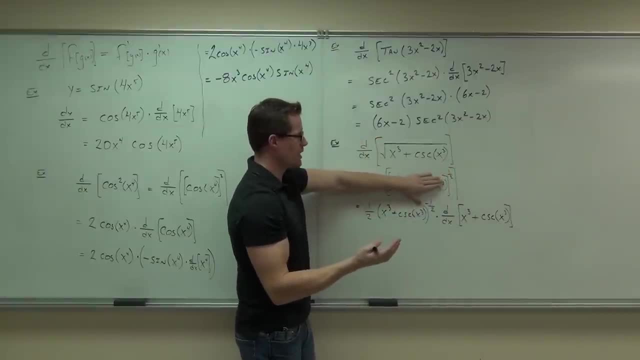 subtract one, just like you normally would with any power rule. only now you have to multiply by the derivative of whatever you covered up, whatever you ignored for a second. In this case, it's the entire expression. So notice how, before you start taking all these derivatives, 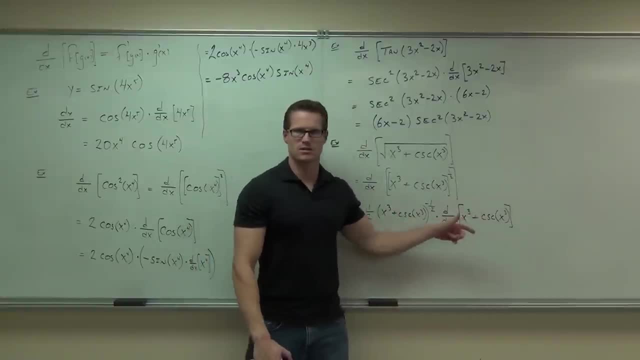 you have the same thing twice. you see that Same thing twice, and then you- I'm losing some of you, You with me. Then you take the derivative of that little piece, This calculus done. Just hang onto it for a while. 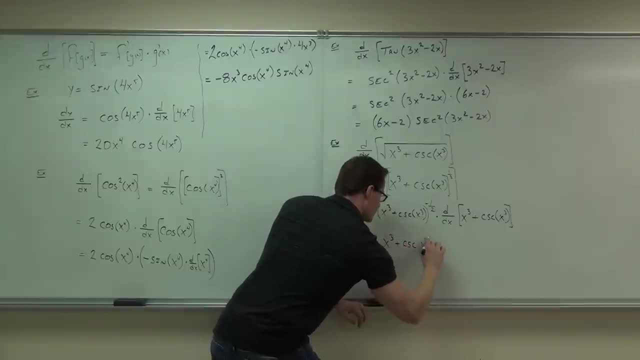 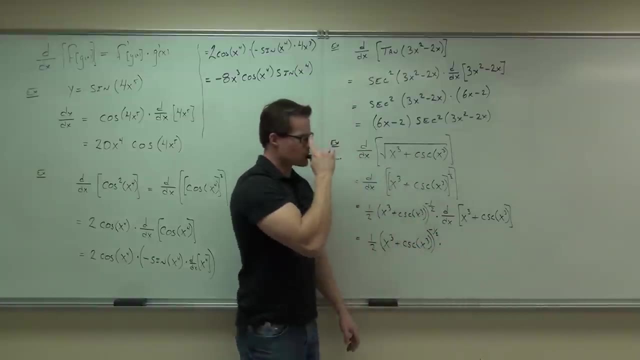 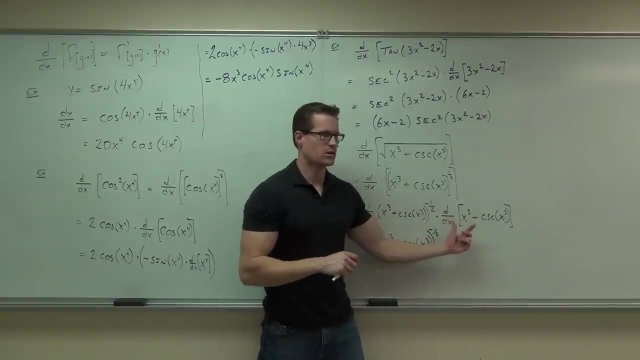 Now let's look at the derivative of this nasty junk here. What is the derivative of this thing? Can you take a derivative piece by piece? Is it okay when I'm adding and subtracting? Do I need a special rule to take the derivative of x cubed? 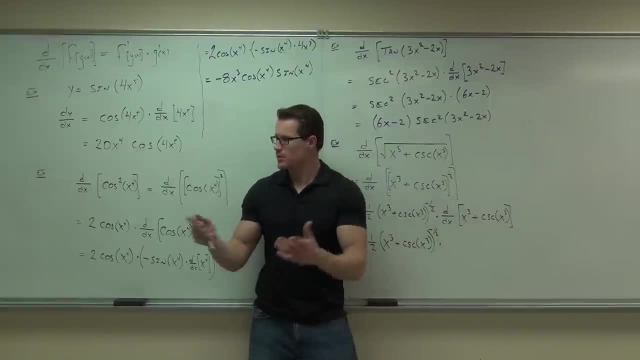 Not at all. I can just do what's the derivative of x, cubed Three Beautiful. Not a problem, It's. the only time you need special rules is when you have a quotient, a product or a chain rule. That's it. 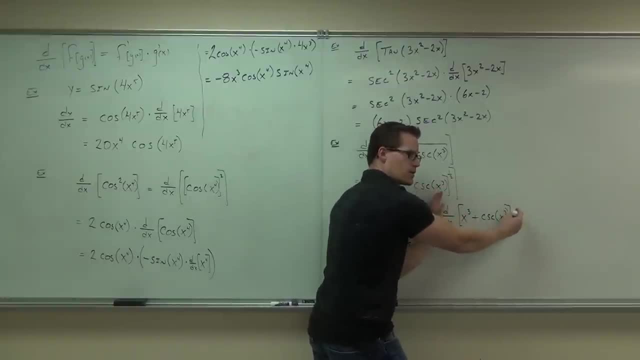 So when you get this little piece, this should be a problem within a problem. Now you look at this and you go: how do I take the derivative of x cubed? No problem, It's being added. Remember, derivatives are separable. 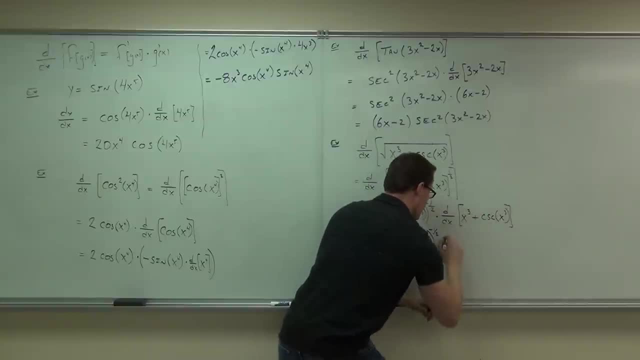 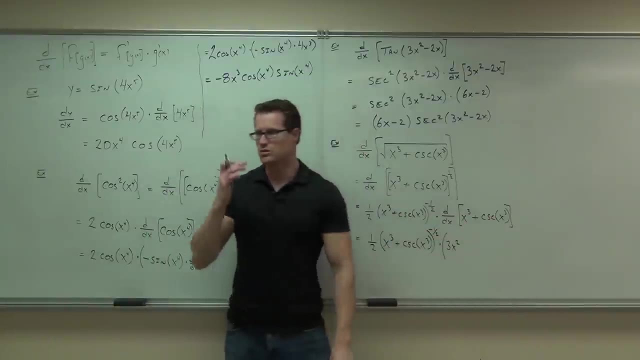 by addition and subtraction, and that's okay. So I just take this and go: oh, yeah, yeah. yeah, I do three x squared, Not a problem, That's fine. Can I take the derivative of cosecant x cubed? 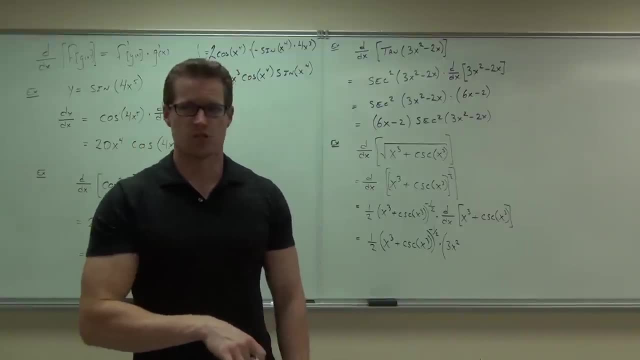 Can I take it directly or do I need a special rule for it? Three, Not a problem. Do you see the chain rule here? Chain rule says: sure, it is cosecant, but if there's something special in there besides an x, 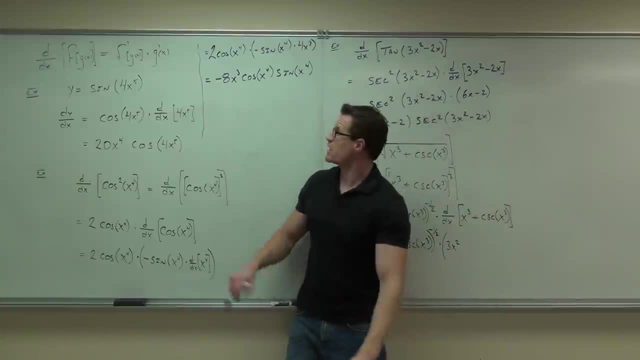 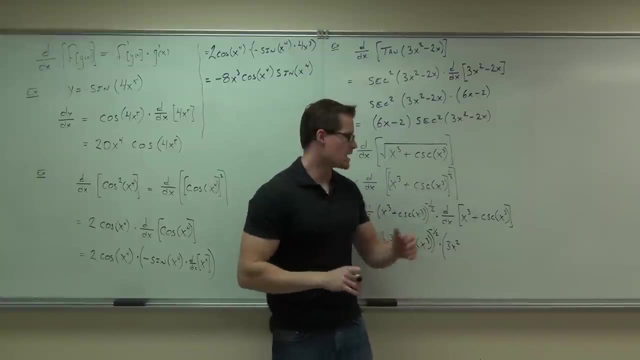 that means a chain rule, because that's a composition. just like this one was, just like- oh, what's the other one? Just like that one was, just like this one was. That's a composition. You need a chain rule there. 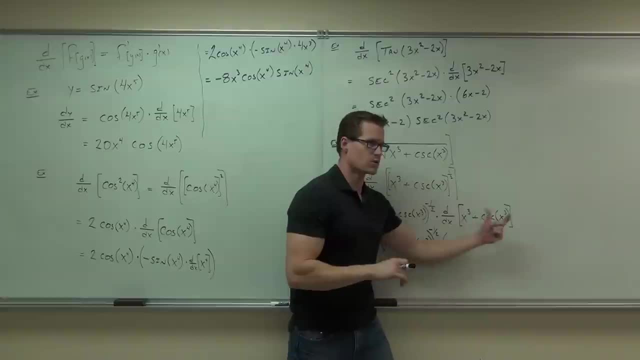 If you just give me the derivative of cosecant with x cubed or the derivative of cosecant with three x squared, you're not hitting the money on this class. all right, You're missing the chain rule. You're missing some factors of x. 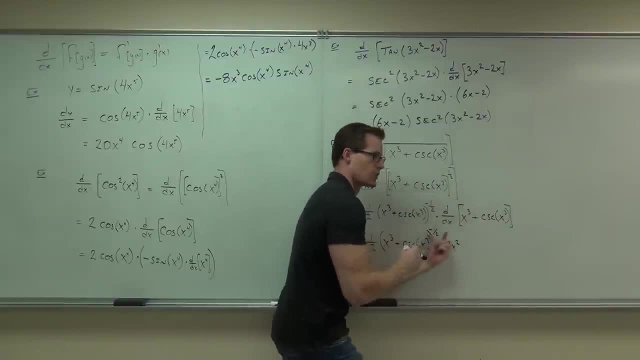 You're missing a whole lot of stuff here. So this is great, sure? Now let's take the derivative of cosecant x cubed. What's the derivative? the chain rule says: take the derivative of cosecant. so what's the derivative of cosecant? 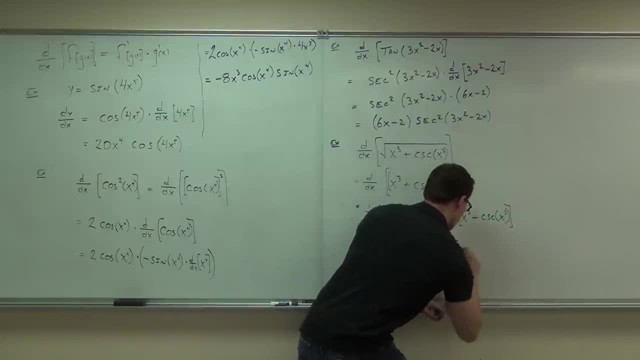 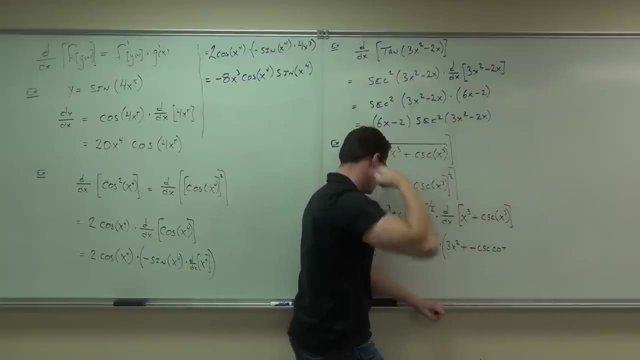 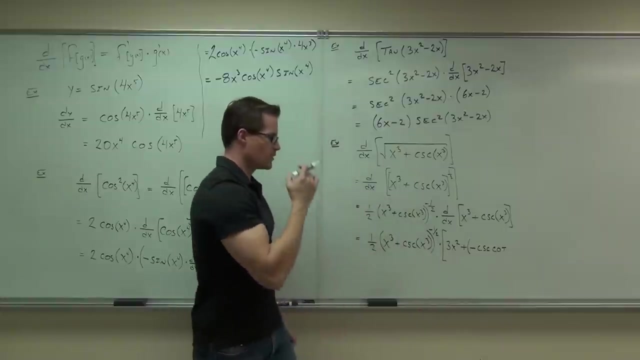 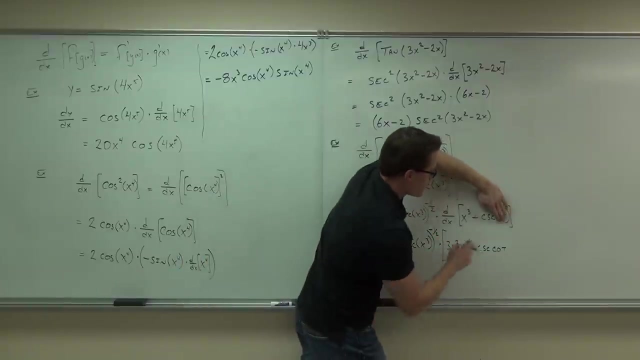 Negative cosecant over tangent. Okay, Let me change that to a bracket too. Negative cosecant cotangent of of what. X to the third. Good, because this says the chain rule. you take this derivative? great, I just do that. 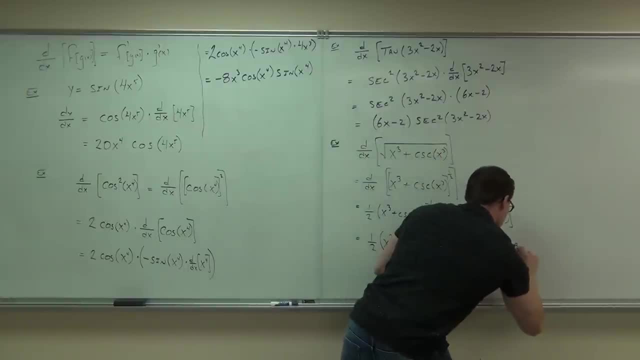 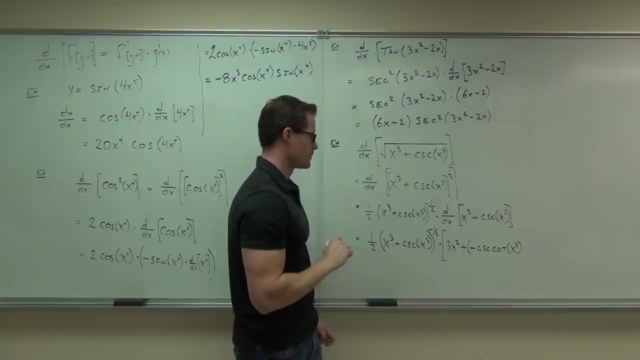 but you leave the inside alone for now. That'd be cosecant x to the third, cotangent x to the third, Or is it okay to leave it? Oh yeah, sorry, Did I forget? oh, I did forget that, shoot. 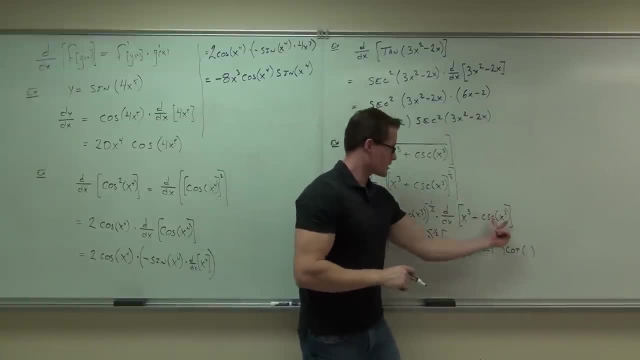 I knew something looked funny, thank you. So this says: when you do this, cosecant is cosecant cotangent. so cosecant x was cosecant x, cotangent x. What our x is is x to the third, in this case. 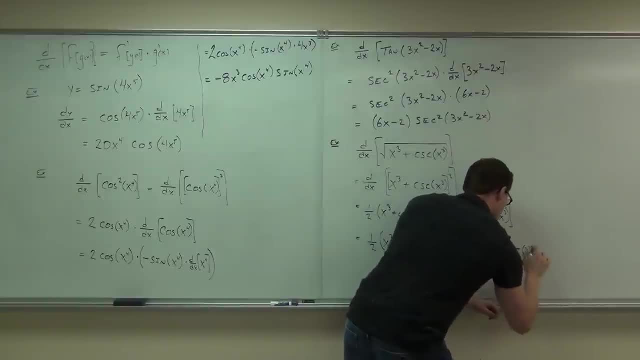 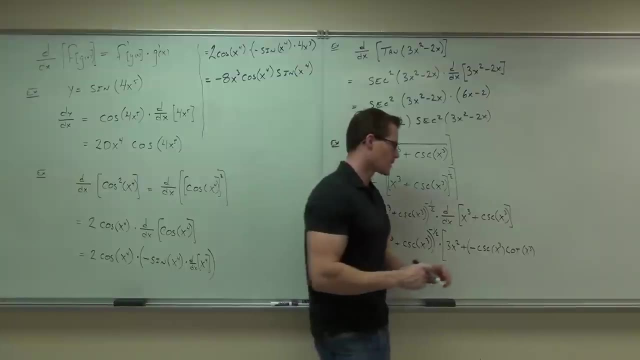 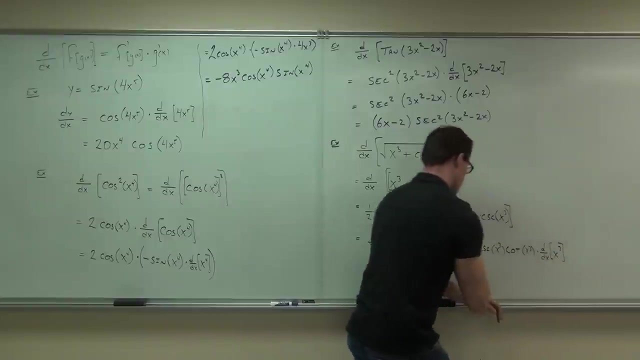 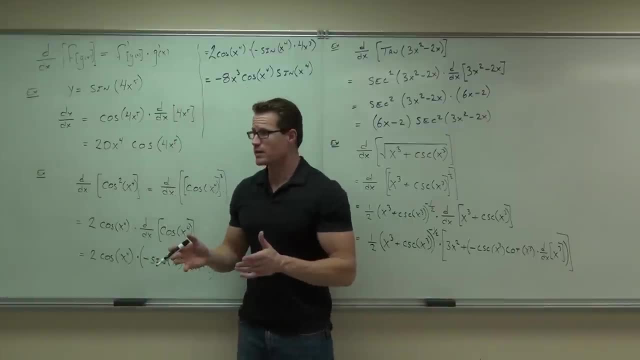 Sure it looks ridiculous. yeah, I know that, But can you do it? Do you see where it's all coming from, how it's all fitting together? Is it really really all that bad? Not really. it's just you gotta be careful, really careful. 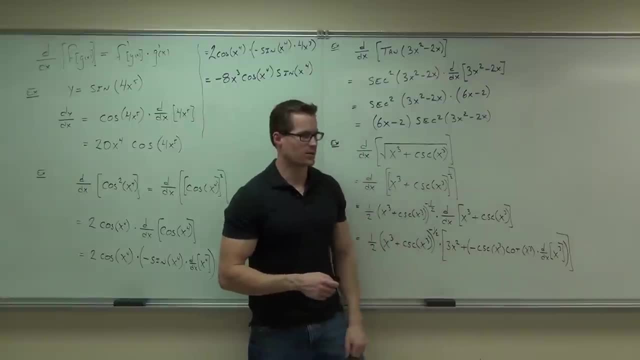 I mean, the only, probably the hardest thing is memorizing cosecant and you go. hardest thing here is derivative of cosecant, is negative cosecant cotangent. Hopefully that's right. is that right? Just check your notes. Good, all right. 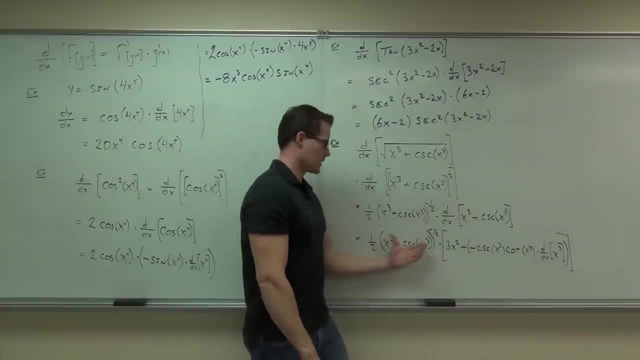 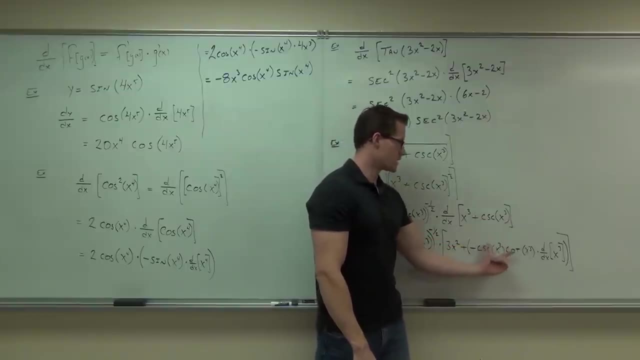 Because here well, general power rule, sure, we got that down. Calculus is done Here. derivative of this one: very easy, 3x squared. Derivative of this one, that's chain rule. This is negative cosecant cotangent. 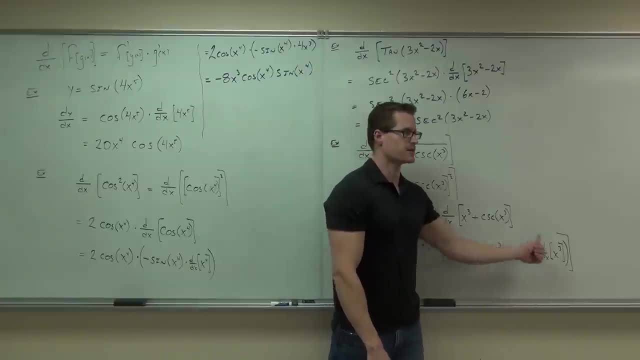 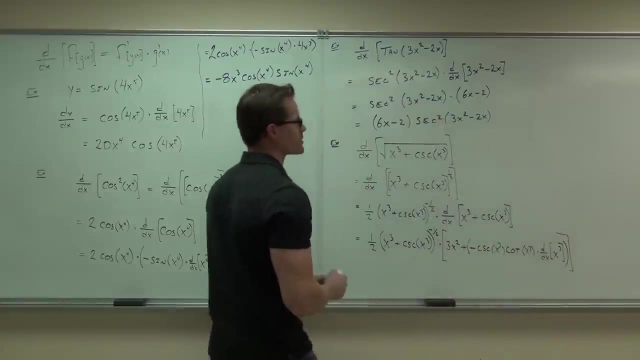 You do not change the inside. You multiply by the derivative of the inside. That's gonna be 3x squared. That's where we're getting 3x squared. Are you with me on this so far? Let's see if I have room for this stuff. 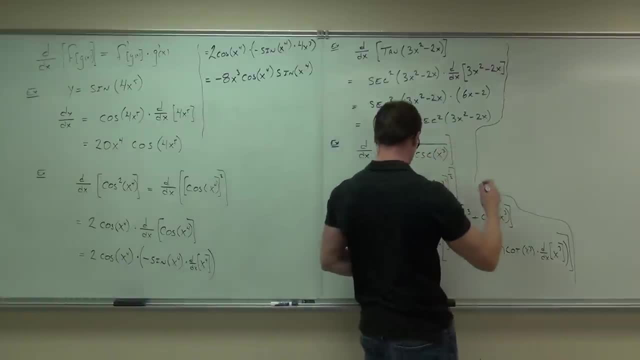 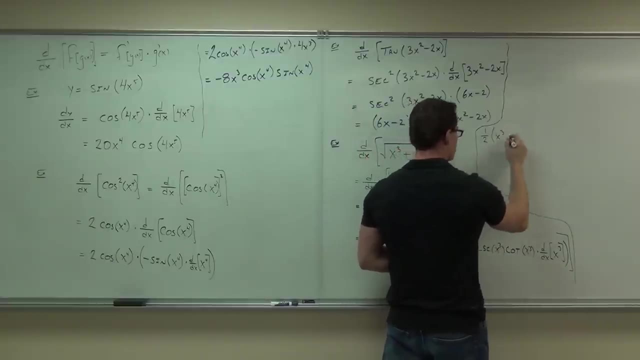 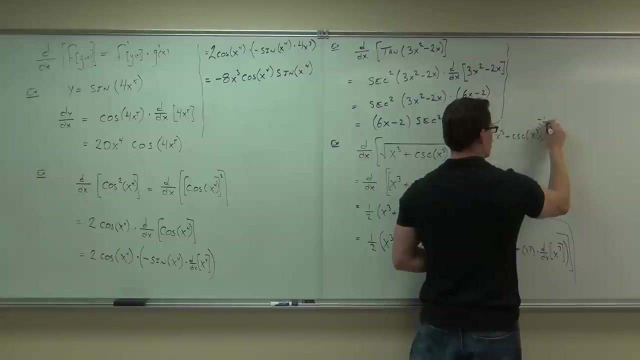 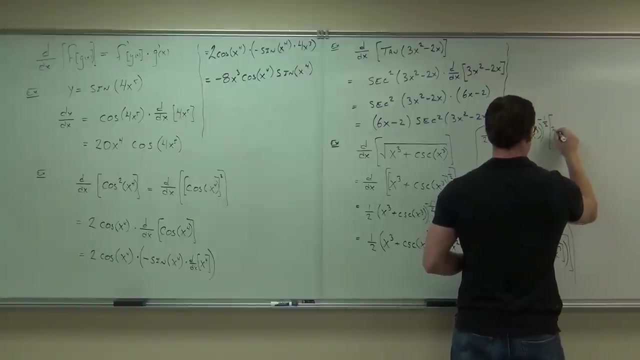 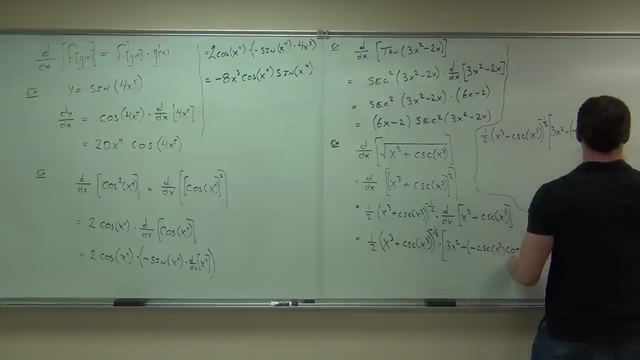 I'm gonna go right here. So one half all this to the negative one half, 3x squared, negative 1.5.. Okay, All right, All right. So we have negative cosecant, negative cosecant cotangent. 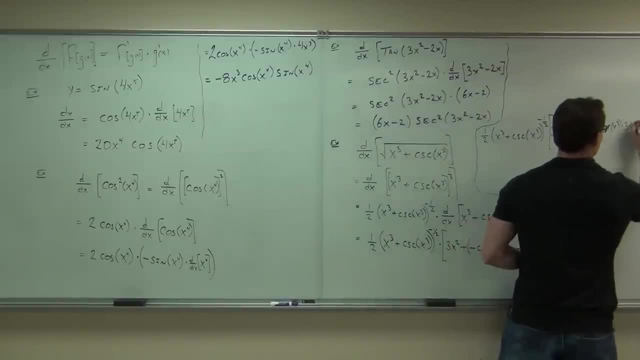 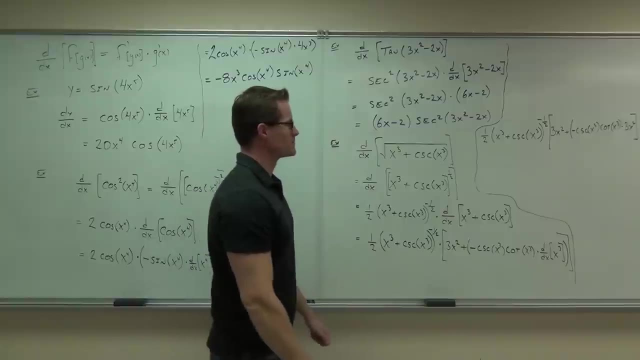 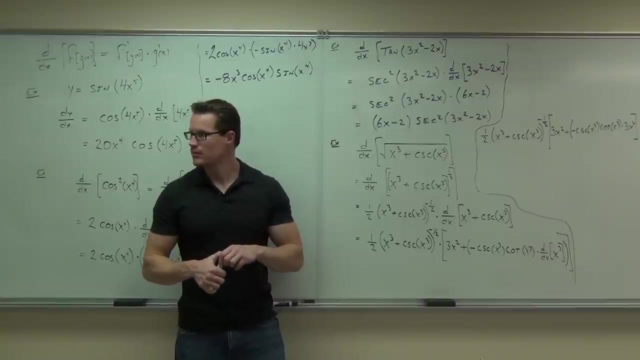 and lastly, we have a little piece 3x squared. Hope that fit. I think so. Uh, one second. Sure, No, it's fine. Okay, No, the 3x squared. is that going to get multiplied with both of those terms, the x cubed plus? 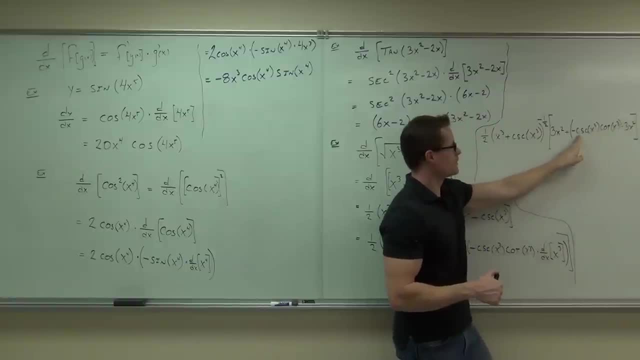 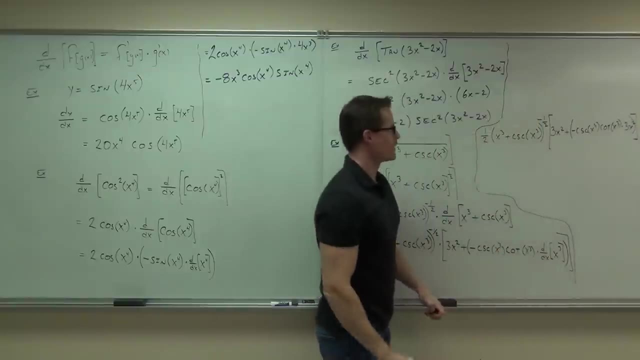 You mean here and here, Right, or just stay with the cotangent. This right here ends in parentheses, right there, So that 3x squared. this 3x squared is not associated with the x cubed, So this does not get distributed to here. 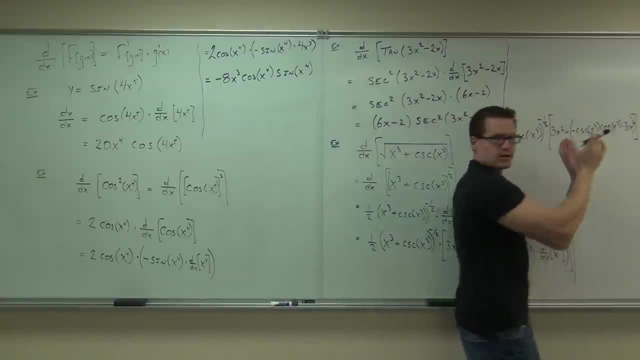 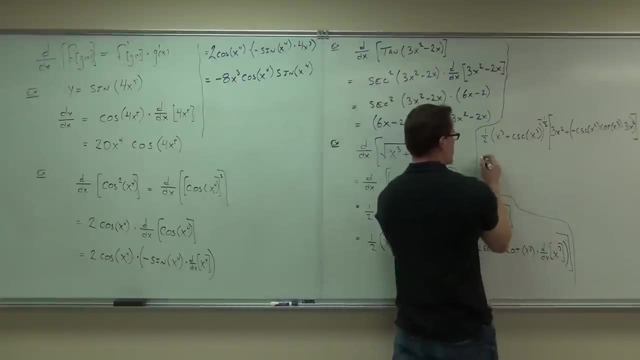 This right here is 3x squared plus this entire nasty looking expression. That's what that is. So when we try to simplify this just a little bit, let's look what happens. We're going to get 1 half x cubed plus cosecant x cubed to the negative 1 half. 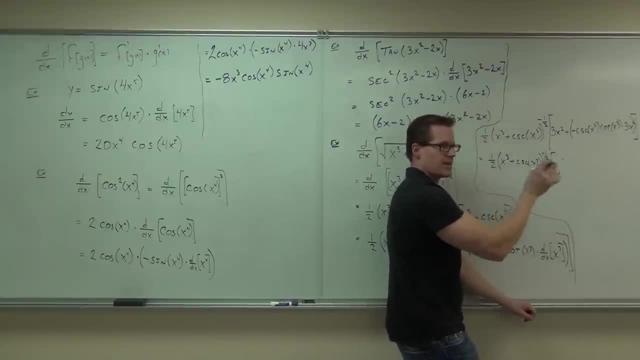 We're going to get a big bracket. 3x squared doesn't change. you don't distribute to that. That was just a standalone, Just a small derivative of 3x squared. This we're going to pretty this up a little bit. 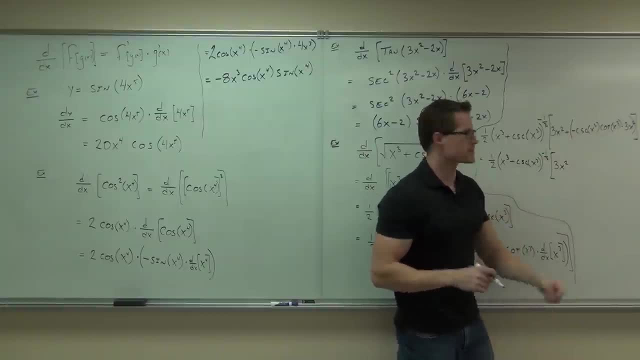 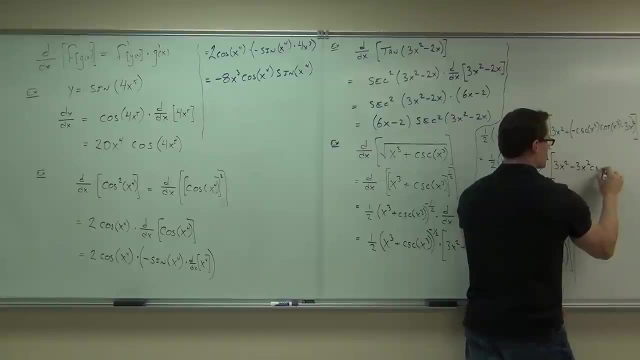 Positive, negative, plus, minus. what's that going to be? Minus? I'm going to move the 3x squared out front, So this will be minus 3x squared: cosecant x cubed, cotangent x cubed. 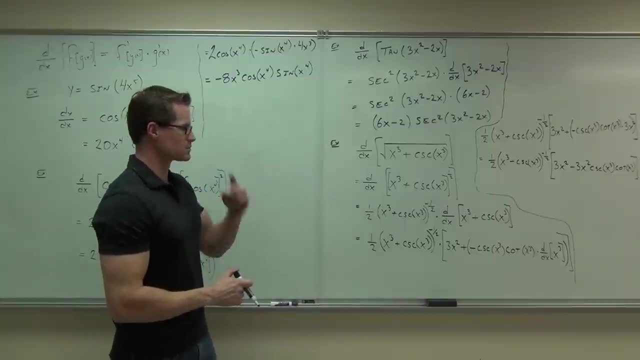 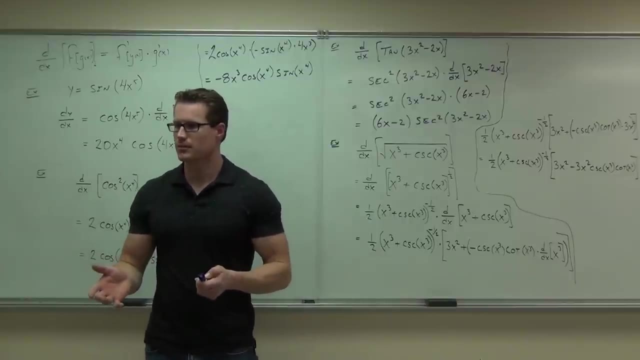 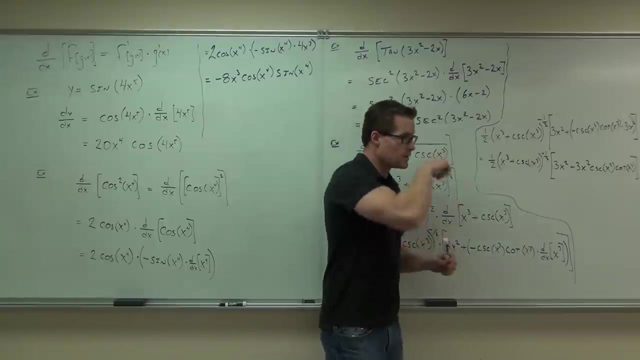 And that's your derivative. That's pretty nasty. Can you follow it? Yes or no? Yeah Or like who? There's no simple way. So can you? would it be correct if you would go 3x squared minus 3x squared, cosecant x cubed? 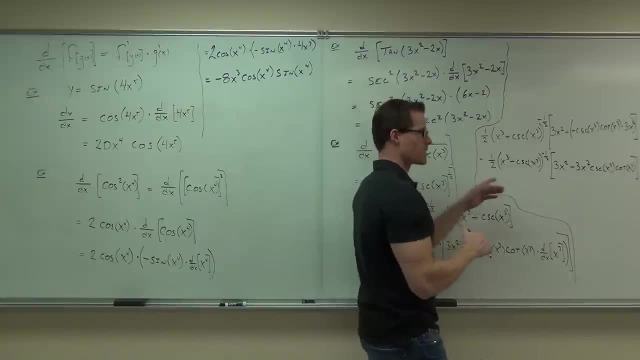 cotangent x cubed over 2 times. Sure, Now I'm going to show you that right now. So if you do want to put this back into this format, this would be. I mean, like, do you want us to, or can we just leave it at that? 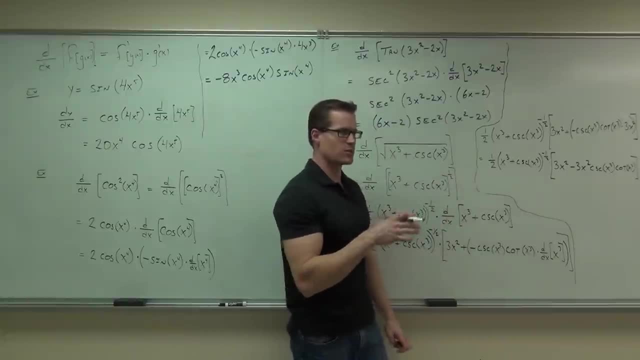 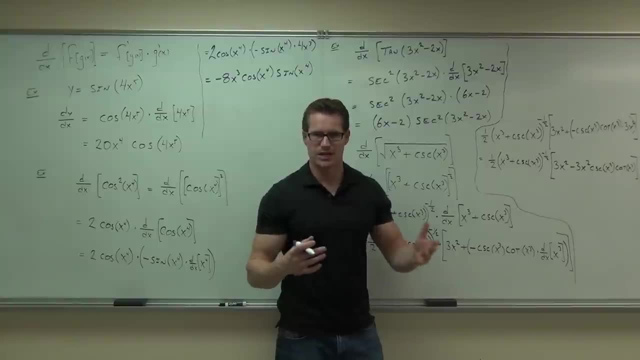 probably think of, that gets a root. That's generally the idea. if you used exponents, leave them at exponents. Also, one more thing: If some of you guys don't get fancy with this, in fact you're out 3x squared. 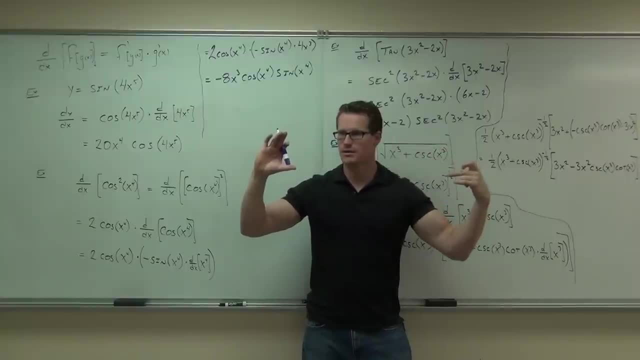 you'd have 3x squared times that Sometimes identities will help with that, sometimes you can do system or a lot of one minus step in your squares happens. this is the three. I don't know to even supply anymore, not because I can make stuff up in my head. 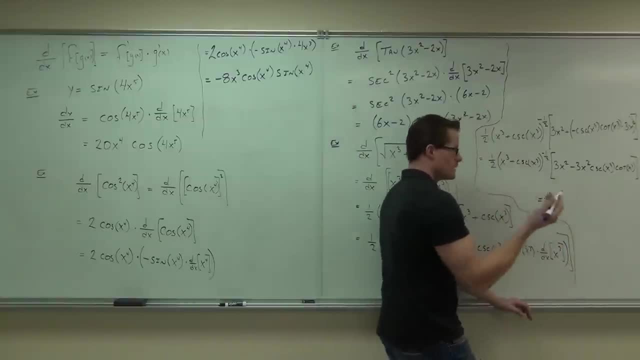 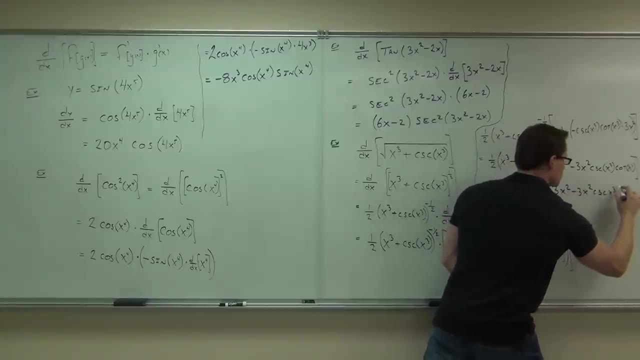 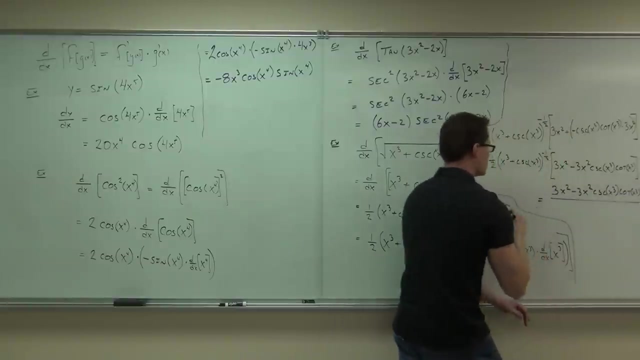 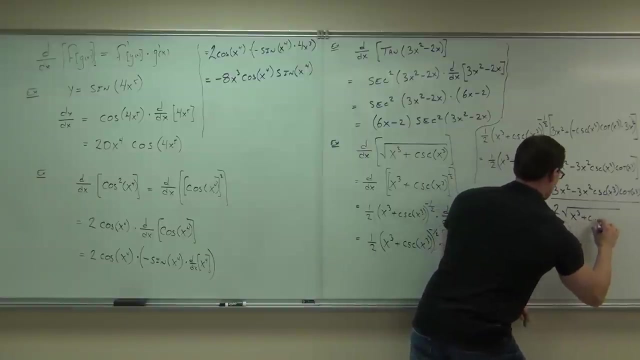 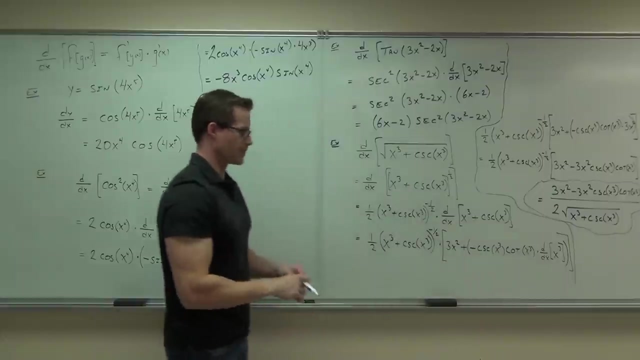 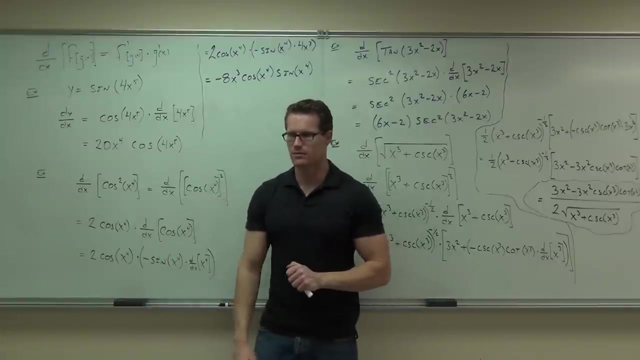 but what you could do. one last final thing would be this: if you made it there, you can make it there. that's fine for me that's great. so we did general power rule. we got it here's inside, not changing derivative. inside got it. we're going to do 3x squared derivative. this is a chain rule. 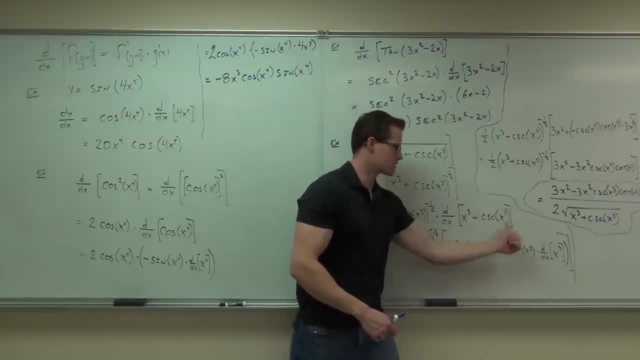 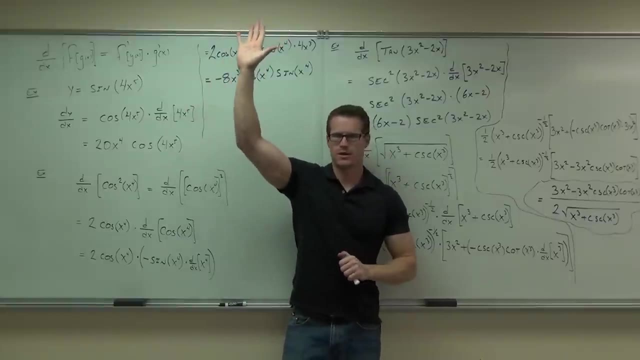 chain rule says negative: cosecant X, cotangent X. so we leave that inside alone, multiply by the derivative of the inside and then, after that it's eliminated. I'm going to go over this implication. originally, I feel okay with this problem. sure they're nasty? yeah, I get it. they don't look fine, but they're useful. 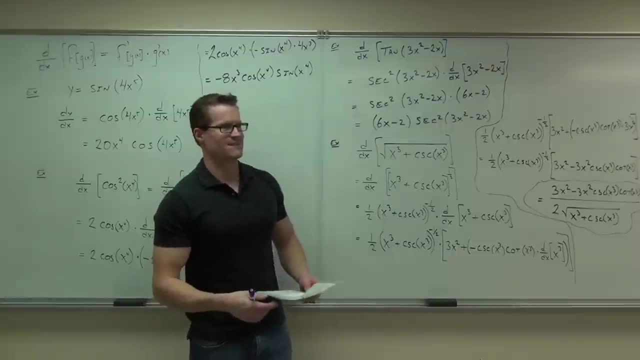 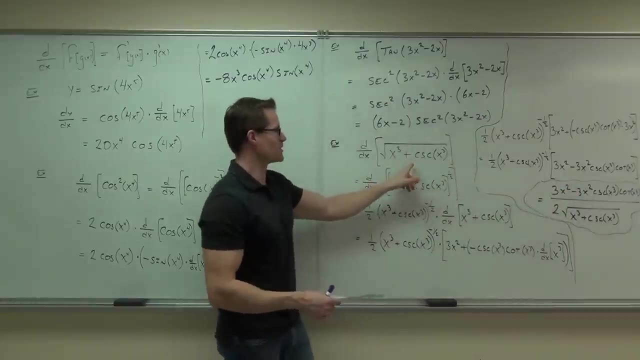 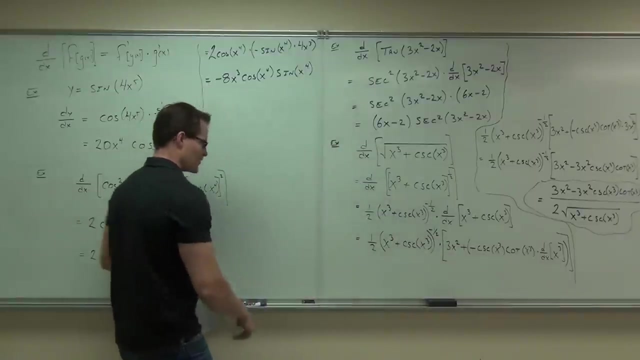 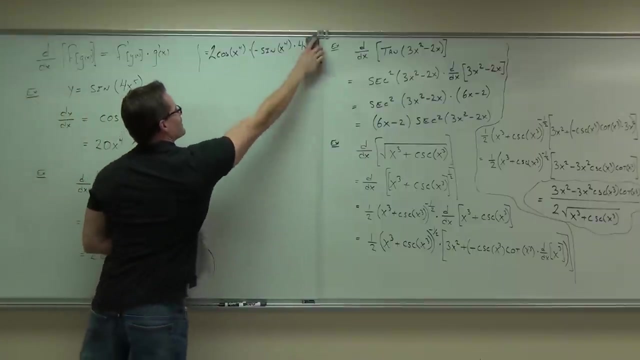 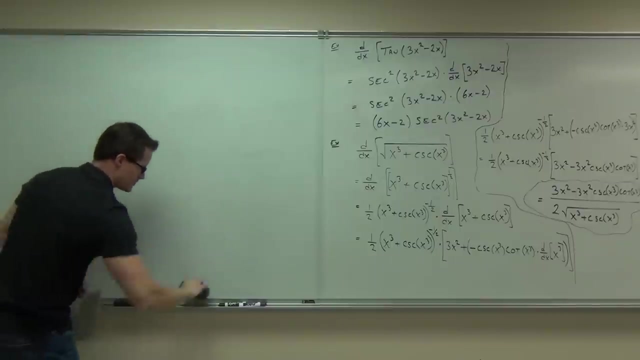 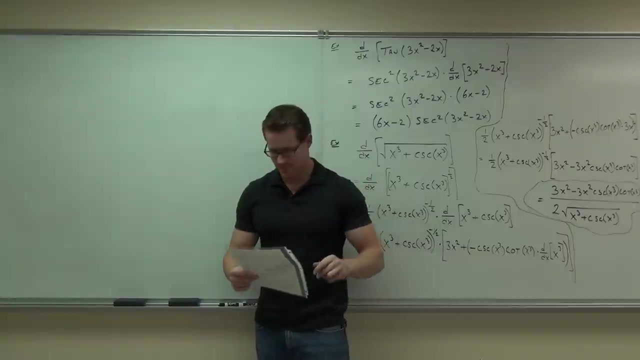 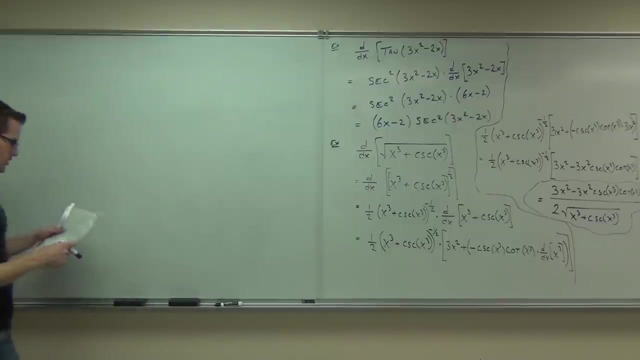 what did you just find slow? all this means is M M for this. oh yeah, I don't know. that looks like not a clue. don't really care. honestly, ready to keep going. two more, two more. what you want to do first. you want to do the hard one or the harder one? you want to do the harder one, yeah. 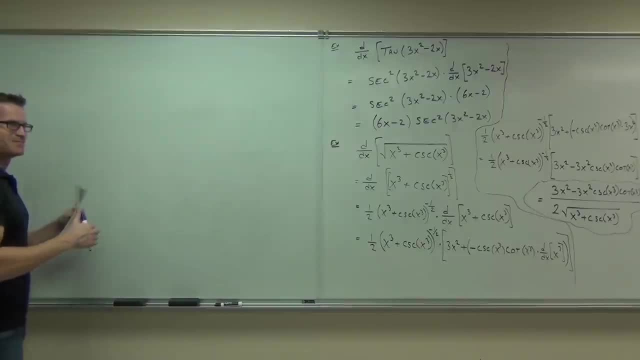 all right, you asked for it. we have three more. actually, the hardest to last. two more. yeah I'm. that's not a good sign. nope, nope, that's not a good sign. I got a little high. I'll just give you a minute until we get you to the other side. 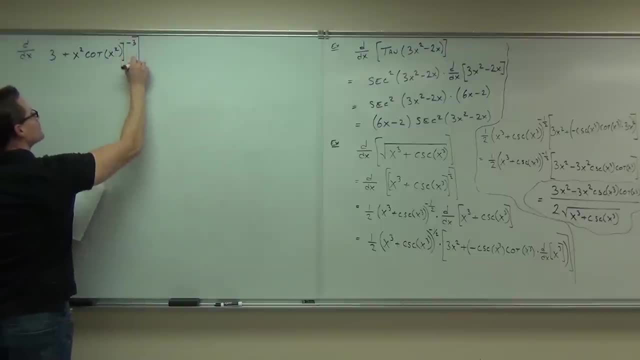 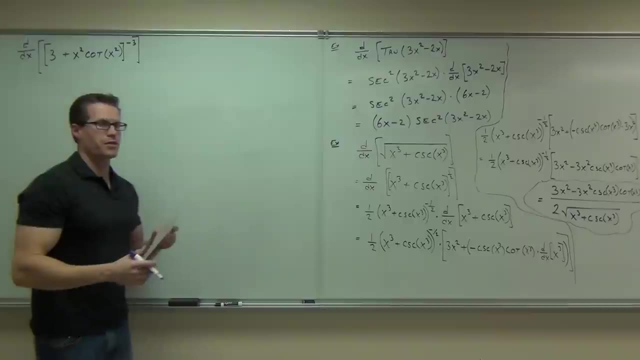 yeah, okay, you're going to just push this into the other side. you're going to get into the other side. you're going to get into the other side. okay, notice one thing, please. I could give this to you with a slightly different look. check this out. if I gave it to you, like this: 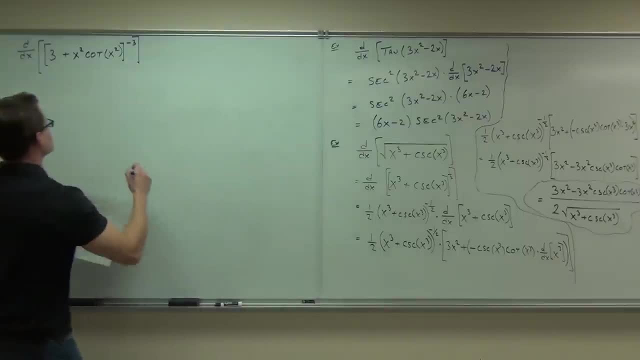 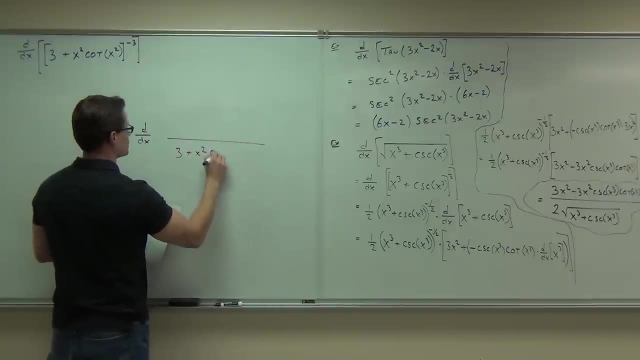 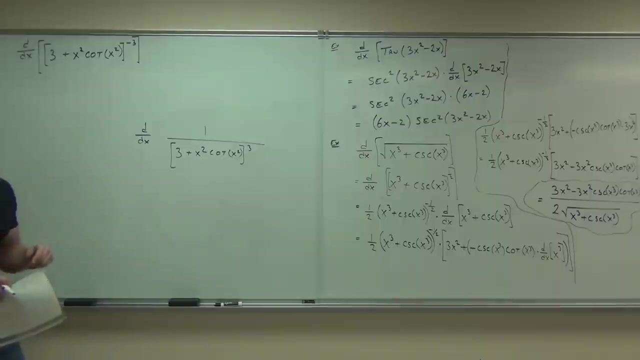 if I gave it to you like this: look, check this out. if I give it to you like this, Would you verify that? that's exactly the same thing? You probably, unless you have a function of x up there- probably shouldn't use quotient rule here. 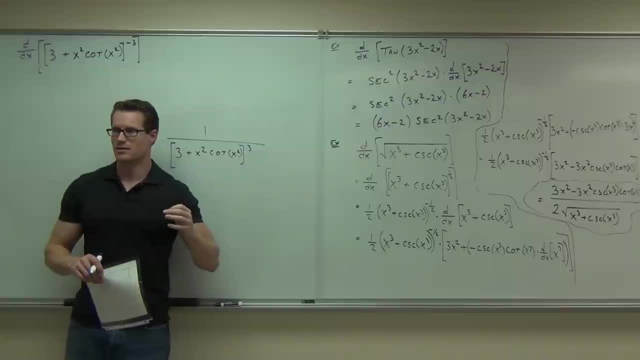 If you use quotient rule with this, it's going to explode in your face. Paper's going to be like no Done, It's not going to handle this problem. It's going to need a special paper for that. That'll sell me. 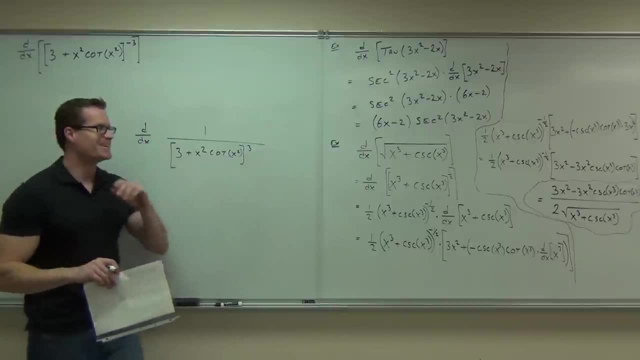 No, do this Unless you have a function of x, because you don't want to deal with that either. If you had a function of x and you move this up top and you're talking about product rule, you can do that, It's fine. 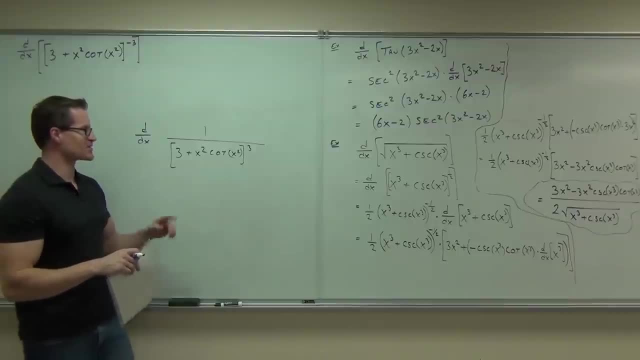 But that's just a constant Move that up for me, would you? And that way you just use a general power rule instead of a quotient rule. A quotient rule would just be ridiculous. So verify that's the same, Then you can start looking at it. 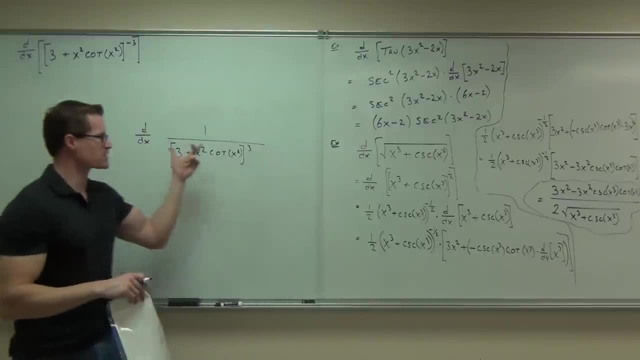 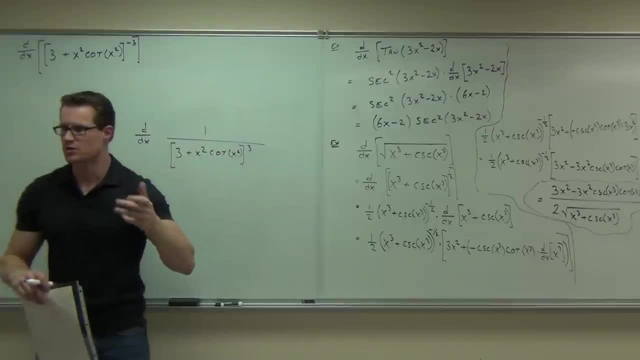 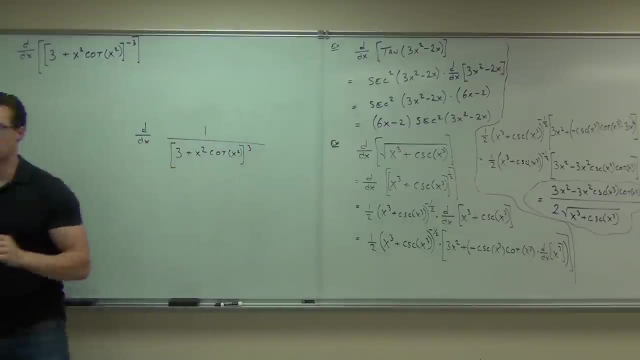 It's a constant. It's a constant. It's a constant. No, Didn't look like that. It's a constant, But look at the size of what we're doing on this problem. What do you think the pi's is? 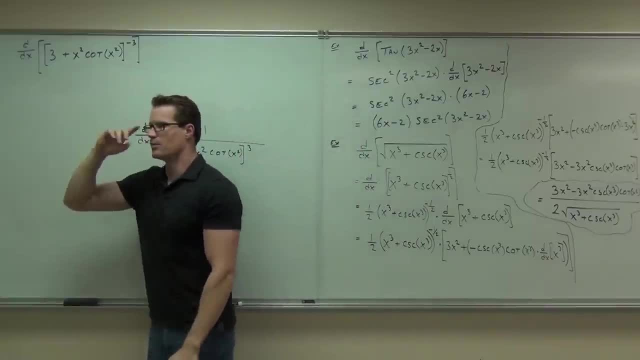 What's the biggest piece? General General power. Very good, General power rule encompasses this whole entire problem. Let's walk all the way through it Within the general power rule. after we do that, we're going to come down to these 2. 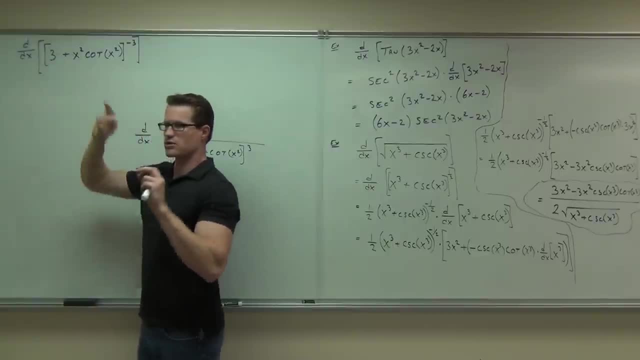 things right. Yeah, What's the derivative of the 3? Zero? That's great. That way, we can do that nice and easy. How about this piece? What encompasses this? just this? Is it product or change? It encompasses the whole thing, doesn't it? 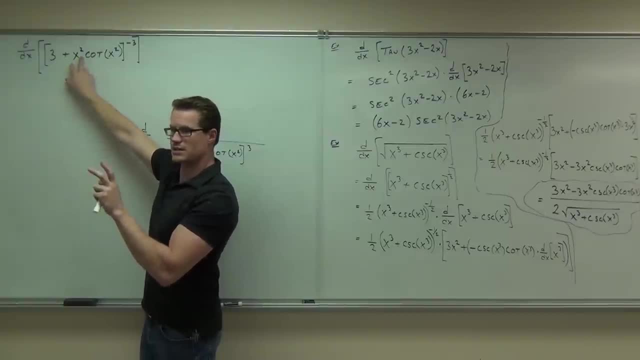 Now, within the product rule, I'll take a derivative of x squared, that's easy, two x. And then I'll have to take a derivative of this little piece right here. What is this little piece? Chain rule, That's the chain rule. 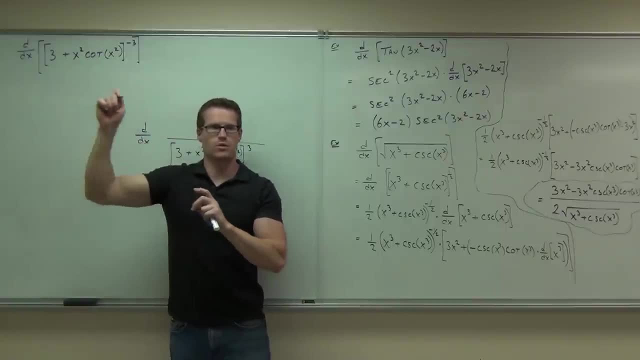 So we're doing general power rule. We will have the product rule within that, we'll have the chain rule within that. okay, It's nice to think about those things, though. Nice to think of it, just kind of like a graphic organizer. 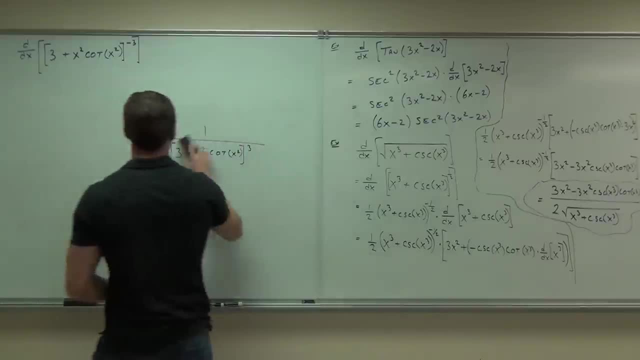 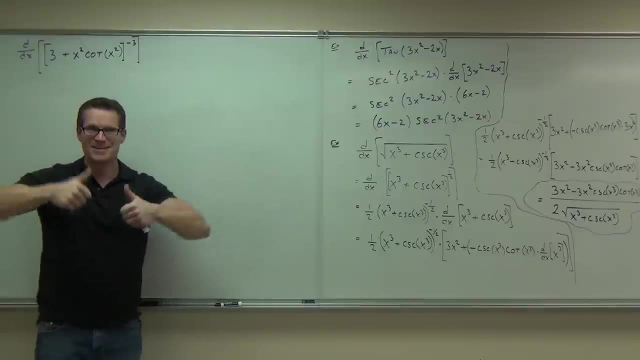 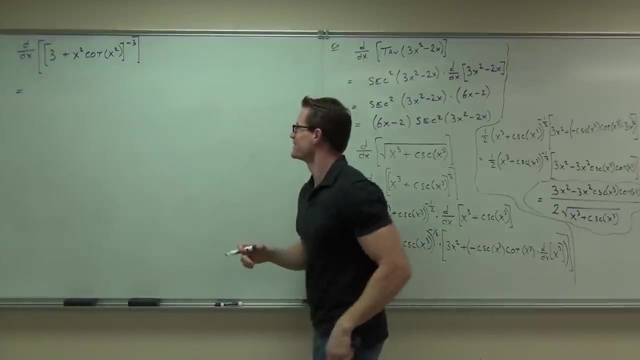 or an organizer, advanced organizer, for your thoughts. Ready, Yeah, Woo, Make me study two more applications. Yeah, yeah, but they're easier. sort of, Sort of, Sort of, Yeah, sort of. Let's get to it. come on, you tell me what to do. 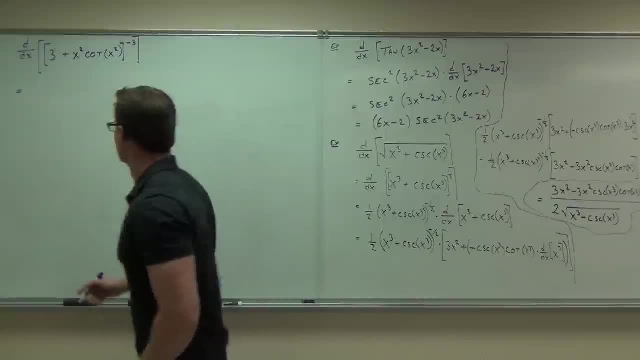 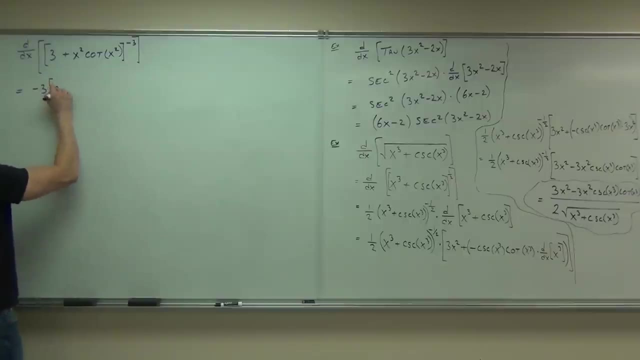 What am I gonna do now? Move the x, drop your x to the x, move it there. Keep everything on the same side. same Good, keep everything the same. So negative x over, not minus one. negative three, which is negative four. 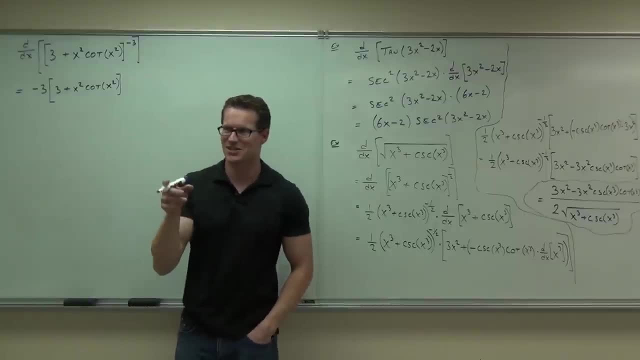 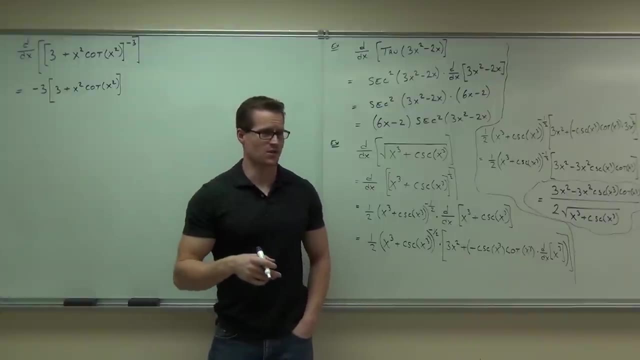 Yeah, negative two, right. You know how many mistakes I saw in your homework with that. Be careful. I mean, it would be so sucky if you knew how to do this stuff. and you gave me a negative two here, right? 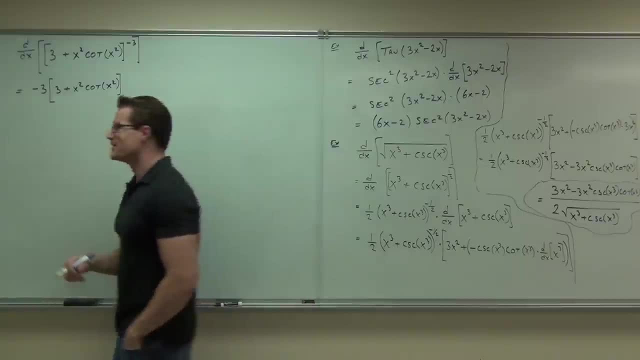 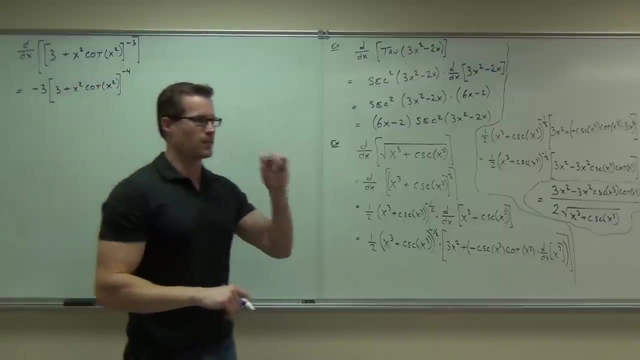 That would suck, because I'm like: oh, you know what you're doing, Gone. No, don't do that. it's negative four, Negative four. subtract one from that. and then what? now That we multiply it by the derivative of the inside? 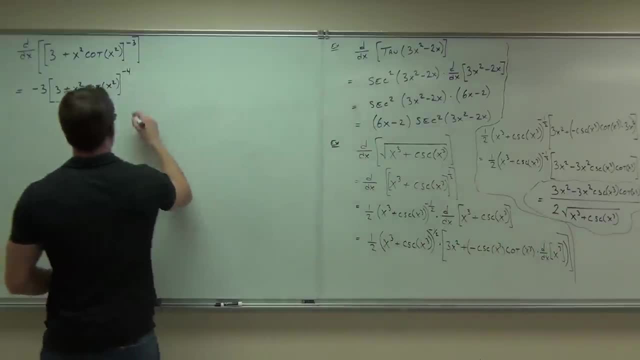 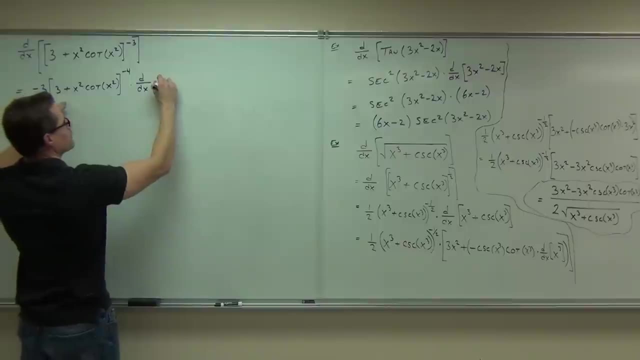 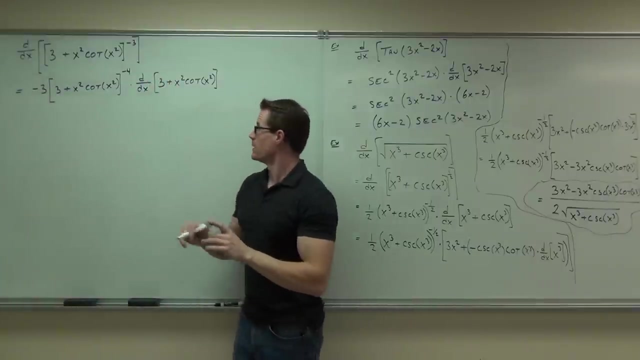 Write that out. go for the derivative of the inside right now. When we say the inside, we mean the entire expression that you basically ignored. So you should have that on your paper. do you have that on your paper? Yes, Hey, calculus is done here. you're done with that. 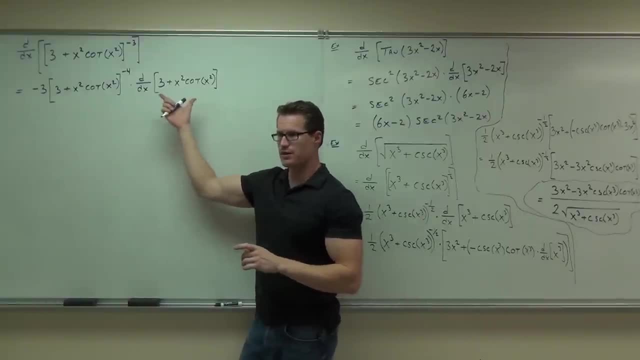 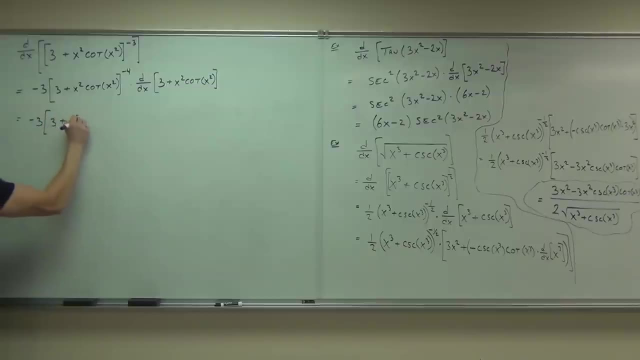 We're just working on this piece over here. Let's take the derivative of this piece over here. So this is negative three. What's the derivative of this piece over here? X squared, cotangent, x squared. all right, negative four: you're done with that piece. times. 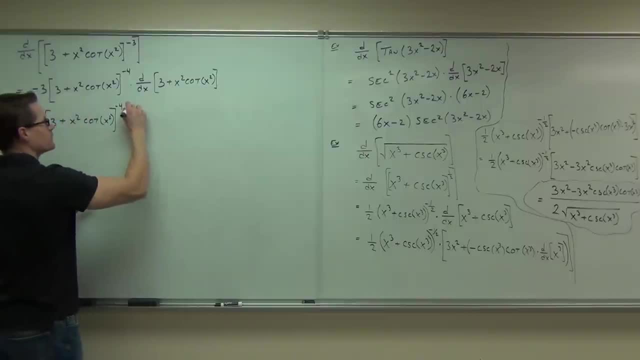 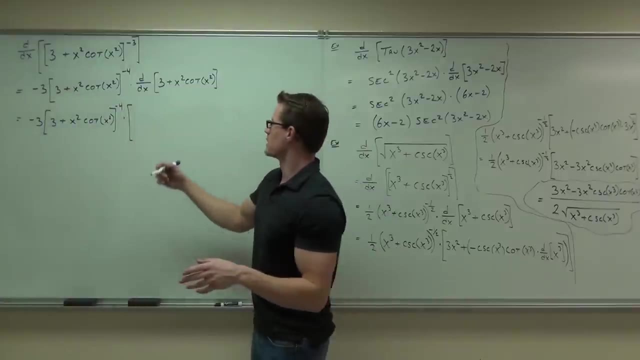 probably want a bracket. you need a bracket, Big bracket. We have a lot of stuff, Big bracket. Why big bracket? Well, let's look at that Derivative of three. Oh, that's nice, that's a nice one. 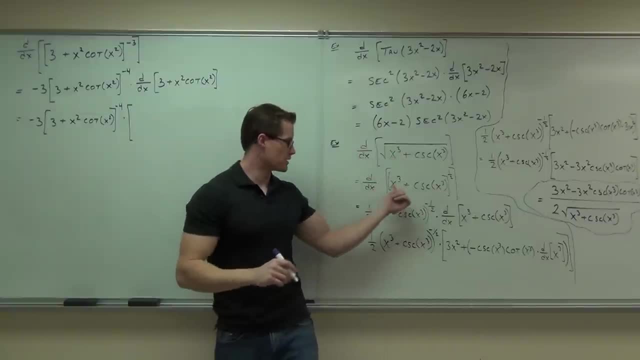 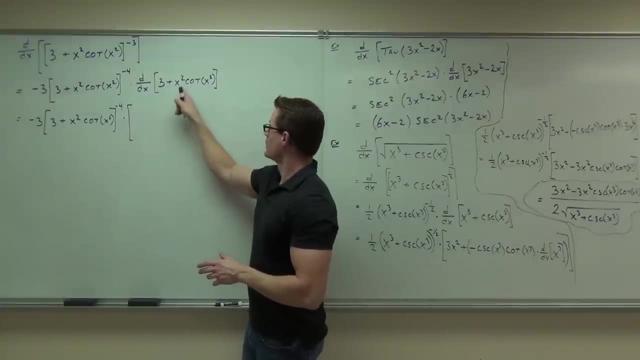 If it was just another expression, we could have taken a simple derivative, just like we did right here, right there. So no problem, This is zero. I'm not even gonna write. the zero Derivative of three is zero. it's constant. 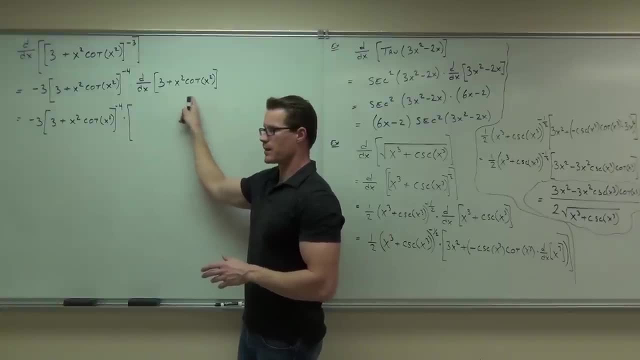 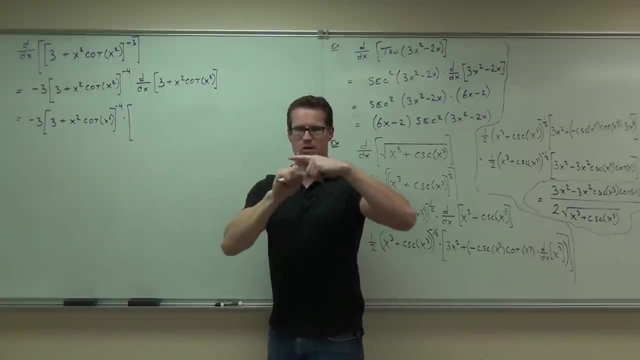 Let's focus on this one. You said what happens here, Which is why we need a bracket, because, oh, I'm sorry, no Product, product, Product, product. Which is why we need a bracket, because we're gonna have an addition in there. 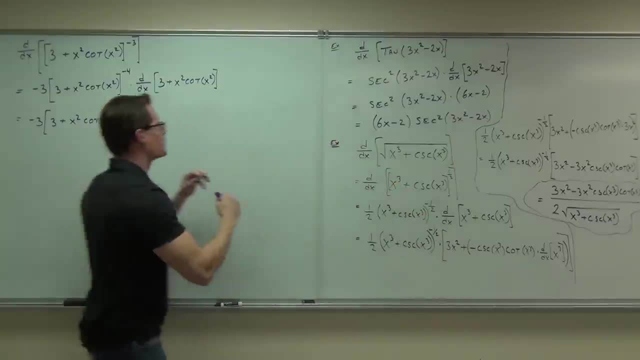 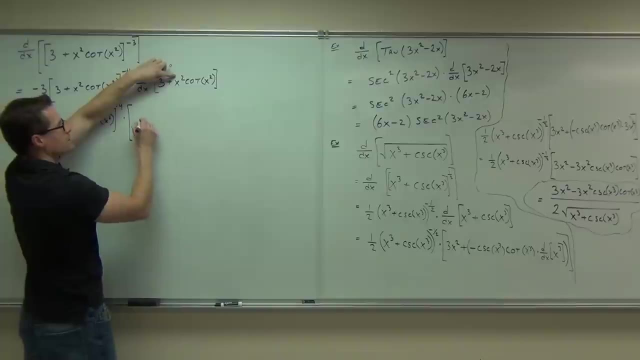 Product means plus you follow, So we need that bracket to organize that. This says: okay, I'm gonna have three's gone. that was a zero, so this goes to zero. This says the derivative of the first times the second. are you seeing how all our rules? 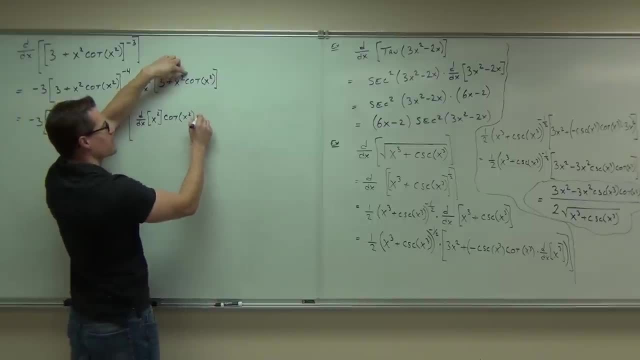 are coming back to haunt us Or help us. however you want to look at it, Plus or minus folks, Plus what? finish this off? You gotta say it Derivative of cotangent x squared. Okay, so I'm gonna do x squared first. 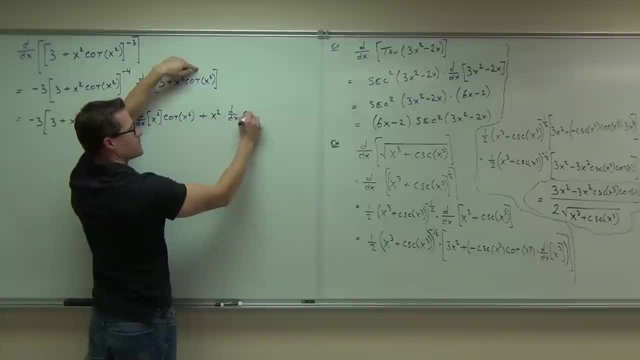 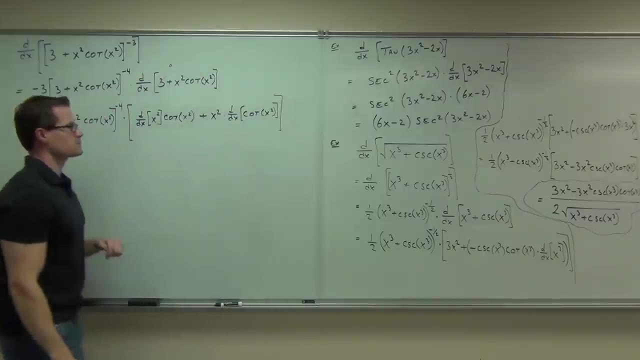 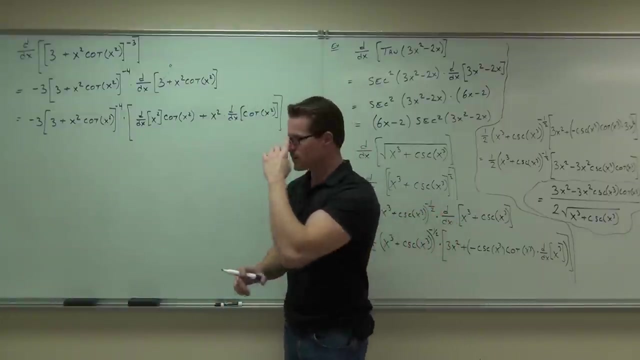 that's how I like to do it. Derivative of cotangent x- squared. Derivative of cotangent x- squared. Derivative of cotangent x- squared. Finish off your bracket. Okay, quick head nod if you can follow that. Yes, okay, cool. 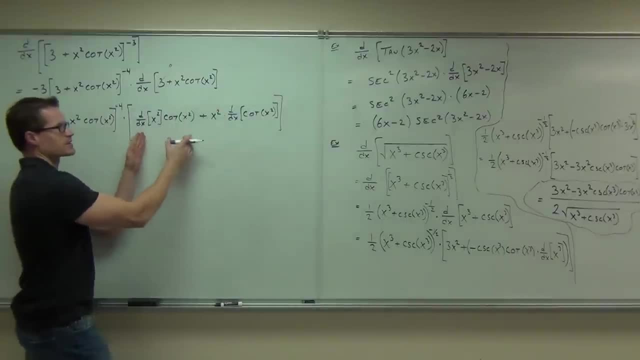 Follow our DDXs Here. no DDXs Here. DDX Here, DDX. Negative three: three plus x squared cotangent x squared to the negative four, power Big bracket Derivative of x squared everybody. what is that? 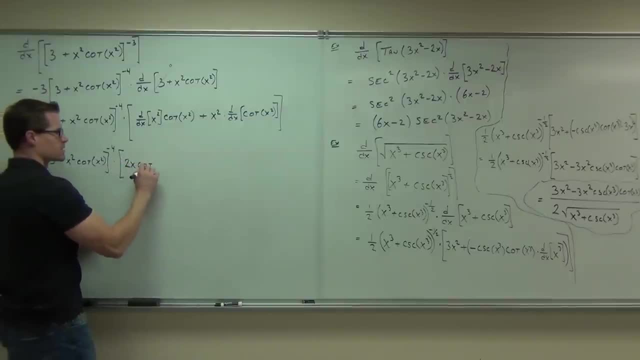 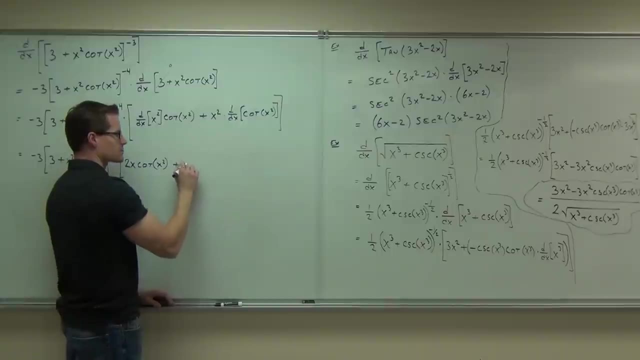 Well, that's nice. two x cotangent x squared. Well, we got that done. Plus, I don't take the derivative of this x squared, I simply follow my DDX x squared. Tell me what happens here, please. 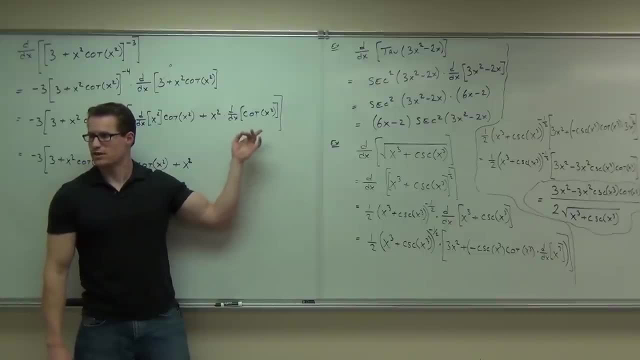 What happens here, what happens Now? I see a chain rule. For sure, that's a chain rule. Do you guys see the chain rule? Absolutely chain rule. We predicted it right. we had general power rule, product rule, chain rule. 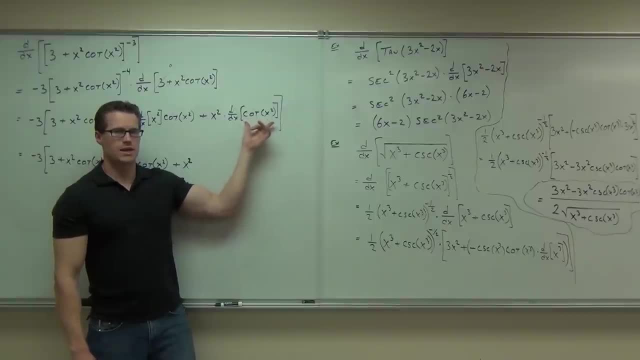 So we had that right. Let's go ahead. let's do follow the DDX, do that chain rule. Chain rule says: here: I'm probably gonna have at least a parenthesis to organize my thoughts a little bit. You don't necessarily need it here. 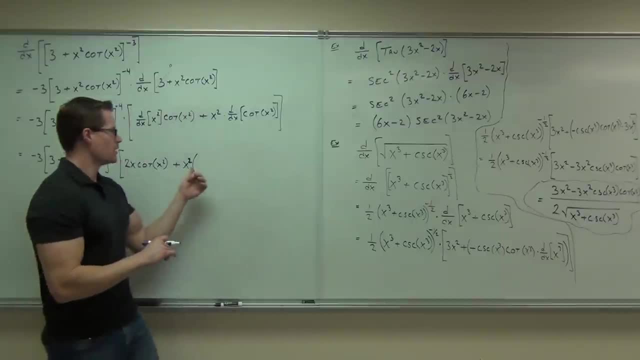 because it's just a chain rule, you're not adding or subtracting, but it's kind of nice to have What happens with that. What's the derivative of cotangent Negative, cosine, cosine, Negative, Negative- Is it Negative? 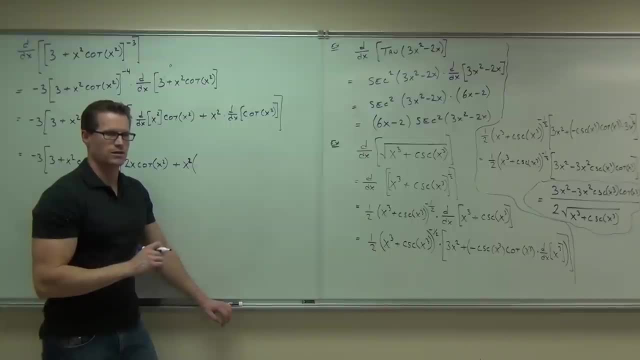 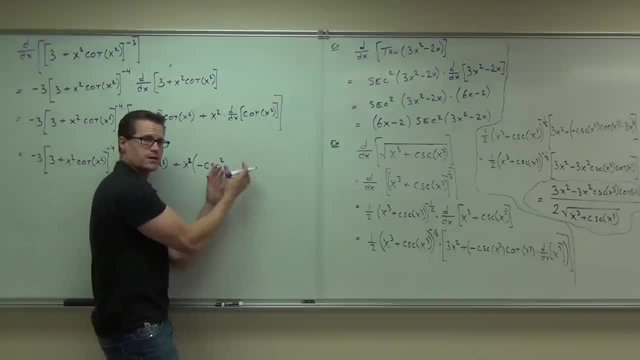 So negative cosecant squared of oh, of what folks? of what? Two x or x squared, X squared, Good, And then we're done, right. No, Oh, there's one thing: if you forget this, oh, it blows your whole problem up. 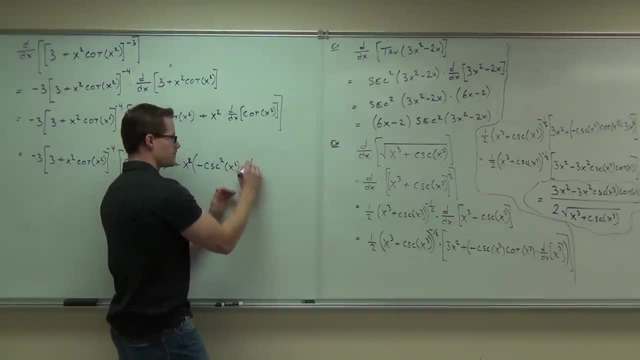 But if we don't forget it, we have the problem right. I want ddx of x squared Times. what? Two x, Yeah, Or d. I want ddx of x squared. This is this parenthesis. That's the bracket. 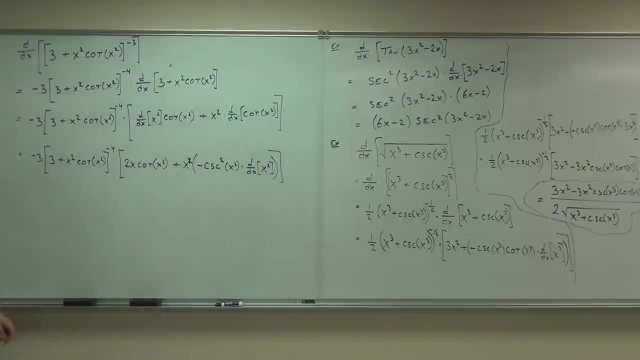 We didn't have five problems on that test. I can give you one. I can give you one problem and it would show you everything. Seriously, I could. I'm not going to Because if you got it wrong, oh, that sucks. 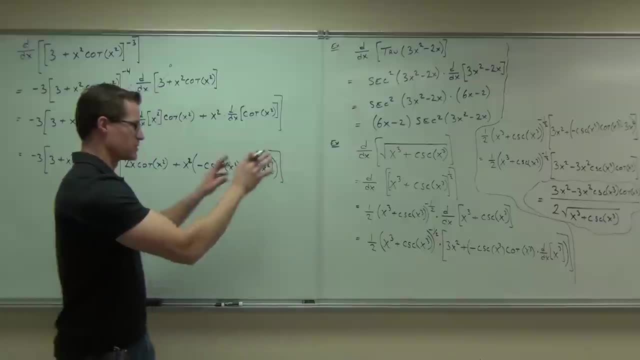 Here goes 20% of your grade. Ha ha, ha ha suckers. No, I wouldn't do that to you. I might do that to you. What about me? I might do that to you. What about me? 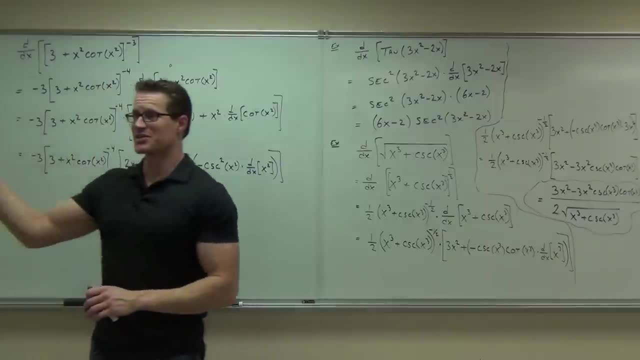 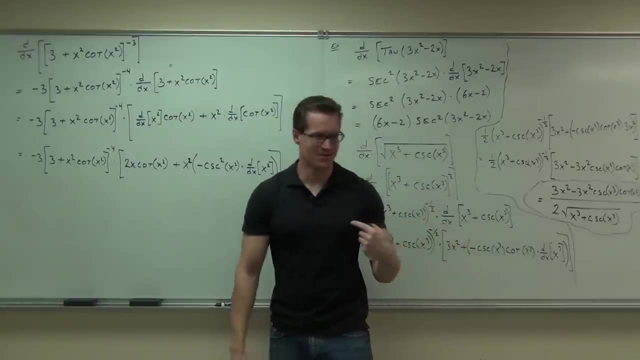 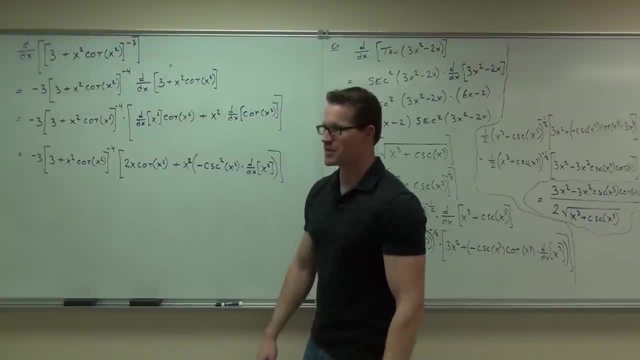 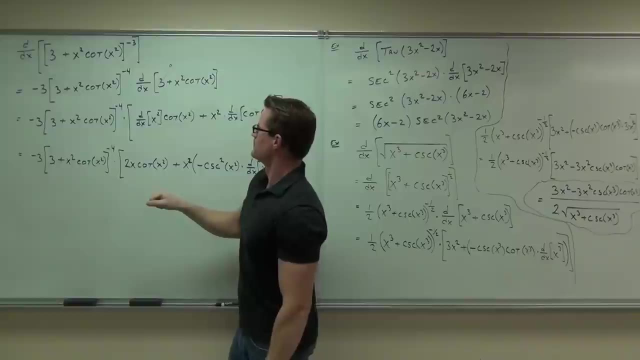 No, No, I wouldn't do that to you. Would that be worse than kicking a puppy? No, I'm about the same level as kicking a puppy. Okay, So Kick the puppy. General power. Ha, ha ha. 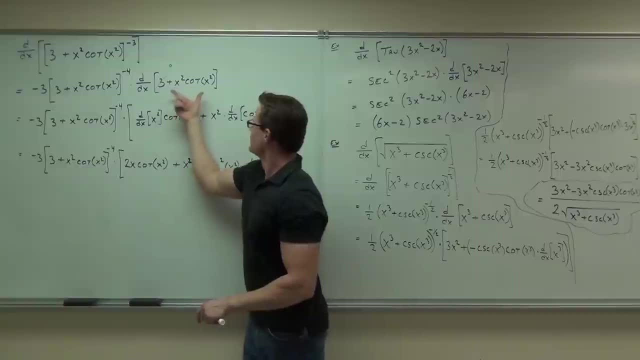 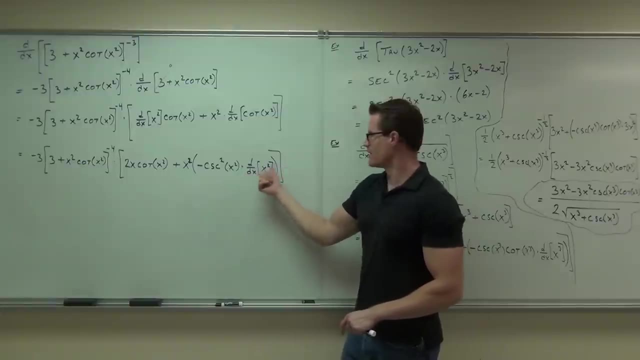 Do it. I kicked the puppy for you. Do the inside Product rule. No problem, Chain rule. We got it Derivative inside, right here. That's going to give you two x and we're done with the calculus. Did we do that? 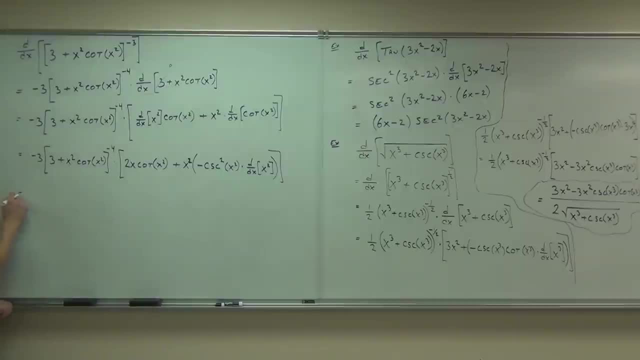 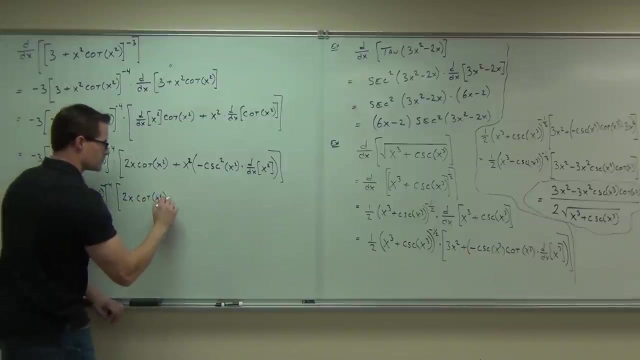 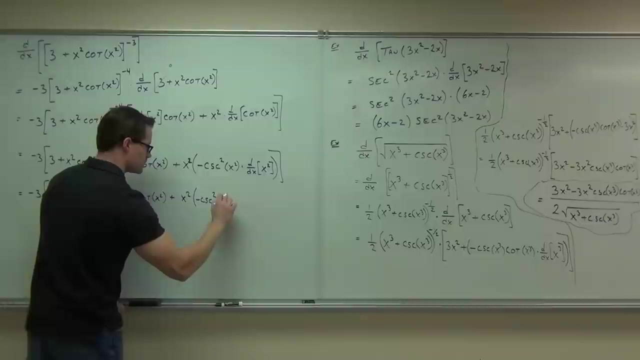 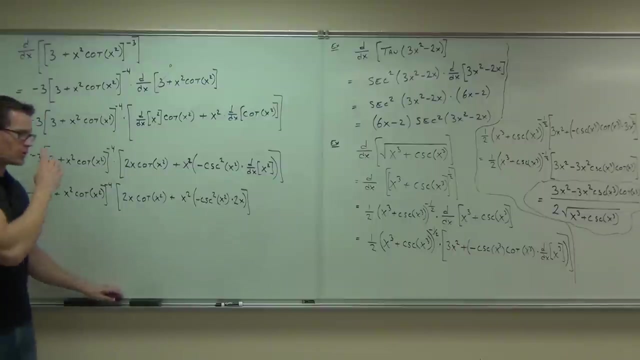 Yeah, Thank you. The last step is just to organize this little piece over here and then we're good, We're fine. Also, if you wanted to write this on the denominator of a fraction, you could do that. I'll show that to you as well. 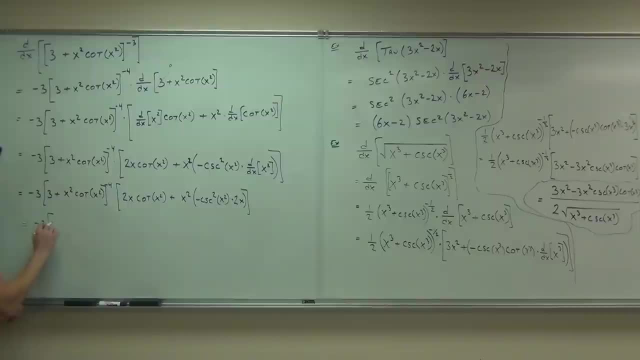 So we have negative 3, all this junk, This over here, since we have all being multiplied together, that's a negative, that's a 2x and that's an x squared- A negative, a 2x and an x squared. 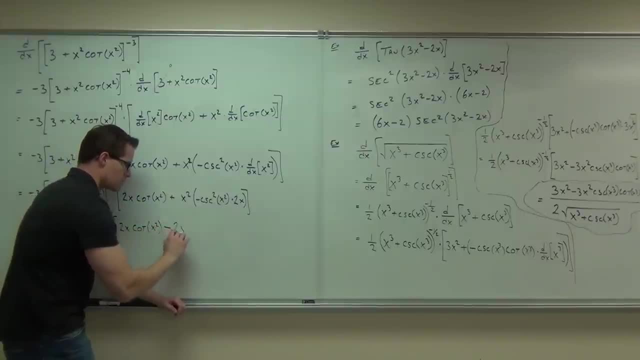 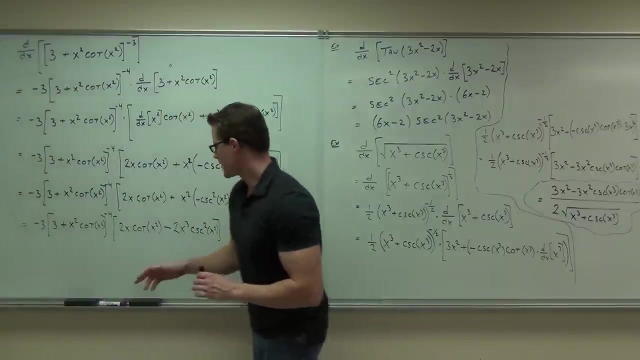 Tell me what I write. Negative 3x squared Good. Again, if you want to write this on the denominator of a fraction, you could do that. If you really wanted to get fancy, you could factor out a 2x here and a 2x here. 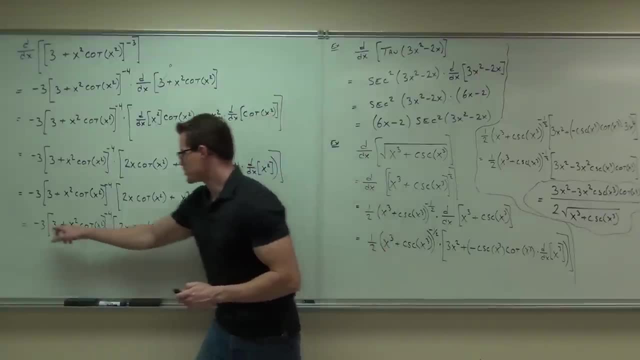 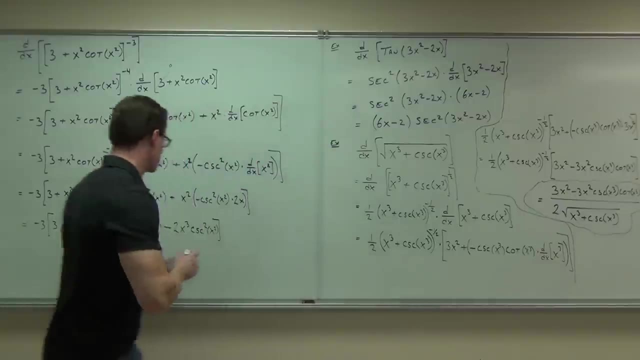 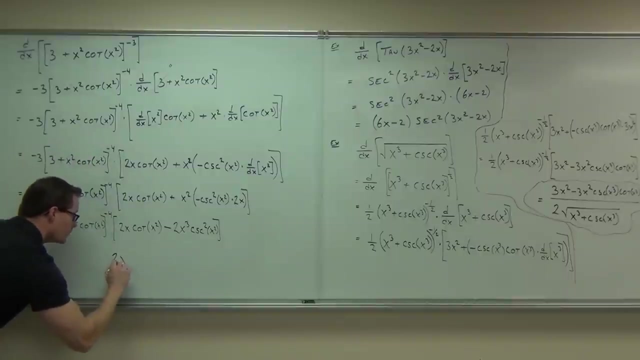 You could do that if you wanted to. You could distribute the 3 across this, but not that because of the exponent. So one last thing you might write It would be: all this stuff Times the negative 3,. that does not move, it's not associated with that negative exponent. all over that. 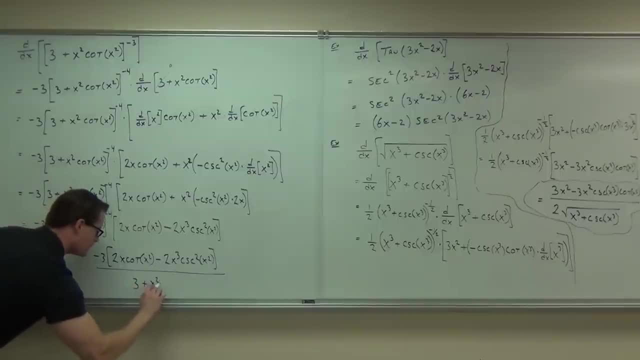 What would we be good with? just the one before it. Most cases. yeah, Actually, it depends on how I gave it to you. If I gave it to you like that with that negative exponent, it would be all over that. If I gave it to you like that with that negative exponent, like I originally did, that's fine right. 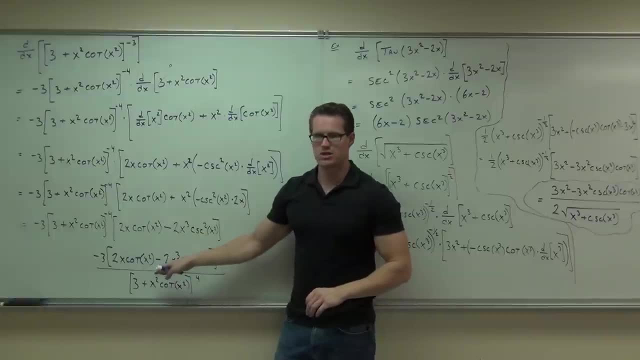 If I gave it to you like one over that I probably would expect you to go back to that So you see the pattern in it. Because if you see the pattern in it you can kind of guesstimate what these derivatives will at least look like. 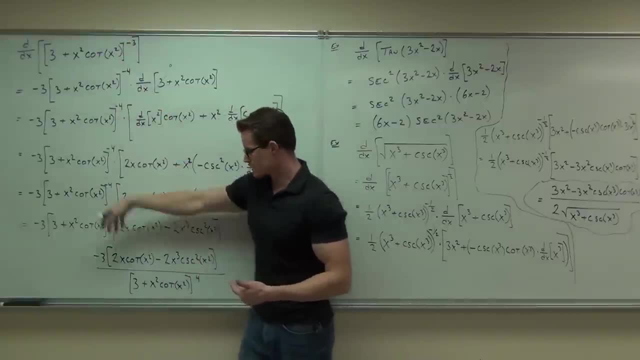 Because remember how this was one over this to the third, and now it's some crap over this to the fourth, That fourth power, and that doesn't come from nowhere and that's still right there. So you have all this junk associated with it. 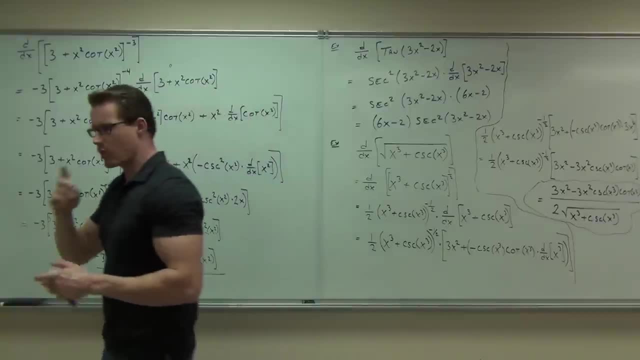 How many people feel okay with what we talked about so far? All right, We start one more. We won't get all the way through it. I have a question. Yeah, Can you factor out the 2x right there? Yes, Yeah. 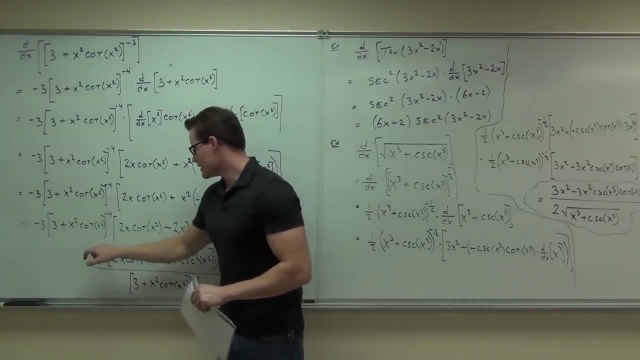 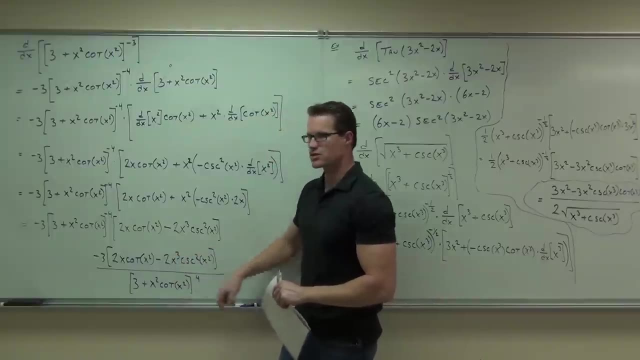 I was saying that you could factor out the 2x, This would become negative 6x. This would be cotangent x squared. This would be minus x squared, cossecant squared x squared. Okay, And you could do that. 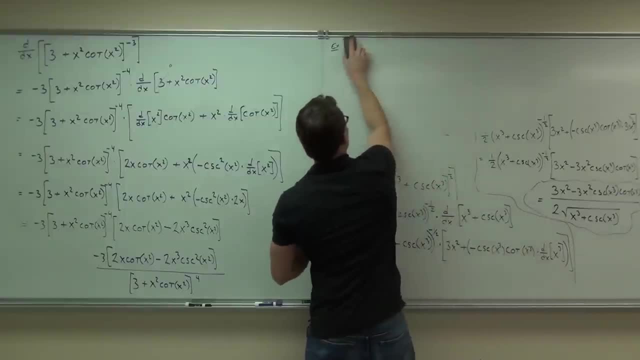 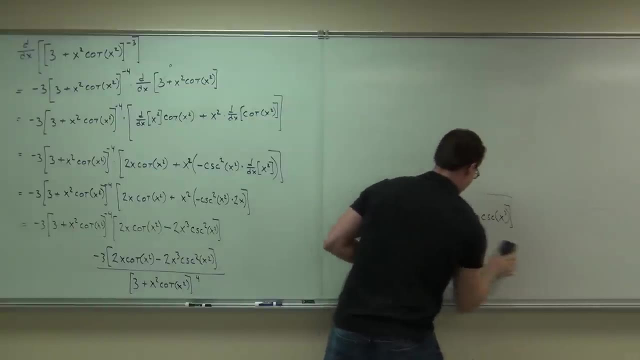 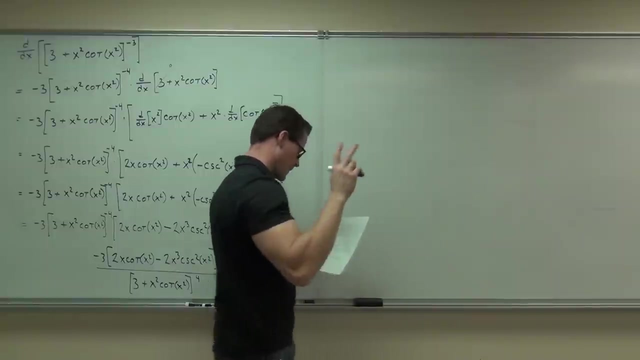 If you want to get fancy, you know, I'm just trying to survive, you know, and get parents in here. All right, Two more, Two more. Maybe we'll just you know what, we'll just talk about them. 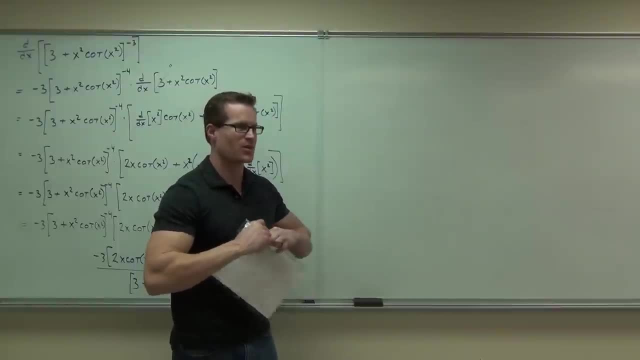 I think you've had enough. This is this is good enough. We'll we'll, I'll put them on the board, We'll talk about what they are, and then you can do them on your own. If you want answers to them, maybe I'll I'll work them out and 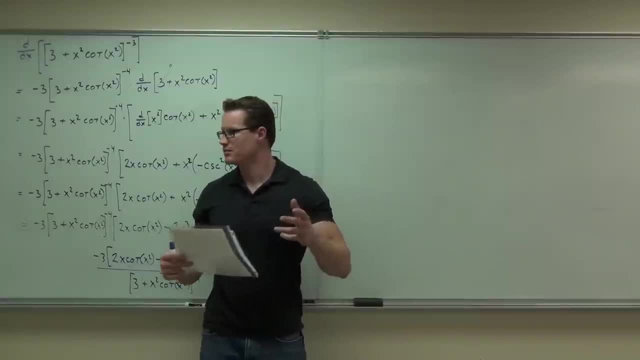 and give you answers at the very end, At the very end of this thing, just so you can. you can see it on the board. But for right now, here's the problems I'll be doing, and then I want to see if you can do them on your own. 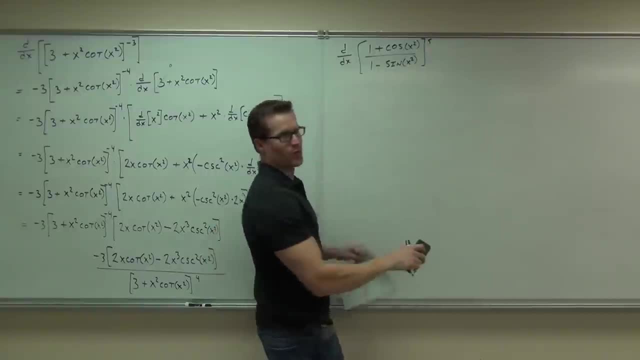 Just kidding. Just kidding, That would suck. Do you see how horrible that would be? Yeah, You could do it, though, couldn't you? Couldn't you? General power rule. General power rule. No, Closure rule, Closure rule. 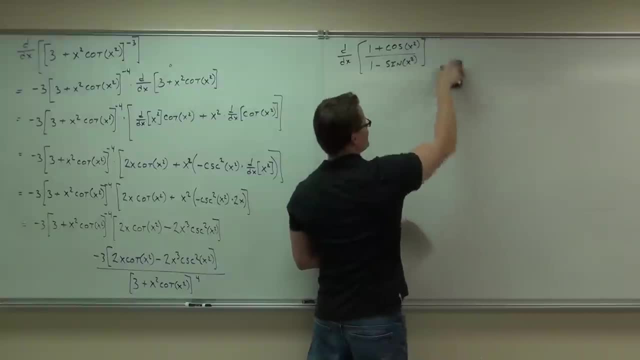 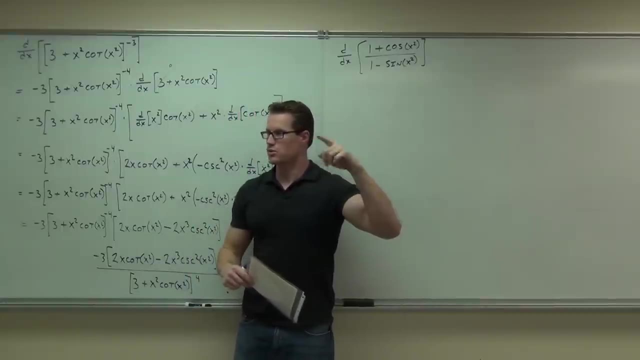 Chain rules. Okay, That would be that. Zip, Zip, Zip, Horrors. Yeah, Twice in there. What's this one? What's this one? Closure rule. Closure rule comes first. Yes, For sure, Because that encompasses the whole problem. 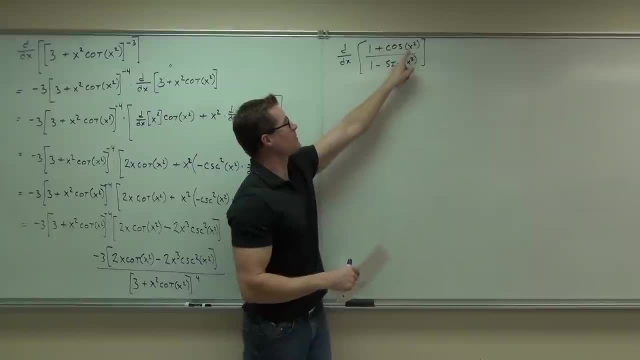 Within the closure rule. do you see the chain rules? Yeah, If you forget that, that's going to have a 2X associated and it's going to have a 2X associated. it's going to affect your problem. So this is closure rule. 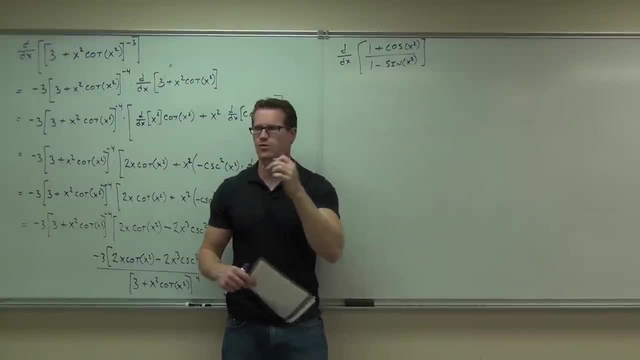 You write closure rule first. You work it piece by piece, You do the chain rule for each little piece that you come across and then you're done All over the bottom square. Remember that I'm going to work this out for you after class.